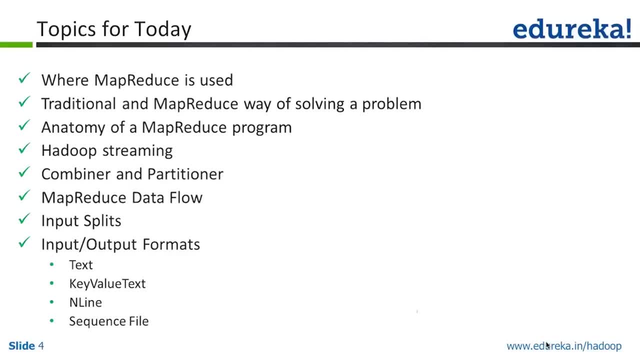 the concept of combiner and partitioner, obviously other than the map and reduce. We'll also understand the data flow. We'll understand how the inputs splits are done and then some of the input output formats. Okay, so these are the topics we're going to cover today. 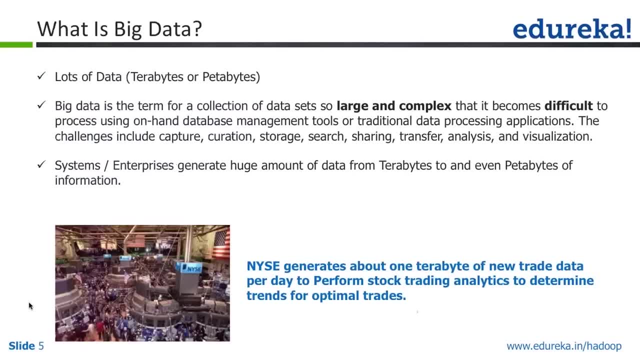 Okay, so let's get started, guys. Okay, so, what is big data? Now, I'm sure everyone has heard about big data, Everyone has done their own research on big data till now and they know So what is referred as big data. but let me also tell you what big data is according. 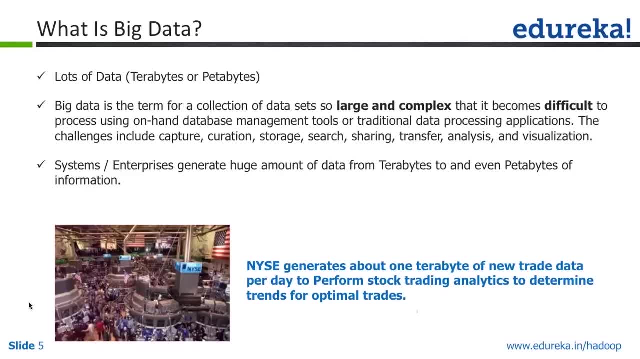 to me Now, not very different than what you've thought. It's lots and lots of data. That's what it's called. That's why it's called big. Now it is not in megabytes or gigabytes. when the data reaches terabytes and petabytes, and if the data is really large and complex in 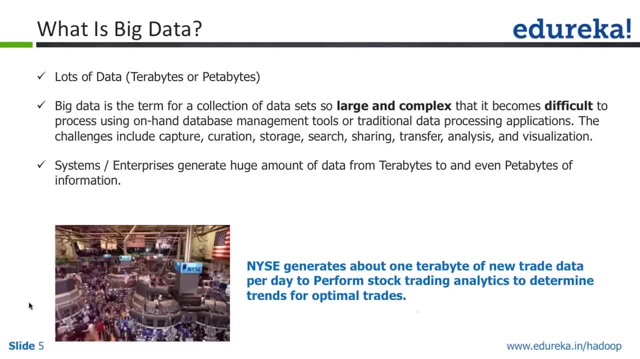 the sense that it is not just structured data. lot of unstructured and semi-structured data is called big data and there are a few differences. There are definitions associated with big data where they say that, okay, big data when you have large amount of data flowing in your system. okay, at a big speed and a big variety. 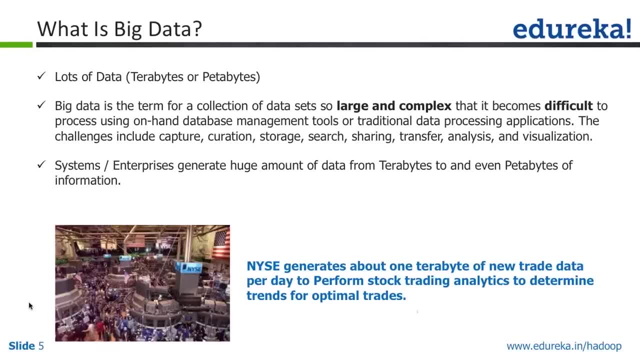 of data. data like extremes from. if you click on something like a like or a share on Facebook, that contributes to big data. large amount of videos, audios, which are shared is called is big data. The amount of data which is the kind of data which is shared in, say, from a 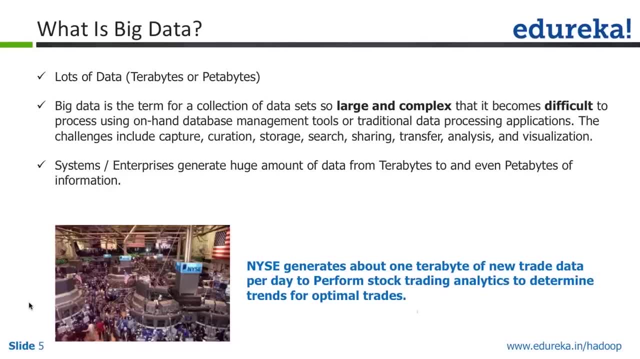 customer. I mean the amount of data, the customer data which you get, the kind of customer behavior data which you get in large organizations. that contributes to big data. Why are people so crazy about big data these days? What does big data help in? So yes, So this is basically. 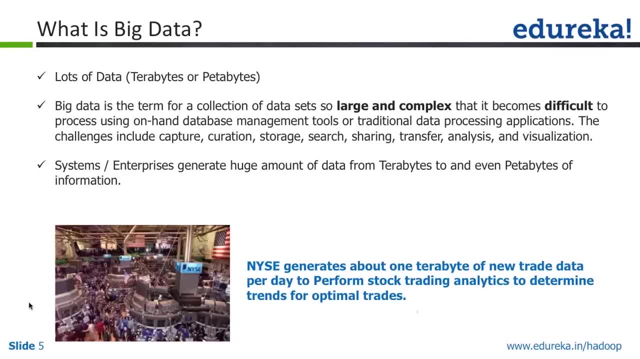 the motivation about the. everyone had a lot of data. It's not that data has come today, but there was not many ways of analyzing that data. Okay, With tools like Hadoop coming in, it has become much more easier to analyze that data Okay. 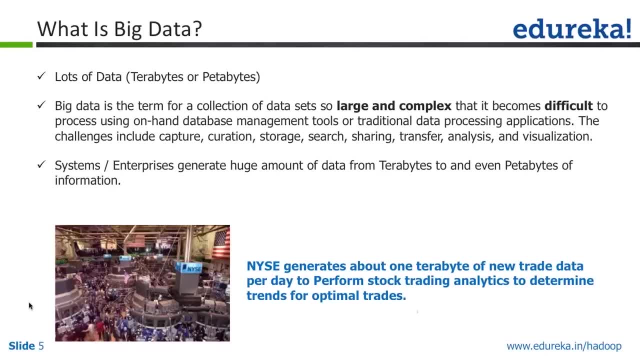 And you can do predictive analysis, You can do trend analysis, You can look at customer behavior, You can run specific campaigns for customers, You can do, say, a fraud analysis using big data. So lot of domains are finding applications there. It's all started with 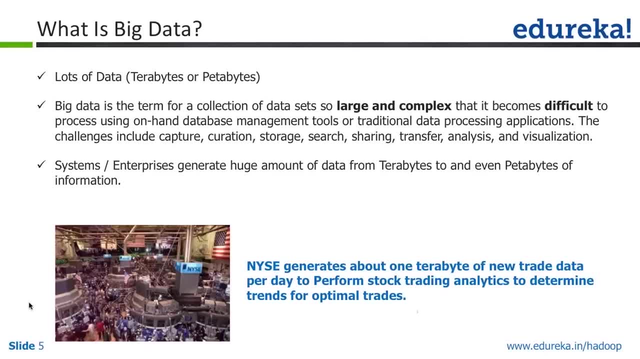 social media, but now I mean right from banks to retail. we will be looking at some examples to go I mean everywhere. people have started realizing the power of big data analytics, and we are. they are doing analytics there. So now there is an example here, which is New York Stock Exchange generates about one. 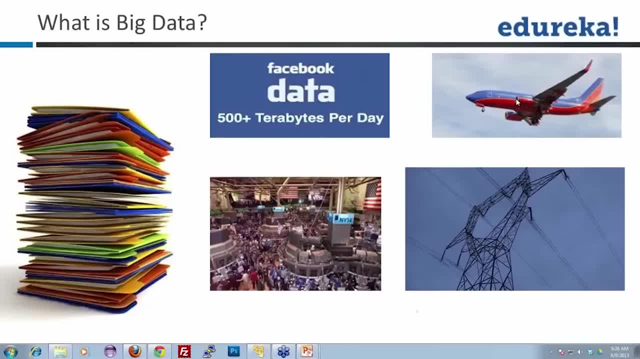 terabyte of new trade data. So what is big data? Now, the first question which comes to us is: why are we here and what is? what is big data? Can someone tell me what is? what does Facebook has to do with big data? Facebook wants to make sure that I mean. 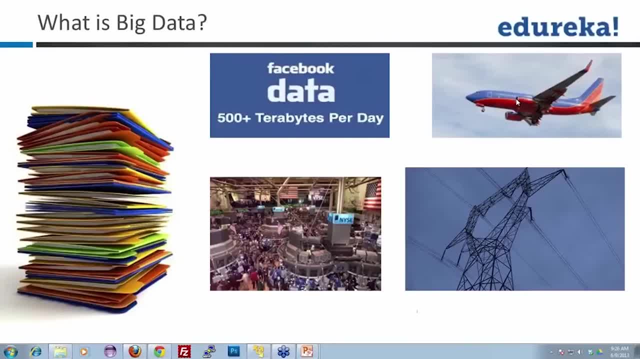 as advertisers, right Edutaker? Edutaker also advertises on Facebook. So as advertisers, we want to make sure that you, the ads, reach the right people, right, So that targeting is done based on that. So all preferences which you have, you must be seeing that. if 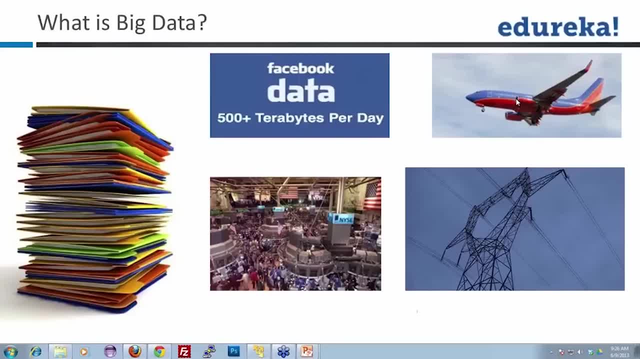 you, if you visit a site, after that you see the ads of that site all for a long time, right? So all that is done by managing that big data only Okay, Is that? is that fine, guys? So that's. that's basically a little bit about big data. We'll understand more about. 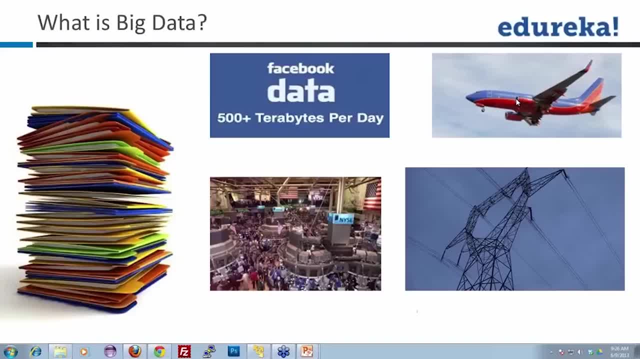 it. Now we have a picture on the right. Can anyone tell me why have we put an aeroplane here on the right? Okay, So Vinayak has given me the right answer. Vinayak tells me that system logs system logs in black box. Okay, So everyone knows what is a black box in. 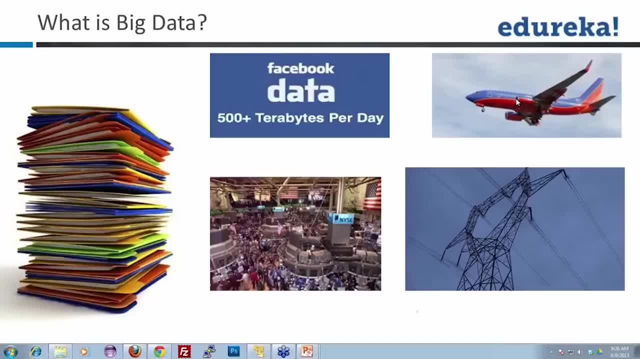 an airplane. Okay, So basically see a black box. black box is a part in an aeroplane where it will be recording everything which is happening. Okay, Whether it is flight information there, whatever system changes are happening in the 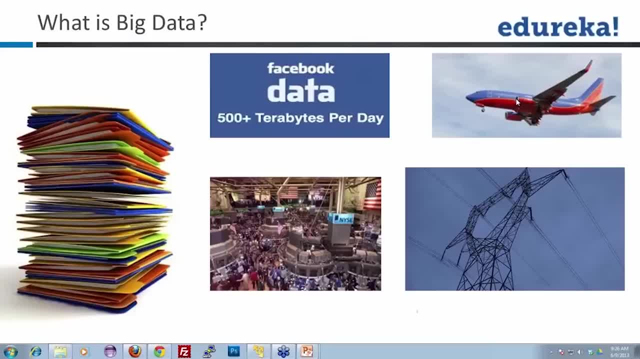 in your speed and everything will be noted down. You don't it. it stores huge amount of data in terabytes, not something which will be used every day, but in case of any eventuality, if there is an accident or a crash, then that is. that is the only part. 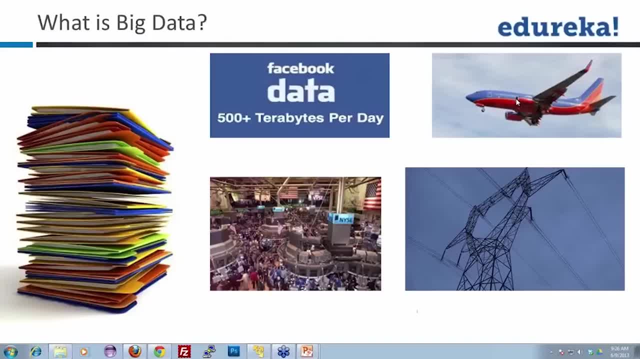 which will be looked at and they'll try to do analysis that what happened and how to avoid that in future. Okay, So that's, that's also a huge amount of unstructured data. Okay, So then we have this electricity. 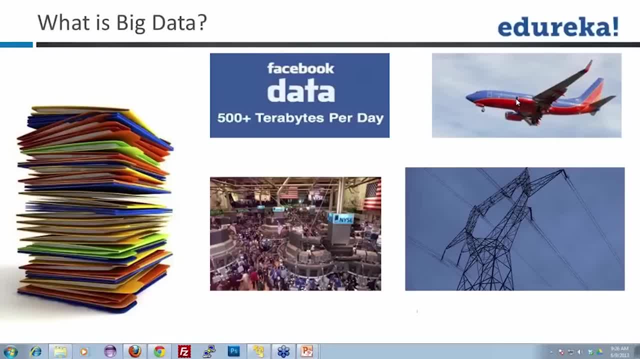 Okay, Well, let's do that thing here. grid here, Now again here in the electricity grid also, there is huge amount of I mean. you must have heard people in India suffer that a lot. Abhishek is probably not prone to that as much and he's immune to that. 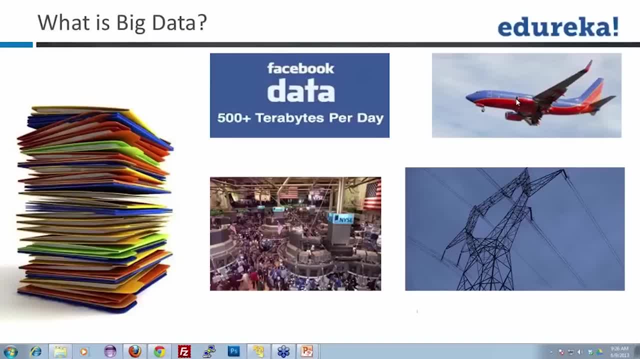 but then people in India have to face these power failures I might be teaching you in another hour- in a completely situation where it is there's no power, but hopefully so have to. there is a lot of data here as well. I mean all the nodes where substation, which 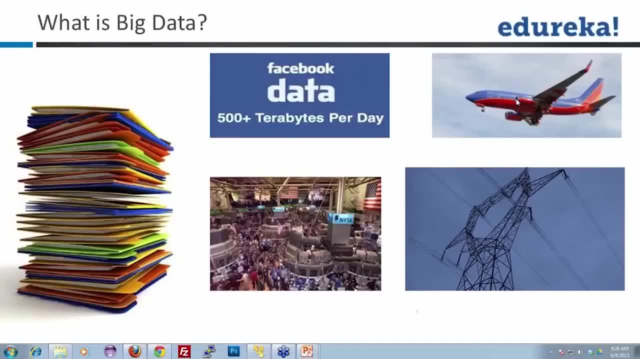 grid point where the electricity is being routed, okay, where is the consumption? so all those, all that huge amount of data, right, is something which is there, which we have to, which we have to analyze. if we analyze that properly, we will be able to probably. 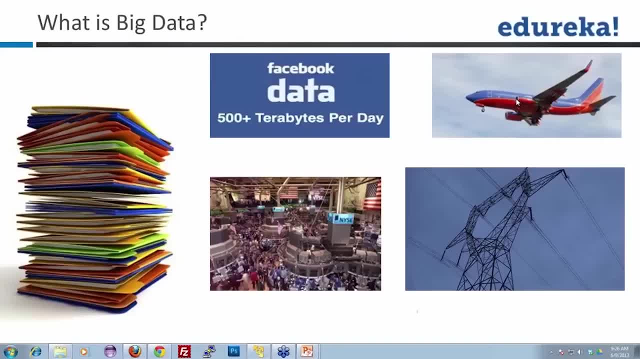 route things properly. Some people from Karnataka and Tamil Nadu here in India will be knowing right the fight which is happening all the time. right, if we could use a good level of analytics, probably a lot of things could be saved there. so that's where, in the real life, a big data analytics 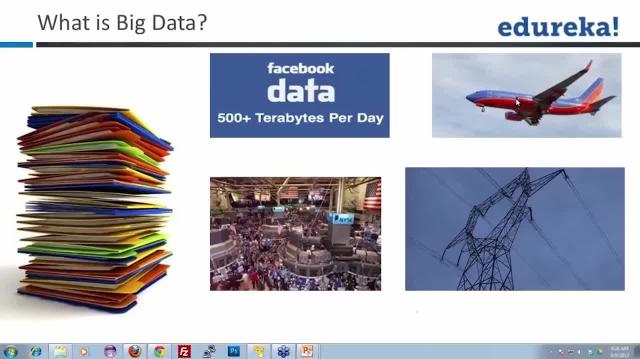 is going to help and the reason I have put all these examples here is because you will be seeing in utilities. you will be in, say, utilities. you will be using big data analytics. now the Aadhaar scheme which is there in. does everyone know about Aadhaar in India? 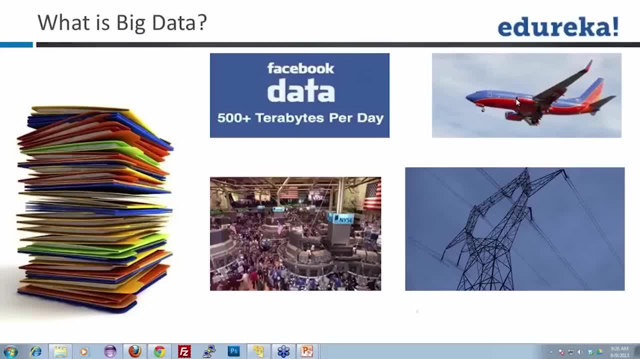 that also uses Hadoop, okay. So Abhishek Aadhaar is like a social security number thing here, which has been started in India. It's like a special biometric card, okay. so it's like a SSN for you. so there also. 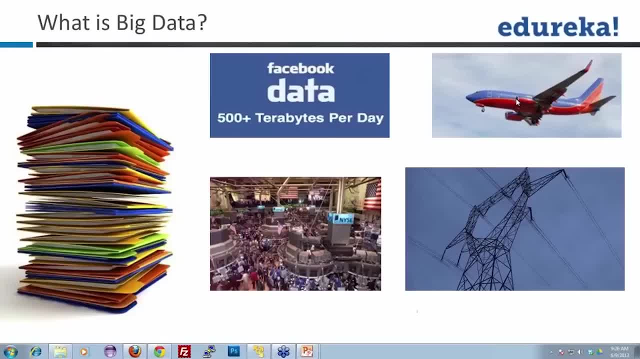 all the citizens are being mapped and I mean I am sure everyone else has looked at it and so there also we use Hadoop. okay, so you will be seeing going forward a lot of places where Hadoop will be used. it is just coming up now, and then in the next few years you 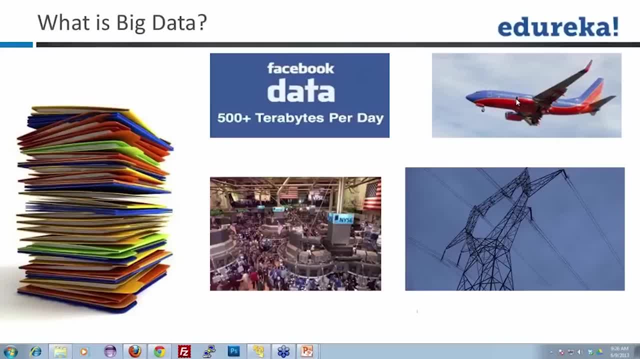 will see everywhere this application will be coming in. okay, So now on the right hand side, I have put this files here. can someone tell me why is this here Now? yes, it is unstructured data. It is physical data and government office files is what Rahul tells me, right? 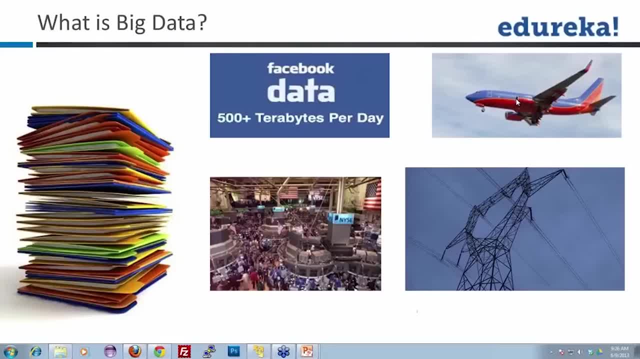 So these government office files have to be. if you could actually get them into Hadoop, a lot of things would have been solved. So now we understand. I mean a little bit of understanding, is there that what is? so now do we know the difference between unstructured and structured data? 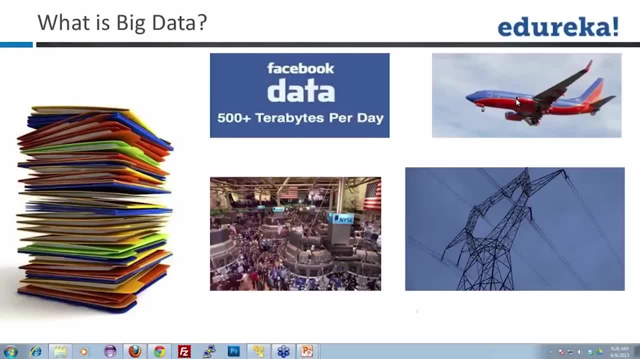 Can anyone answer that? That's very important to understand here. So what is structured and what is unstructured? Okay, Okay, So can anyone answer that question? I will obviously tell you that. Okay, So Abhishek tells me. okay, Abhishek tells me that structure is tables and columns, right? 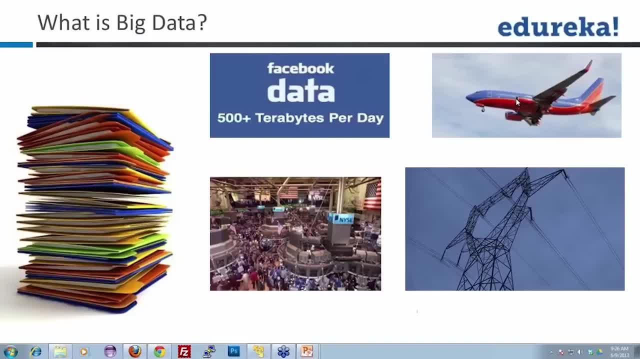 Vijay, who is? I really like your answers, Vijay. Vijay is telling the difference is un. Okay, good question, good answer. So structured isn't tables. structured could be table of format, columns and rows, right. And Vijay also tells me. now Vijay has gone a little deep. 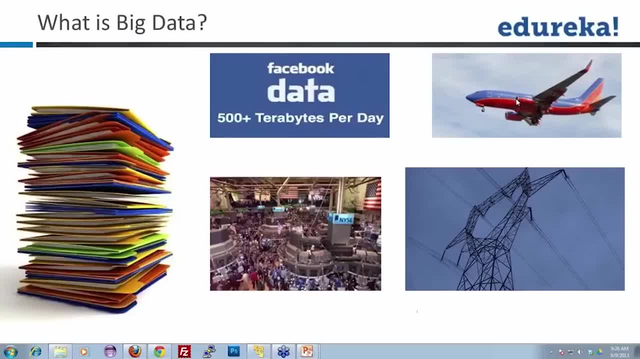 He tells me, schema. So yes, a fixed schema is something which, or a schema is something which is a characteristic of a structured data. right, very nice. This unstructured data is something which has been growing a lot in the past few years. 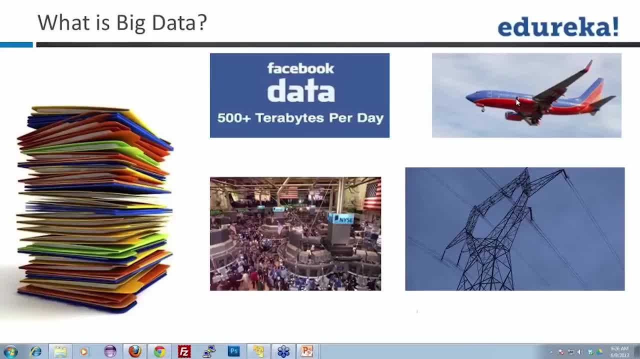 okay, In the past few years, we have seen that lot of unstructured data is being dumped by. it started with social media companies. now almost all the companies are actually getting there, Okay, So we have to analyze that, okay, And it is growing really fast. 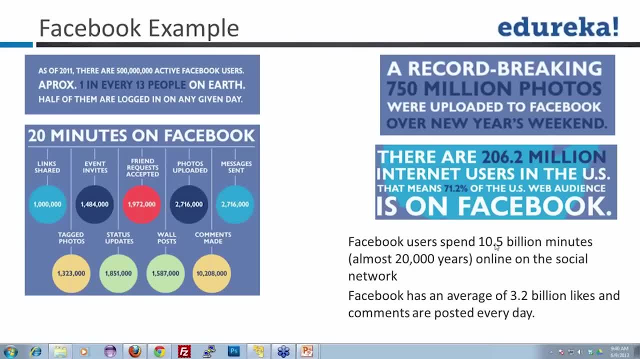 You'll see in the few slides, next few slides, how does that grow. So now, if we go forward, so this is a Facebook example where we see that, okay, there's so many people on Facebook, I don't even, I can't even read this. 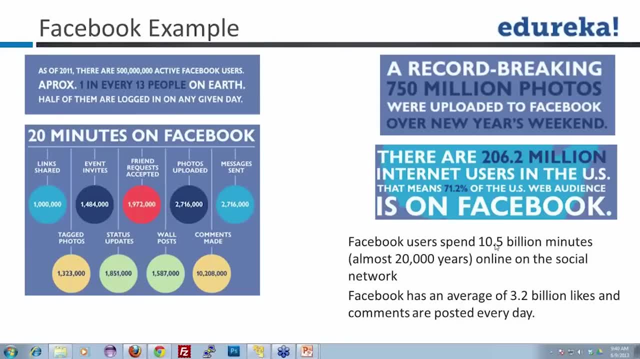 It is probably 500 million active Facebook users- okay, in 2011.. So I'm sure it will be 1 billion by now. There's so many, so one out of every 13 people on earth. I'm sure this is an old one. 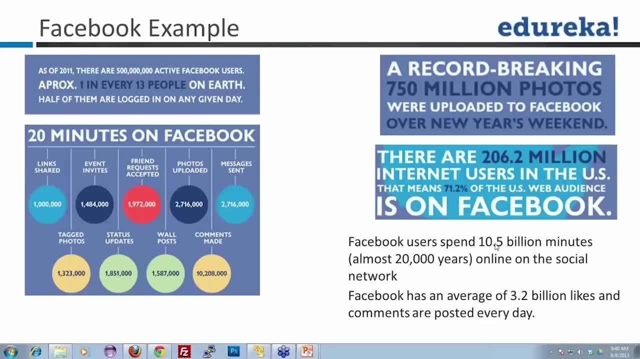 So there will be many more people. The idea is to actually give you a view on not exactly these numbers, but to just to show you that the huge amount of data which is being dumped every day, So these many links are shared every day, these many friend invites to tag photos status. 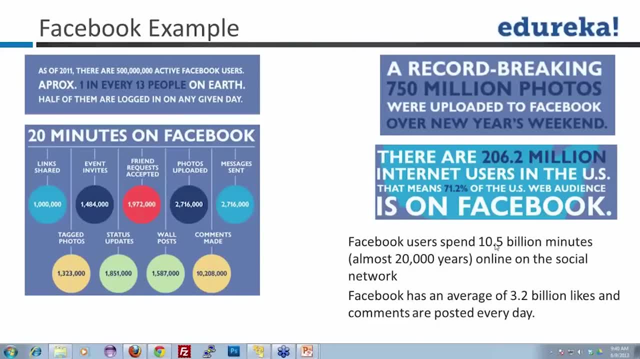 updates. Facebook has to actually do analysis of everything here, okay, And it becomes very, very difficult. We'll see what are the challenges just in a while, But here in this slide I just want to show you that okay, what these are, the this is. 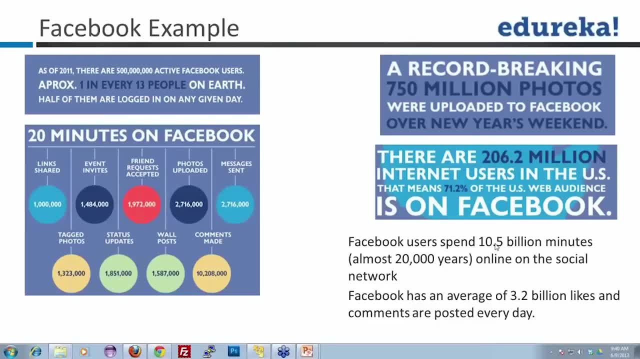 the kind of data we are using. This is the kind of data we are talking about. okay, Few years back, this was not the case. No one was actually analyzing this data. Now there are a lot of manufacturing companies in India who will be getting these this amount. 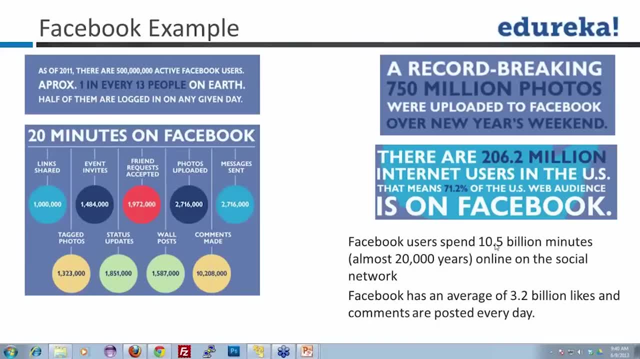 of data, but they will not be able to analyze it. okay, And therein lies the opportunity. okay, There are a lot of utility companies- oil companies, the electricity companies- who also have that data, But then analyzing that data is the challenge which every company is facing. 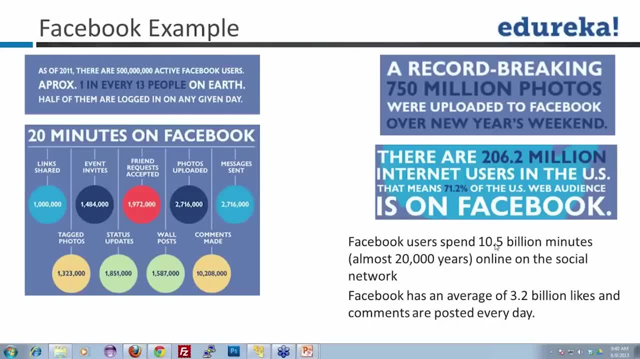 And that's where, that's why we are having this class today, right? So you get a feel of. So what is Facebook? up to right, If we go ahead, let's see another example and see what is Now Twitter- again, right? 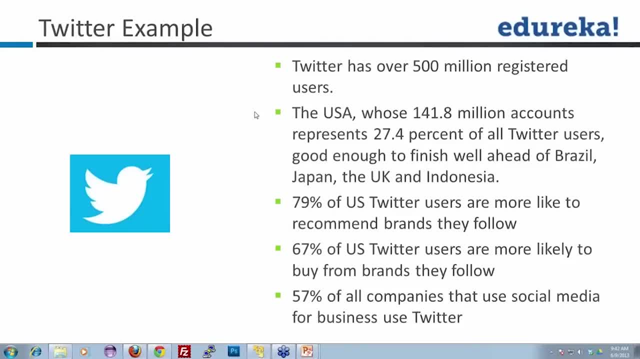 Again a social media company. So Twitter has what Twitter has: 500 million registered users. okay, In USA. I'm not a big fan of these stats, but then I mean these have been taken from some blogs. The whole idea, The crux of the matter. 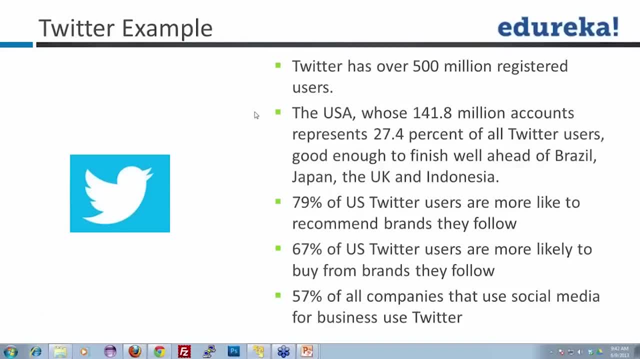 Here is the whole idea Is that a lot of people are there, lot of activities happening, and one very important thing here why we are doing all this analytics is 79% of US Twitter users are more likely to recommend brands they follow. okay, 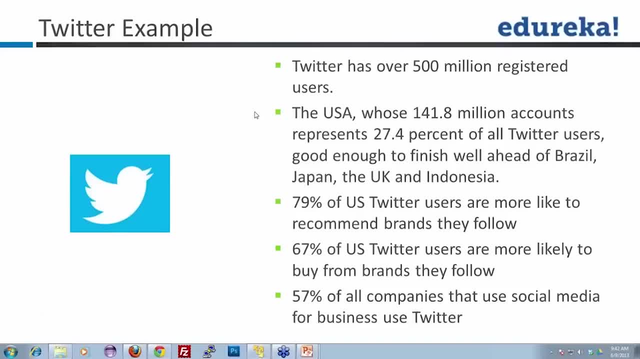 And 67% of US Twitter users are more likely to buy from brands they follow. okay, So that's the idea and that is why this is so much important. It's not just sheer fun, Facebook or Twitter. Now they're serious business. 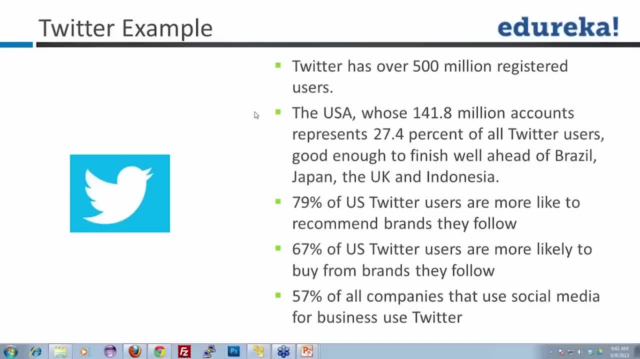 I mean, I'm sure a lot of you guys must be using Twitter and Facebook as their marketing, as the companies must be using as their marketing engines, right? So, basically, and they need to do a lot of analytics, They need to understand which users to target, whom to target, what time of the day to target. 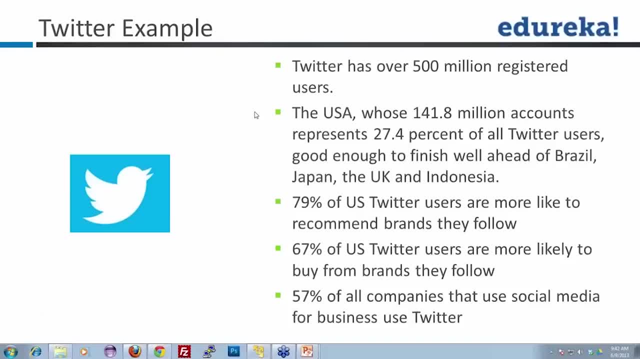 So all that analytics say, for example, if I run an ad at 4 PM in the afternoon in India time, most of the people in India will be working at that time, because that is the time anyone works, right, Okay, Okay. 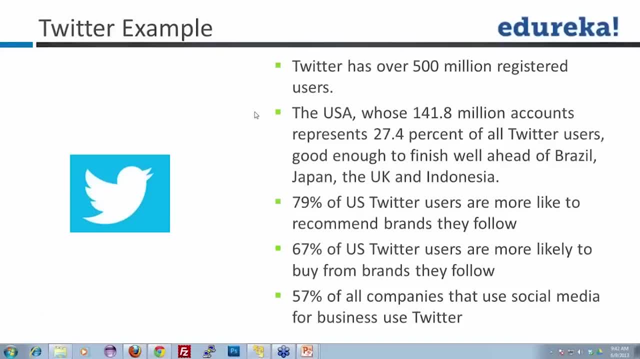 Sure, I think it is. you can use that and then, so now a lot of people. but if you target an ad at, say, for example, six o'clock in the evening, okay, a lot of people will be traveling. So it is. they may not be on their systems and that may not be a good time. 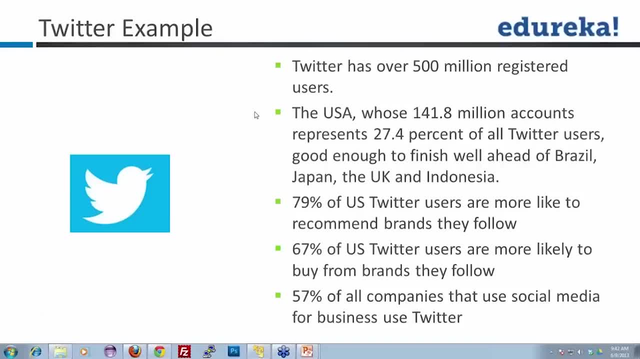 So when is a good time? which is a good time? What type of audience are available at what time? All this is the analytics which we want to do with the data which we have, right? Is that? is that clear guys? Does that make sense? and the is this? is this something which you've understood properly? 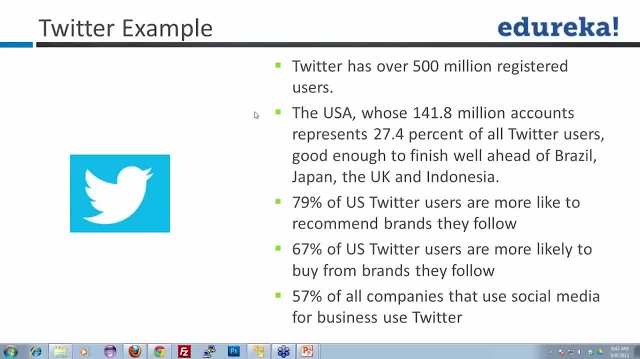 Can I quickly get a round of smileys? if everyone has understood it, or if you have any questions, I can quickly answer them as well here. Great Vikas, thank you very much. Great Thanks, Anoop. Okay, So I understand. everyone has got the idea. two things which I wanted to make clear from. 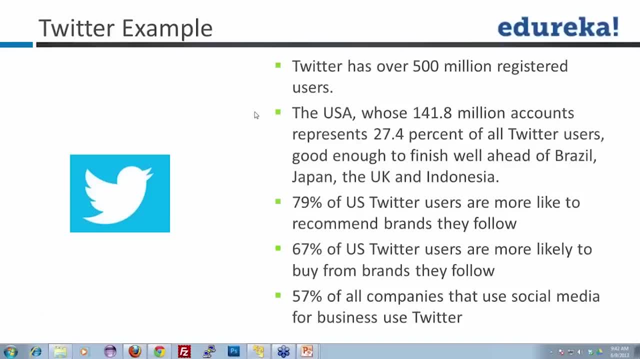 last few slides was that one: the rise of unstructured data, the difference between structured and unstructured data, The kind of industries where it is applicable and where it is happening, the dumping of the data. Okay, And some examples of the companies which are actually doing big data analytics and they 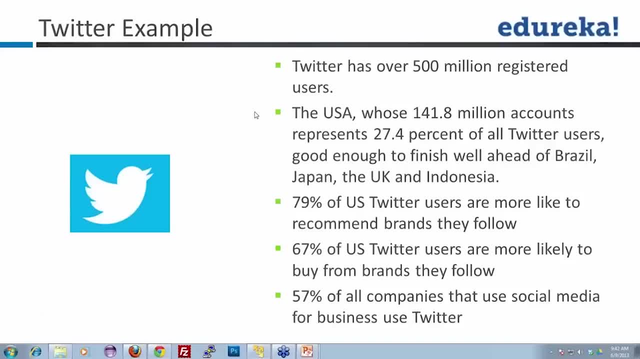 are successful. Okay, So Facebook and Twitter are two such companies, right? So, if that, if that is something which you've understood, we are. that is all I wanted to convey from these foils. Okay, The numbers. exact number: it is 79% or 67%, that is for I don't know which exam we'll. 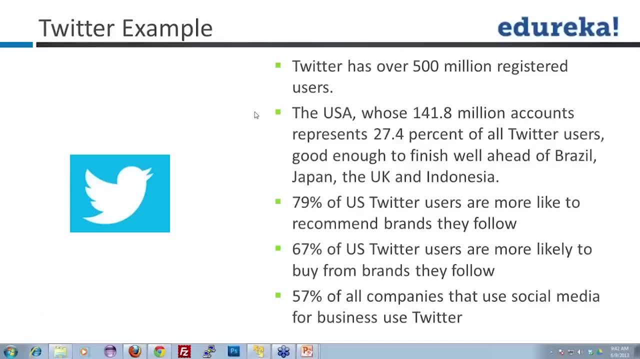 ask you. if they ask you don't answer that question, Ignore it. I don't want to answer that you. if you've got the idea right, Okay, So let Okay. Very good question. Is Hadoop only for unstructured data? 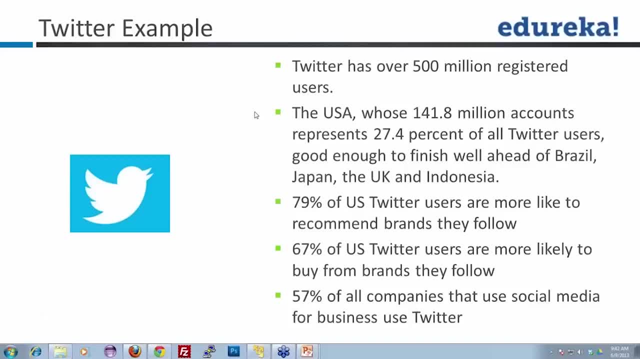 Does it also work on structured data is what Abhishek has asked me. Now, Abhishek, for unstructured data, largely Hadoop is used and HDFS is used. there's something called HBase in Hadoop. we will come to that later. it we do analytics on structured data. 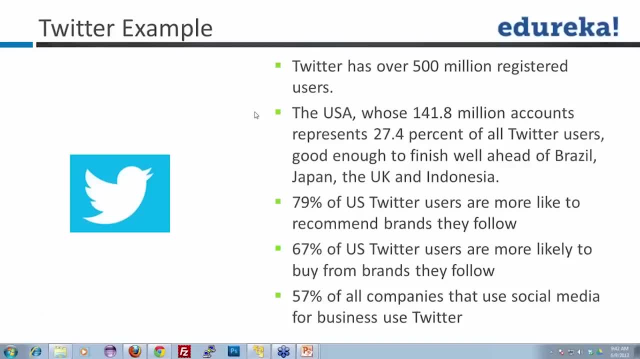 as well Going forward. there will be a time when all side of data could be analyzed using Hadoop. Okay, It started for unstructured data. Okay, Is that clear? everyone And Abhishek, Great. So the whole idea is, if we can distribute things, okay, and I'll tell you why it is. 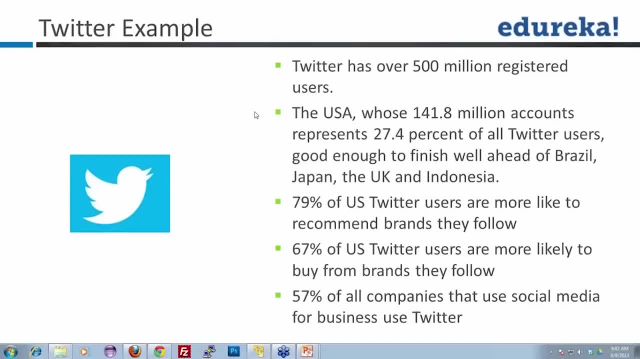 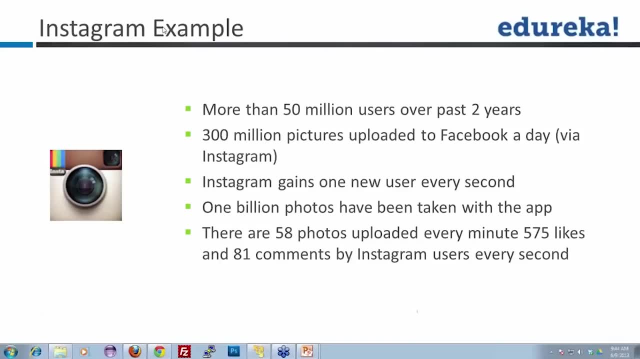 required in just a short while. in just a short while. Okay, Great Shyam, Thank you very much. Okay, Now let's go. let's move ahead. Everyone knows Instagram. Is there someone who doesn't know Instagram? Okay, 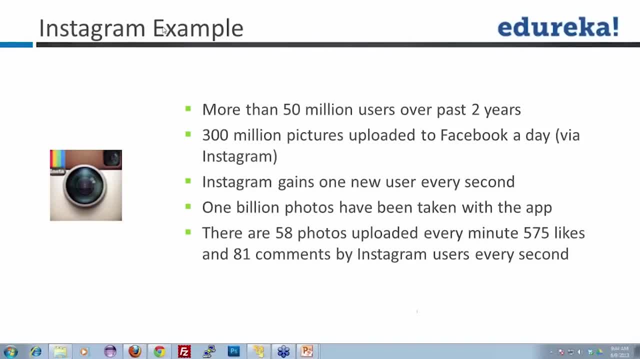 So Instagram? I mean Instagram is one of the big successes of the social media time- and I mean it's an app. it's an app which takes pictures and the difference is just: can someone tell me what is the difference between, say, a Facebook picture, click and share, and between Instagram picture, click and share? 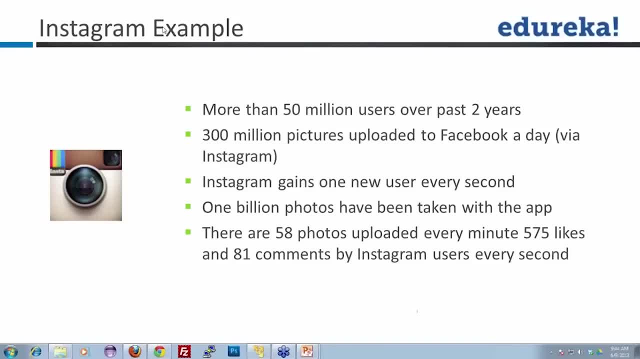 anyone who has, who knows that, who has been using Instagram, while others can read through this slide and see Instagram grains. Okay, Instagram grains. one new user every second. Okay, Instagram was sold to Facebook, probably for a billion dollars, Right. 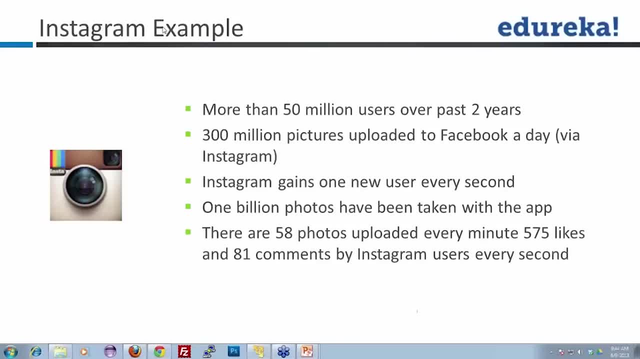 So Puneet tells me it has image filters, Right? So something that you could do in Photoshop earlier, and some of that part can add effects in Instagram, Right? So that was just a small innovation with Instagram and it became an instant hit on internet. 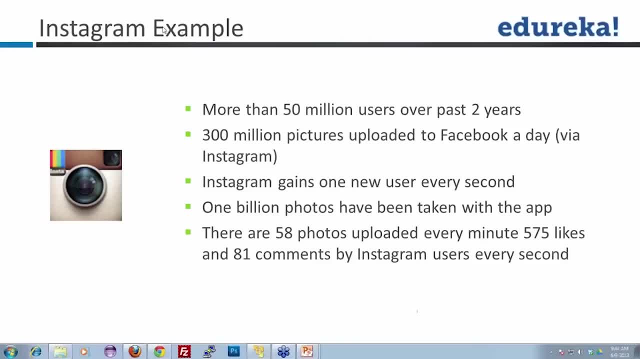 Okay, So that's, and then so much, so many, one billion photos have been taken with Instagram. So you can imagine the kind of data which Instagram has, Okay, The kind of data which Instagram has to handle And with those, all those effects and filters it is, it becomes huge right. 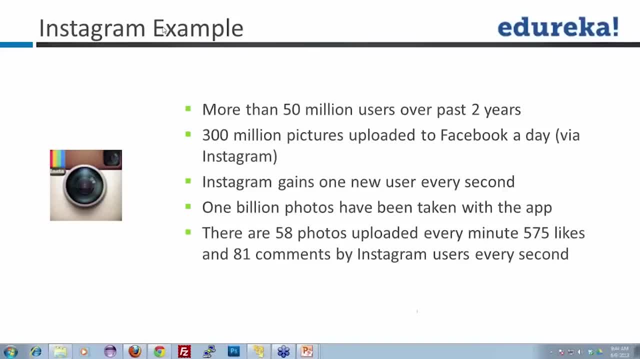 So that's, that's again one company which will be using a lot of big data analytics. Okay, And there are many more such companies. We will come to that as well. We'll, we'll know And I'll also tell you a link from where you can go and read what all companies are using. 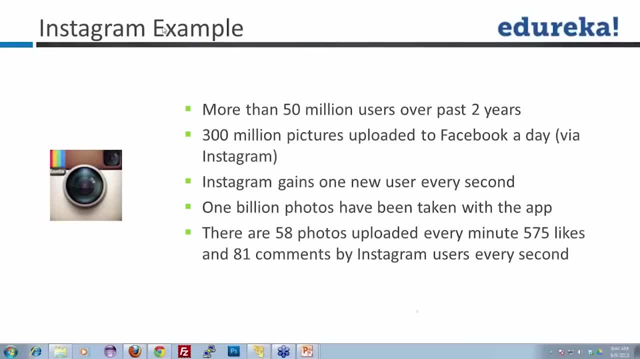 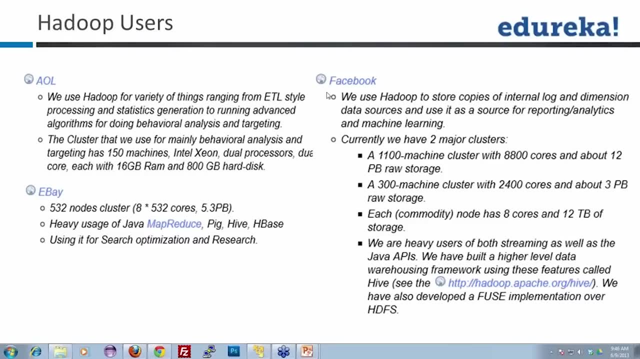 Hadoop, and what do they do with Hadoop? What is their cluster size? All that information is also available in public domain. Okay, Now, this is there's one. there's one slide which actually tells you about that. There's AOL. 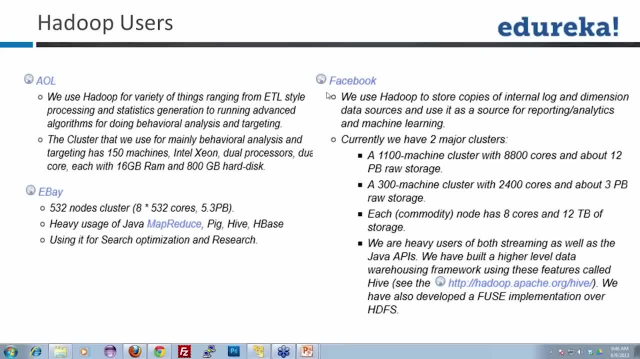 There's eBay, The. they use for different, different reasons, reasons. I mean I want you to actually go through this. I'll, I'll, I'll share a link with you, A Facebook, for example. let's, let's talk about Facebook. 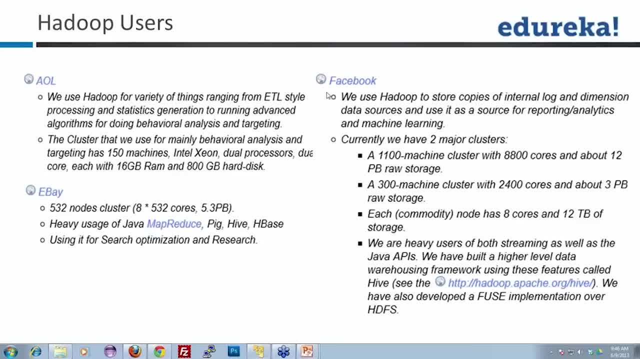 Okay, Facebook uses a Hadoop to store copies of data. Okay, And they do machine learning as well. So I'll tell you a little bit about machine learning in just a while, but not in detail Now. it has 1100 machine cluster with these many cores, right? 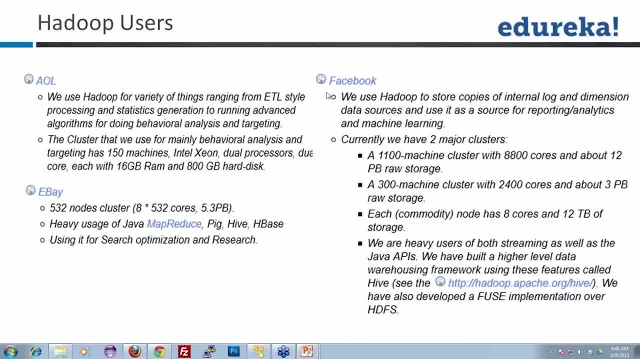 So each commodity, node, commodity. what is commodity is something which you should think about right now. I'll tell you just in a while. Okay, So they use eight core and 12 TB of storage on each machine. Okay, So this is. this is the. this is a typical data node in I'm using the term data node. 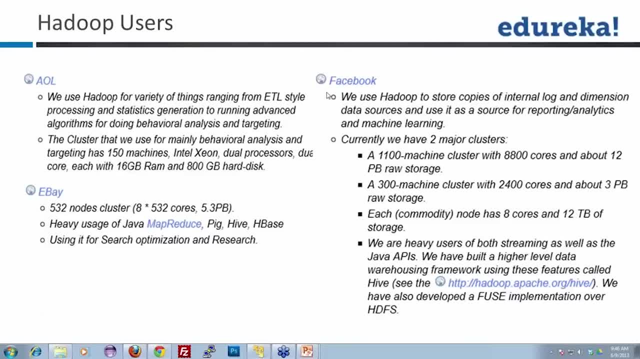 I'm just using the liberty of using the term data node. I'll explain that in a while. Okay, So has eight cores and 12 TB of storage. Okay, This is the storage capacity of each node there in the cluster. It has a 300 machine cluster with this, this kind of thing, right? 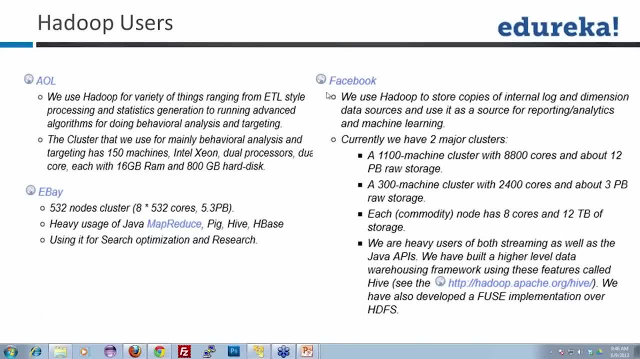 So basically, and then we have eBay, which has a five to 32 node cluster. Okay, Heavy use of Java, MapReduce. So MapReduce is the programming model, that big high wedge base. All these tools, guys, we learn in this course. 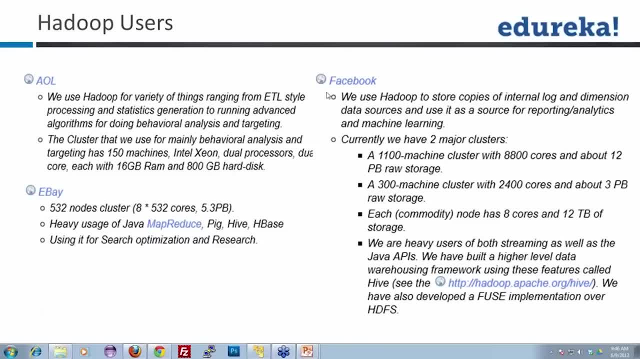 Okay. So if you, if you understand this well, you will surely have options to moving into any any of these companies. Now, eBay uses for search optimization and research. Okay, Now on eBay. if you go, if you go to eBay and if you look for some product, okay, there'll. 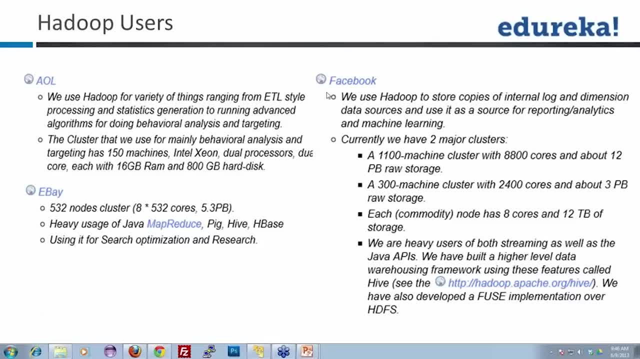 be thousands and lakhs of products there. different search they should be. you should be able to search them on various terms. So that is where Hadoop is used there. Okay, Let's move ahead. Anyone has a question here, And shall I move ahead? 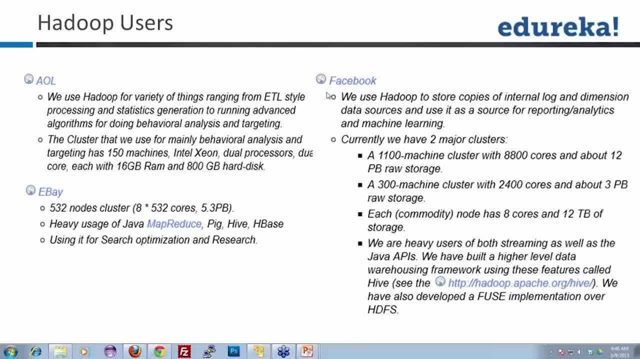 If, if this is clear- quickly can you can. can you quickly? Okay, Let's move ahead. Okay, Can you say yes or no? Okay, Hadoop tells me yes. If no, I mean it's okay. 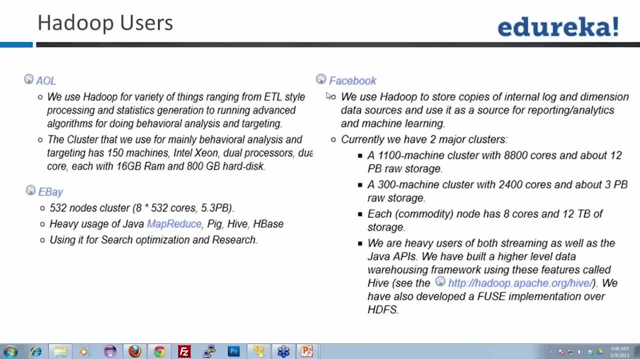 If you don't write, I'll assume that we can move ahead. Okay, Hello, Don't let you type. Sometimes I'll force you to type so that you are not sleeping. Okay, Just to make sure that you're not sleeping. 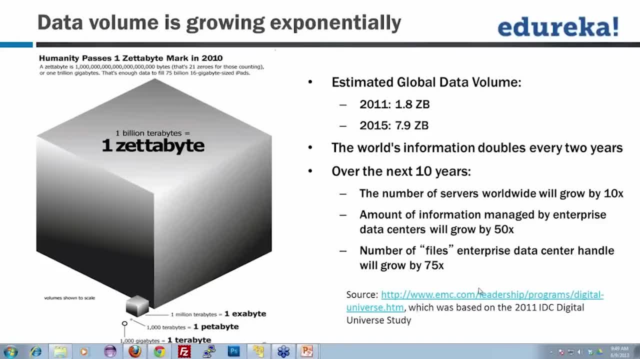 Okay, Okay, Now we have this data volume growing exponentially. Now, what? what does this mean? Okay, Now we've we've been seeing, we've been talking about a lot of companies till now. Now, this is one, one infographic. 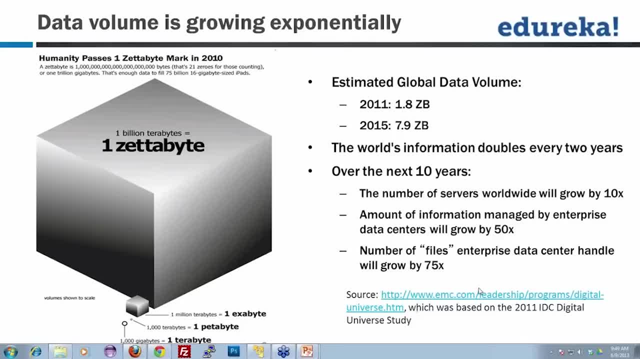 It has been taken from EMC. Okay, So EMC here, which shows the amount of data which is growing. now one terabyte is here. Okay, So this is one terabyte of data. What we're talking about are zettabytes of data. 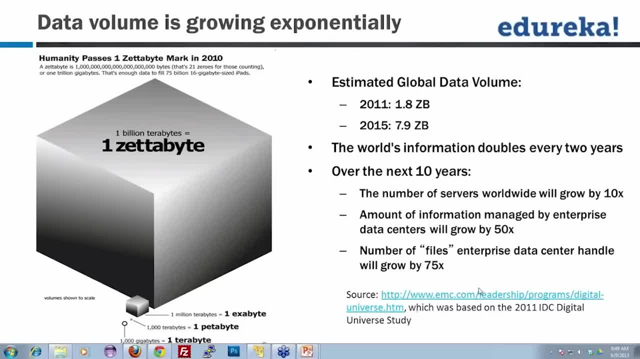 Okay, Which is 1 million, 1 billion terabytes. Now some estimates said that to 1.8 zettabyte will be there. These are again old slides. So I mean the whole idea is not to know these exact numbers, but to understand the amount. 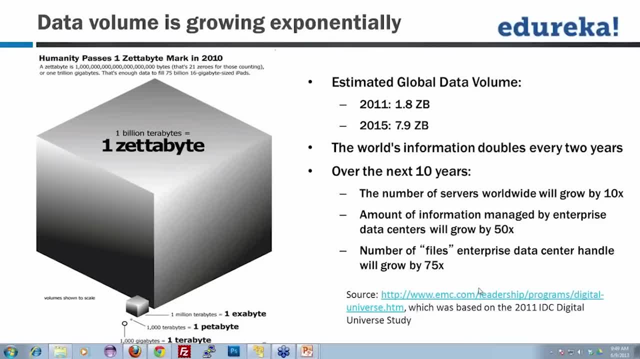 of data which we're talking about, And this is very important. The world's information doubles every two years. Okay, In the next 10 years, this is the opportunity. So this is where the opportunity lies Now. all of us who are working in this big data domain- and a lot of you will be working- 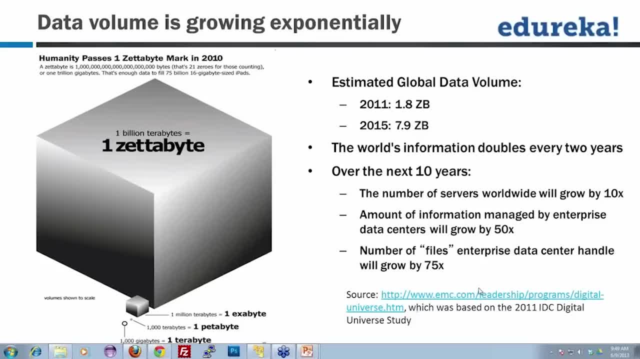 on that going forward. whether you like it or not, you- most of the people here in India, as well as in the U? S- will be working with big data in some form or the other in the next five to six years. Okay, 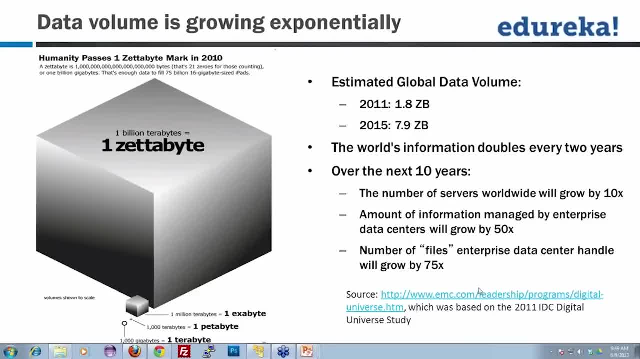 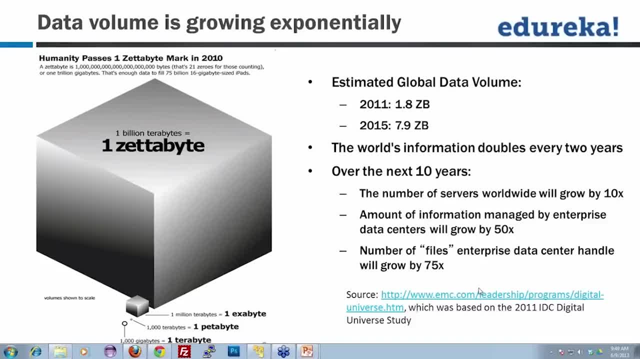 how it's going to grow, and everyone will be a part of this revolution. Big data analytics will be a part of it, whether you like or you don't like it. So it's better to actually understand things now and and be early adopters there of this. 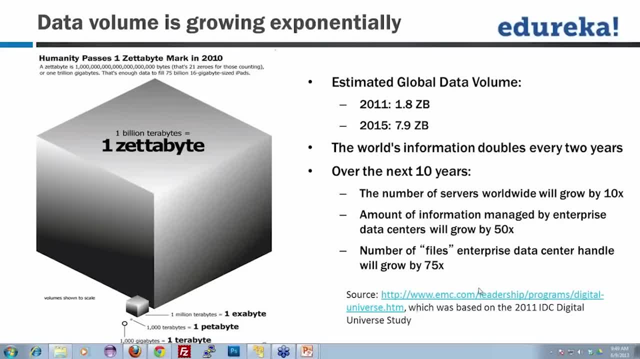 technology. Okay, Great, So, yeah, So Narayan has told me yes, sure, And I think I lost the chat window. No one has said yes, Okay, Sorry, Okay, So guys. So this: Okay, Anyone has a question here or I'll I'll move ahead. 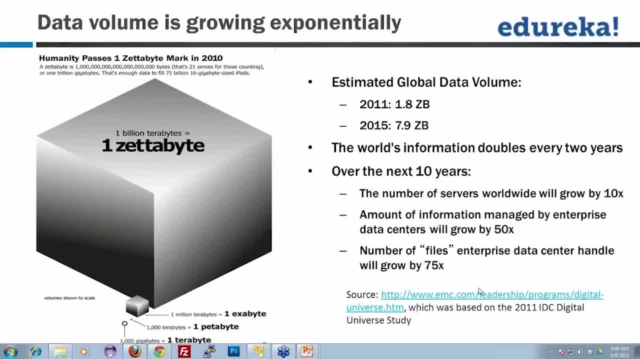 So basically, till that, till this time, I just tell them, just rephrase, and I'll make sure that everyone understands: We talked about unstructured data, right? We talked about the different companies which may be using the unstructured data that we. 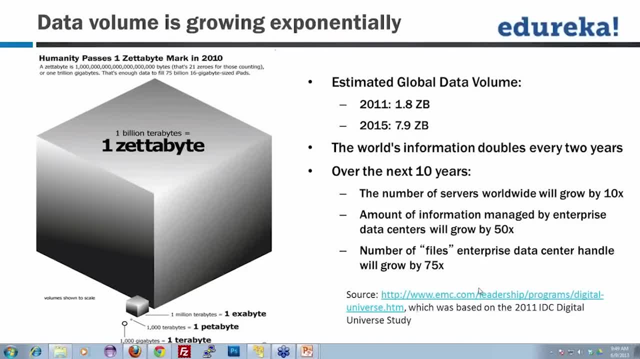 also talked about some of the companies who, which actually went very- become became very successful using big data analytics. Okay, And we also showed you how the data volume is growing. now There's another infographic and after that we'll move on to why Hadoop. 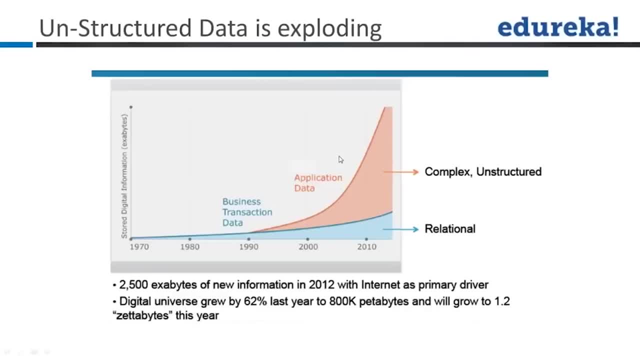 Okay, This is. this is important again. Okay, Now Vikas is asking me a question. Can we? we can use Hadoop for structured data as well. Well, Vikas, the same question was asked just a while back by Abhishek. 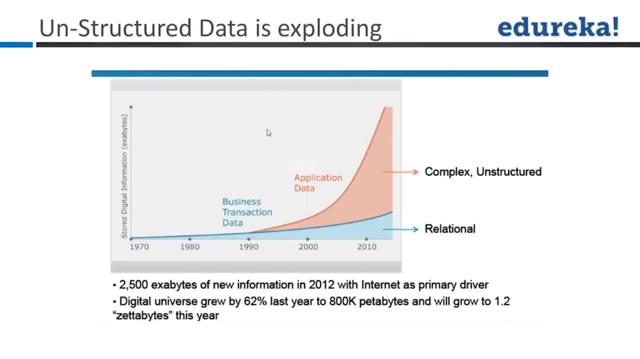 Yes, you can. Yes, you can. There are some limitations, but you can. Okay, And we will. HBase is the component of Hadoop which is used to store structured data. Okay, Now, that's. that's not really completely like your relational database. 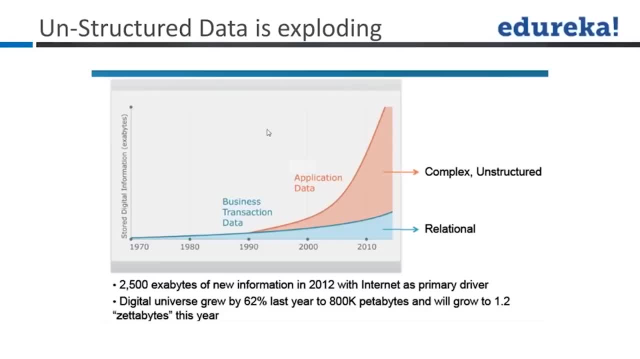 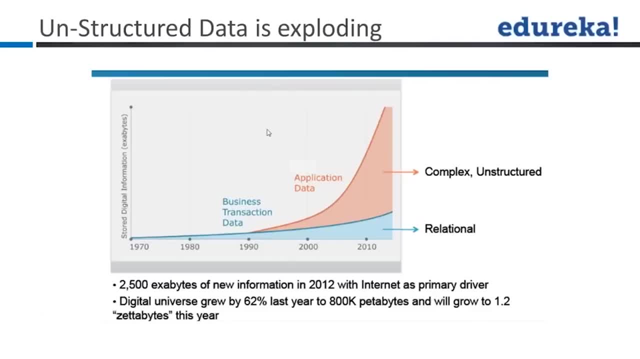 We're going to use HBase. We're going to use HBase. We're going to use HBase. Okay, So HBase is the component of Hadoop which is used to store structured data. Okay, Now, that's. that's not really completely like your relational database. 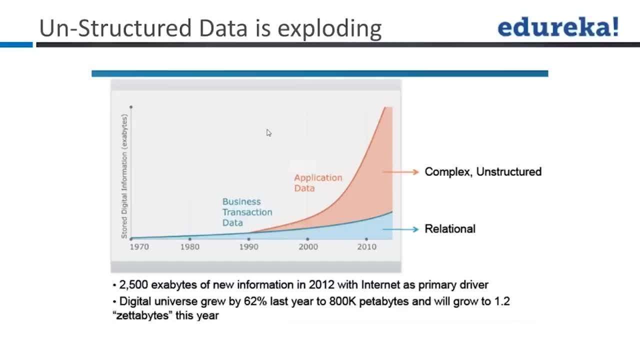 It is. it's a different kind of database. We will be talking about it when we reach HBase. But yes, that's true, You can. you can use it, Okay, And as we go ahead, in a year or two you will see that there will be provisions where you. 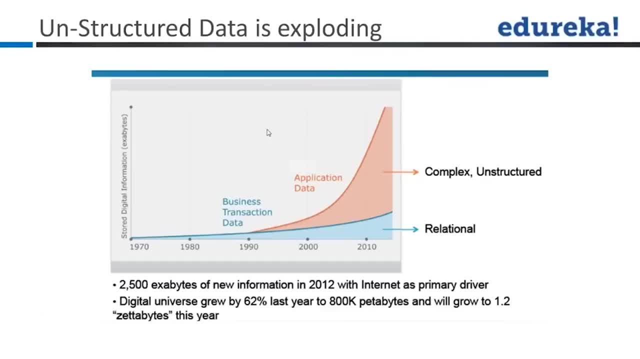 can completely replace your MySQL with a Hadoop kind of thing. People are working on that, Okay. Now this, this graphic shows you how the how the overlap has happened, So you can see that HBase has been replaced. You will see that there will be provisions where you can completely replace your MySQL. 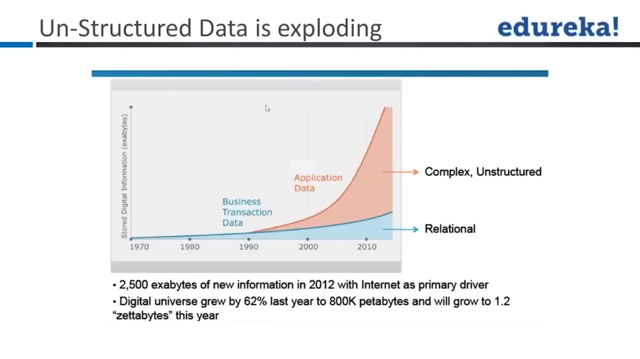 with a Hadoop kind of thing. People are working on that. Okay, Now this, this graphic shows you how the how the overlap has happened between structured and unstructured data. So in the times of when Shah Rukh Khan came in or Mene Behar Kiya came in in 90s, there. 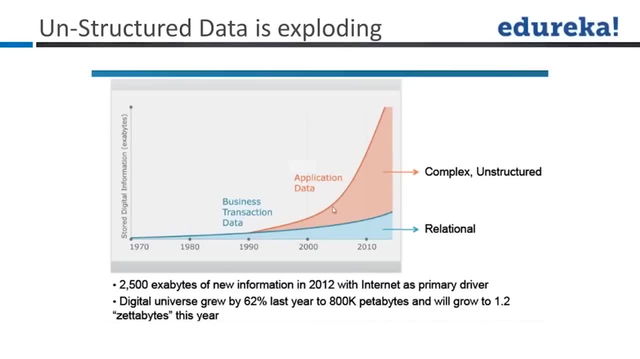 was no unstructured data. Okay, It's only after that that unstructured data grew. And the age of Ranbir Kapoor. this is the situation. Okay, So now? and relational database? Okay, Relational databases are I mean relational data or structured data. that that's it's. 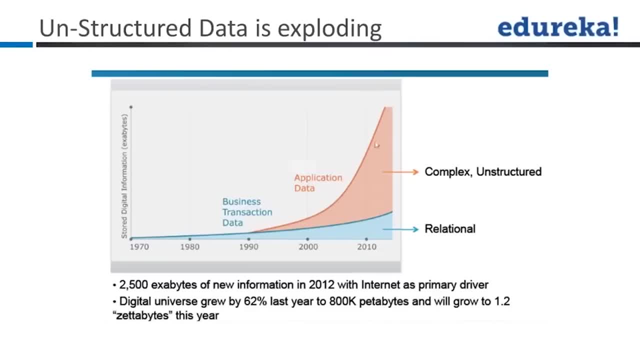 see. the fact is that this data is also growing, But the speed at which this data is growing is something which is phenomenal, and that is where the challenge is and that is where the opportunity is Okay, So let's, let's move ahead if, if, everyone is fine here and let's see a few more things. 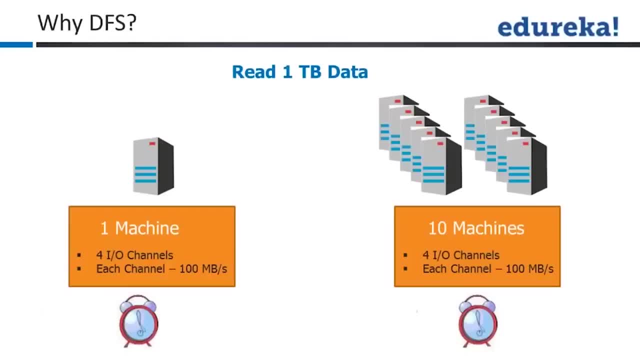 We'll do a small exercise also now. Okay, So now we've seen that huge amount of data is being stored. Okay, Now the challenge challenge here. The challenge challenge probably, I mean, is not the storage. You have storage capacities of, scaled up beautifully right. 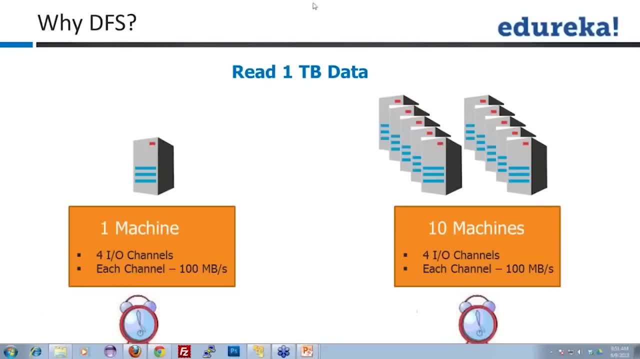 The challenge is something else, And let's try to see what that something else is. If you've seen this slide presentation earlier then, then probably this is a very easy question to answer, But still, I want everyone of you to actually answer this. 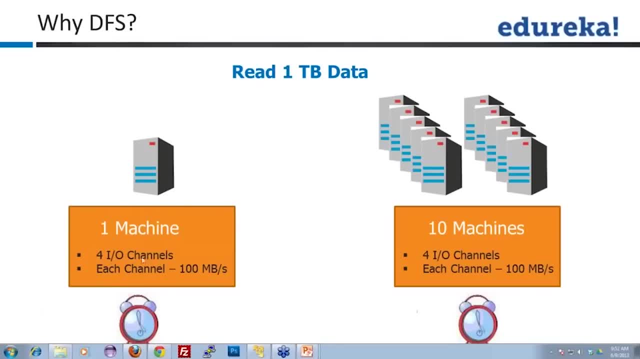 We have this one, one machine here with which has four IO channels. Each channel can run a hundred, can do a hundred MBPS of input and output. How much time will it take to do a one terabyte of transfer? Can someone tell me that? 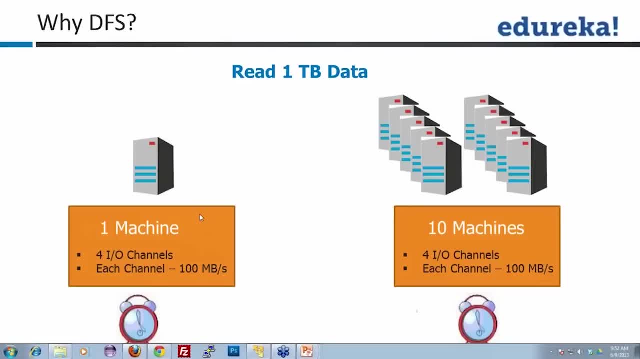 Can everyone tell me that I'll give you, say, 30, 40 seconds to calculate that? Okay, Abhishek has given me an answer. Okay, Vinayak has given me an answer. Tell me. okay, guys, when you write this answer, also tell me if you've seen this earlier or. 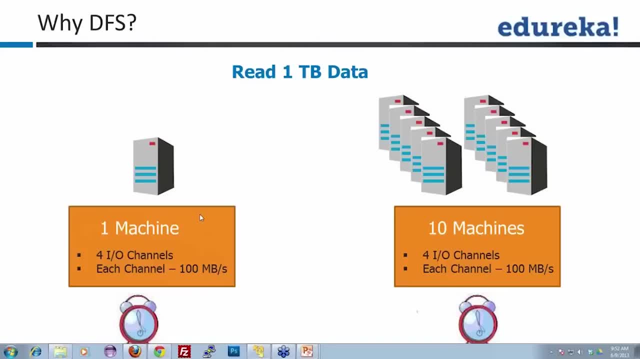 or not. Okay, If you're calculating here, Okay, Everyone is getting giving me good answers. Okay, Everyone is getting good, right answers. The first time I'll tell you guys for the first time when I when I showed this thing. 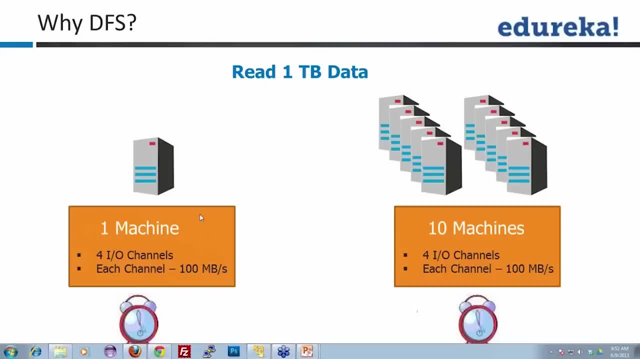 okay, no one actually answered this question right. The few people did, And you'll also have to tell me how. how did you calculate this? So I won't answer from everyone. Anoop, Vikas, Vikas. everyone has to answer this. 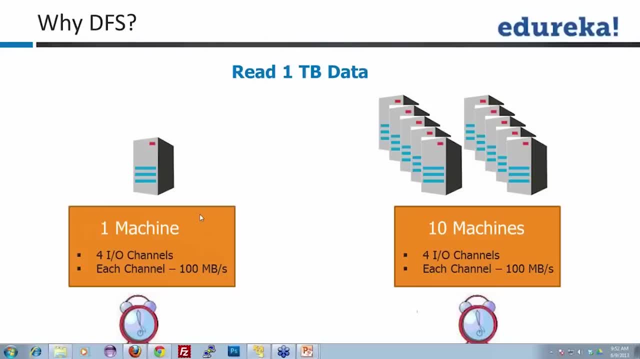 Okay, And do not worry if the answer is wrong. Okay, It doesn't really matter. That's not the purpose of doing this exercise: whether to get the right answer or not. Okay, The purpose is to for you to actually calculate and understand. 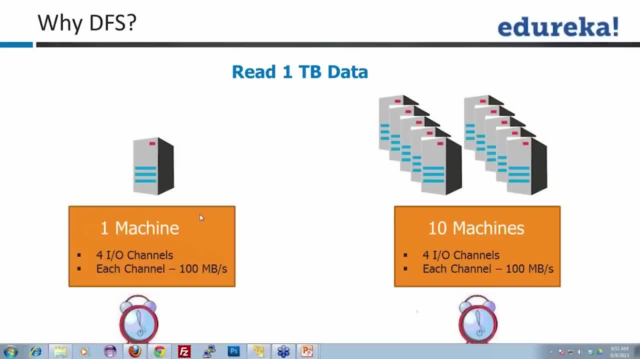 Okay, Abhishek has given me a big calculation. Abhishek, very yes, it must be right. only If you've done such a big calculation like an old professor, I'll say, yeah, you have done it right. 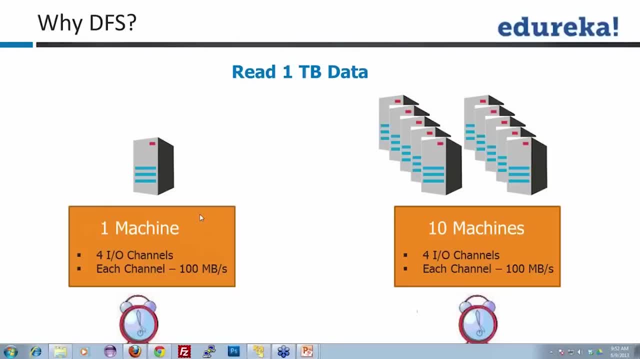 So, like like the time in college, right, we used to fill in a lot of things so that the professor thinks that this guy knows, knows something. So we'll give him some marks. I'll give you marks like that, Okay. 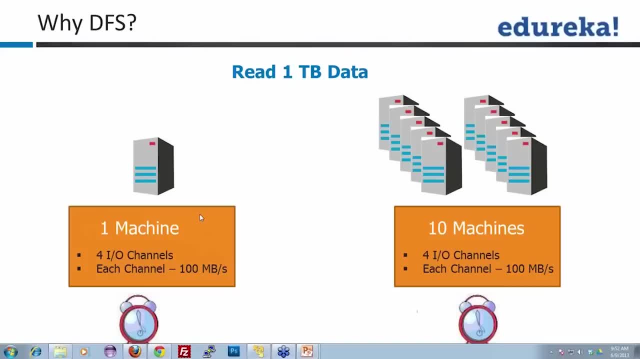 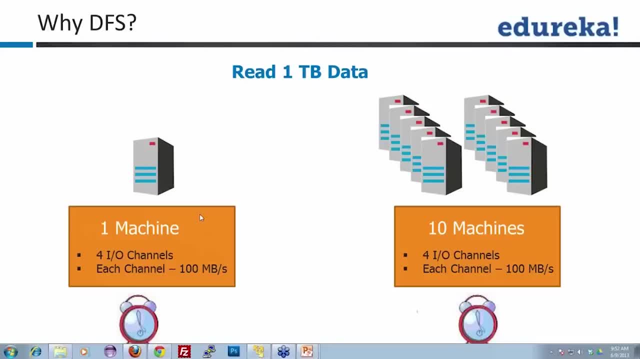 Okay, So I I am still waiting for answers from Rahul Shyam. Rahul has given me great. Okay, No problem, sure, thanks, Rahul has given me an answer. How did you get the grade? We had one interesting lesson there. 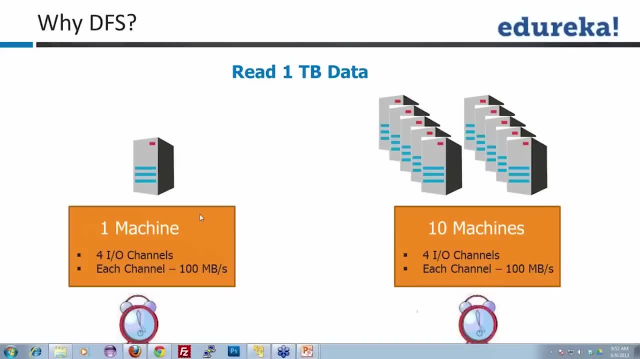 Shyam has given me an answer. Dayanand, are you with me? Vijay has given me an answer. Vijay always comes with Vijay. what is that 400 slash 4000,? give me answer in minutes here. I am bad at calculation. I am very bad at maths. I am not. I am actually decent in maths. lot of other subjects I am very bad at okay. 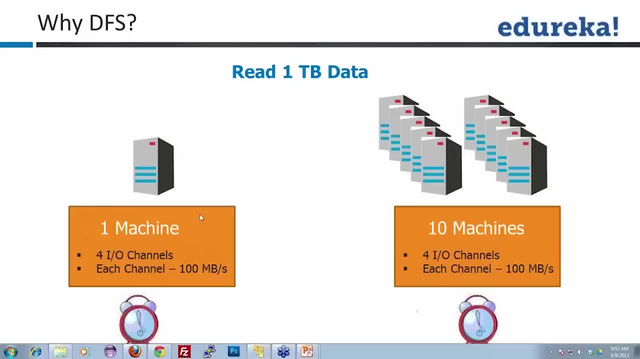 Okay, Dayanand, are you calculating? Yes, Vijay, you can use a calculator, man, if you. I will not use a calculator in front of you guys. you can always use Google for answering. okay, if I ask questions. and the reason why I tell you that is because it's not only, it's not only from here which you are learning you can. if you Google things, you will probably get a lot of other perspectives as well. 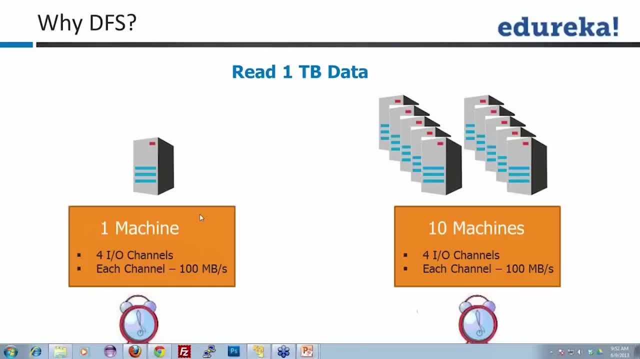 So Pralad has given me some answer which reads into 10737.. 418 seconds approximately. Pralad looks like something which has gone above my head. okay, but never mind. just important thing is to understand that it takes a lot of time, okay. 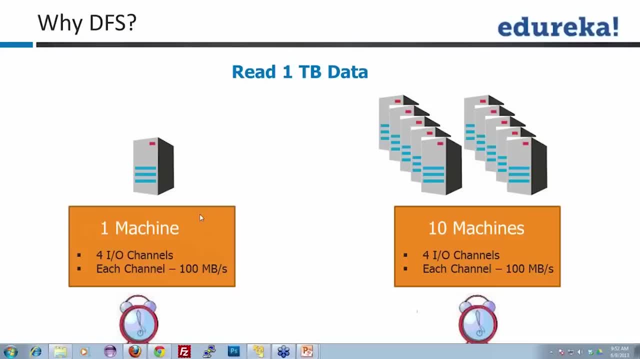 Okay, Shyam has given me the right answer. Shyam has told me how to calculate that, and thank you very much, Shyam. Shyam tells me 1024 into 1024, divided by 100, divided into 4, divided by 60, is the answer in minutes. yes, that's right. 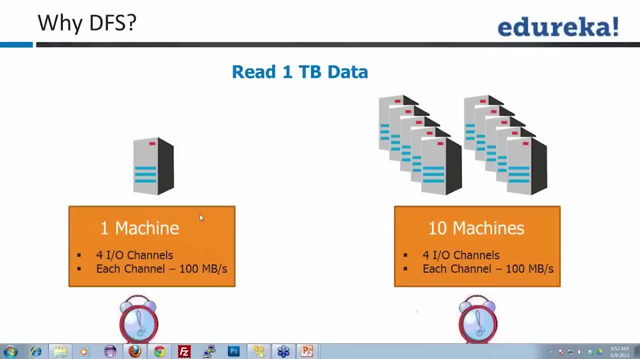 Okay. so, Dayanand, Are you there? Are you? are you actually calculating it? Okay, great. So see, the answer is. the answer is 1 terabyte. so 1024 into 1024 MB is 100 MB. is per second what it is able to do. so 1 terabyte will be 1024 into 1024 MB divided by 100, also divided by 4, because there are 4 IO channels. you can do that. 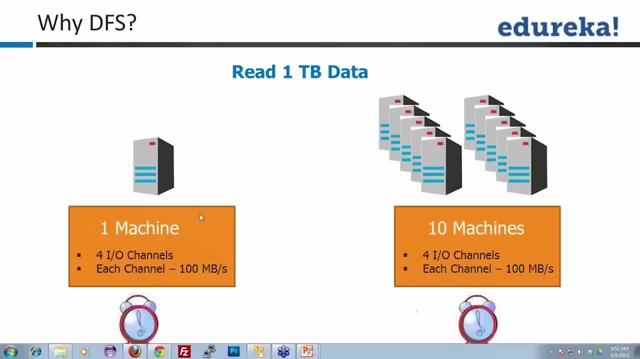 You can do 4 reads in parallel and then divide by 60,, as Shyam has rightly said, and a lot of other people have said so, it approximately takes around 45 minutes to do that. Okay, right, so now. now, the whole idea is not to actually make you calculate this, but the idea is to show you that, for 1 terabyte of data- okay, it is taking so much time to actually read it. 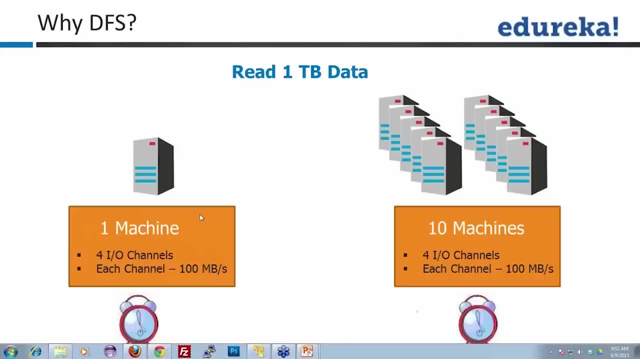 Now, what do you have to do? in real time, real life- All this data is dumped somewhere. If you have to read it back, you have to calculate the values. You gotta calculate the values of the data. Okay, back, you have to read it back multiple times. right to do analytics, right, is that right? 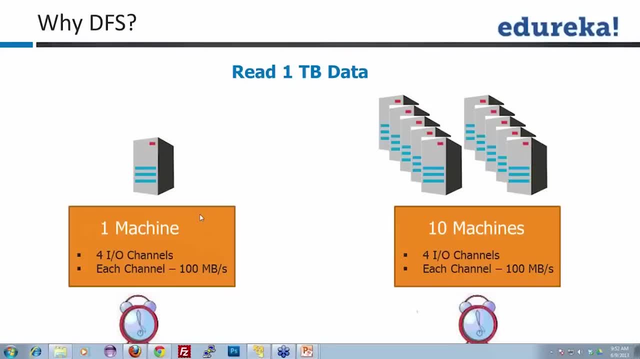 guys, yes or no? is this making sense? yeah, so, if you have, if it takes for 1 terabyte, it takes so much time. when we talk about zettabytes of data, think of it this way. Facebook had to read it in this manner. what analytics would they be able to do every? 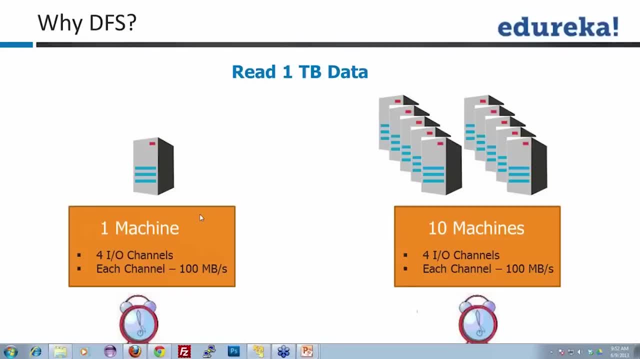 day they have 500 terabytes of data and that is old estimate, okay, so a traditional way of doing things like this vertically scaling things. vertically scaling thing means for the people who don't understand this jargon- I really don't like these jargons vertically. 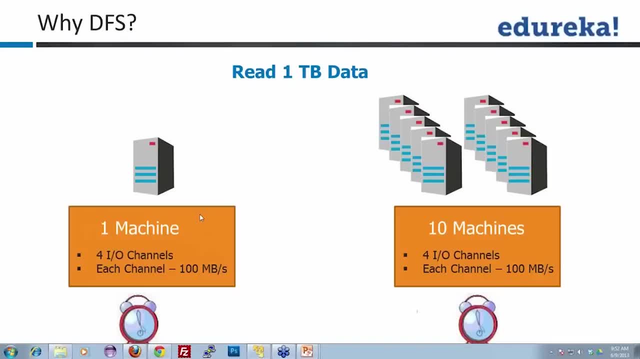 scaling means that you improve the system, put a better machine, improve storage in a system. so vertical scale is not going to help. put more expensive machine- okay, that's not going to help much. is that clear everyone? so the solution to that is something like: 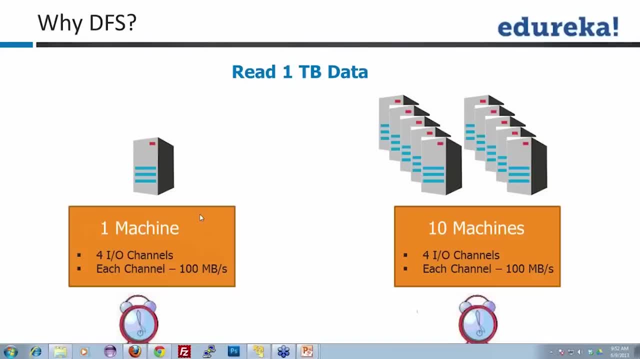 this. so if imagine if you could do the same thing, if you could partition, if you could partition that data and put it into 10 different systems, how much time will it take? now, I want this answer in 10 seconds. everyone has to answer. Vijay, you don't need math. 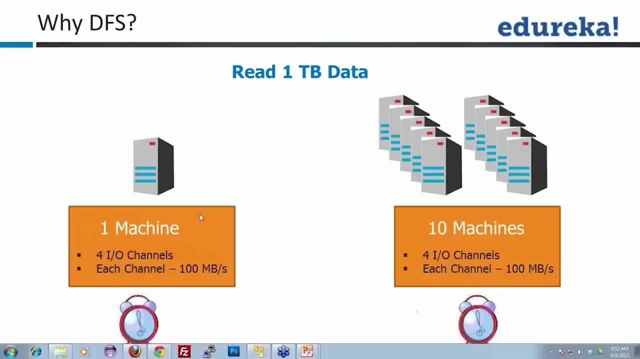 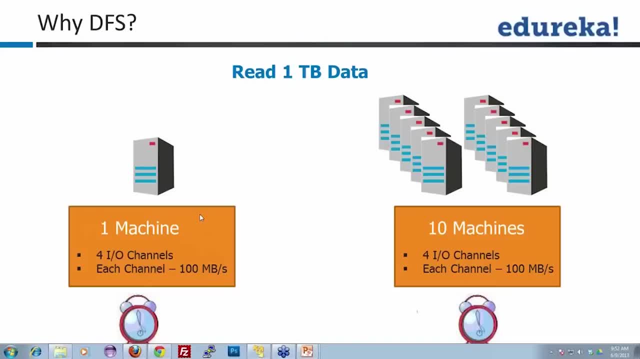 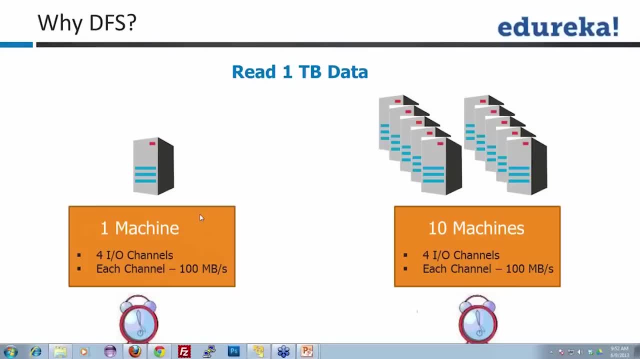 it. yeah, 45 by 10 is the right answer. now, that's a very, very simplistic view of saying things. this could be one solution. now vertical scaling is not going to help. that is clear, right, we understood. even if I add, say, 10 channels here, not possible, the maximum. 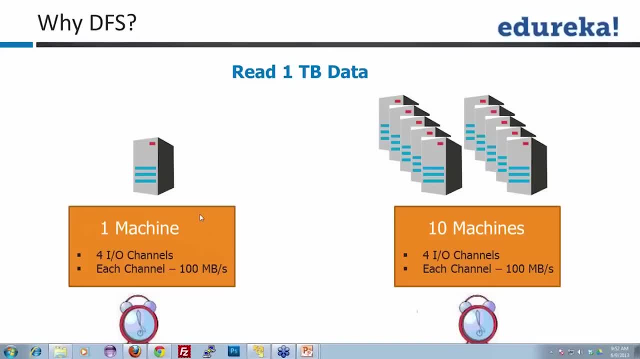 speed of SATA 2, which is which is the hardest standard, is how much like 500. I believe it is 500 MB per second, or or SATA can read it in. I believe SATA 2 can do it in 500 GB per second and that's gigabits. okay, so that's not those things. 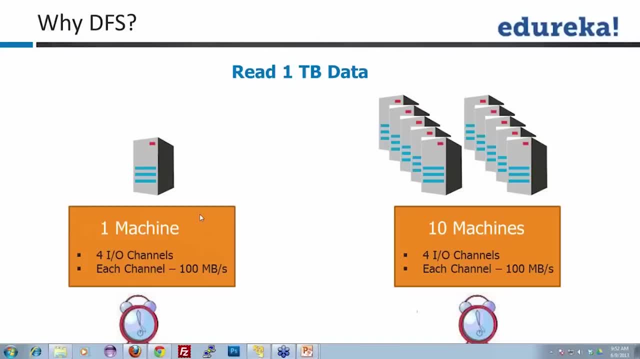 are not going to help much. okay, you cannot go ten times there, so probably a good solution. and a solution could be horizontal selling, which means add more machines. if you can partition this data, do it in a distributed way. so now, around 10, 15, 20 years back, there was a time when this grid computing or distributed 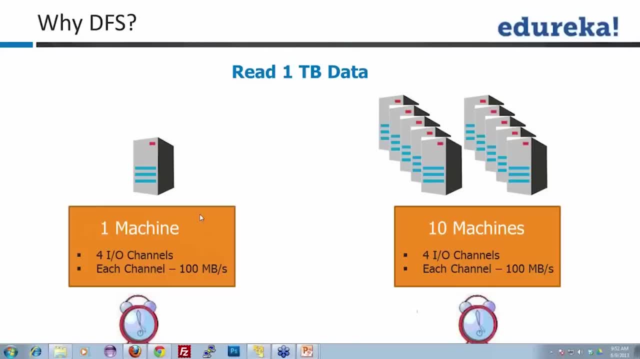 computing or parallel computing was very much in thing. okay, and there was. so there is a difference between grid computing and what we do here, right, okay, so there, that time the challenge was CPU speeds, so you wanted to distribute the compute. have if you have a big equation to solve which you cannot solve in one. 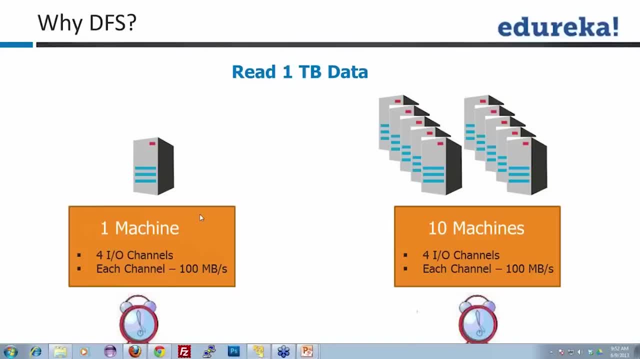 machine, you distribute it across clusters of computers and let those clusters actually solve that and give it back to you. right, this is this what we used to do earlier. okay, when we what is does every is, is everyone in sync with whatever I said? now, quickly a smiley: if everyone is. 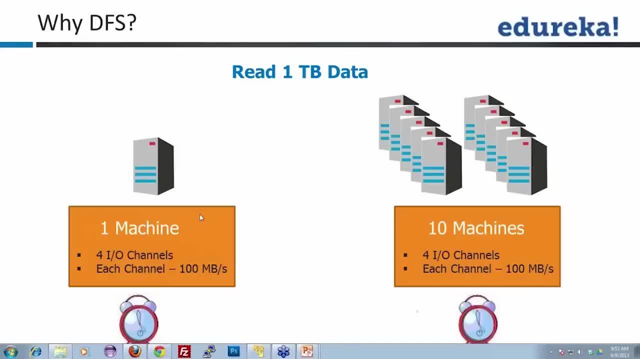 understood. okay, s is also fine. if someone has not got it, please tell me. great, so at that time, one solution which we, yes, great. so everyone, everyone is in sync. anyone who is not, please, please, do, let me know. okay, I'll really appreciate. okay then, and no problem. so then, and wants me to repeat. 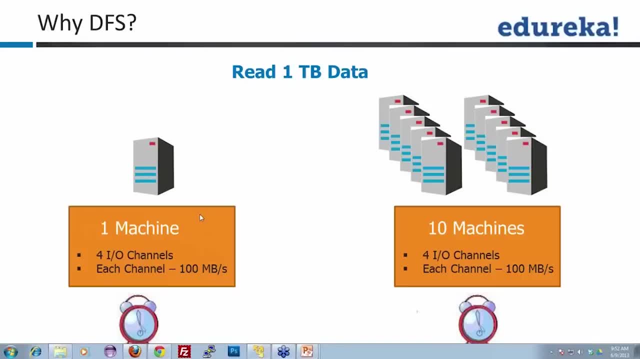 this. so then- and I was saying that there was a time earlier when computation speeds were a problem- okay, so you were restricted by computation speed. so if you had a big problem to solve, today also that problem is there, but that the computation speed problem came much earlier than this problem which we are. 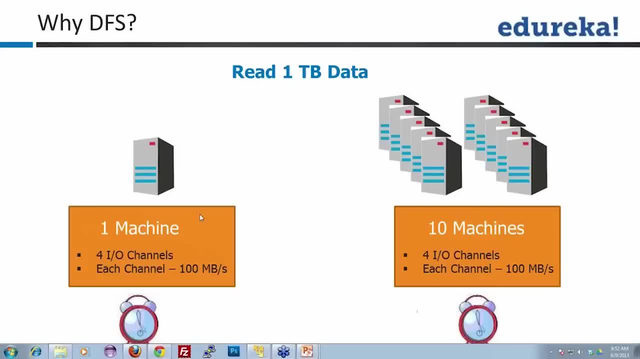 talking about today now. so at that point of time what we did was we called something called parallel computing or distributed computing. I am sure everyone has a And anyone who is from a computer science background has read that theory. subject: distributed computing, which no one understood why it is there, and you had to write a big answer: what are the advantages of distributed computing? So go back to that, think about it. So that was the time when challenge was CPU speeds and that time what we did was we distributed a particular task across various machines and then got a consolidated answer. 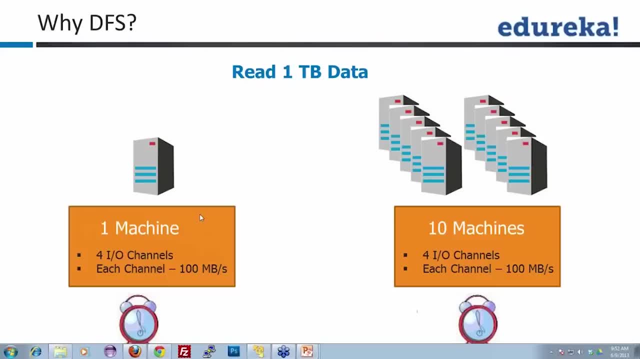 So that's how we used to do that problem there. A similar problem now is not in computation, So this is not parallel computing. What we are talking about is not parallel computing, but this is distributing the data across multiple channels, and it's not because of the computation speed, but because of the IO speeds. 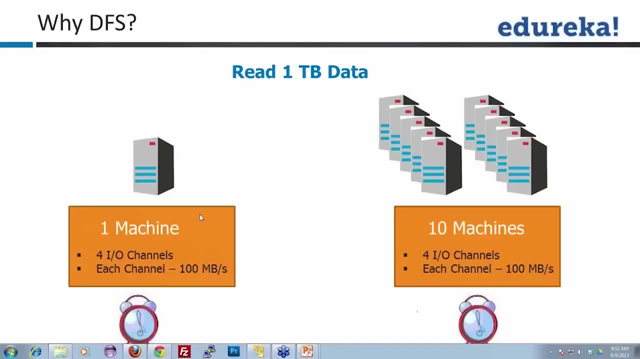 So this is the difference which I want to bring out here. Is that clear to everyone? Can I quickly get a yes or a smiley from everyone If you have understood the difference between parallel computing and what I'm trying to tell you here? Great Thanks, Vijay. Vijay says perfect, Thank you very much. Great. So, guys, you can keep encouraging me sometimes, Okay, But yeah, I mean fine, Thanks, So great. So Anoop is probably not answering. Anoop, are you liking the class or you want me to change something here? 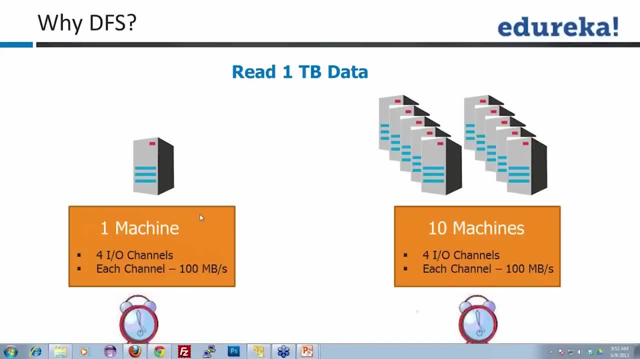 Are you doing something else as well? Okay, Great. So, Anoop, I really appreciate if you can just quick Keep writing things, yes or no, everything is fine. I want to make sure that. Yeah, No problem. No problem, Anoop. So you can see the chat window right. So, no problem. 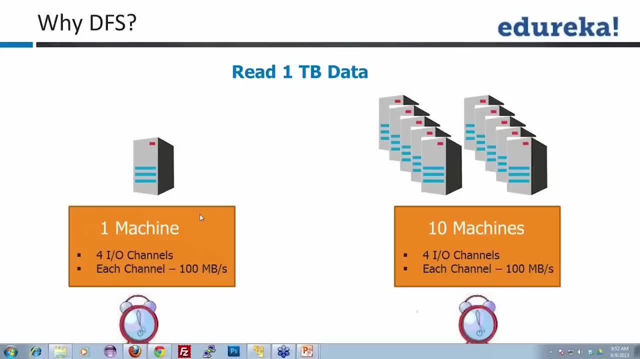 See, if this class- I am never limited by time- Okay, I have a lot of time. if, after this class also, I can be online for a one-on-one session with any one of you who has not understood something, Okay, Just, I'm never limited by time. Okay, I've never considered I have a lot of time in my life, Okay, So please make sure that you ask me questions. 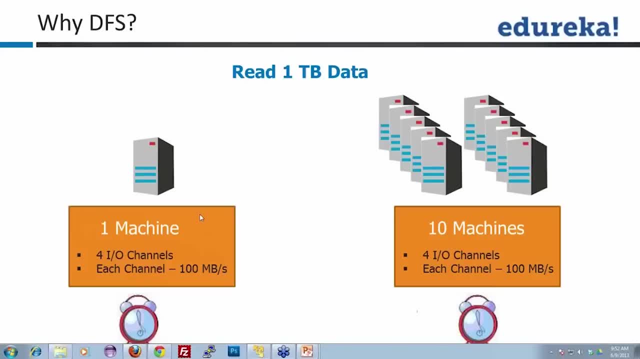 everyone here in the class has already said that they are okay if we go a little slow this time. okay, from this week onwards you will have one more week, full week. you can ask questions, you can get up to speed. this is the first class, so we can be. 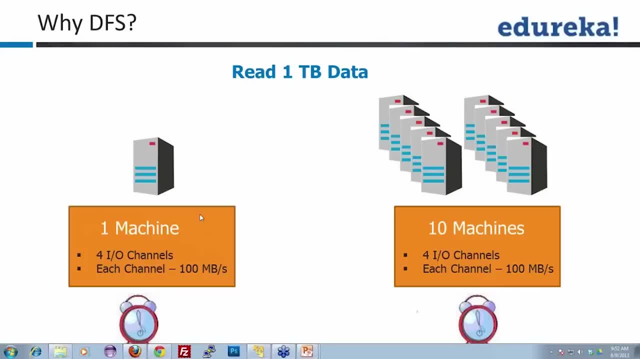 slow. okay, Anoop, is that fine? so anything if not understood, please feel free to ask. I can also unmute you if it looks like. if it is a little difficult to actually answer questions, write questions on this chat window initially. okay, I can unmute you and you can ask questions. 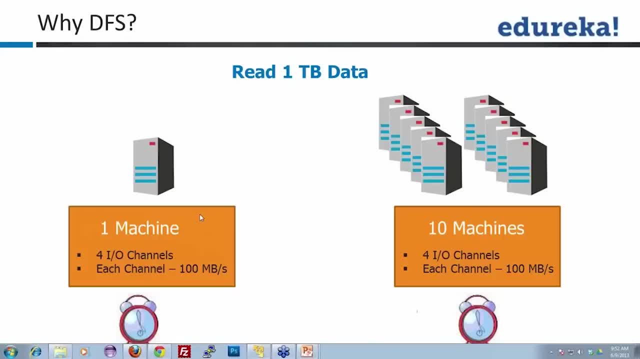 okay, sure, great. so, and don't worry, all of us are new to this. I am also new to this. I also learn a lot of things in the class itself and Vijay Prahlad everyone. please make sure that. 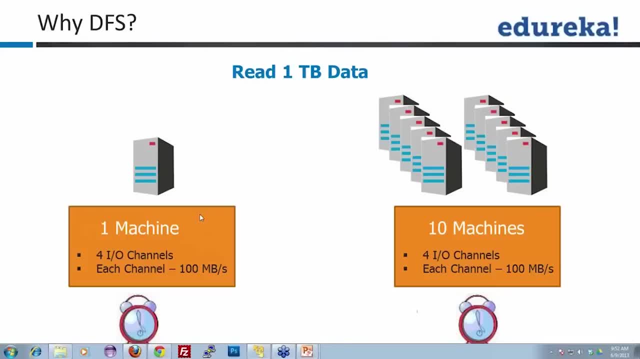 if there is anything which is a doubt, don't keep that doubt with you. you can ask me and for some things, if you want anyone of you who wants to speak to me after the class as well, one on one on Skype or something, 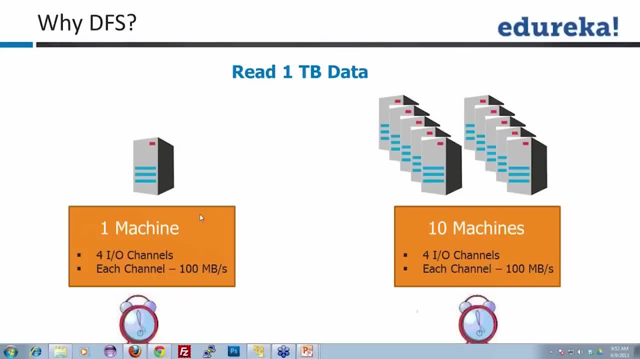 we can do that as well. today itself, we can do all the doubts. okay, guys, thank you very much. and everyone is that fine. I mean, I hope everyone understands that there will be some people who will be completely new, who would be coming in this class, who would have actually enrolled. 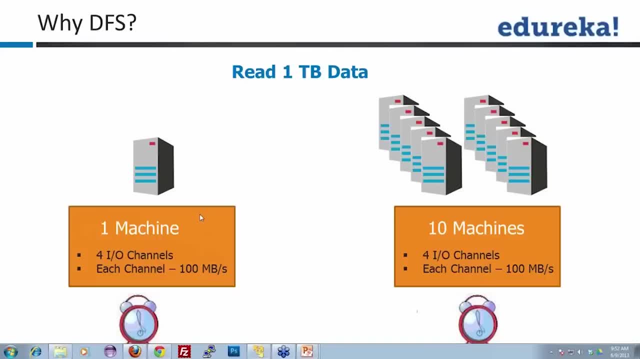 for the course last night and just thinking that I will also learn something. so we just want to make sure that we are with everyone, okay, so if this method of teaching is fine with everyone, I quickly want a yes, right, right, thanks, Abhishek. Abhishek is saying great. thanks, guys, okay. 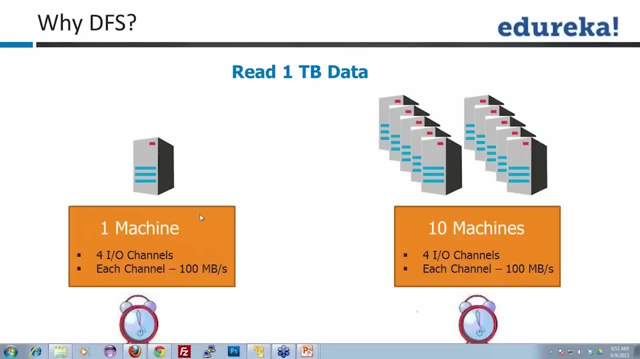 fine, so we will just go a little. we will go a bit extra with everyone today. next time onwards we will be a little fast, but we will make sure that everyone with us. that's why we have a limited number of attendees in the class, right, so we can handle everyone now this. 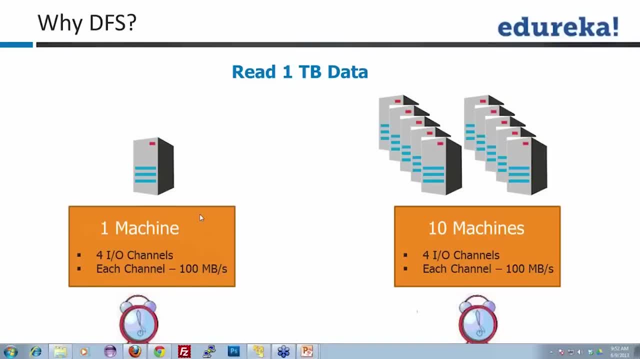 class is actually. I can handle 15, 16 people. now they are 11,, so it's not all that difficult. okay, great. so now everyone understood the fact that the challenge is not in storage space, it is not in computation speeds, it is in the IO speeds, right, yes? 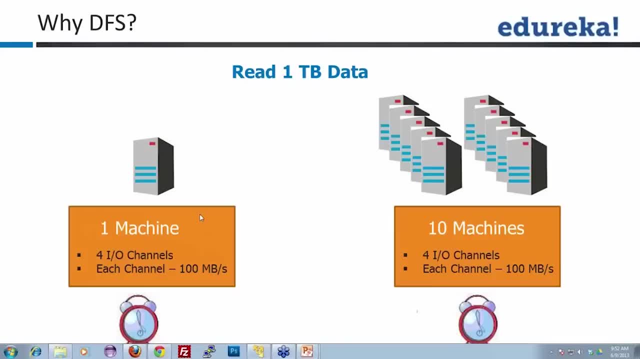 or no, quickly a smiley or a yes. this sentence which I said. everyone is crystal clear with this, because this could be one question which can be asked to you in an interview. if someone comes to me for an interview, I ask this question, okay. 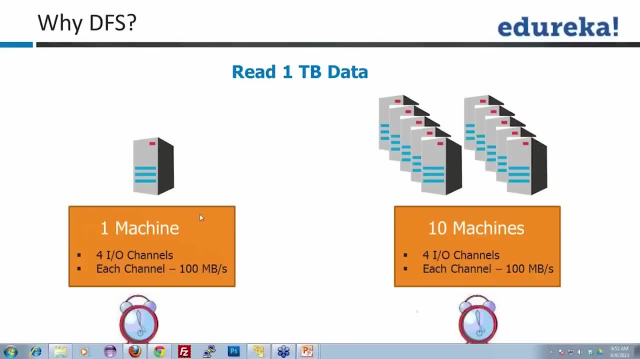 so please make sure that you understand this. great, so the challenge is not this: okay, someone has given me a smiley. thanks, someone. okay, now a probable solution is distribute the data across multiple machines. okay, and so I just gave this. 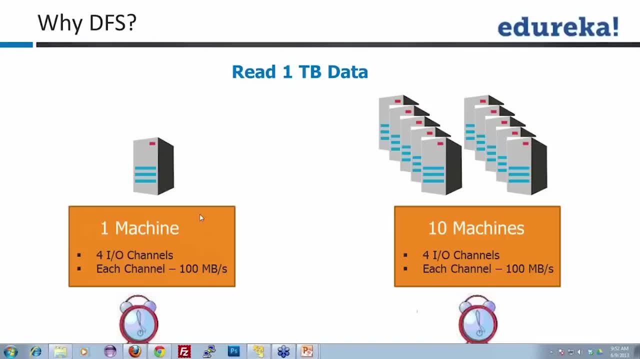 answer here. now let's see what is distributed file system. okay, now, when we agree that distribution is the way, how do we do it? let's understand that, okay, so before. so this is a picture here which shows you how actually a distributed 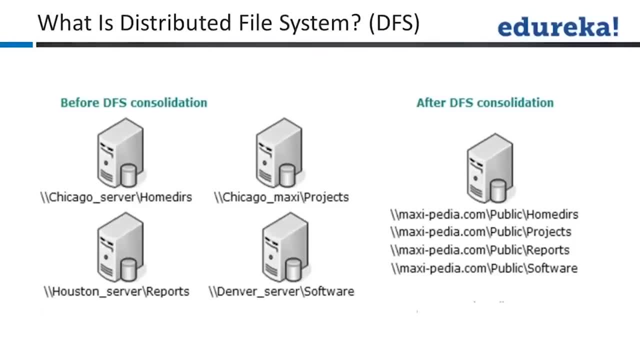 system looks like okay. distributed file system looks like. so here we have. we have different machines at different locations, physical locations. in Chicago there is one machine. I mean some example, don't worry whether it is Chicago or Denver or Bangalore, or or, or say what say Noida, it doesn't really matter. so these are machines which. 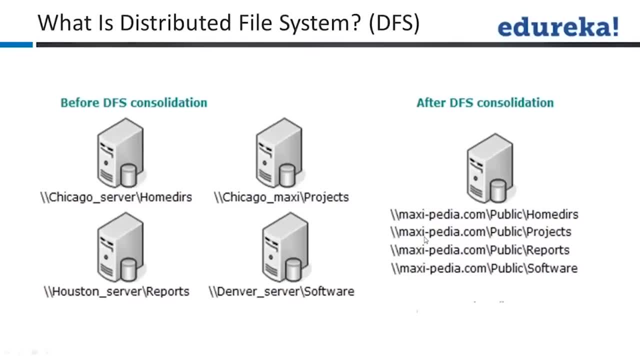 are kept at different physical locations. now, when you do a DFS consolidation, which means when you make a distributed file system out of this Narayan, what are you doing when you are not looking at this slide? I have a tool to know who is not attentive, so come. 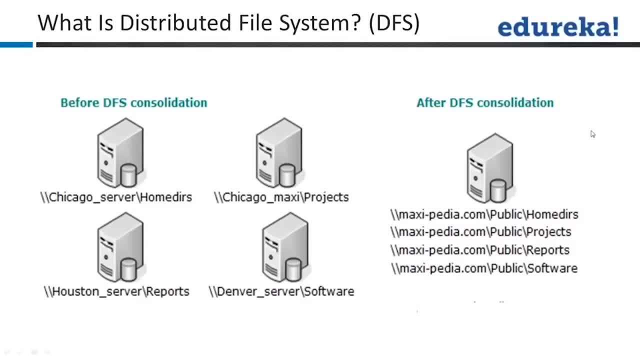 back. okay, I play this game in guard mode. okay, Narayan, so you have to be attentive here. okay, Vijay has gone- non attentive. okay, Suman has gone- non attentive, okay. okay, now one has gone offline, okay, no problem, so. yeah. so now, once we do this, DFS consolidation. 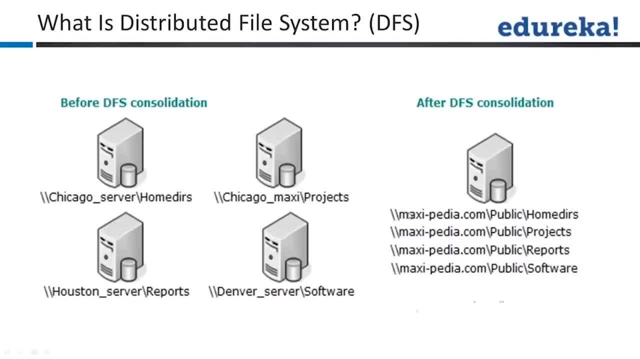 then, though, these machines are still at different locations, but on a logical level they look like directories in a single file system. okay, is that? fine? so this is what DFS or a distributed file system is. so machines will still be at different locations, but 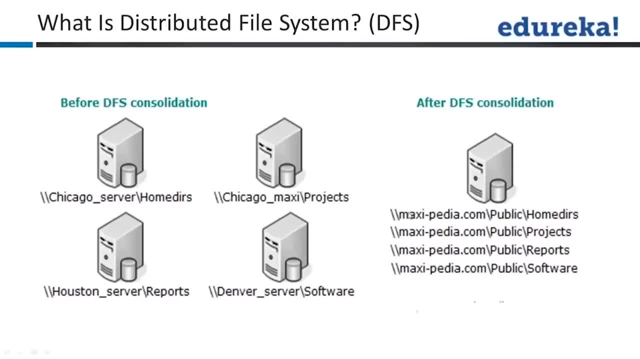 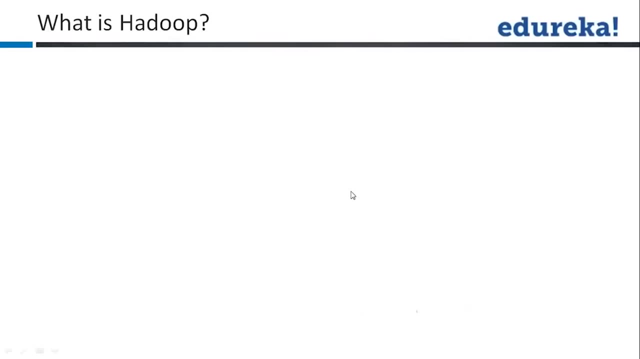 on a logical level, if to a client, to a user, it will look like different directories in the same file system, Fine, is that? okay, guys. so this is about how do we, how does a distributed file system look like? okay, okay, so what is Hadoop? now we have understood what is big data. we 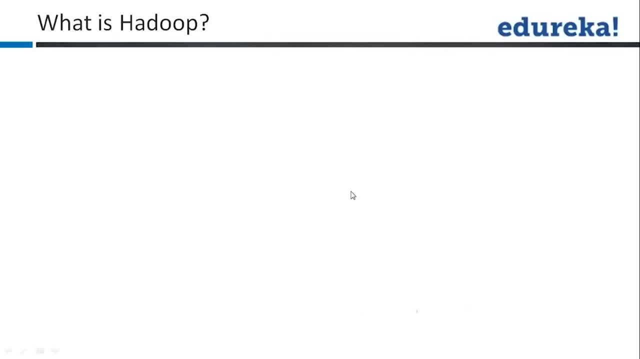 have understood what is the need of unstructured data. we have also understood that the challenge is not to store data, but to read, write data, to analyze data, and we have also understood to do something like this. we need something which can support a distributed file system. 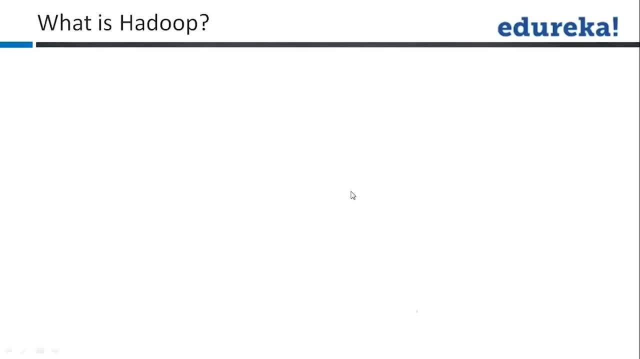 okay, so Hadoop is actually a framework which solves this problem. okay, so all of you understood the need for Hadoop. now can you quickly give me a? yes, I'll understand what is. you'll understand what is Hadoop, but has everyone understood the need for Hadoop? anyone who? 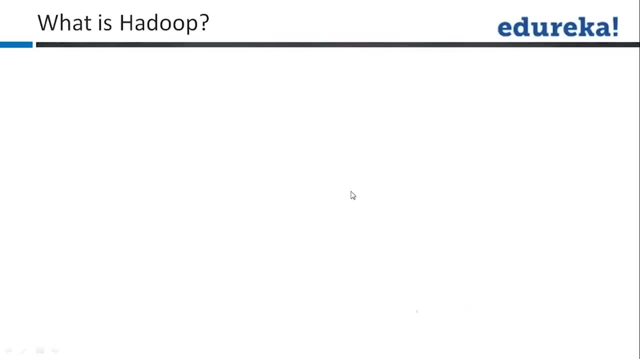 is not okay. can I get a smiley from everyone? okay, lot of people are writing and smiling as well, Okay, okay. so Rahul says: can you repeat? Rahul, are you joking with me or you really want me to repeat? okay, so I'll just repeat it for the sake of Anupam and everyone. so, 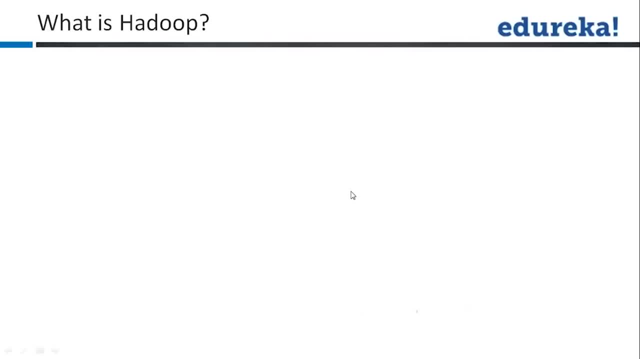 see basically who have joined late. we've understood from right from the first slide that what is big data. we have understood that. so we have huge amount of data, unstructured data, getting dumped in some places. okay, then we understood that the challenge to analyze 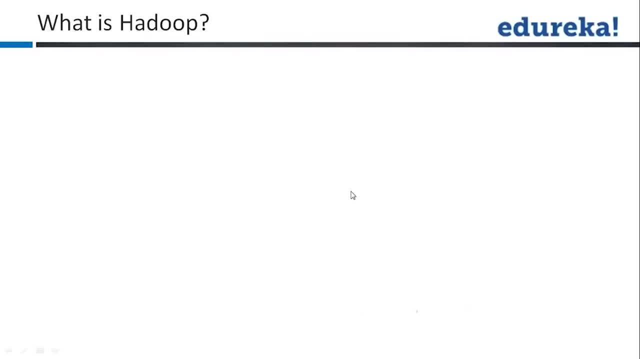 this big data. we have to read it back. okay, Rahul, please play attention here. Now the challenge is not to store the data and how to store the data. technology is scaled up there. the challenge we saw was to read that data back. okay, to do analysis on it. 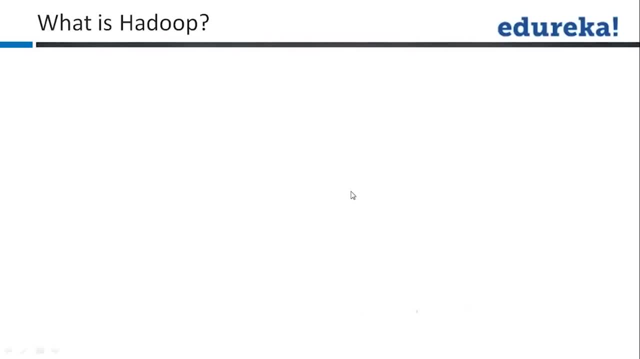 and then we understood that reading it from a single place is not going to solve the problem, so we understood that it there has to be some distributed way of storing this data. and then we understood what a distributed file system is. and now so we know that there. 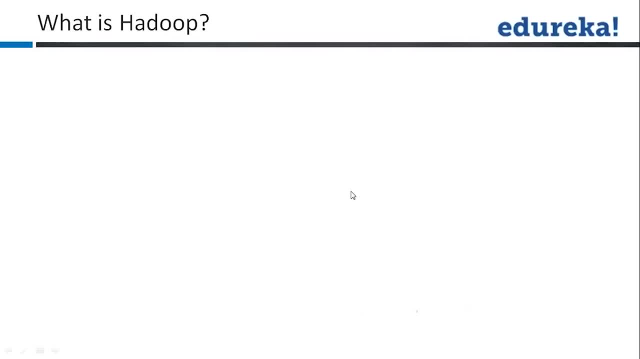 is a need for something which can solve this problem of storing data in multiple nodes across a cluster. So is that clear to you, Rahul? that is why we need Hadoop. great, so that is okay, great. so now the need of Hadoop is this: everyone has understood that. let's see what Hadoop 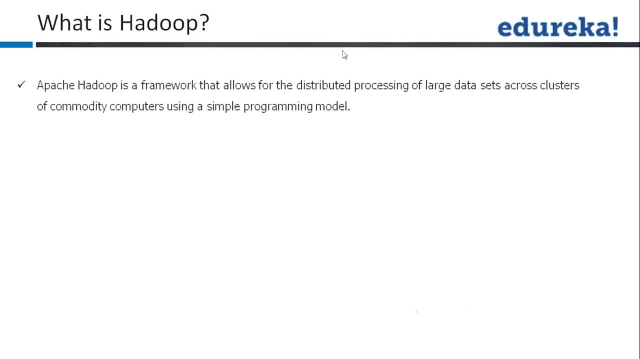 is, I will go with the formal definition of Hadoop, and this will. I promise you that this is the last formal definition I will talk about in my whole life, after this one. okay, I hate formal definitions, but this way, this time I had to put this in. okay, so Hadoop. 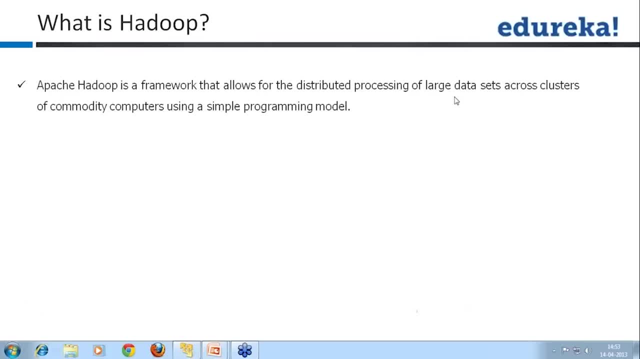 is a framework that allows for distributed processing of large data sets or running on commodity computers using a simple programming model. okay, so now there are a few few things which have to be noted here. okay, that's why I put this definition. so Hadoop is a 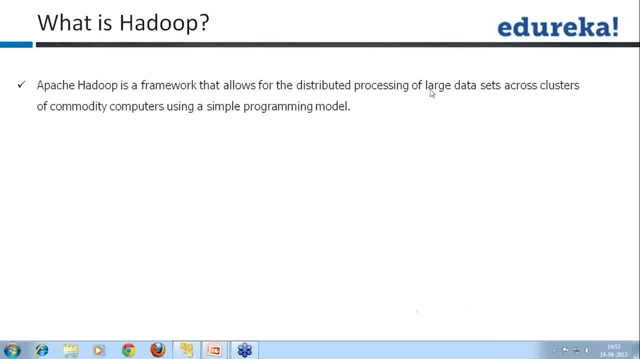 framework that everyone understands of distributed processing of large data sets. so Hadoop is useful only when you have large data sets, okay. if you have small files, it is not of use. So this is a very important thing: large data sets and that to unstructured data- okay, across clusters of commodity computers- okay, I'll. 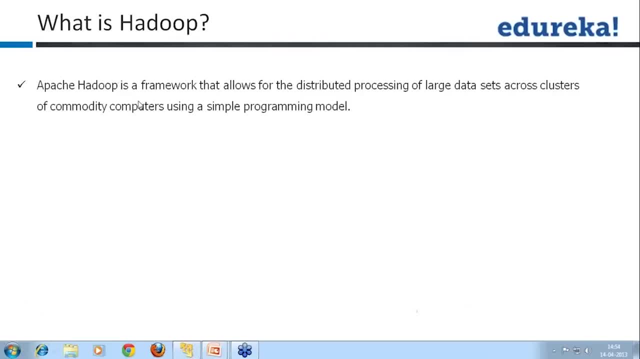 make you understand this term- also commodity computers. so basically, Hadoop does not require the nodes on the Hadoop side do not need not be high quality, high availability machines. they can be simple hardware, commodity hardware. we'll understand this in more detail using 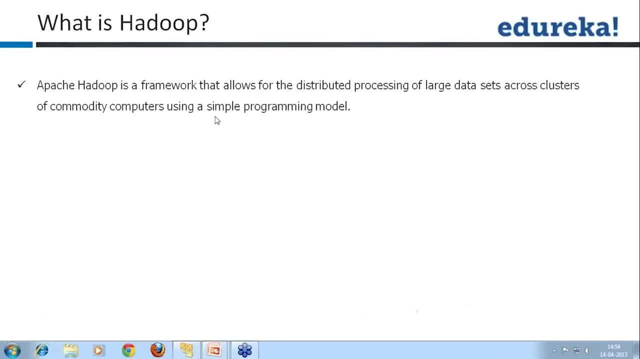 a simple programming model. so the simple programming model is called MapReduce. I will not explain you anything about MapReduce today, in today's class, but you just try to understand that there is something called MapReduce. just get this term in your head in the next. 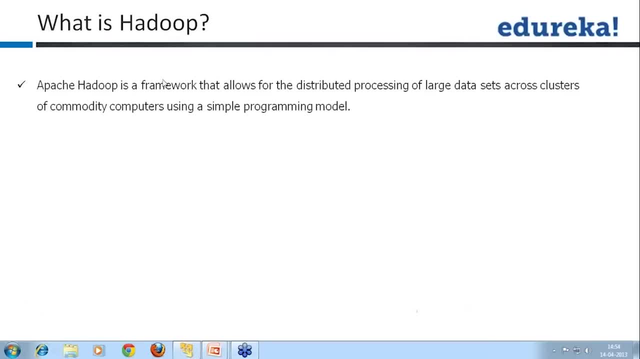 few classes. we'll understand that in more detail. okay, is that clear to everyone? so it's a framework for distributed processing, large data sets, commodity computers and simple programming model, so we will understand each and everything in detail. going forward is: 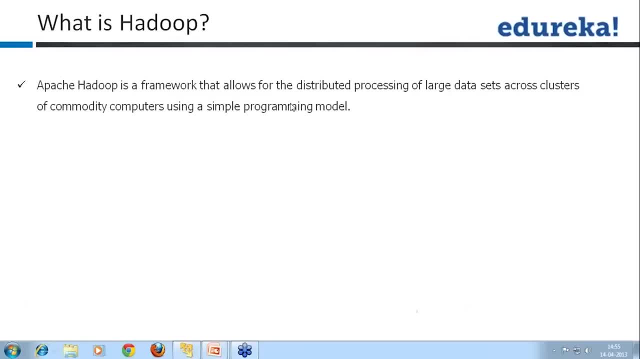 that clear to everyone, guys. anything which you do not understand here, it's very important to understand this, okay. so, yeah, I think everyone will understand this. okay, so, I think everyone has understood it okay. so, good, good, good, thank you, guys, if you. 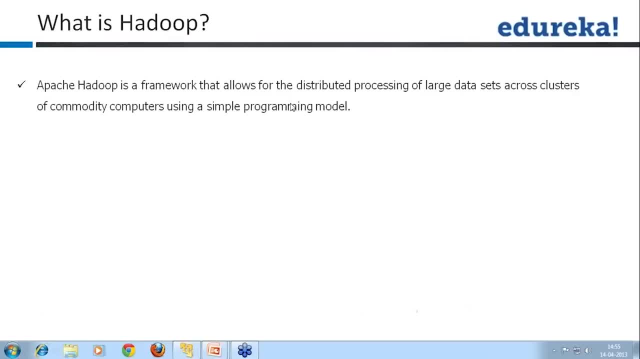 keep on. if you keep on giving me these yes or smiley, I know that I am doing a decent job here and you are not getting bored, okay, so please do not hesitate to write that, okay. thank you very much, Ajay. Mohan is not doing that. Mohan is not happy anymore. okay, don't. 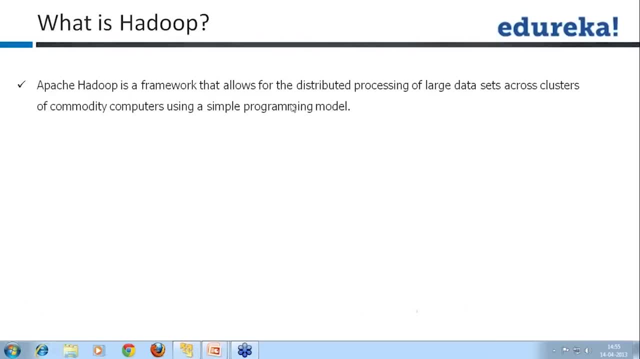 worry, there are enough people to keep me going. Syed has given me a smiley again. thank you, Syed. okay, Mohan is saying not true. Mohan is saying not true. Mohan is saying not true. Mohan, you can just give me a smiley, man. okay. so now companies using Hadoop. 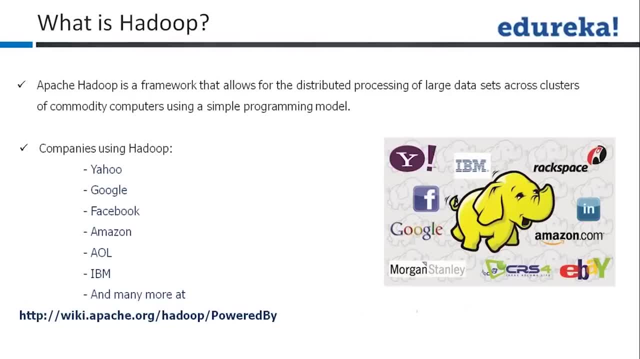 now this is again a question, a question which people ask. which are the companies which are using Hadoop? so I am sure a lot of we had Sandeep from Yahoo, right? okay, no problem, Mohan, please take your time. okay, so Sandeep is from Yahoo. so Sandeep, Yahoo, is a company. 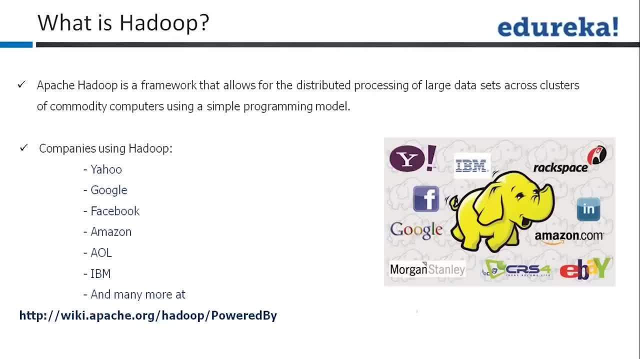 which uses Hadoop. Google uses Hadoop, Facebook uses Hadoop, Amazon, IBM, AOL, a lot of other companies- you can find that here. I mean LinkedIn also uses Hadoop. so basically, the funda is that any company which has to do a big data analytics and we 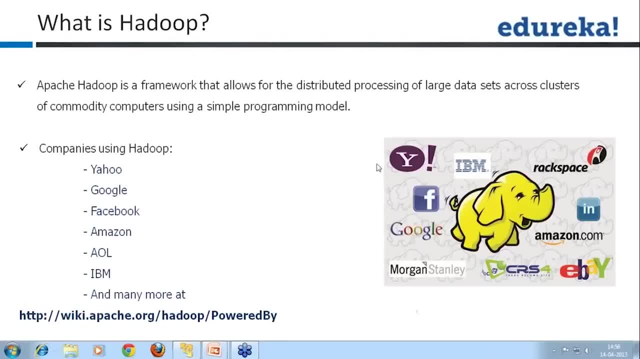 have an expert on big data analytics here, Ajay, Ajay. can you tell me one Indian company which is using Hadoop? Ajay, okay, so Google says okay. yes, Vidya Sagar, that's right, Google had released their own version of DFS. 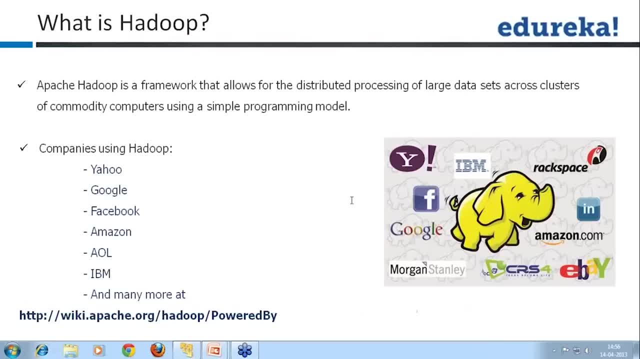 Sure not today, but definitely we will understand it. okay, not today. okay, Cloudera is not an Indian company. thank you, okay. so, Vidya Sagar, yeah, Hortonworks is also not Indian. I believe EMC is also not Indian. 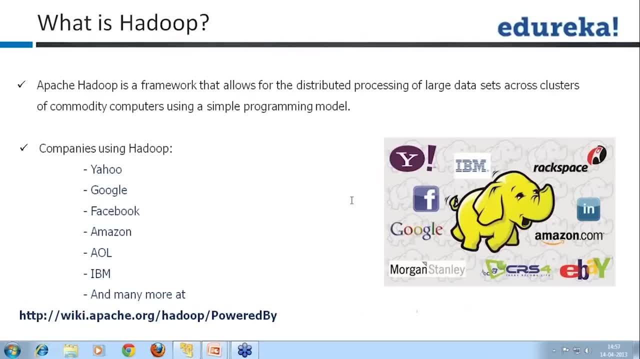 well, I have been told, I have been told that the Aadhaar scheme is going to use Hadoop. okay, so Aadhaar scheme, everyone knows about that. does everyone know about that? okay, so, Aadhaar scheme is going to use Hadoop, so that will probably one. okay, so now, now, guys. 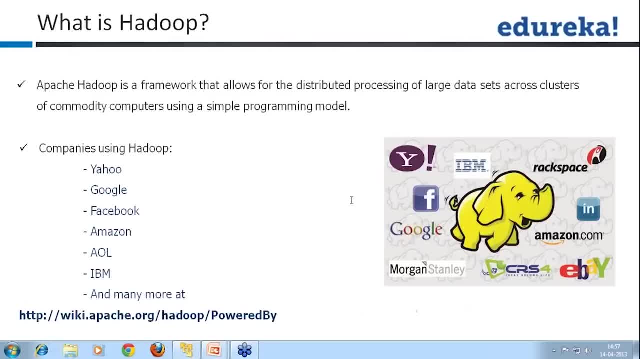 there may be some answers which I may not be able to give you right now, and the reason, the reason why I don't want to give those answers is maybe they will take you a little off topic, so I will not answer them right away. we you can always write those answers on the 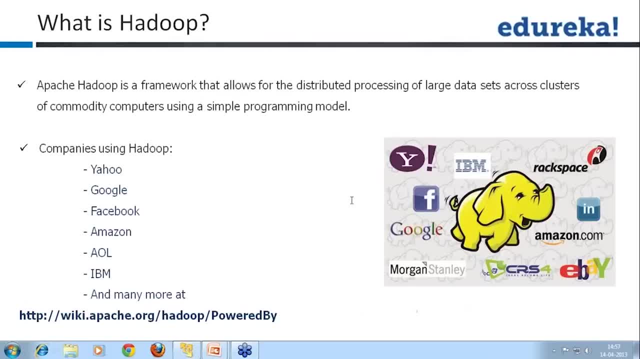 on the chat window. we will respond them offline and also, if needed, we will be covering a lot of those things as we move on in these sessions. is that okay with everyone? okay, cool. so yes, these are the companies which use Hadoop. okay, so now let's move forward. now I have a very 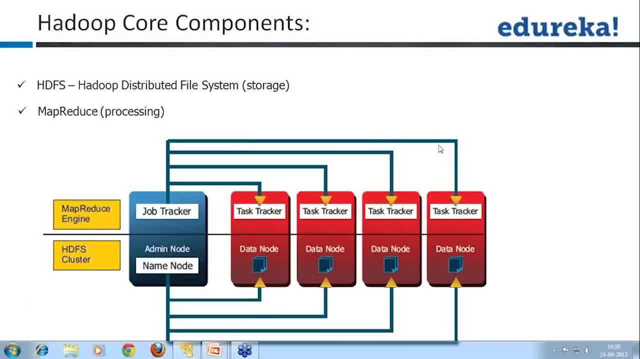 now, this is the first technical diagram on my slide, okay, and I want every one of you to actually look at it for some 10-15 seconds and don't worry too much about it for now. I I I bet that by the end of it you will all become experts in this. 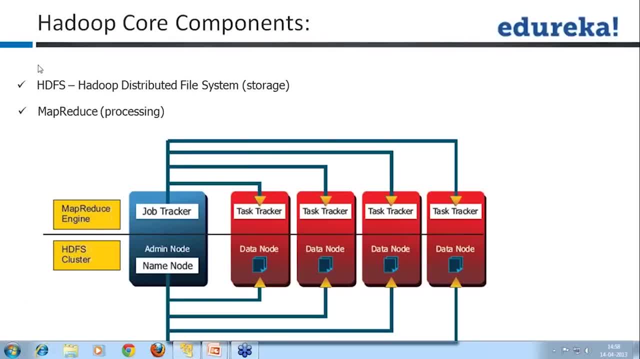 okay, so Hadoop basically has two core components. okay, I want all of you to actually look at this very with pay a lot of attention here. okay, because this is the first time when we are talking about Hadoop and that's why you paid for. so if you don't understand this, there is no point in. 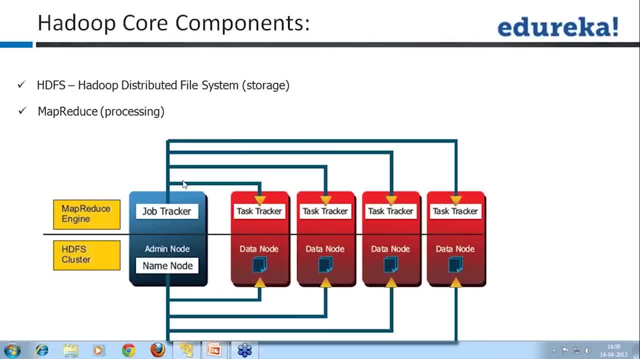 you are making this payment to Edureka, which is, by the way, doing very good these days. I have seen the kind of attendance and the kind of demand there is. so, just joking I, I asked them for a hike, so yeah, so basically, 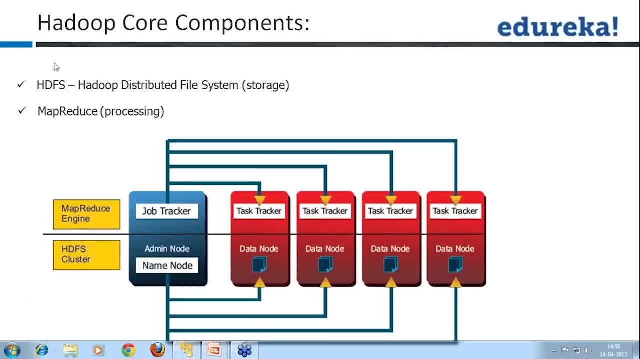 we. we have two major components. one is the HDFS, which is the Hadoop distributed file system, and the second one is MapReduce, so distributed file system is used for storing and processing is done by MapReduce. we will talk about MapReduce later on in the next few classes, not today. 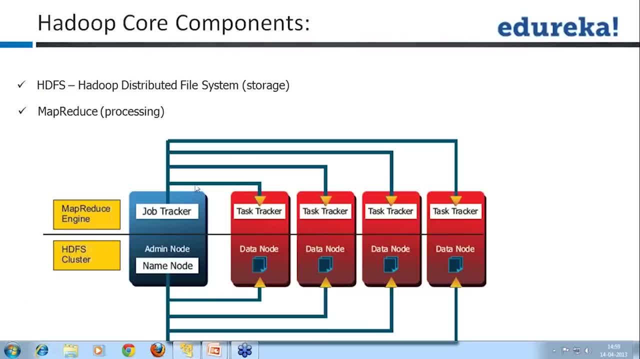 on this diagram. there are two things which are very important to note. we said there is a, and I will not explain it here. okay, just note that there is something called a name node, which is the admin node. it's a master-slave kind of configuration. 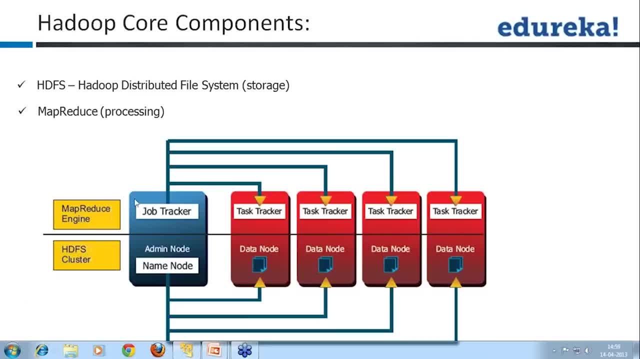 so there is something called an admin node or a name node, which is the, which is the master, and then there are slaves, which are called data nodes, okay, and then there is something called a job tracker. you have to understand, remember these terms. don't understand them, just remember. 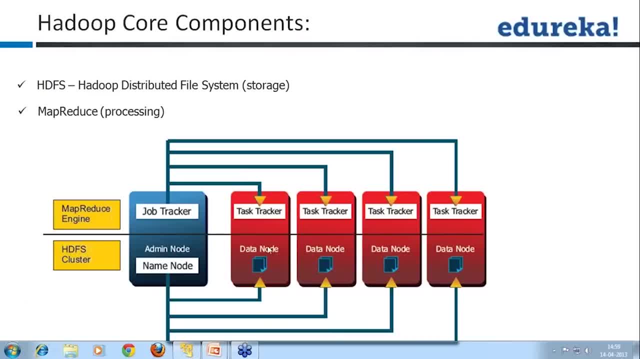 them, which is associated with a name node, and there is something called a task tracker, which is associated with a data node. okay, is that? is that clear to everyone? you don't have to understand it completely, we will. this is what. 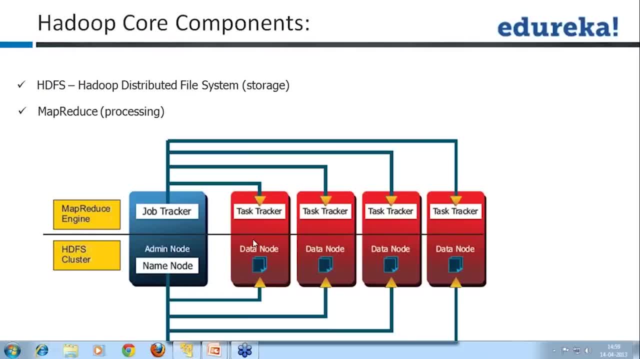 we are here for we will understand it by the end of this session. for now, just remember that there is something called a name node and a job tracker, which are associated, and there is something called a data node and a task tracker, which are associated. okay, and name node is the master. 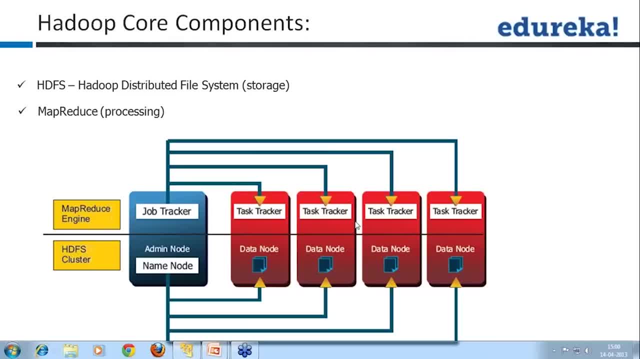 and task data node is the slave. is everyone clear with that quickly? can you give me- you don't have to understand it completely- if, even if you don't understand it completely, if I ask you a question, what is? 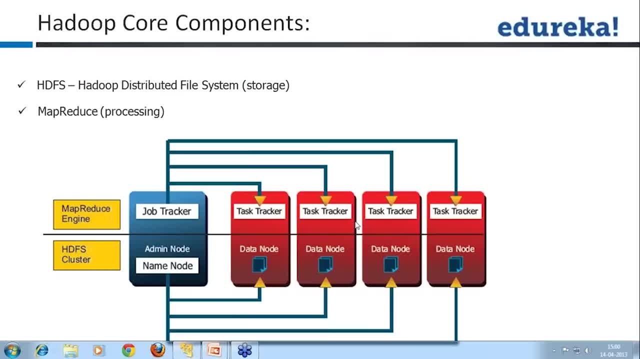 name node associated with. if your answer is job tracker, then you're. you're good enough for this slide. okay, so can everyone quickly answer: what is name node is the master? Rohit gives me the answer: name node is the master and it is. there's a job tracker associated with it. what is a job? 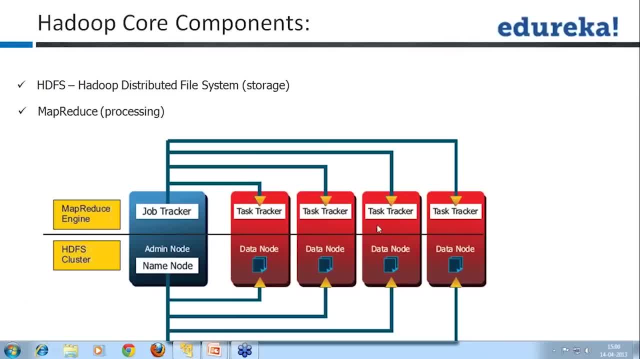 tracker. what is a name node is something which we'll cover. good, great. so yes, so data node is a slave and this okay. so there's another term here. don't worry, Sandeep, I'll explain it. Sandeep asks me: what is the difference between MapReduce? 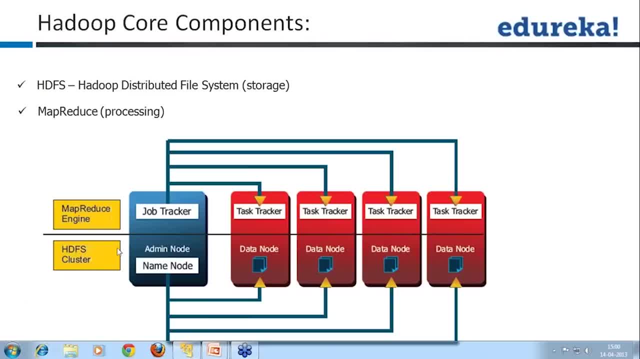 engine and HDFS cluster. okay, so basically, HDFS cluster is the is the name given to this whole configuration of masters and slaves where this data is stored. okay, so that is the HDFS cluster. so this whole thing is a HDFS cluster. MapReduce engine is the programming model which is used to 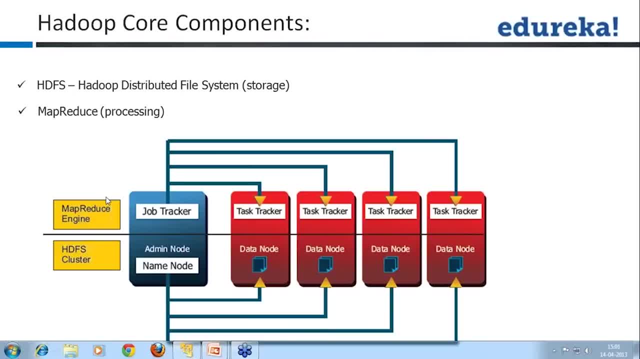 retrieve and analyze this data. is that clear and I'll not tell you anything more than that in this. you don't have to understand anything more than that. if this is much as clear, you will understand everything going forward. I'll not go into more. 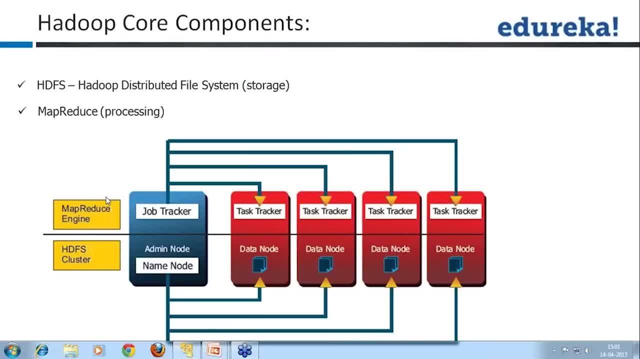 technical details right now. so two, three things on this slide. one: there's something called a name node associated job tracker, something called a data node associated task tracker. then we have HDFS cluster, which is the combination of these name nodes and data nodes, and then we have a 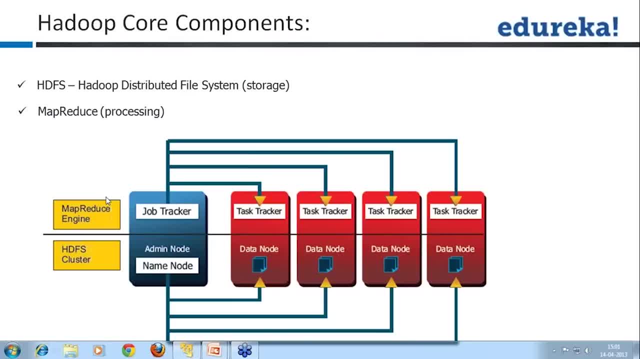 simple programming model which is called MapReduce engine. is that fine, everyone? can I quickly get a smiley from everyone other than Mohan, because Mohan does not want to give that? Yes, yes, Rahul, you're right. Rahul is asking me job tracker as task tracker and task tracker. 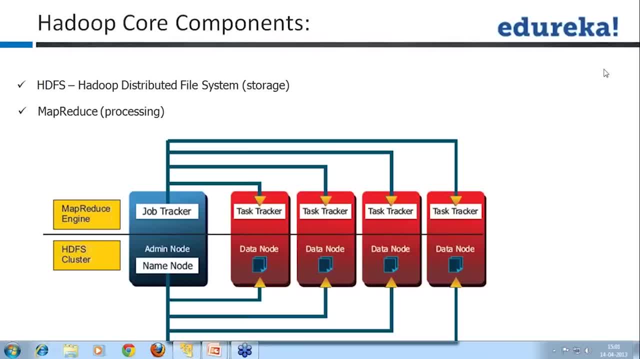 all are separate machines, total five in this picture. so yes, a task tracker is associated with each data node. so multiple data nodes and single name node. that is the very minimal configuration. we will talk more about it as we move forward. okay, so I've got a smiley from. 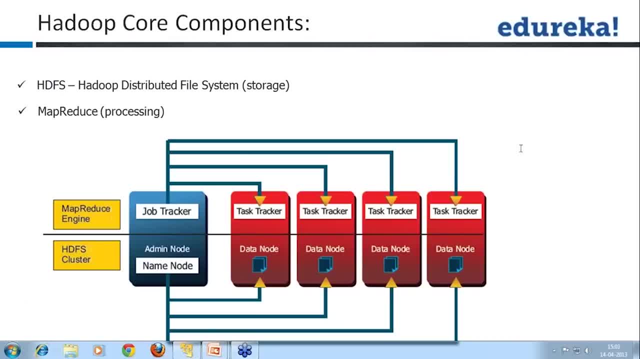 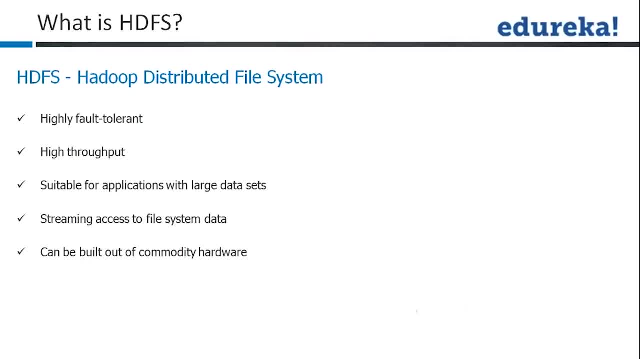 everyone. thank you, guys. okay, so everyone has understood it. now let's move on. Okay, so now, basically, there are a few features of HDFS which are very important to understand. okay, and there may be some reiteration here, but it's very important, so I'll repeat it. 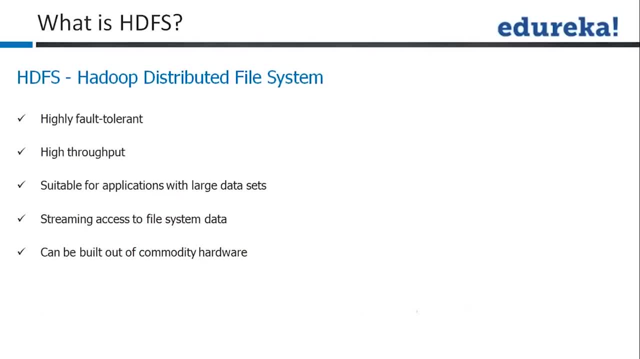 if required. so number one, it should be highly fault tolerant, okay, and it is built in in the system. I mean, see, we've talked about using a lot of data nodes to store data, so basically there's a good chance that some of these nodes can give, can become faulty over a period of time. 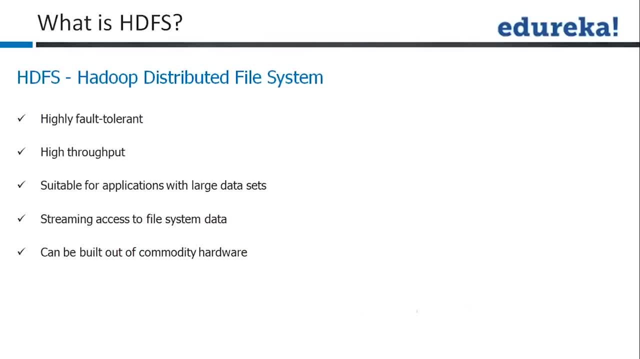 or at any point of time. so the system, the distributed file system, HDFS, should itself have a mechanism to make sure that it is highly fault tolerant. okay, for that. what we do is we replicate data on multiple machines, so a single data block is not stored in a single. 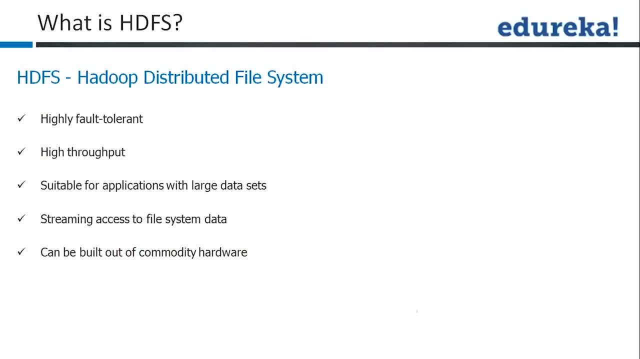 machine, but it is stored in a minimum of three machines. we will know more about it, but that's the way Hadoop makes the system fault tolerant. is that clear? So, by replicating the data, okay, in multiple data nodes, and not by using very high quality. 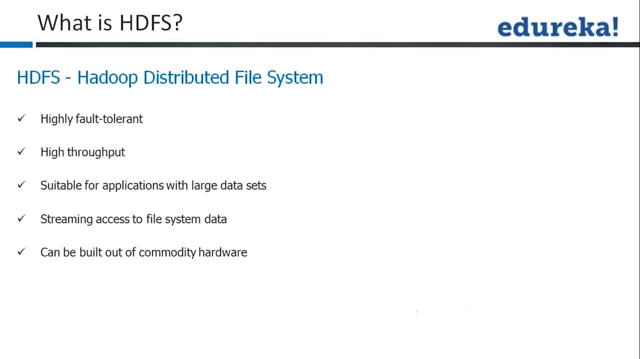 machines, high availability machines- okay, is that clear to everyone? First point: quickly, can you give me a smiley or a yes, Okay, the second point is how to high throughput. high throughput is something which is very clear, because we've just seen an example that 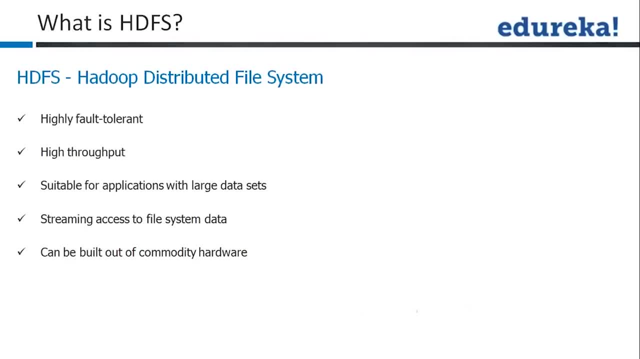 if I use a DFS, then I can reduce the amount of time it takes to read the data by one-tenth if I have ten node cluster. if I have a hundred node cluster, I can reduce the time by a hundred times approximately- not exactly- and if Yahoo uses something like a five. 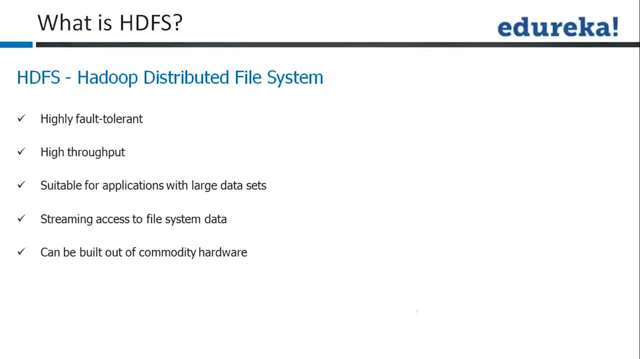 a thousand node cluster. so you can imagine how fast the throughput can be by using this simple mechanism distributing the data across different clusters. is that clear? How does that achieve high throughput? Okay, great, so then, okay, Sandeep says no. so Sandeep. 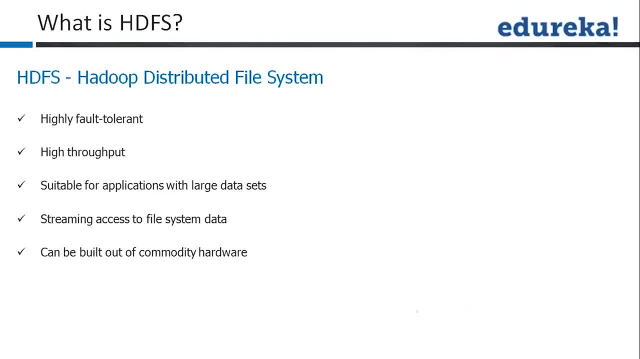 throughput is the amount of time it takes to read the data. okay, and by putting data across in parallel and reading it in parallel, you are actually decreasing the total time it takes to read that data. Okay, As we saw in that, another example of where we're reading one TV data from multiple machines. is that clear? 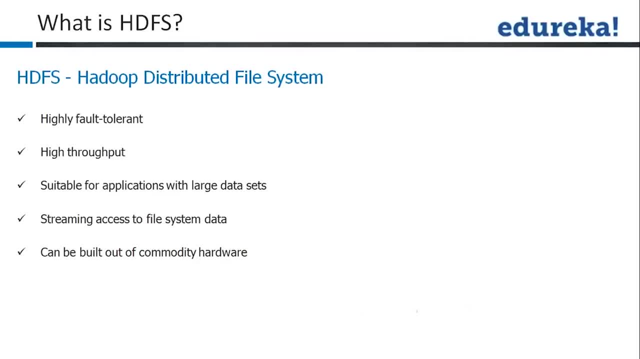 Sandeep. Yes, yes, Sandeep Gaurav, don't worry about data replication. I will cover that very soon, okay. Yes, we are getting the throughput right, right, right: divide the data and get. 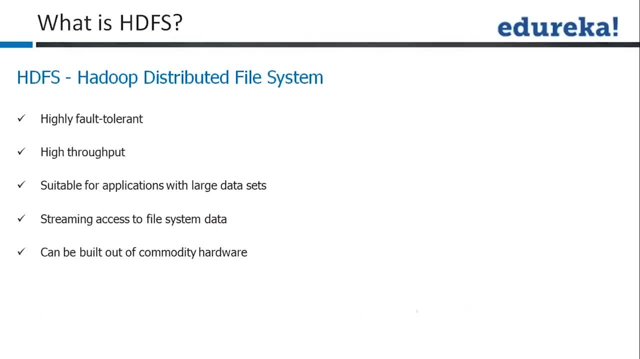 throughput right, but it's not all that simple, but it will. there are a lot of complexities involved and we'll look at that Now. Gaurav has asked me a question. replication causes data redundancy, then why is that pursued? 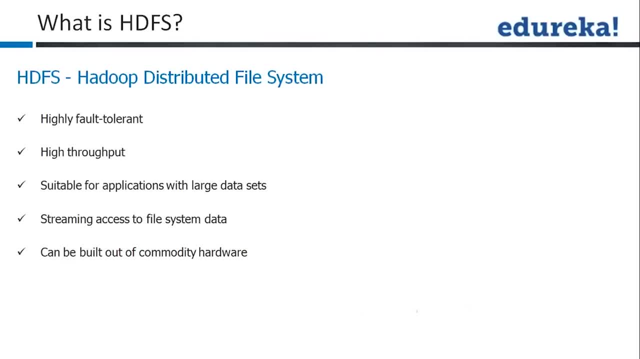 Okay. so the question is that I said right to make it highly fault tolerant. we replicate the data in multiple places. So, yes, it causes data redundancy and it is pursued because these computers, as I told you, are commodity hardware. the places where we store data are. 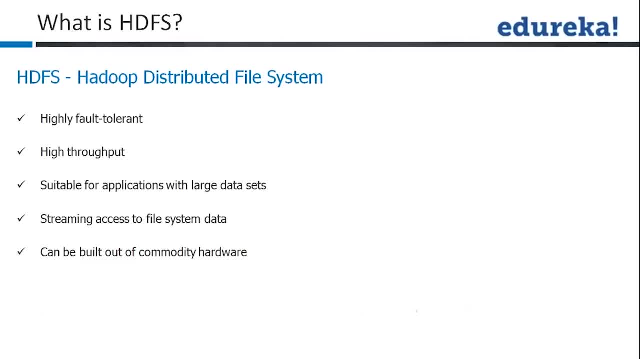 commodity hardware. they're not high quality, high availability machines, so there's a good chance that they'll keep on failing in between You. can I mean the Hadoop cluster can use your and my machine as well? okay, you don't. 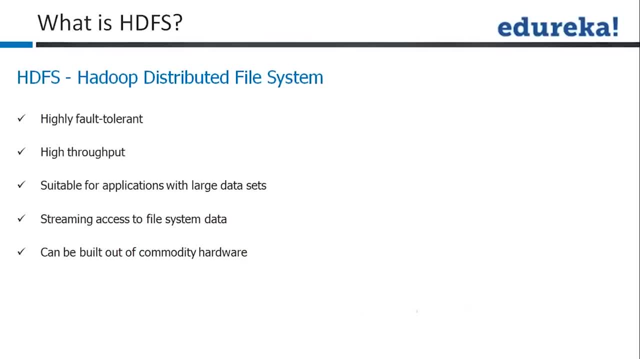 need high quality hardware there, So that is why we do it: to make it high availability. we replicate the data in multiple places and we will look at that once again as we move forward. okay, Is that fine, Gaurav? Is that okay to everyone that? why do we use? 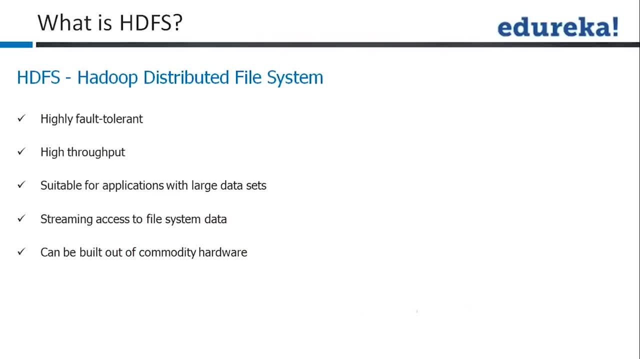 data replication Quickly. can you give me a smiley if it is clear, Great, okay, Great, thank you guys. thank you very much. So, and as I told you, it is suitable for large data sets. okay, So it's not. it's not suitable for applications. 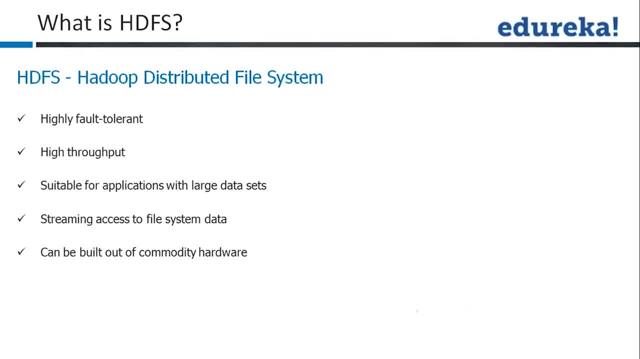 which have small files. okay, So even so, basically, since a lot of information is stored as metadata on the name node, I'll not I'll not get into more into it- it makes a lot of sense if we are storing this data, storing large amounts of data and not small. large. 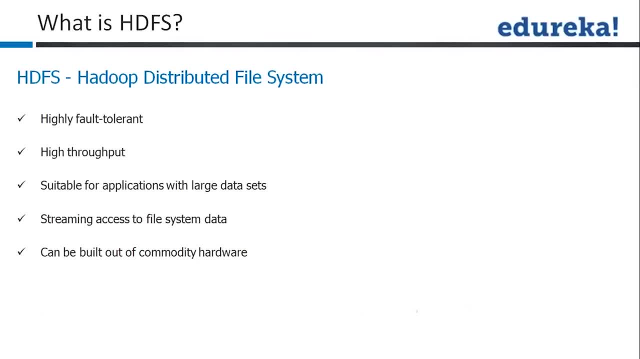 amount of files instead of using large amount of files storing small amount of data. it makes more sense when we have large sizes of files and less number of files. is that clear? If the data set is large, then it makes more sense. HDFS- okay, Each file is huge. 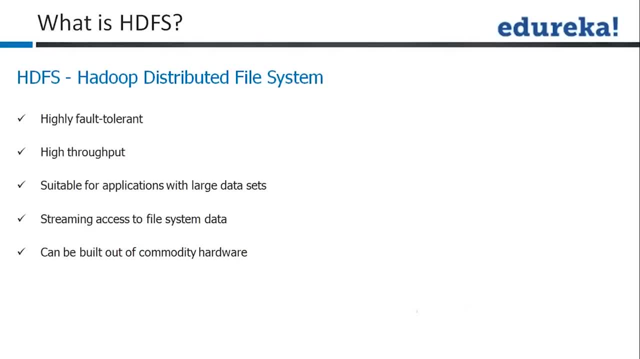 okay, Right, and you'll. you'll understand this very soon, okay? So Anand is asking me to repeat. Anand, I was saying HDFS is more suitable for cases where you have huge amount of data in a single file as compared to small data, small amount of data spread across multiple. 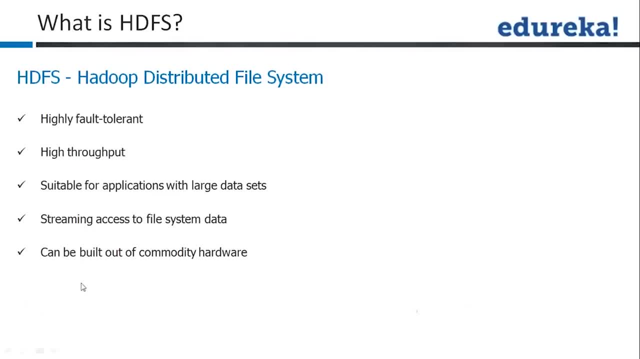 files. okay, Is that clear? And the next point is streaming access to file system data, which means that it should have. streaming access to file system data means that if we we are doing something like a write once and read many times kind of operation, which 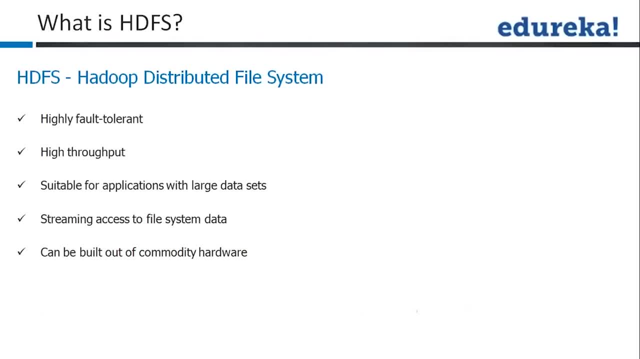 will be the case when we are analyzing logs. okay, So unstructured data, this will be the case. you'll be doing streaming access to data where you will not be updating the records again and again. that's very much different from a bank record, so that is where this 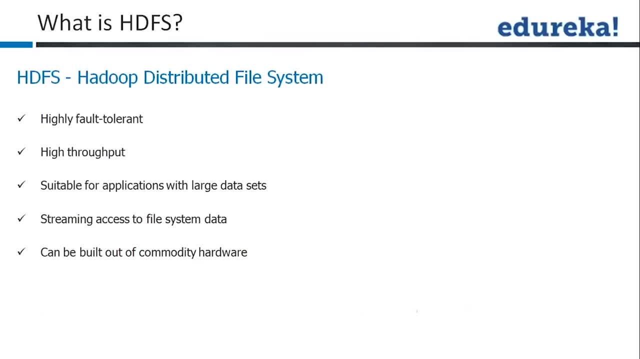 makes more sense where you write once and read many times: okay. And HDFS can be built out of commodity hardware, which means, without using any high-end servers, you can build the high-end storage devices. you can build HDFS. Is that fine with everyone? Is are. 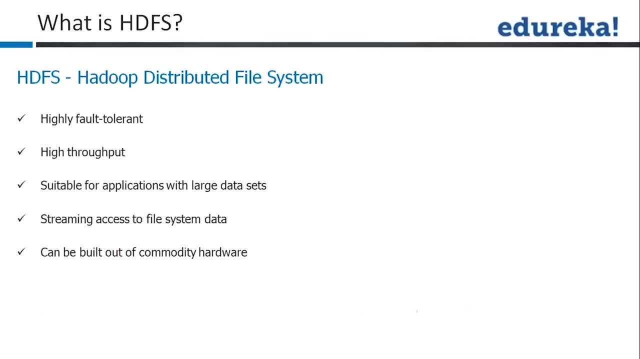 all these points clear to everyone. If nothing is clear, please ask me. it's important, okay, And otherwise please give me a yes or I'll just move ahead, okay, Thank you guys. thank you. Commodity includes yes, yes, it does. it does include RAM, because it has to run a. 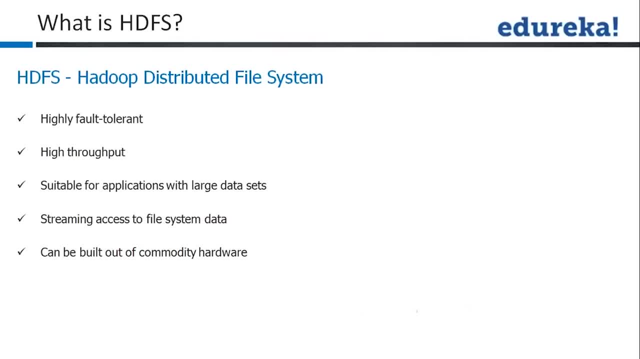 few things there. we'll talk about that, okay. So Anand is asking me a question: does commodity hardware include RAM as well? Yes, Anand, it does. it does include RAM as well. and the reason why it needs RAM? because there will be some services which will be running on. 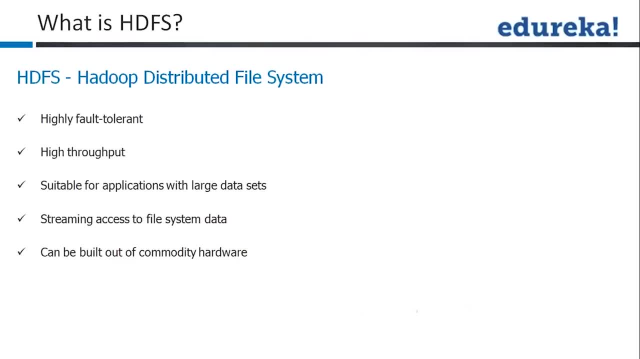 it. the task tracker which we talked about is something which runs on the commodity hardware itself. Okay, we'll, we'll know more about it. Okay, Sameer is asking streaming access. please explain again. So, Sameer, in cases where you're writing once and reading the data in one shot, where 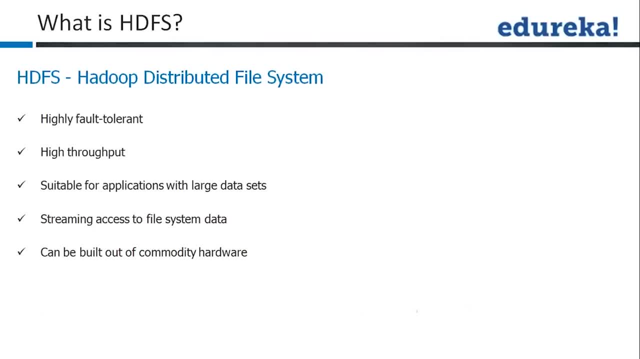 reading the complete amount of data is more important. the time taken to read the complete data is more important than than the time to actually fetch a single record from the data. that is where that is what streaming access is okay, Like a YouTube video, if you, if you want to. it's not important that you seek a particular 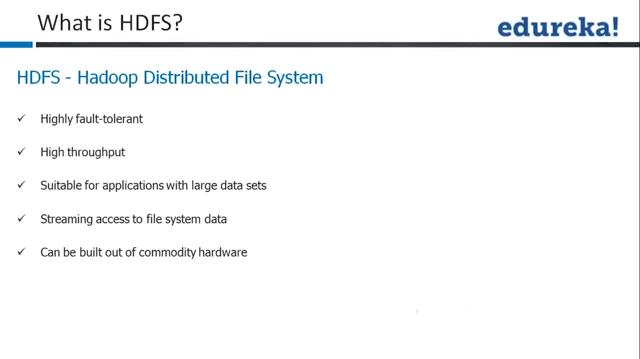 point in that video. more important is: how soon can you get the complete video? Okay, so, and similarly, the Facebook logs. you don't? you don't need to look at a particular what a person liked in that? okay, you need to analyze the complete data together. so 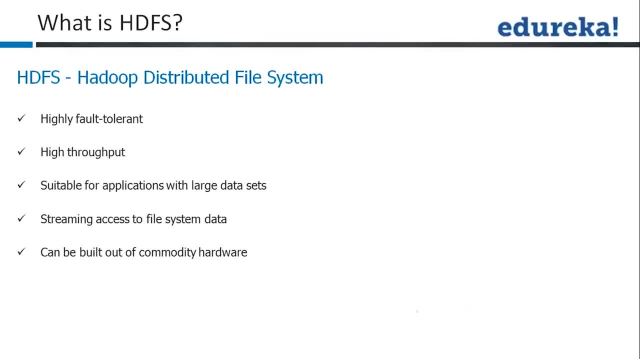 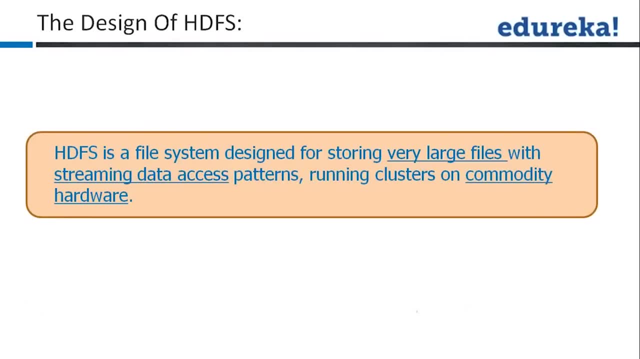 that is where, where you write once and read out multiple times, is what streaming access is. Is that clear to everyone? Is that clear, Sameer? Okay, great, So let's move on. I've written one more definition. I promised. I broke my promise. I'll do it again. Okay, so let's move on. I've written one more definition. I promised. I broke my promise. I'll do it again. Okay, so let's move on. I've written one more definition. I promised, I broke my promise. I'll. 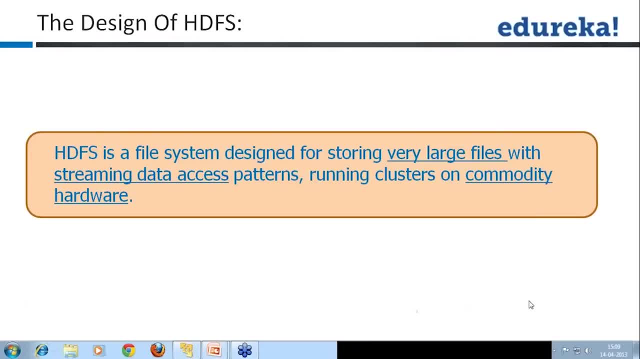 keep. I'll keep breaking my promises, so okay. so SDM is a file system designed for storing very large files- one very important- with streaming data access patterns- that's also very important- and it runs on commodity hardware. so these are the two, okay, Anand. 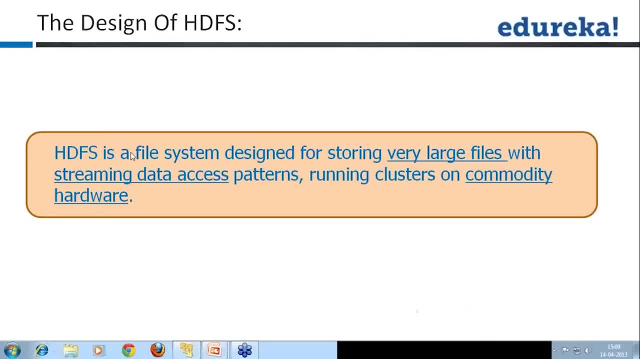 Kumara says promises always to break. thank you, Anand. thank you for supporting me in this. okay, so basically, three important points here: very large files, streaming data access and commodity hardware. these are the three salient points. These are the three salient points which you have to look at when you design a Hadoop distributed. 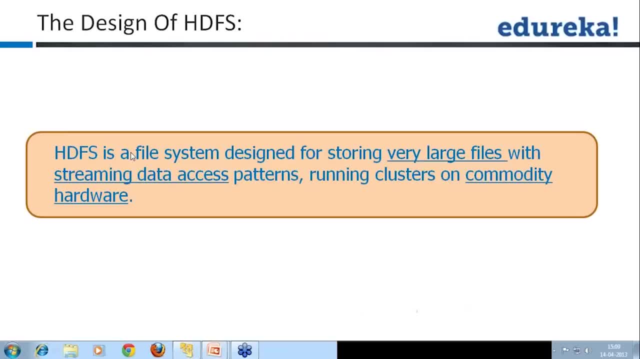 file system. okay when you, if you have to take a decision whether you should move to Hadoop or not, these are the things which you should look at. so people from the architecture kind of background or who are looking at, who are business analysts, if they have to. 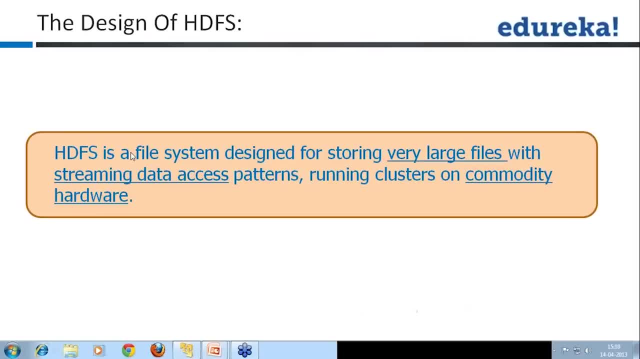 talk to your clients. these are important things. when the client ask them: why not? we also move to big data and Hadoop. you have to answer, you have to look at these points. is that clear to everyone? I believe Devasheesh was from that background, right, Devasheesh? 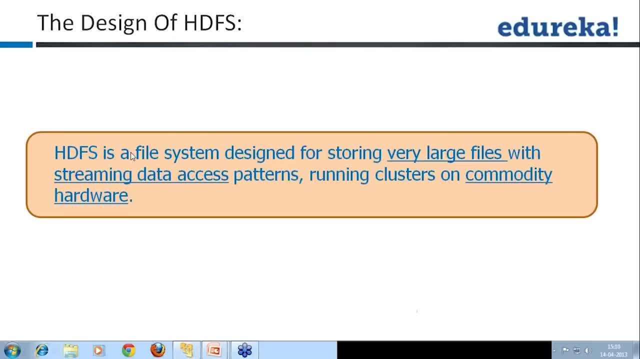 So you might have to answer such questions. so files should be in terabytes- okay, great. the file should be in terabytes- okay, great. so, Anupam, Anupam, you had given me your introduction, which I missed. I believe you are in the. you are an architect, is that correct, Anupam? 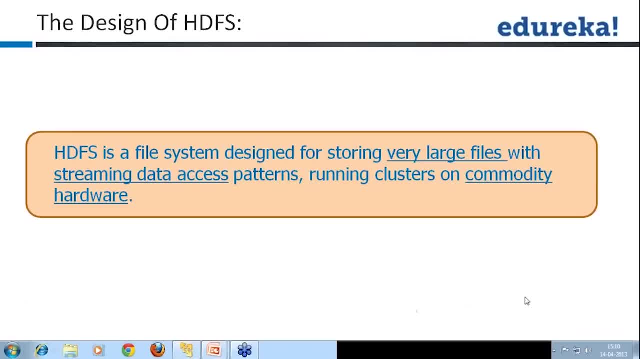 can you please tell me yes or no? okay, yeah, so people. no, I am sorry, Anupam, can you please introduce me to yourself? Okay, Anupam, Can you please translate this all once again? what do you do? okay, while you write, I will. 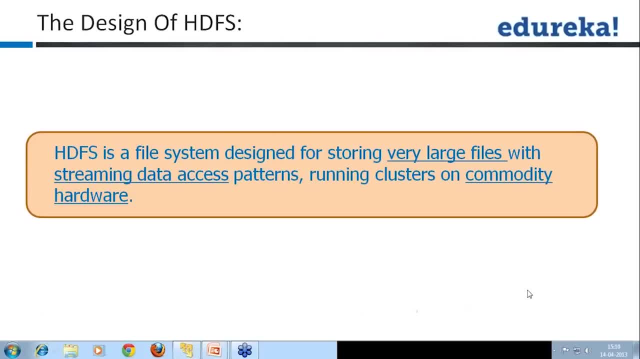 explain so people who are going to take these decisions in their organisations or are going to talk to clients on these, where a lot of clients, because of the hype around Hadoop, they will be asking why we should also move to big data. okay, okay, okay, you are an. 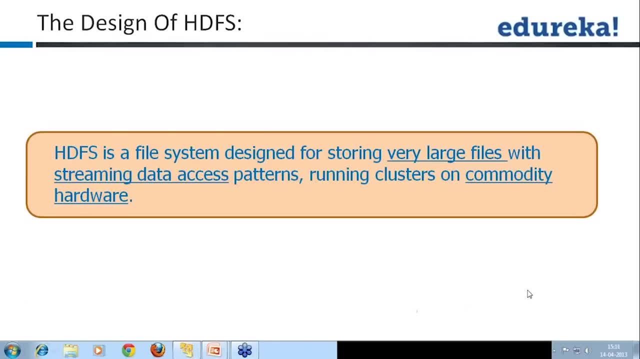 ETL developer: okay, great, so okay. okay. so you work with TCS with 6 years of experience- great, great, so yeah. for you, probably PIG and HIVE will make more sense, which is fine and yeah. 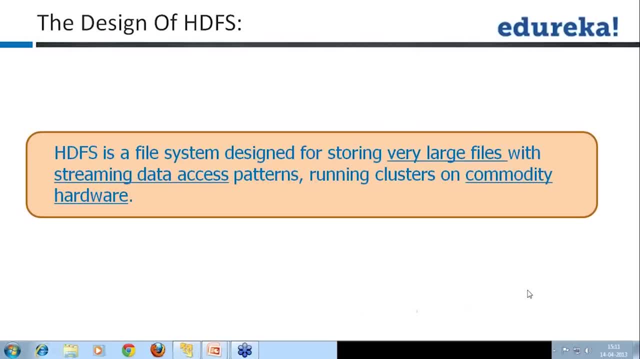 So, basically, for people who are doing, who are into this, decision making, whether we should move to Hadoop or not, whether we are ready to take this big data, these are the things which you should look at. Okay, is that fine? 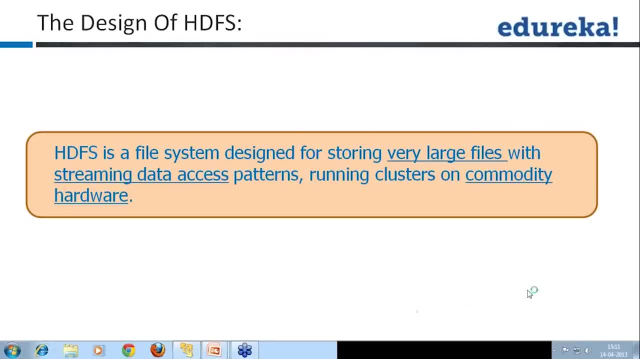 Rohit is a solution architect and Rohit says: I am a solution architect and these definitions will really help me as I have to read between lines and explain our customers. So you keep breaking your promises. Yes, thank you, Rohit. Thank you, Rohit, that I could actually help you in talking to your customers. 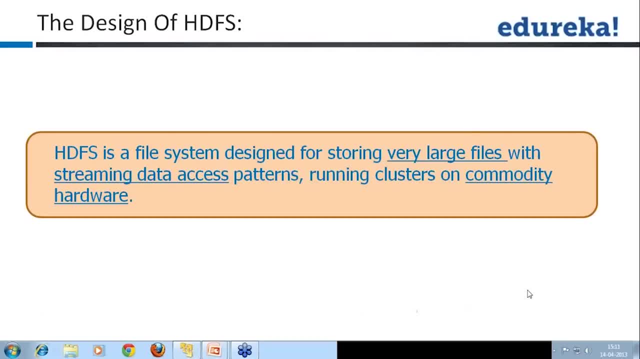 Thank you very much. So, yeah, very important point, very important definition. Some definitions I will keep here and unless and until I believe that definitions are not important, I will not keep them, But in this case it is very important. Okay, so, even if you are not a solution architect, even if you are a developer, it is very important to understand the bigger picture. 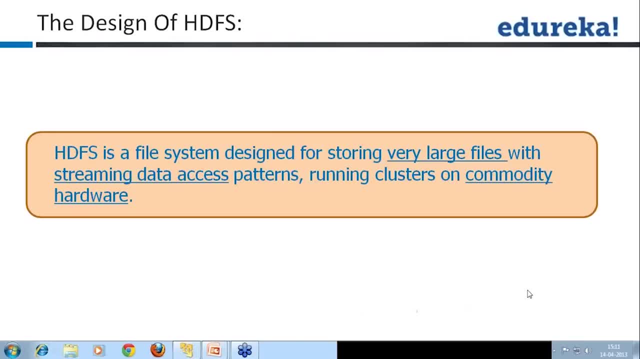 Okay, and otherwise you will just be doing some what I should say bull's job, not donkey's job. Okay, so let us move ahead. Can I get a quick A smiley from everyone if you guys want me to move ahead? 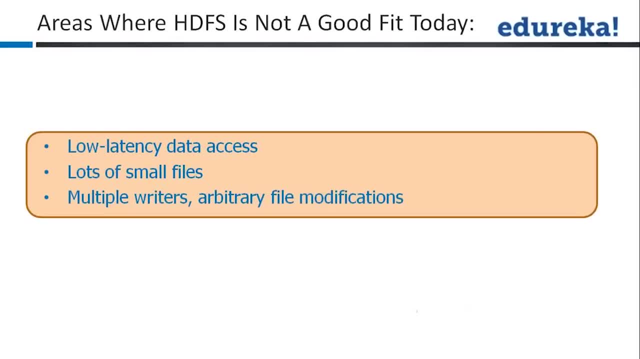 Okay, and then I will tell you where HDFS is not a good fit today. Again, Rohit Mohan, please pay attention here. Ajay, all the people who are looking at telling people and telling people to implement Hadoop, please make sure that. 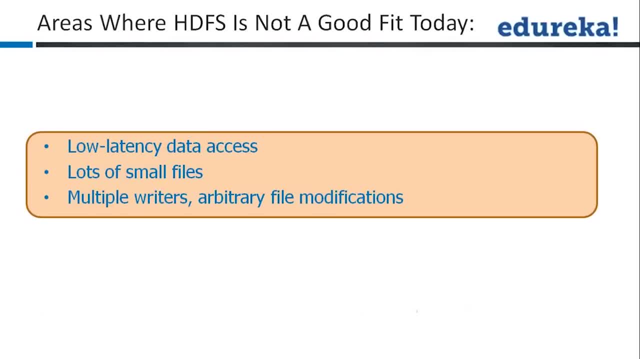 Okay, yes, thanks Anand. Okay. so where you have low latency data access, which means that you have to quickly read a record for a bank kind of transaction, kind of thing, Please don't move to HDFS, even if you have a huge amount of data. 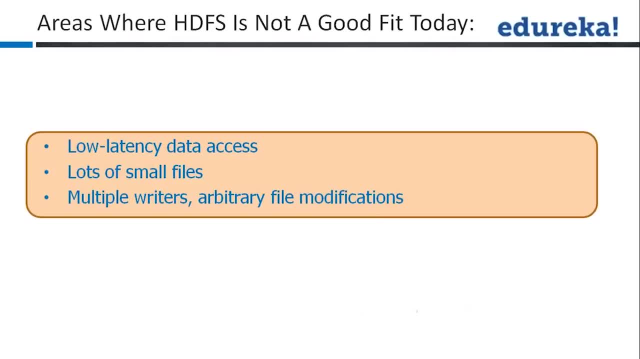 Okay, fine. Lots of small files again, because the file information is stored in as metadata. And if you are, yeah, I'm telling you that Sandeep, just give me one second. Okay, because one if you store these. see, Sandeep is asking me why. 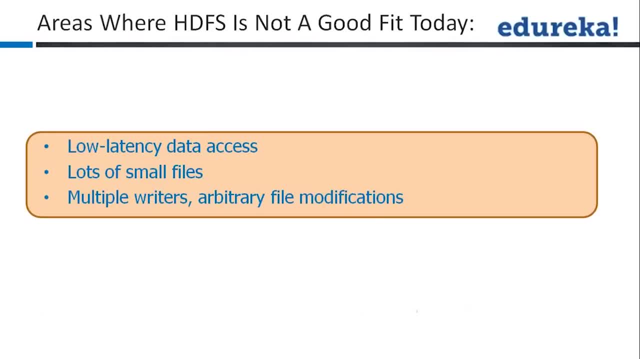 Okay, and I'll answer this question as before. we move on out of this. Okay, and when I say where HDFS is not a good fit, I also Add something called today. So going forward, Hadoop is working on it. 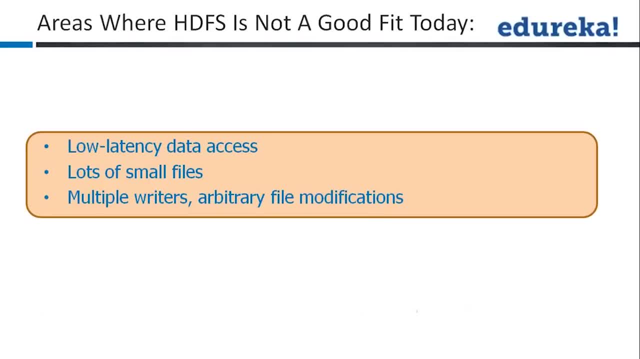 It might become possible to do all these things also as efficiently as a traditional database can do, But as of today, Hadoop is used for reading out huge data sets in one single shot. Okay, if you are. if you want to seek a record from a file, this probably is not the best way of doing it. 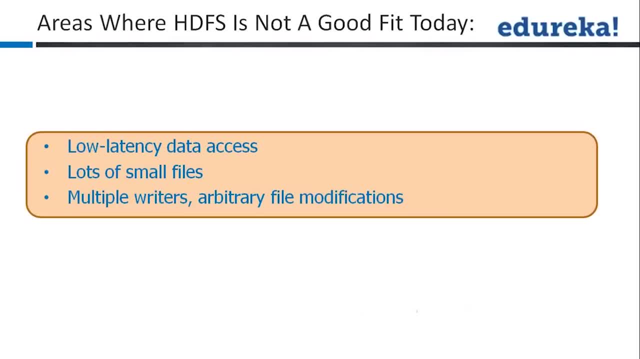 Okay, because you will not know where a single record is kept. The information is kept at a very, very high level in terms of blocks, And The data is usually unstructured. There are no tables and columns. The data is stored as multiple logs. 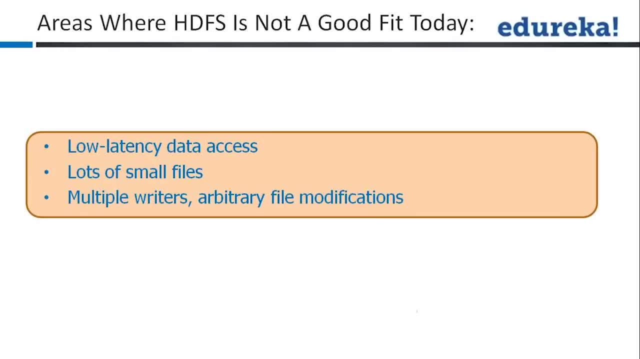 Okay, and if you have a lot of small files, then also this doesn't make sense, Because for each file you'll have to store a metadata which will make things very difficult to seek whenever you want to. Is that clear? Is that clear to everyone? 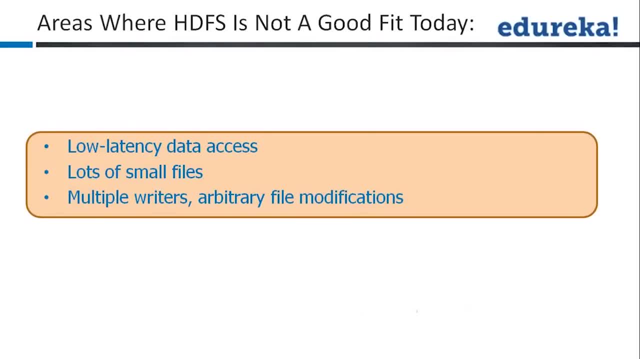 Okay, and that's most important point- is that if you're writing data multiple times and if you're doing arbitrary file modifications, HDFS is not a good fit. Okay, which means that if you're updating the data again and again- the same row or row, same column again and again- then HDFS is not the right place to do it. 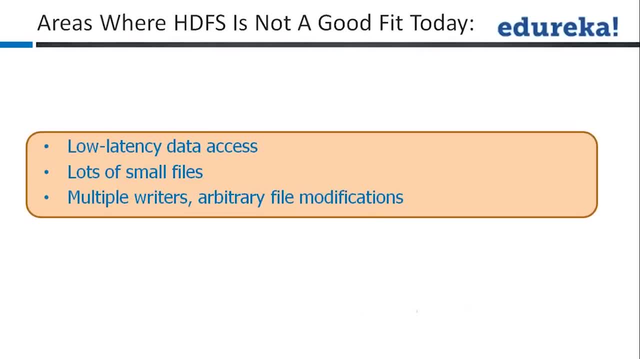 A traditional RDMS works better. Okay, so see, Rohit is asking me a question: If not Hadoop, then which tool is a good fit today? Any recommendations? So, guys from the from the Teradata and Oracle background, can you boast about that? 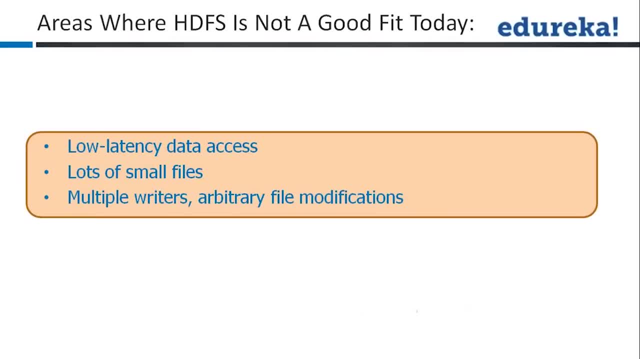 Now can Sayyed answer that. Sandeep, just give me a second. Sayyed, would you like to answer that question? Yes, RDVMS will be used for this right. So, Sandeep, the question is: low latency data access means that if you have to quickly seek one data, one particular data from a file, okay, then this is not the best thing. 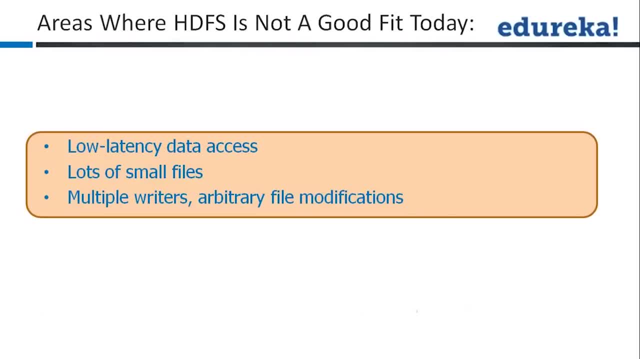 Hadoop is better when you have to read the complete file in one shot and then do analysis over it later on. Okay, Okay, now there are. there are frameworks which are available on top of Hadoop- as big actually is, is something which which can do some SQL like operations. 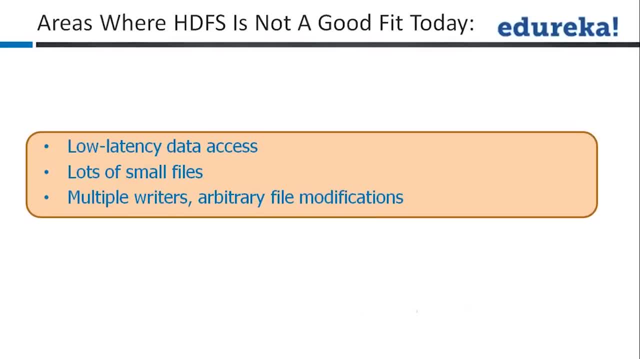 Hive is the Hive is the place where you will be doing a lot of analytics there. We will talk about those as we move forward in the course. Okay, fine, Sandeep, is your question answered? See, I'll not get into details of any of these things right now because not everyone would be interested in it. 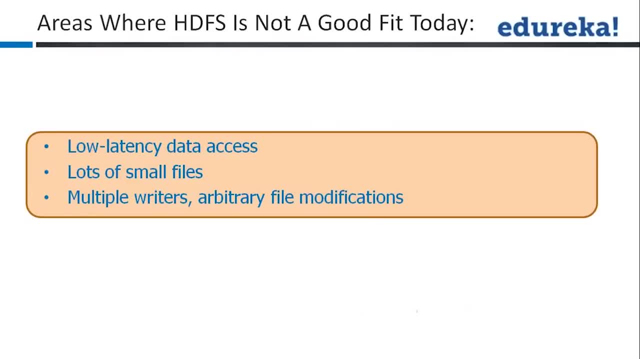 Right now number one, and not everyone will be able to understand it also. So please be patient with me, and some answers I'll give you later on. Okay, As we move, I mean I can, I can ensure if you attend all the eight classes you'll understand everything. 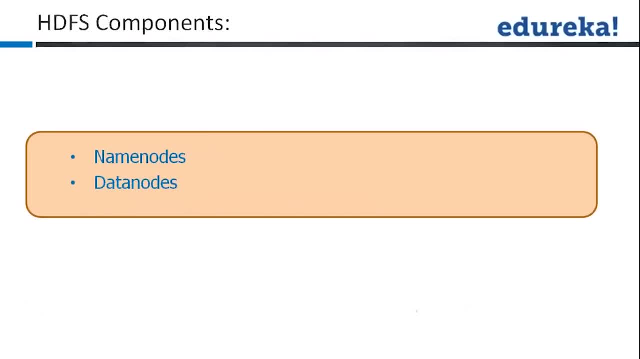 But today also, you'll understand HDFS. So can I move forward, guys, if this is clear to everyone? Okay, I'm getting a lot of yeses, Great, So now. now we talked about name nodes and data nodes. Now it's time to remember. 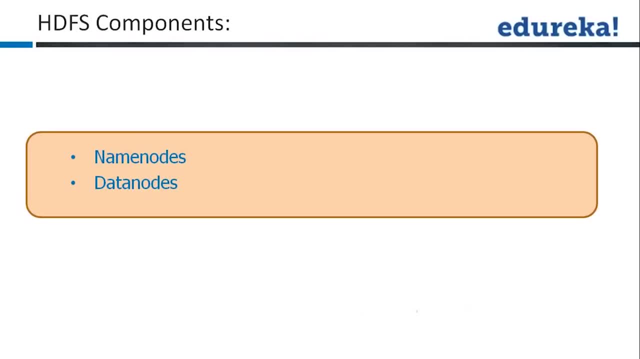 What I told you in that slide where I told you just remember something. Okay, so there was something associated with the name node. Can you quickly answer that on the chat window? What was associated with the name node? I'm getting some answers. 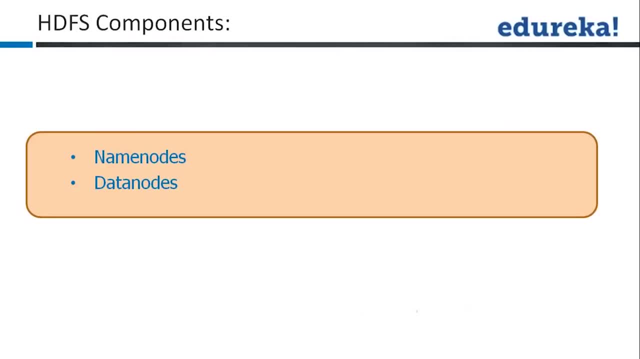 Okay, okay, okay, Sandeep, I did not tell you that. Okay, so everyone has given me the answer, which is job tracker. Okay, Yes, So job tracker is the thing which is associated with name node. Okay, 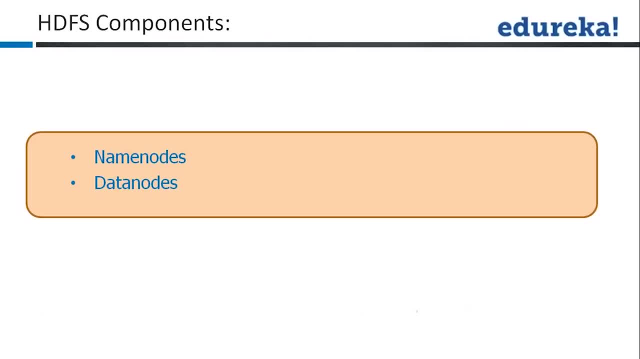 Yeah, And data nodes. What was that with data nodes? Task tracker, Correct, Correct, Correct. So basically there are two major components of HDFS: One is the name node and the other one is the data node. Name node is the master node. 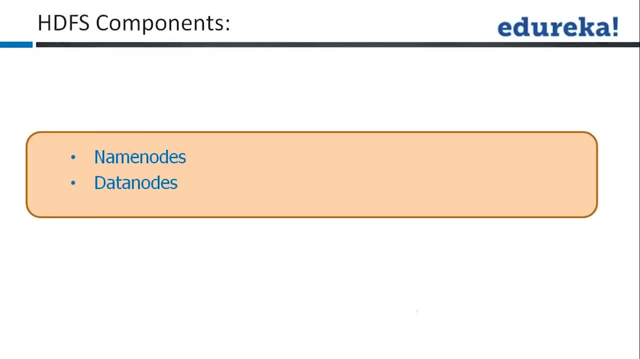 Okay, On which the job tracker runs. Okay, Job tracker is a daemon Right Which runs on the name node And data node is again that commodity hardware on which another daemon called task tracker. Okay. So now I'm introducing these two terms in slightly more technical language. 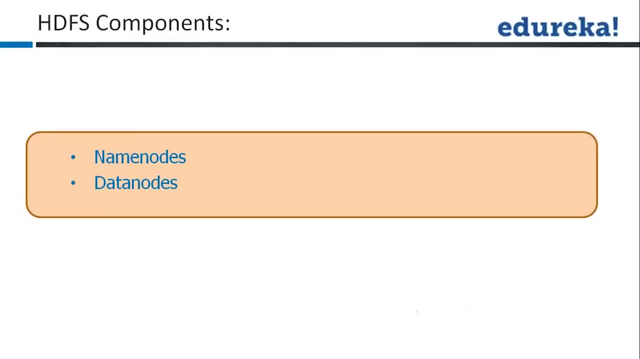 But going forward in the next couple of slides we'll understand more details about it. Okay, Is that fine with everyone? So major components on HDFS is name nodes and task tracker and job tracker and data node and task tracker. Okay. 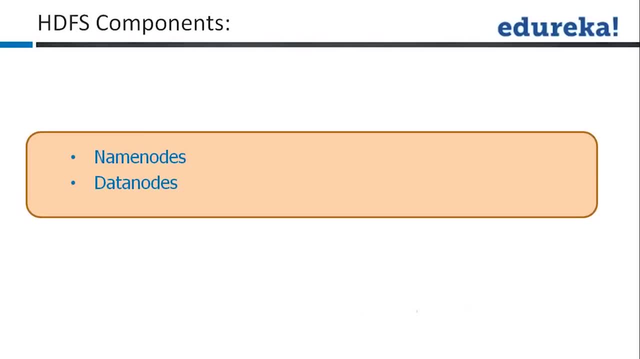 Okay, Sameer is asking: what is a daemon. Can anyone answer that question? What is a daemon? Quickly, Okay, Rahul wants to answer that question. Rahul is with me. Rahul, you want to answer that question? Hi, everyone. 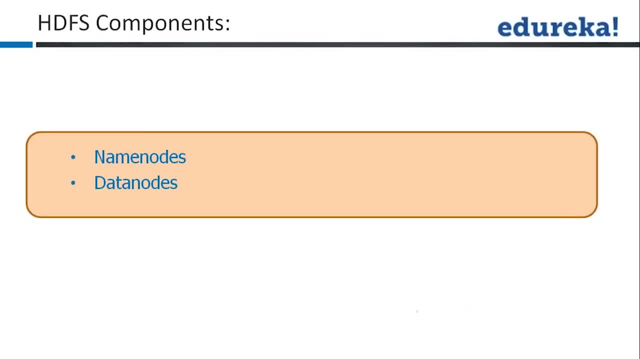 This is Rahul Sameer, to answer your question. what is a daemon? Yes, It's basically a process or a service that runs in background. It's a very well said, Mohan. It's a resident program. It's a resident program. 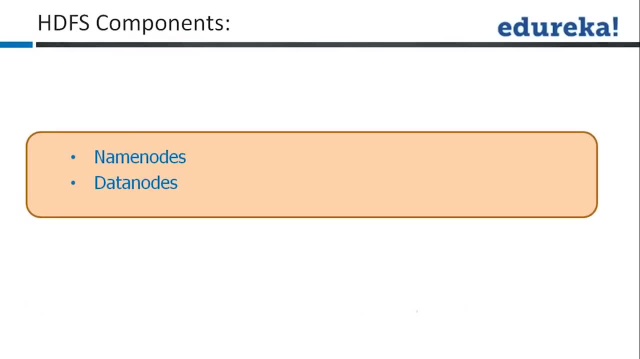 And it is a service. It's a service that runs in the background. You can call it a process also. Okay, So that is what a daemon is and is used in the Unix environment. This terminology is used in the Unix environment in general. 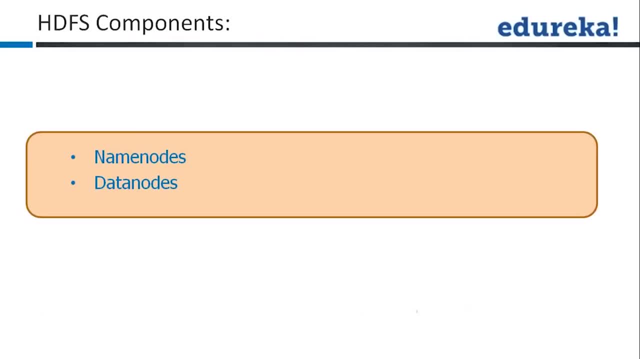 Does that answer your question? Sameer Mohan says the equivalent in Windows is a service. Yes, Mohan, It is a service in Windows And in DOS is a TSR. Yes, definitely, That's a definite yes, Yes, it's a TSR. 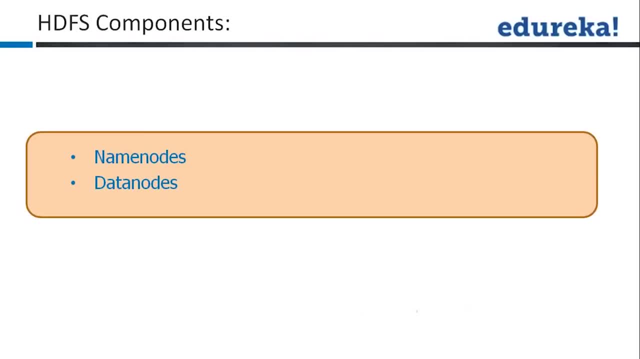 So I'm handing it over to Abhishek now again. Yeah, So thanks, Thanks, Mohan, for the insight. So Mohan has told us more about daemon. So Mohan says that, yes, they run in background, Sameer. 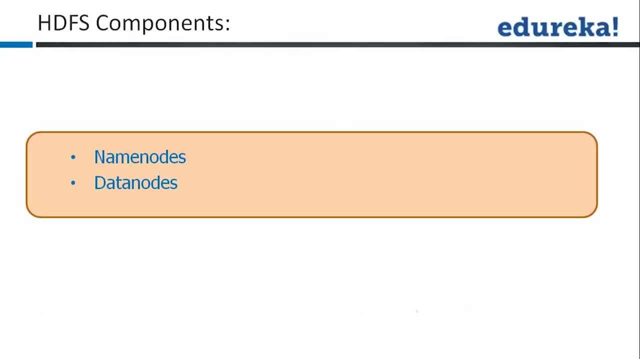 So Mohan has given us some very good information. Mohan tells us, in Windows equivalent of a daemon is a service, And in DOS it's called TSR. Okay, So can we move ahead guys? Okay, Yes, Sameer. 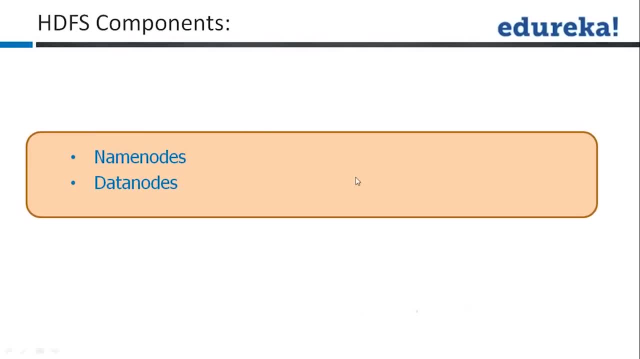 Yes, Okay, Guys, I'm really sorry. I grabbed a couple of chips in between while I handed over the mic to Rahul, So if you're hearing some crunching noise, I'm really sorry for that. So Mohan is giving me one more thing. 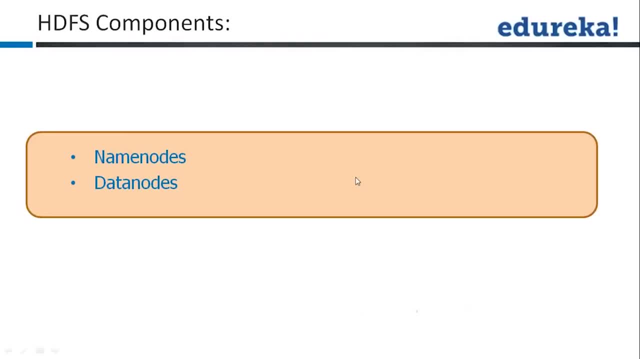 Mohan is saying: I am proud that I am going to be the only ex-DOS programmer here. I am the only one. There won't be anyone, Okay, There won't be anyone else who is a DOS programmer. Anyone else who is a DOS programmer here? 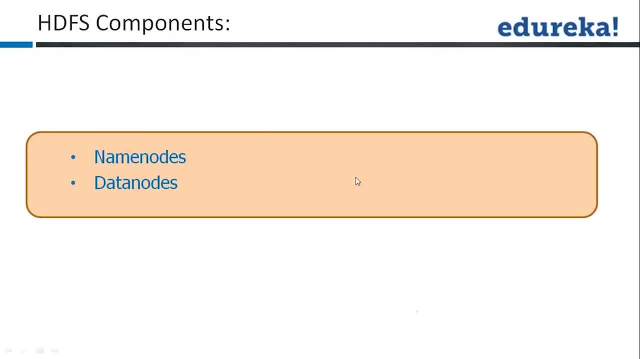 Mohan, I have done something in school, Okay, But I'm sure I've not done anything as much as you would have done in your days. So Mohan is an ex-DOS programmer, And is there anyone else who has done programming in DOS? 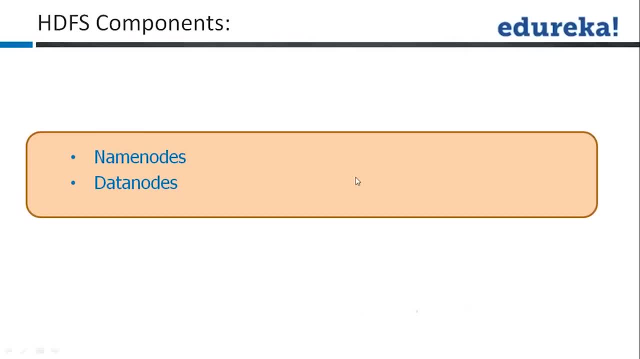 Syed Munawar is again saying: I've done it. So, Mohan, you're not alone In school. Okay, Hey, Mohan. Mohan, thank you very much. Mohan says I've written the first version of Norton Antivirus in DOS and Windows. 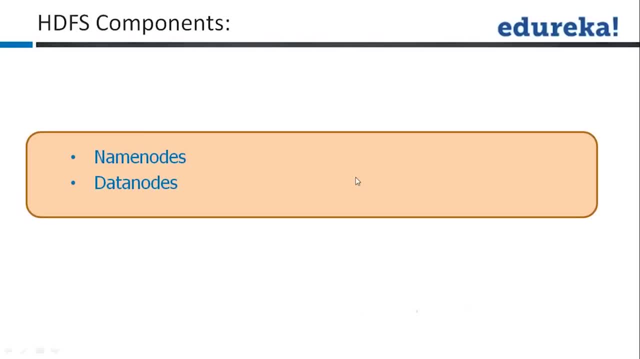 So Mohan, really, really great to have you here. I'm sure we'll learn a lot from you. sir. So Mohan is the guy who has authored the first version of Norton Antivirus in DOS and Windows. Great, Great to hear that. 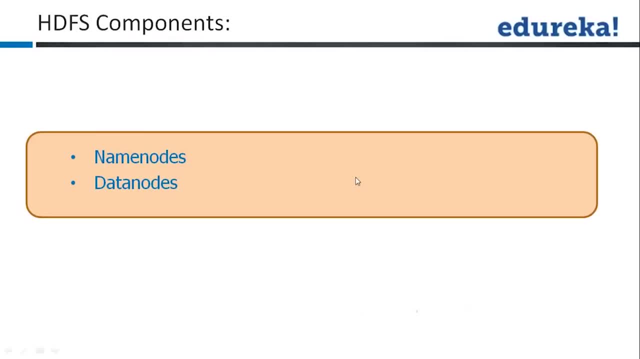 Can everyone give me a smiley or a clap for that guys? Wow. Syed says wow, Great clap says Gaurav. Awesome Mohan says Rohit Malik, Okay, With claps, he has shown. 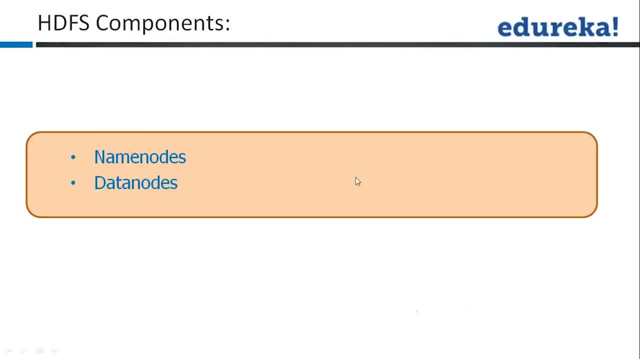 Ajay has given smile. A big applause from Anupam Mohan rocks says Rahul Tiwari Clap for Mohan, Anand Kumar. Okay, Great guys. So thank you very much everyone for appreciating Mohan's effort on antivirus. 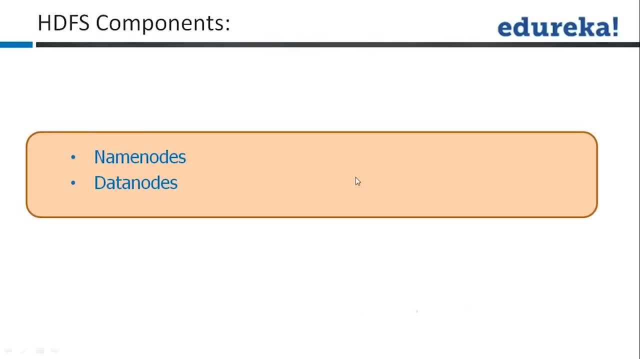 Otherwise we would be right now. Maybe some virus would have been injected in this system itself And we would be. We would have gone for a toss. I could not crack a joke here. I'm really sorry guys. Not every time I'll be able to do that. 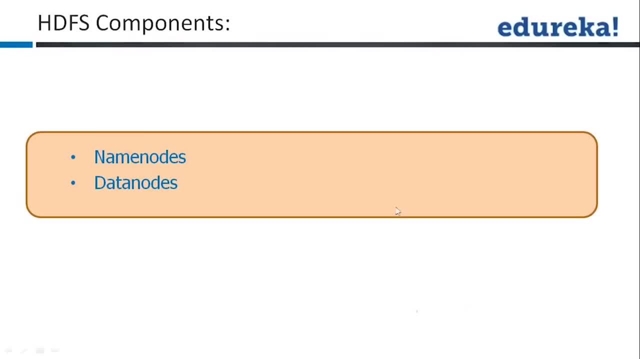 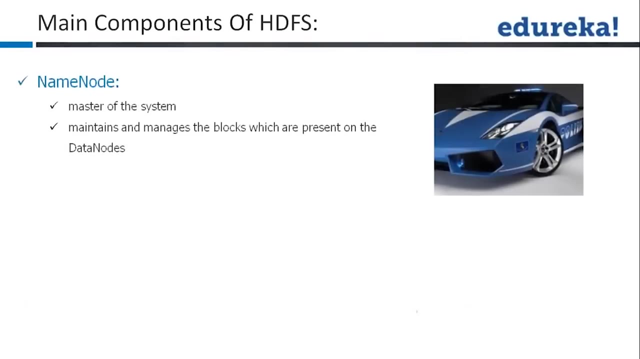 Okay, Mohan says it's ancient. Mohan, you're young. Okay, So main components of HDFS. Okay Now. okay, Now we have. I've put a picture here. Can everyone identify with this one? Can anyone identify with this one? 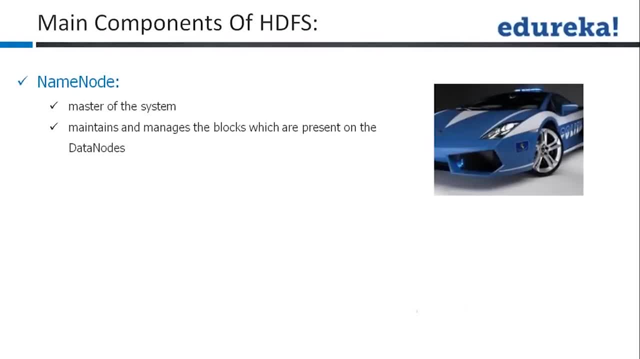 Can anyone tell me If anyone has ridden this vehicle any time? Mohan, I'm sure you must have been. You look like you must be having really deep pockets with all those authoring And you've exited from your company as well. 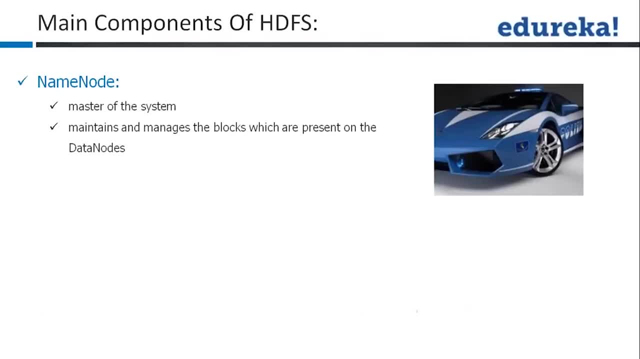 Okay, So everyone has. This is their dream car. Mohan, have you ever taken a ride in this one? Rahul Tiwari has taken it. Great, Rahul. where did you get a chance to do that? This car, Mohan, can you? 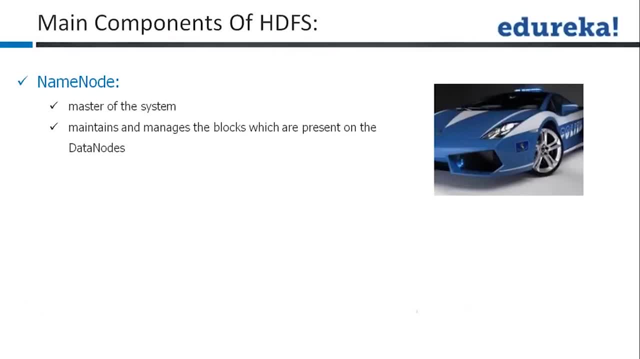 Can you identify this one? Sameer has also done it. Sameer, Sweden. Okay, Great, So this is a Lamborghini. Okay, Sandeep tells me, I also have taken this in dream. So with whom did you dream this, Sameer? 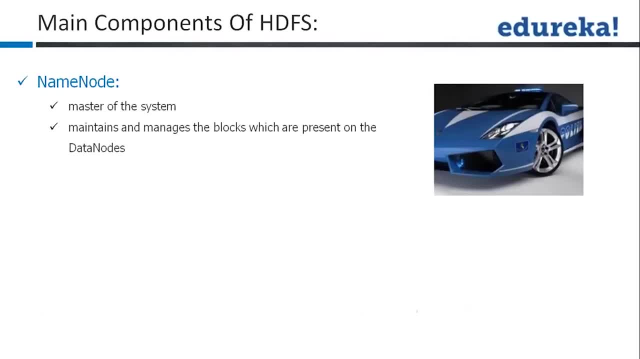 So sorry, Sandeep, Katrina Kaif, Oh, your tasks were covering. But okay, Sandeep says my wife, Okay, Okay, Sure, Sure, Sandeep In your dreams, Okay, That's really good man. 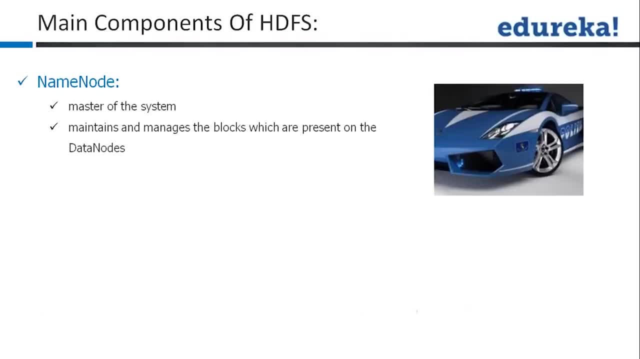 Really loyal husband. Your wife will be happy to hear that that in your dreams you dream about her, And that too, in a Lamborghini. Okay, So, Mohan, did you take a ride in this one? Okay, Gaurav says Sandeep is a liar. 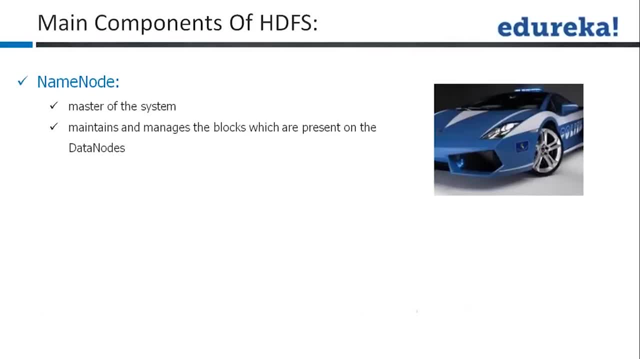 So it's getting great here. We have got a great environment here, Okay, Okay, Okay Okay. Mohan says not wealthy enough, Okay, Okay, So Gaurav. Gaurav says Sandeep is a liar. Okay, 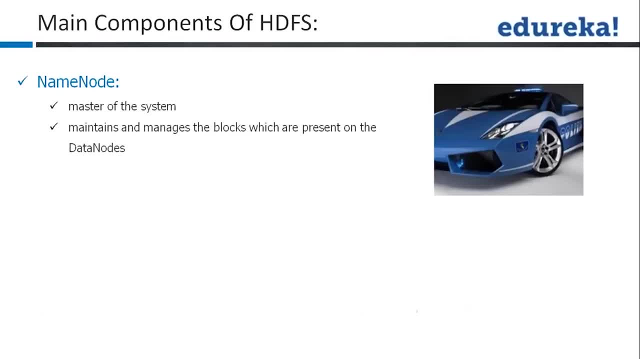 I kind of agree with Sandeep, with Gaurav, or with Sandeep, I don't know. And Sameer is giving me a smiley. Okay, So now the reason. I mean, let's get a little serious here. 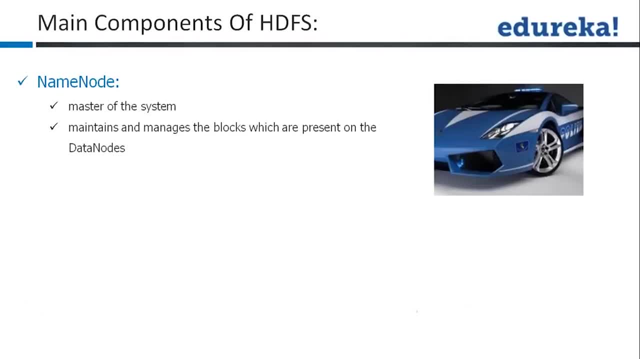 The reason I put it here is that this is the name node, and the idea behind putting this car here is that you need to understand that we have to put a very, very reliable hardware here. Double, triple redundancy hardware- Okay, High reliability machine. 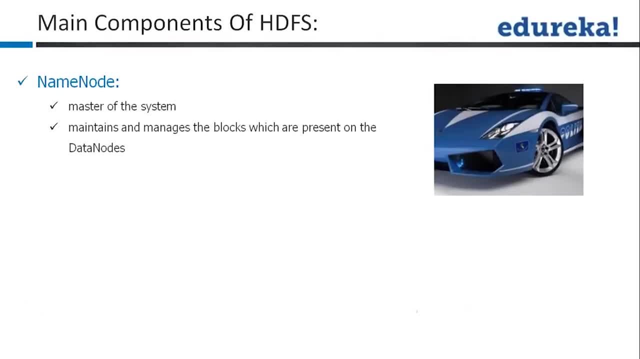 You might end up putting a raid here. Okay, So name node is the master of the system. It maintains and manages the blocks which are present on the data node. Okay, Please note that it doesn't store any data. It maintains and manages the blocks which are present on data nodes. 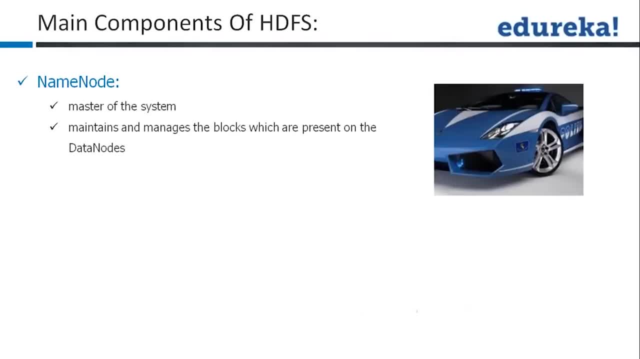 So it is the data nodes which actually keep the data. Okay, Is that clear to everyone? And the reason why I put a Lamborghini here? it will be a very, very expensive hardware and it will have a double and triple redundancy there. 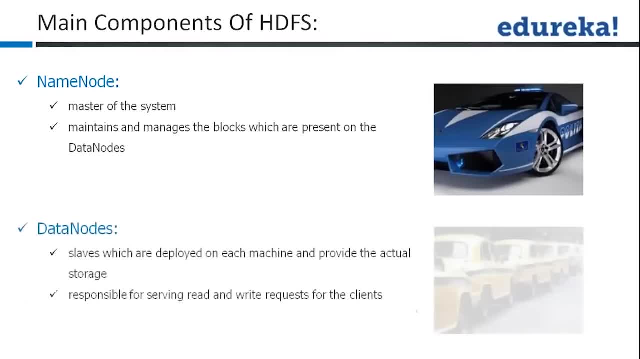 Okay, Is that clear? Okay, Now, can anyone identify this picture? Sandeep, have you taken a ride in this one in your dreams? Kolkata taxis? No, Sandeep doesn't dream about ambassador. Okay, So these are ambassadors. 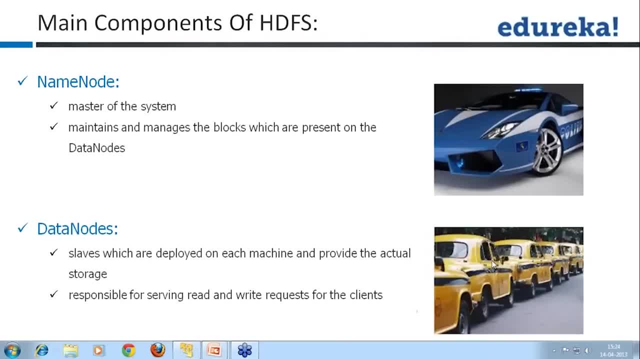 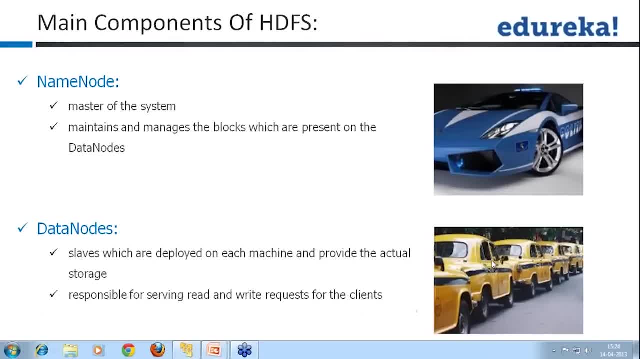 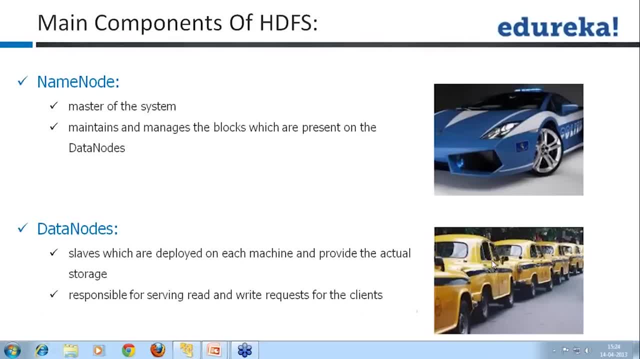 Oh. so Vidya Sahab told me: oh boy, I thought you would go with nano. Okay, Saya tells me, still in Kolkata, these are the taxis which are run Now Iactuallyactually, Ambassador, is much more expensive than a Nano, but I still. 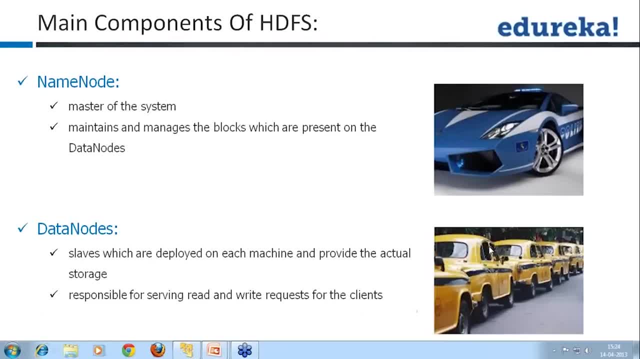 would like to take this analogy to tell you why I said commodity hardware. okay, So a name node is like a Lamborghini and the data nodes are like ambassadors. Okay, does that? does that? did you like this analogy? Do you want to praise me on this? 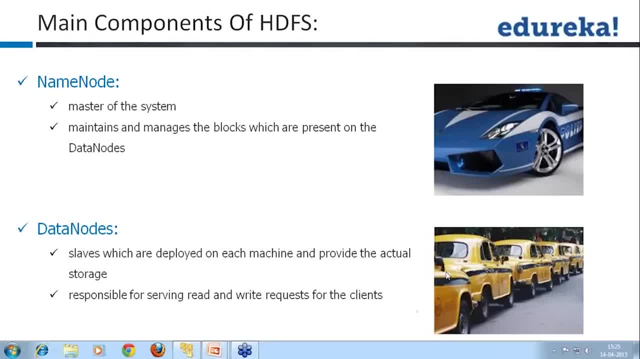 Okay, so don't praise me. It was put by Hisham, who is the guy who is in the support team. I just take the credit. Welcome to GoToWebinar. Web Events Made Easy. Welcome to GoToWeb. 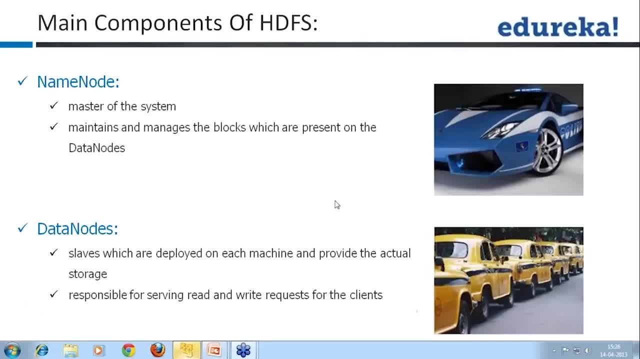 Welcome to GoToWeb. Welcome to GoToWeb. Is that fine, Can? is that okay? Everyone is able to hear me. guys Now back. am I back with you? I did not get any response. Okay, great. 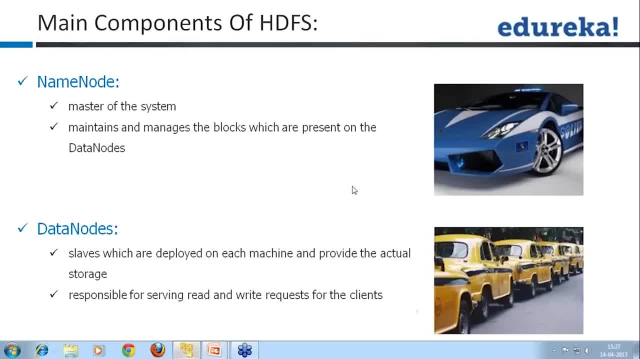 So sorry for that. Okay now. now data nodes are we say? when we talk about data nodes, these are slaves, as I said earlier, deployed on each machine and provide actual, actually the actual storage happens on data nodes and not on name nodes. 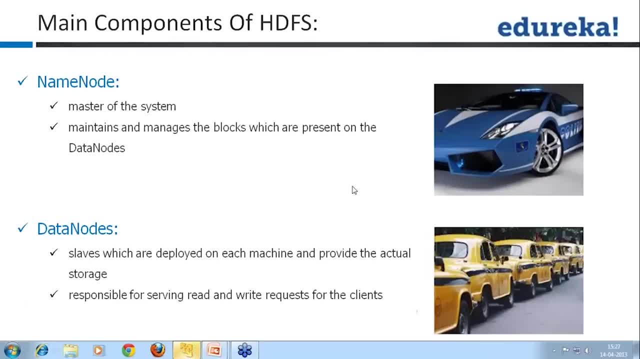 Okay, and these are responsible for serving read and write requests for the clients. Okay, so the read and write actually directly happen from data node. Now, don't worry about that, I've just said something: that read and write happened directly from the client. 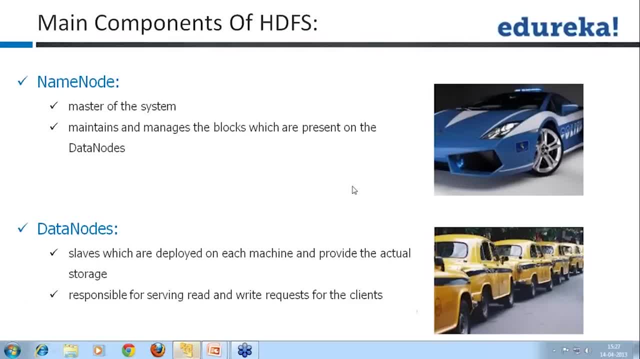 I'll explain that in detail as you move forward. Okay, just keep this thought in your mind. Okay, is that fine guys? Can I move ahead? Yes, Mohan, the task tracker runs on each data node. Okay, great. 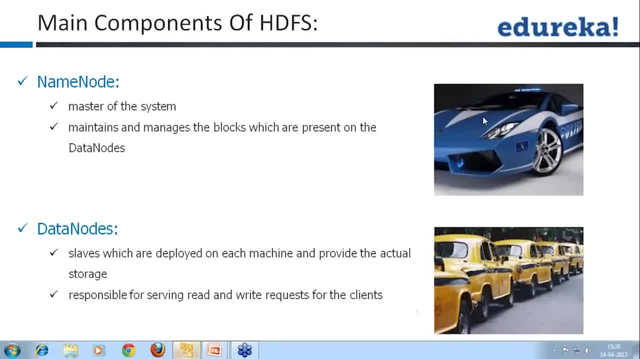 We'll, we'll, we'll, we'll understand all this. I'll ask you questions in the end of the class and I'm sure all of you will be able to answer that. Okay, Sandeep is asking me a question. 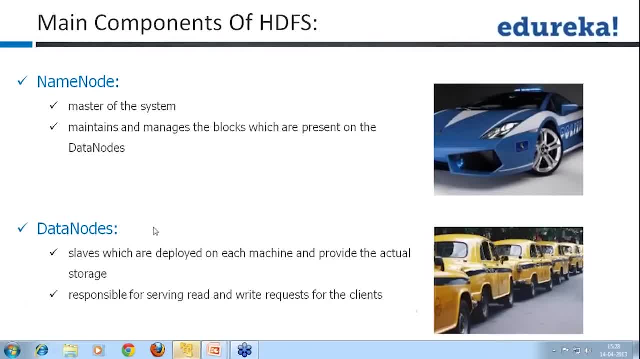 If data node increase, then do we need to upgrade name node Sandeep at the at the beginning of the, when we define the system, we see that, okay, what till what level do you want to scale up the, scale up your cluster? 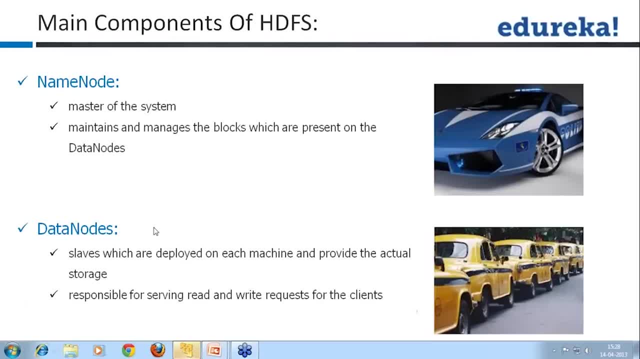 Based on that, we choose a name node Most of the times. yes, you do not have to upgrade your name node If you increase the number of data nodes, because data node does. name node does not store much information, It is just RAM and it it stores. it stores mostly the metadata. 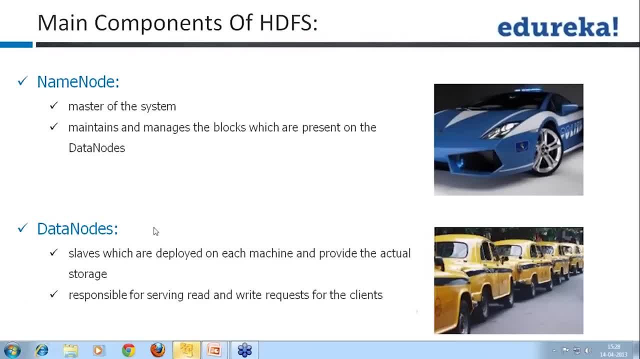 I'll I'll I'll make you understand more about this. Anand is asking a question which is an interesting one. He says two servers are required for name node, data node. Well, ideally, in the real world, there will be a name node which will be on a high availability software. 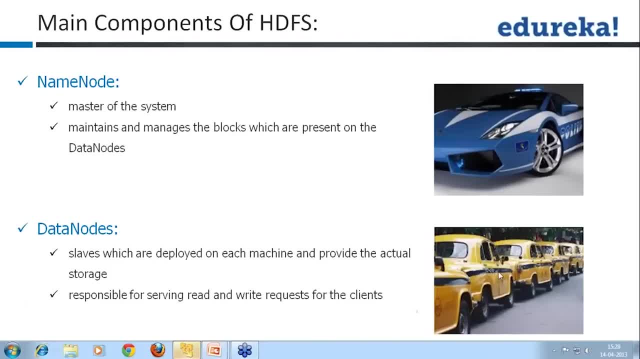 hard machine like a Lamborghini, and data node will be like ambassadors. But if you want to try out something, then a same machine can be used to create one data node and one name node. Okay, it can run on the same machine. 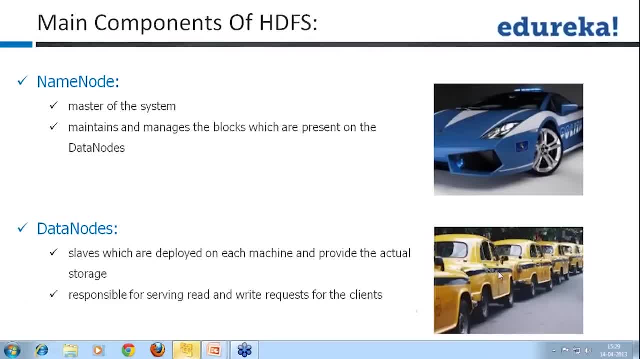 Okay, now Mohan has asked me a question: is the name node also commodity? No, Mohan, that was the whole point in actually putting this Lamborghini picture here. Name node has to be a double, triple redundant machine which can be even a RAID. 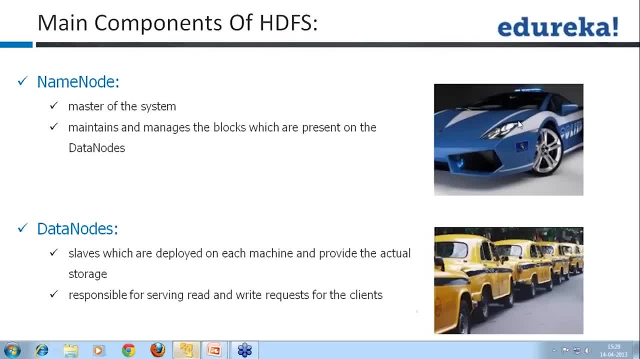 Okay, so it has. it cannot be a commodity hardware, Because this is the single point of failure in the system. And when I say single point of failure, I'll explain it, So don't worry about it right now. Okay, we'll understand. 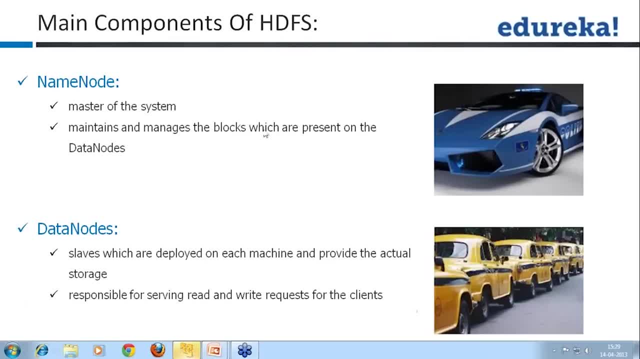 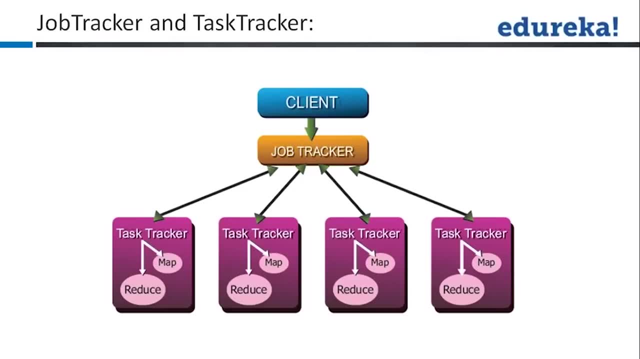 Does that answer your question? Can I move ahead? Okay, great Data node can be redundant. Okay, now let's go a little deep. Mohan, we'll answer these questions as we move ahead. Okay, is that fine? Okay, as we move ahead, we see we've introduced a new term here. 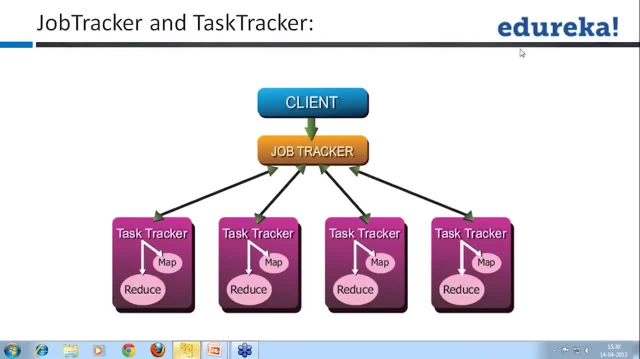 Can everyone look at this diagram for 10 seconds, take a deep breath and think about. think about what Sandeep can think about his wife and I'll think about Katrina Kaif. Okay, and look at this and client job tracker, task tracker map- reduce. 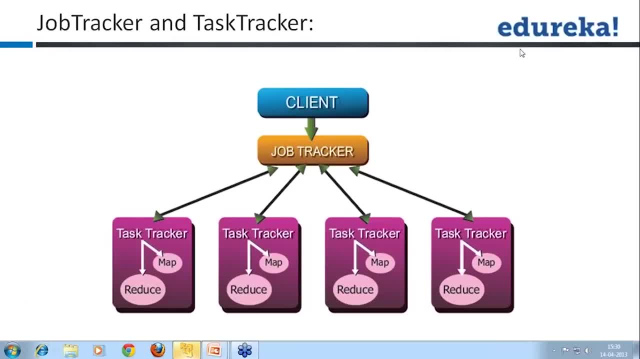 What is the new term here? A client right, Anything else which you see as a new term on this slide. Do you understand everything else other than the client? Everything else we've covered, Okay, map reduce: yes, We've talked about map reduce earlier as well. 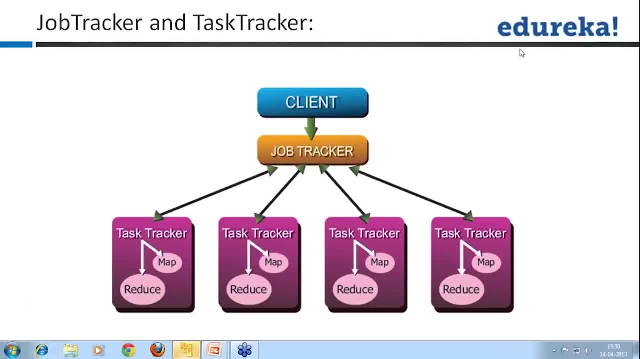 We've said, map reduce is a programming model to retrieve and analyze data. Only this much has to be understood today. Okay, it's a simple programming model. Okay, is that fine? So, other than the client, everything else is clear to everyone. 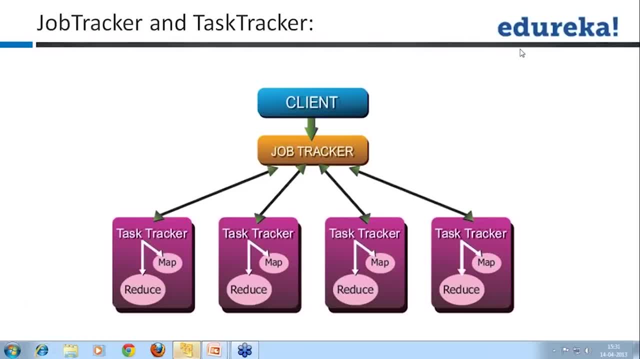 Okay, cool, So client is actually client is an application which you will use to. I'm giving the answer: A client is an application which you use to interact with both the name node and the data node. Okay, which means to interact with job tracker and task tracker. 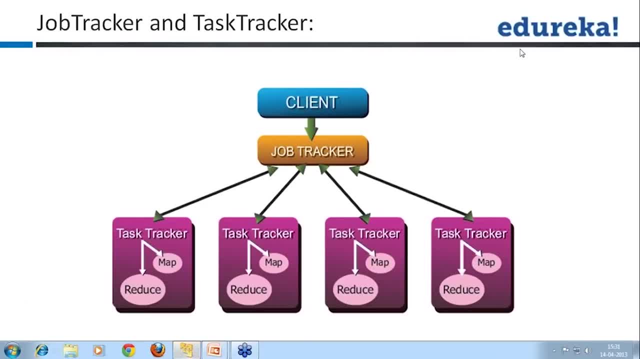 Is that fine? Is that fine? As a very simplistic definition, a client is an application which will be running in your machine, which you will use to interact or give commands or look at the statuses from a job tracker or task tracker. Is that correct? 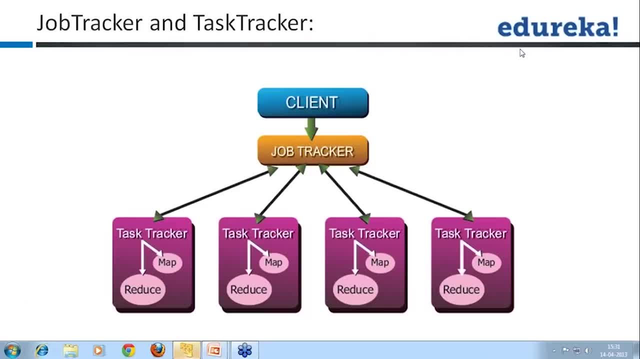 Is that okay? So interaction between the user and the name node and data node is done through a client. Okay, and it is called the HDFS client. Is that fine? everyone. Can you quickly give me a smiley on this, Or else I'll move ahead. 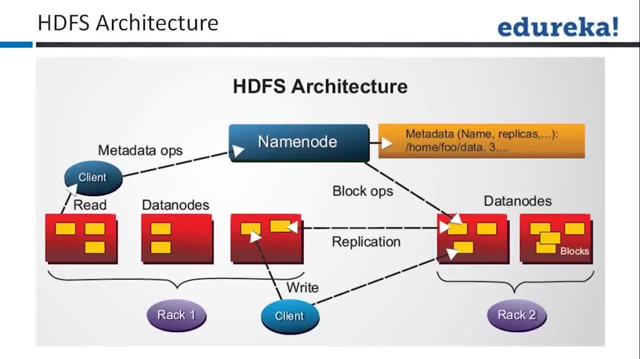 Okay, Cool, Okay, let's, let's get. Okay, Sandeep is asking a question which will answer Sandeep, you'll get an answer, Don't worry. Okay, Devashish. client is a client is a application or a software? 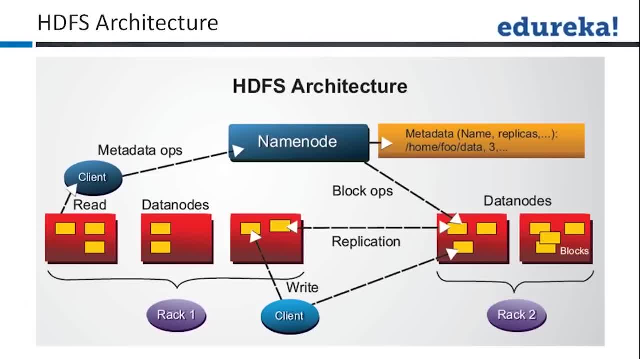 which will run on your machine. Okay, we will see an example. We'll show you how a client looks like by the end of this. Okay, client is an application which runs on your machine. Okay, which you will use to. you will use to interact with data node or a name node. 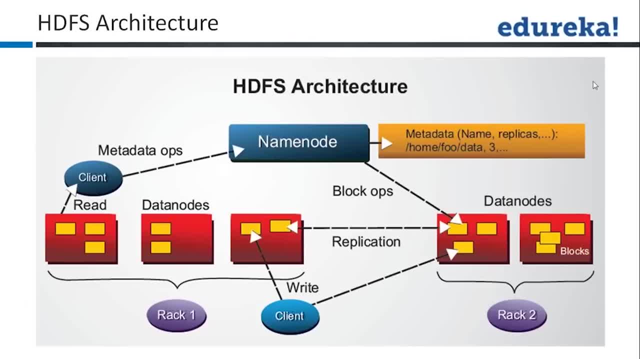 which in turn means the job tracker or task tracker. Okay, we will. all your questions will be answered. Anand and Sandeep, your question will also be answered, Don't worry. Just keep that in your mind, Just keep these questions in your mind. 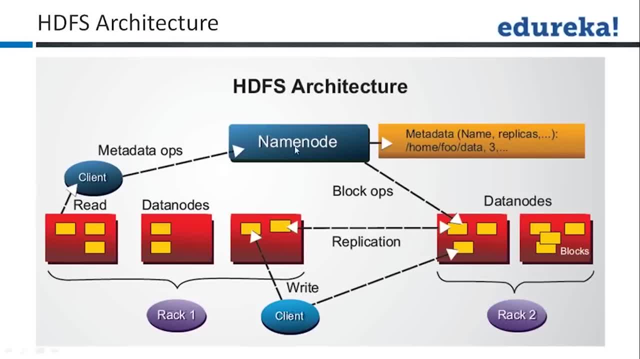 All these questions will be answered. Okay, so let me, let me, let me just, Rohit, I'll answer your question as well. Just give me one second. Okay, Now let's look at this diagram, This: this is a little more complex than the earlier diagrams. 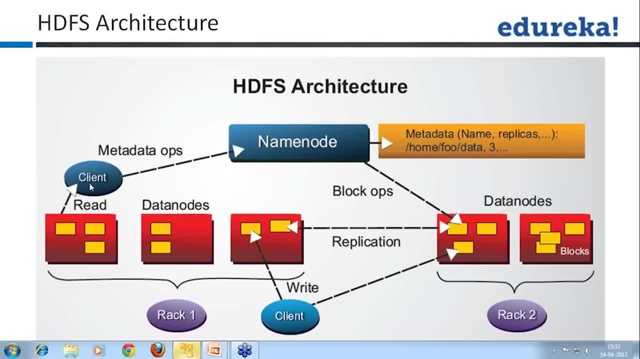 A few more new terms are also introduced in this. Okay, and- and I'm going to explain this, Don't worry You will. by the end of, by the end of this slide, you'll understand each and every term. We're okay. 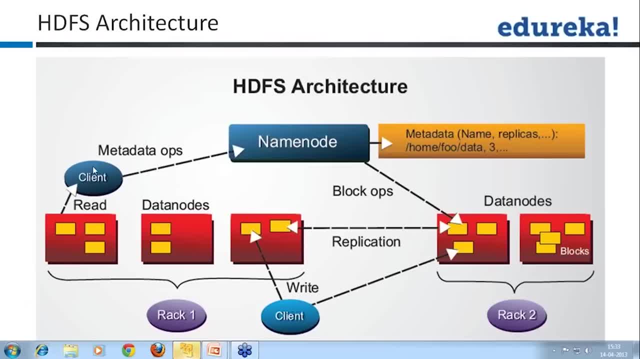 So we have a name node here which is clear to everyone. We have a client also, which we've understood. We've understood that as well, And now there is something called a rack. Can anyone explain me what a rack is? A lot of people will be knowing that it does any. is there anyone who doesn't know what a rack is? 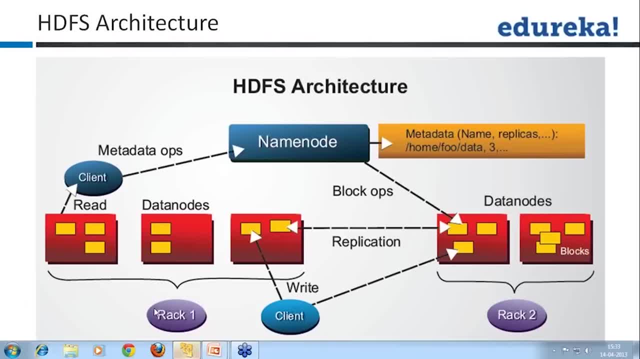 Okay. Sandeep tells me it holds hard disks right. Gaurav asked me to tell you. okay. Ajay is asking me what a rack is. Okay, can anyone give me a? okay? Anand is telling me rack is a storage area, which is right. 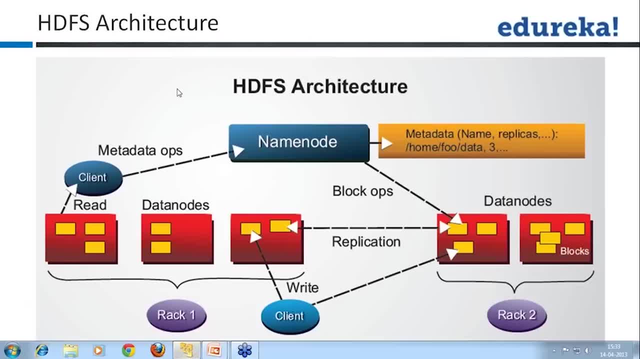 Can any anyone else add to that? Deva, she tells me the storage mechanism. Can anyone else add to that? Okay, okay, okay, There are more people, Okay, So, yes, we have some answers here. Sameer Mahapatra tells us that it is a group of nodes. 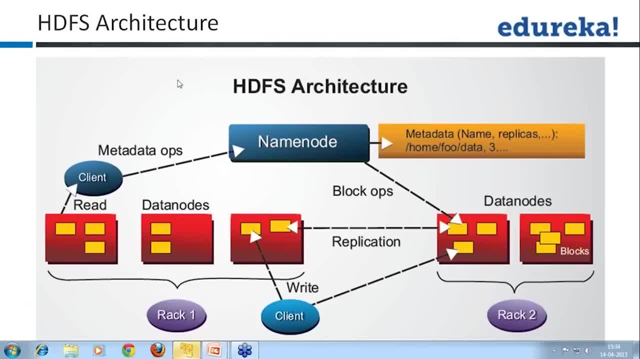 Yes, it is, That's right. Data stores and clusters in a cluster- right? Yes, Gaurav, collection of data nodes in a cluster is so. a rack is a. I believe Syed will be the best person to answer this question. 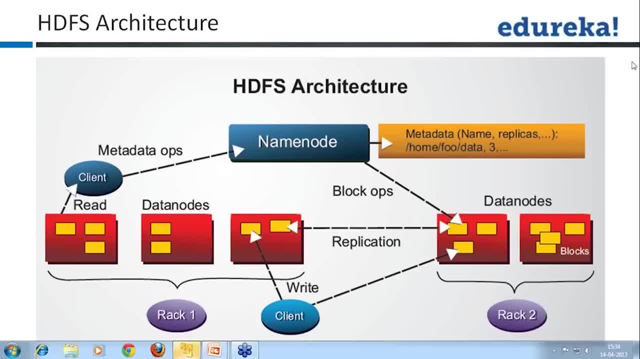 Syed, can you answer this question quickly? Can you give me an answer and tell me if you're with me? Looks sorry, Okay. So basically, rack is a is a storage area where you will have multiple data nodes put together. 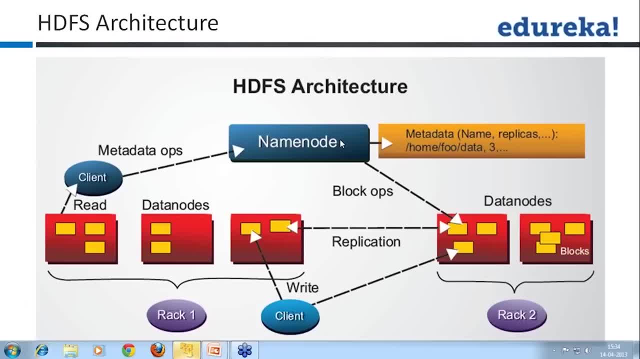 Physically. we said that all these data nodes can be physically at different places, right? You remember the first diagram, when we showed you four different machines at different physical locations, Do you remember that? And then we created a DFS out of it. 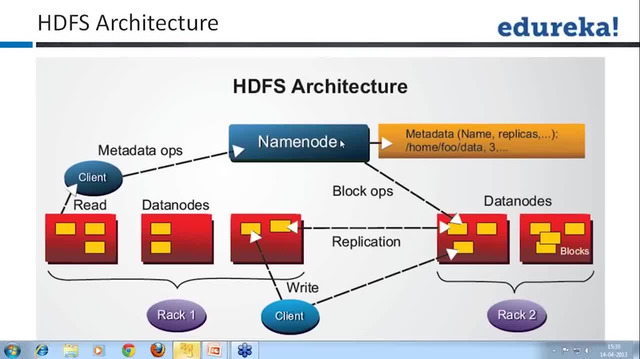 So basically, a rack is a physical collection of data nodes, Okay, which are stored at a single location, Okay, So basically, there can be data nodes stored in Bangalore, There can be data nodes stored in Kolkata, There can be data nodes stored in Australia. 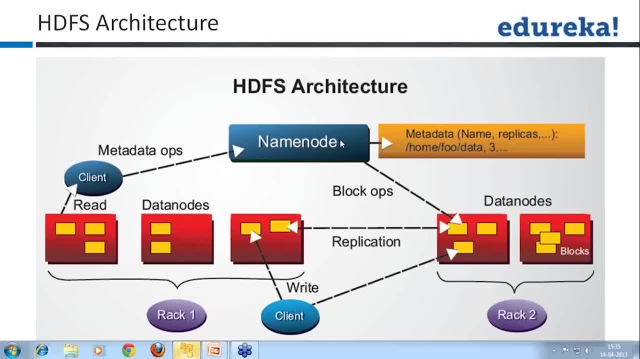 Together we can have a set of data nodes can be stored in a physical location in a rack. There can be multiple racks also in a single location, So it doesn't mean that all the if it is stored in a single physical location, it will be stored in a single area. 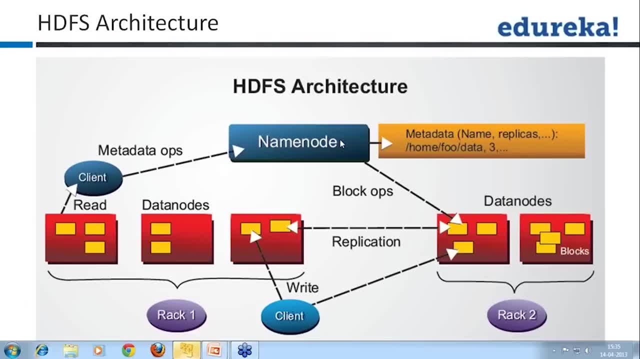 Is that clear to everyone now? Rack is just like a rack. You have a rack of shoes right Where you store All your shoes. Similarly, we have a rack of storage devices. Is that clear to everyone? Can I get quickly get a smiley here from everyone who said no then? 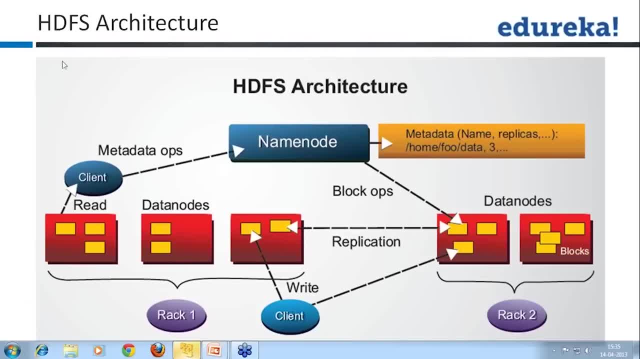 Okay, cool, Everyone has understood that. Great, Then. so we, what we, what we're showing here- is Ajay, Thank you very much. So what we're showing here is that we have a name node, We have a client which interacts with the name node and Rohit. I'll quickly answer your question here. 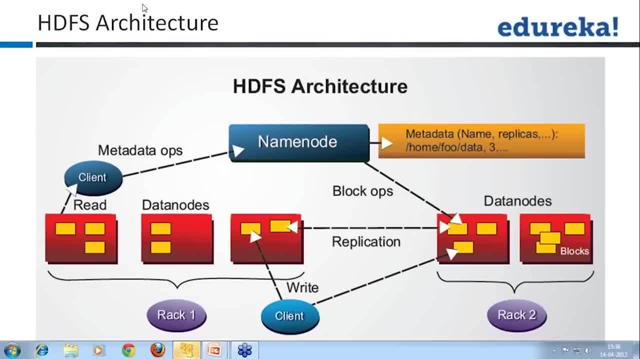 Rohit had asked me what is the mode of communication. Is it HTTP, HTTP? No, Rohit is SSH. Okay, I will answer Rohit. Is that clear now? So Rohit had asked me a question that: how does client interact with name node or data node? 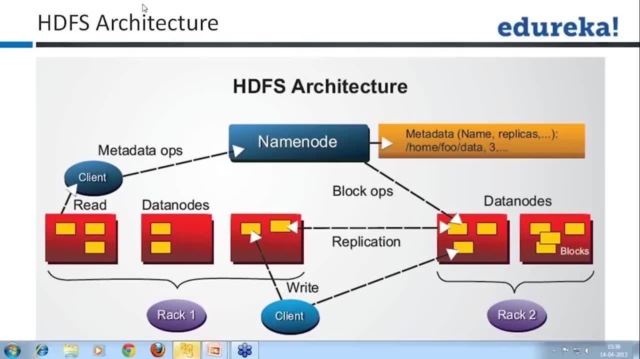 Is it through HTTP? So, Rohit, it is through SSH. Okay, and for everyone else also, this is the answer. Now we also see a term called replication here. Okay, so, as I told you earlier, data is always to maintain the fault tolerance on a Hadoop system. 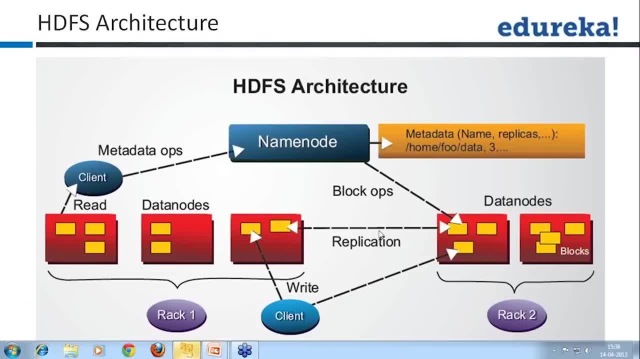 Okay to maintain fault tolerance on a Hadoop system. We replicate data. We maintain multiple copies of the same data on multiple data nodes. We'll understand how it is done in very clearly. We'll understand minimum. minimum number of replicas should be three. 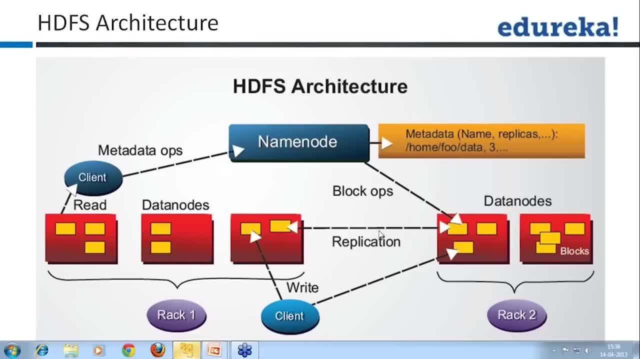 That is the minimum number of replicas required by HDFS. Okay, and it can be defined by the user. Okay, so so, basically, when you write a data on a HDFS, you replicate it and it collects three data nodes. Is that clear? 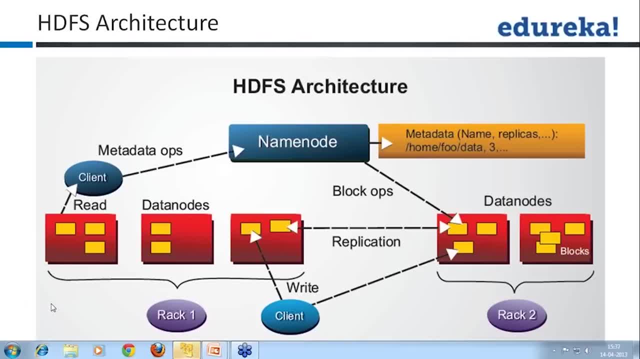 Okay, is that clear to everyone? Okay, great, Then. then there is something called block ops. Okay, so, basically, the operations are to perform in terms of blocks. Okay, Now the block size. in a block size. Rahul, you have to Hadoop. 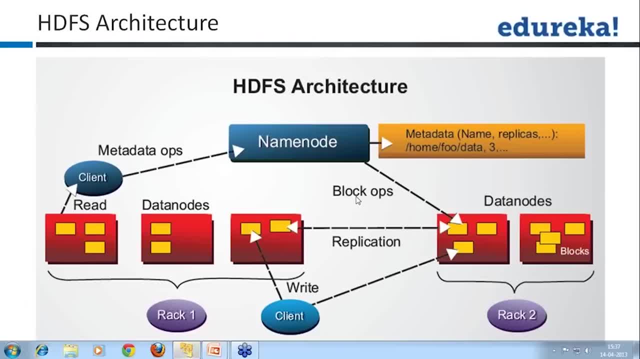 Advises You to. at least Raul is asking: is it compulsory? if I didn't, that, if I didn't want see, as I told you, right views commodity hardware here and we still tell, don't want to lose data and there is a good chance that the some of these machines will keep on failing. 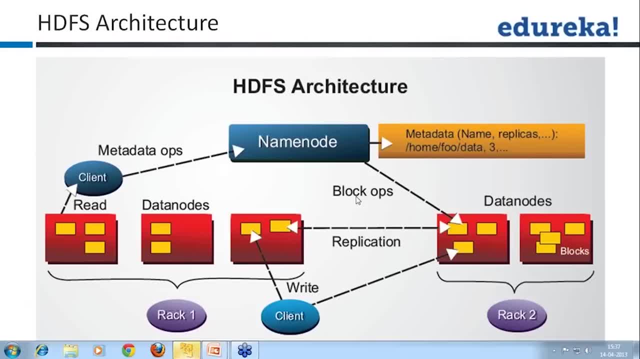 So we keep, we need to keep data in multiple places. Okay, the redundancy has to be maintained, application has to be done. Okay, Okay, is that fine, Raul? Okay, now, Okay, Now, the other thing which I was telling you was that the block size. 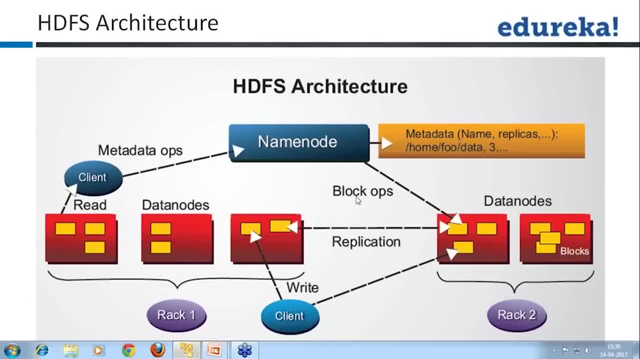 Let's block size in HDFS is. can you someone? can someone tell me other than more on what is the block size in Unix? Can someone tell me that? What one quantum of block, how big is that? No one knows about it. No one has answered that question. 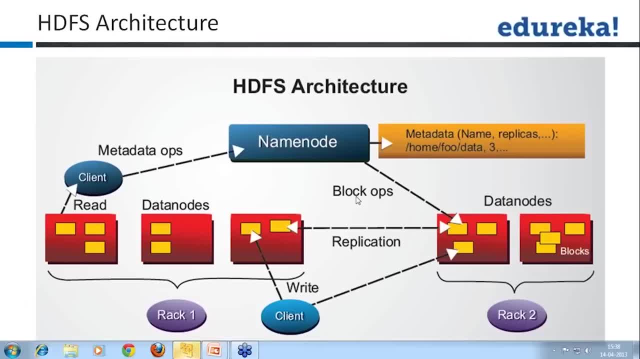 I'll let Mohan answer that one. Can you please tell me what is the block size in Unix or a Linux machine? Guys, you can do Google as well. I'm not your teacher. I'll not stop you from doing Google. Please. Google things which you do not understand in the class, which you, which you want to ask actually. 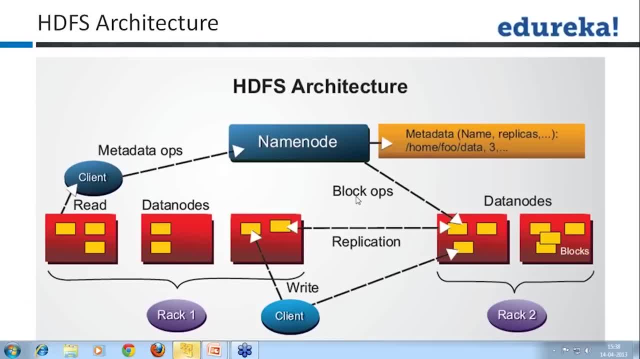 Okay, Okay, no problem, And can, can you guys, Google, don't think that I am the only source of information. You can also be the source of information. Google is the biggest source of information. I have also learned everything from Google. Can someone give me that answer quickly? 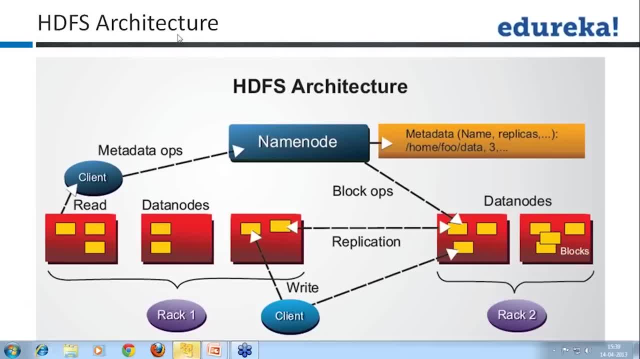 Rahul Tiwari. where are you, man, And where is our friend Devashish? I have not heard from a couple of guys for a long time. I want them to answer now. I haven't. I haven't heard from Dinesh. 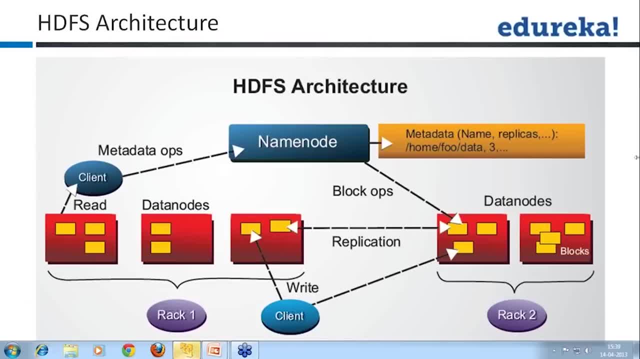 I'm asking the default size, So I just giving me an answer: 8192 bytes. Pawan Pawan, You've not. you've not answered anything, friend, Can you, can you get quickly Google this and give me an answer? You can keep this answer for yourself. 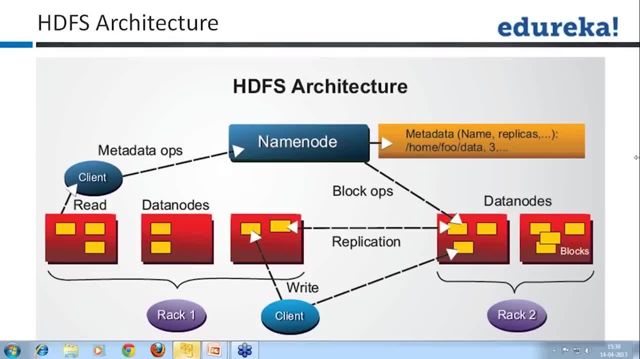 I'll tell you: Okay, So we've got a lot of people giving me the right answer. Okay, So now the block size in HDFS is 64 MB. Okay, It's 64 MB, And the Block size in Linux is 8192 bytes. 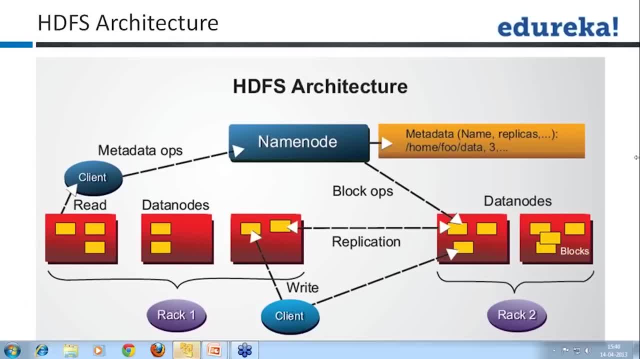 Okay, So basically HDFS is built over Unix and HDFS, as I told you earlier, also is used to store huge amount of data, The single block of operation, and I'm asking about the default size. It can be configured to a bigger size. 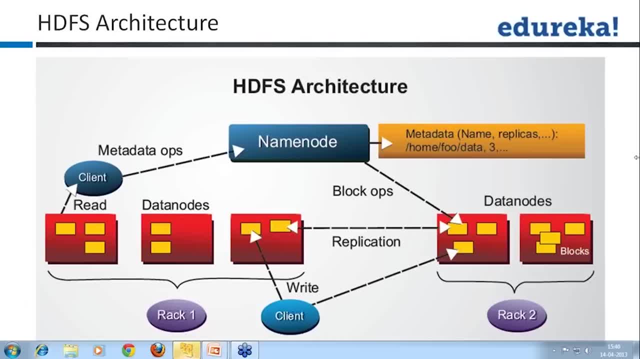 The minimum is 64 MB. Okay, is that? is that? does that make sense? and this also: this clearly tells me: if you have smaller file sizes, there will be a lot of metadata which you'll have to store, and it will. it will not be a very useful. 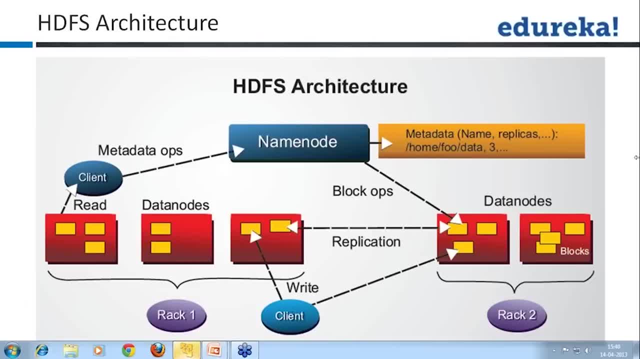 System to use. is that? is that clear to everyone? usually it will be much more than 64 MB. We'll be configuring it in a few GBs or maybe sometime TBs- Is that fine Does? does this answer that question, which everyone had that? why do we want to have? why can't we store many small files in HDFS? 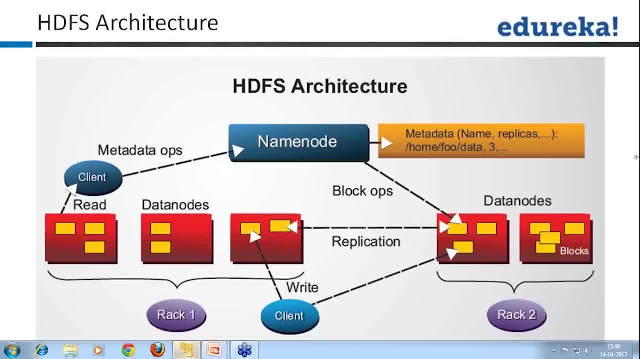 Is that okay, guys? Okay good. So everyone has understood that. I've got few yeses. I did not get a response on power and power. Can you quickly answer this if you have understood this? Thank you for one. Thank you very much. 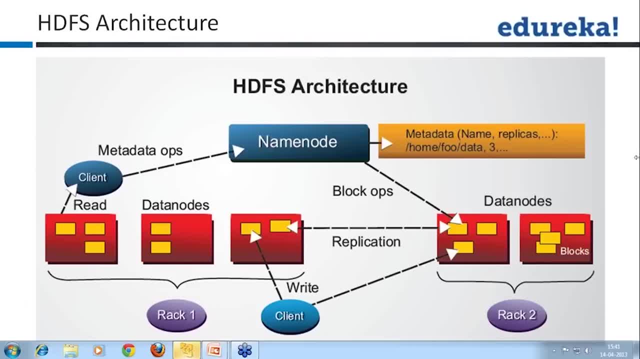 I might think you were out for lunch for some time, Is that correct? or you were here, You were attending everything. guys, I'll be asking questions in the end and everyone will have to score 100 on 100.. Okay, 10 on 10.. 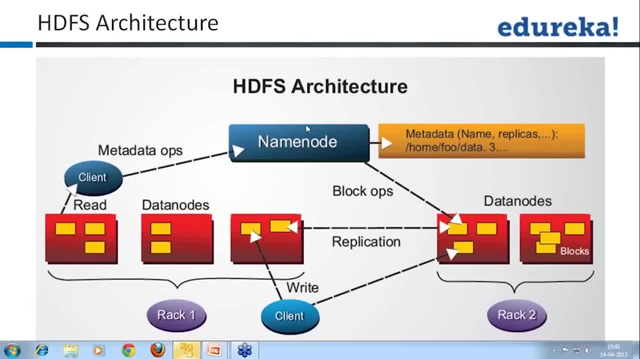 So please pay attention now. Okay, so we've understood most of these things here. Now I'll just explain this diagram once again. So we have a client which interacts with the name node. It also interacts with the data nodes. Okay it, the client, does a read and write. 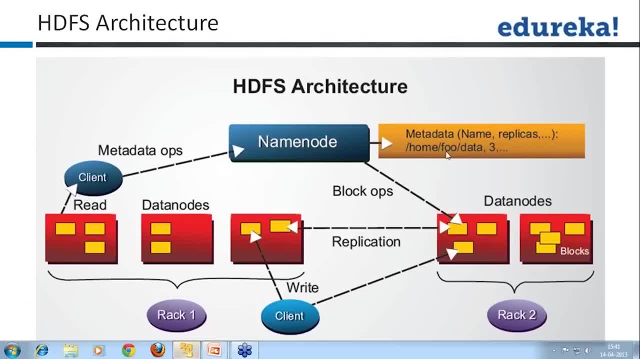 There's something called Metadata here, So name. can anyone tell me what is the metadata quickly? Can someone tell me a metadata? What is the metadata? Okay, so a lot of people have tell. told me the right answer. It is a configuration data data about data, data into data. 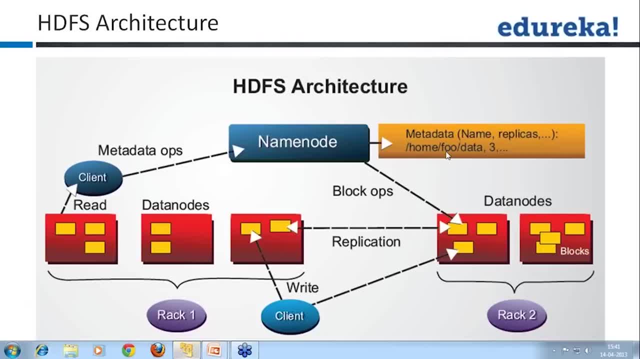 Yes, that's true. So metadata is not the actual data, the actual logs which will be storing, but the data about data, which means: where are these? if I am, if I'm storing a block name, what will have this information that? where is this block get? where is this data getting? 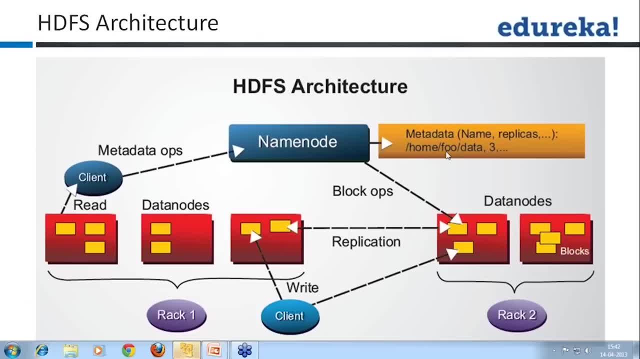 Stored. Okay, that information. which are the? which are the name nodes? Where is the? where the? where are the racks there? Where, which rack, on which rack? which data node is there? all this information, all this information block map is Mohan, is what? 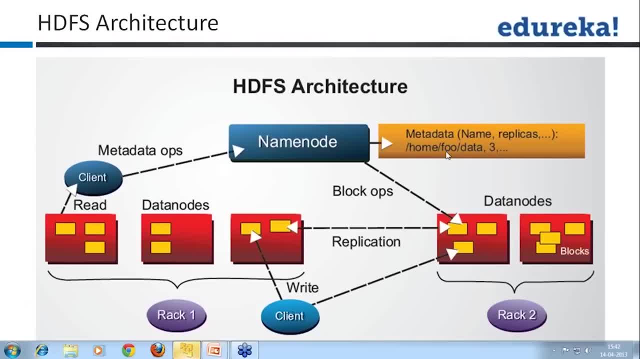 Yes, exactly So. a block map is what Mohan has told me. This is exactly correct. So all this is metadata and all this data is stored in the name node- name node. This data is stored in the RAM, Please, please, remember this. 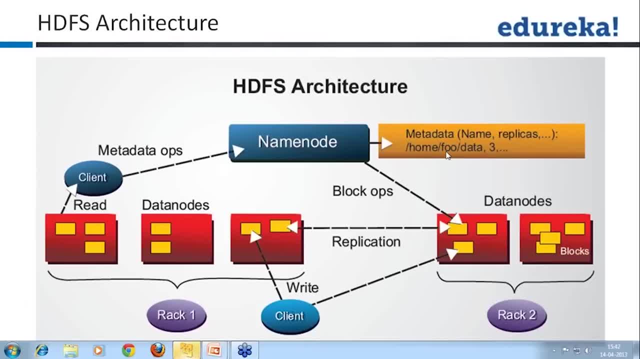 It's stored in the RAM. I tell you more about it, But for now let's understand. It's stored in the RAM to have fast access, Okay. and actual data is stored in the data nodes, Okay. So is that clear to everyone? 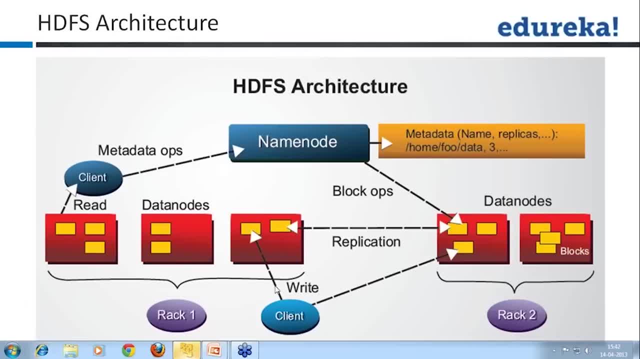 We will go into more details of these operations- read and write- as we move ahead, But for now, kick. does everyone understand what a name node is? What are? what metadata is? What replication is? Why do we need replication? What data nodes is? what a client is? 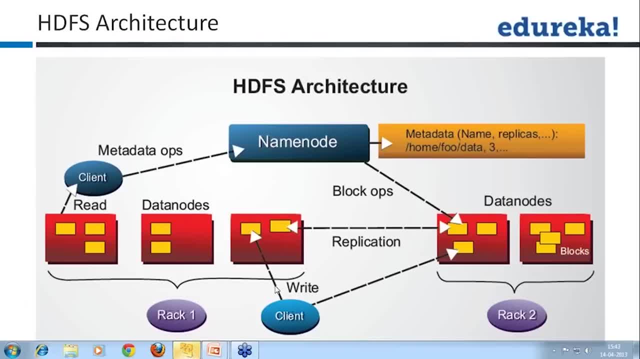 What a rack is all these? if? if the answer to all these questions is yes, please quickly give me a smiley. If you don't understand anything, please put that Name there. I'll explain it again. Looks like everyone has understood. 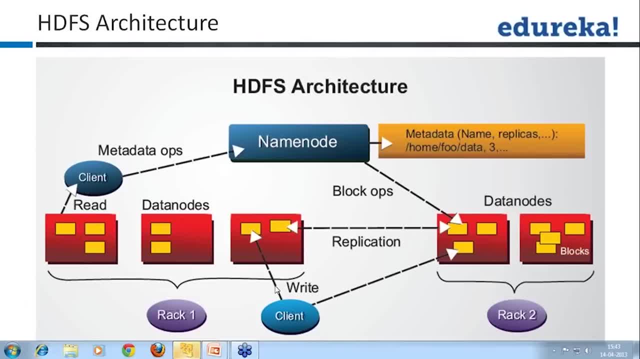 I'm doing a great job. Okay, Sameer is asking me: What about block operations? Sameer, I'll answer that: go going forward. Okay, Don't worry. So each time name node, create metadata. when we are on cluster Sunday. 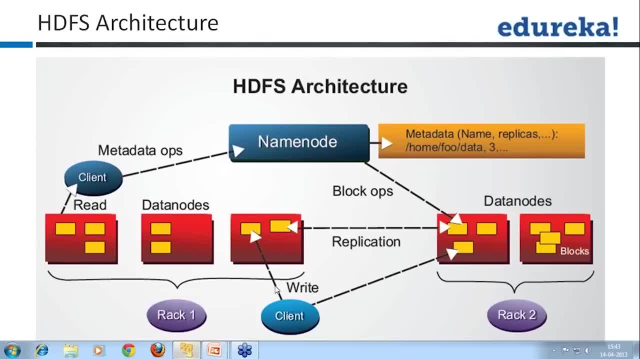 Can you re, re, re rephrase your question? So name node is a high availability machine. a Lamborghini which will Be stored anywhere with it should have good protection. Yes, it will be Okay. So suddenly better question It. just all this metadata is stored in a RAM. 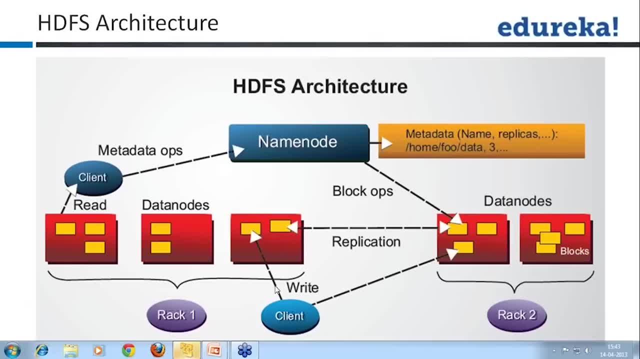 There's something called a secondary name node- and I am introducing a new termers here, So please pay attention. There's something called a secondary name node which is used to which, which periodically reads the data from the RAM of the name node and persists that data into a hard disk. 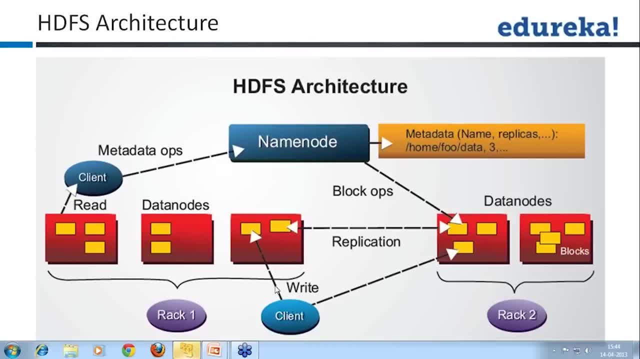 So name node does not write it into a hard disk. name node keeps the data in the RAM. It does not spend time or operations or cycles and writing into the hard disk. There's something called a secondary name node which keeps on reading from the name node. 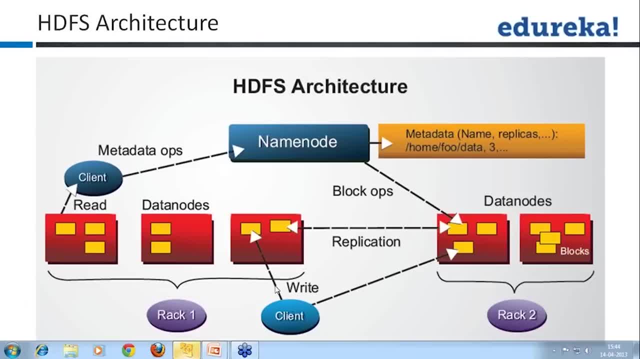 Okay, data from the RAM of the name node and writes into the hard disk. Okay, is that? is that clear to everyone? But secondary name node is not a substitute of a of a name node. Okay, So if the name node Fails, the system goes down, and that is the case in Gen 1 Hadoop. 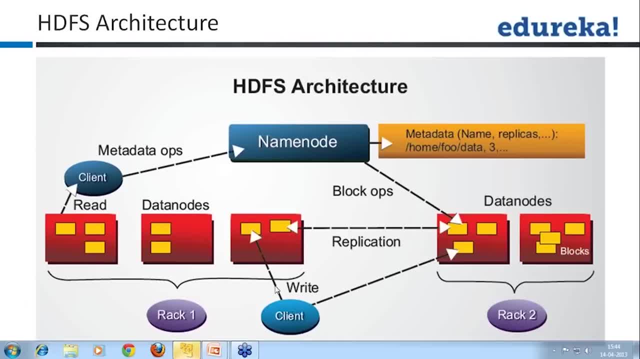 I'll tell, tell you what happens in in the Gen 2 Hadoop, But for now let's try to understand that name node. a single point of failure. There's no, there's no, there's no backup name node, which though it is called a secondary name node. 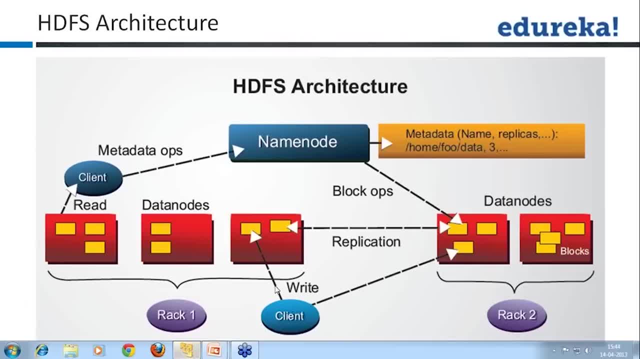 It does not become an active name node. If the name node goes down, it just reads the data from the method, from metadata, from the RAM of the name node periodically and keeps on writing into a file system. Is that clear to everyone? It does not come into picture. 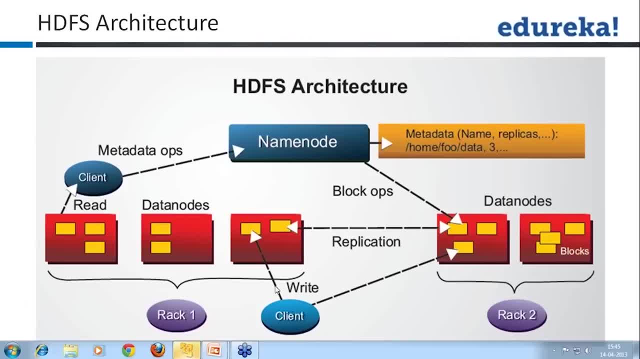 If it keeps a macro metal backup of metadata, Okay, so it does not. it does not if I. if the name node fails, it does not become the name node, Is that fine? So in Gen 1 Hadoop, when we talk about Gen 1 Hadoop, there is just a single point of failure, which is name node. 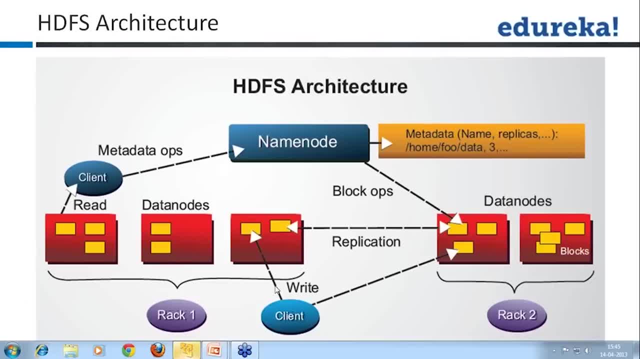 If the name node fails, the system crashes. Okay, and to get the system back You'll have to put another name node and read the data back from the secondary name node, and you cannot retrieve the data from the The time the last backup was taken. 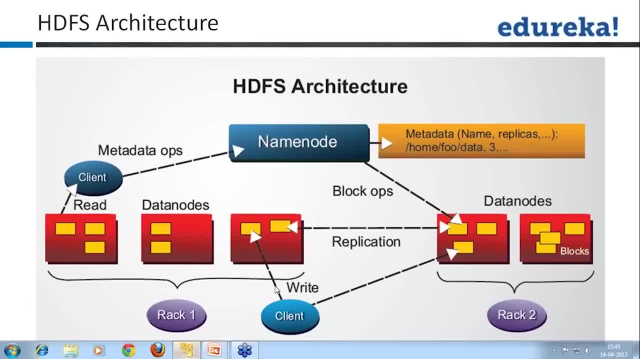 Is that fine to everyone? That is why we need a Lamborghini for a name node. Does that make sense to everyone? Is there anything which is not clear here, guys? Okay, good, So everyone has understood why we needed a Lamborghini there, because we do not have any backup to it. 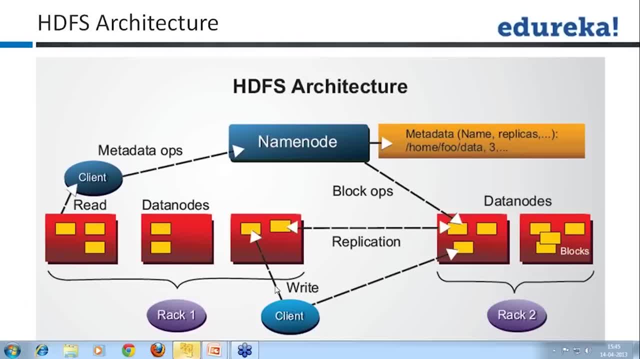 Sandeep, just give me some time, I'll explain everything. I'll explain everything. Okay, just give me some time. All these things are going to be covered in the next slides, Okay, Yeah. so basically, The important thing to understand here is that. 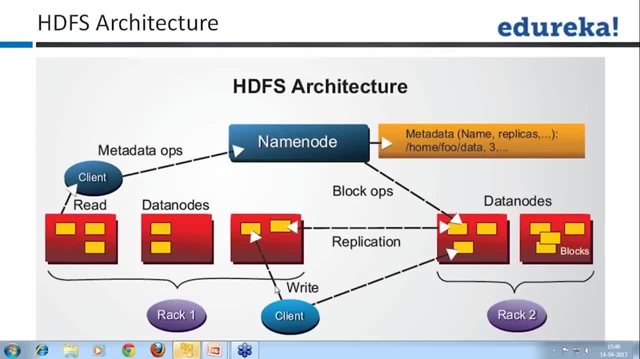 The important thing to understand here is that the name node stores all the data in its RAM. There is a secondary name node which keeps on reading this data from the RAM and keeps on writing into a file system. That can. it is not a data node. 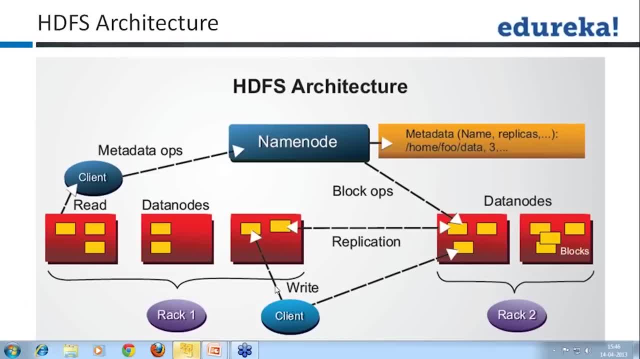 It's a separate file system where it keeps on writing, Raoul, Okay, so to make sure that we are storing what was happening in the in the RAM and it keeps on syncing that data time and again with the. what is there? Okay, so to make sure that we are storing what was happening in the in the RAM and it keeps on syncing that data time and again with the. what is there? 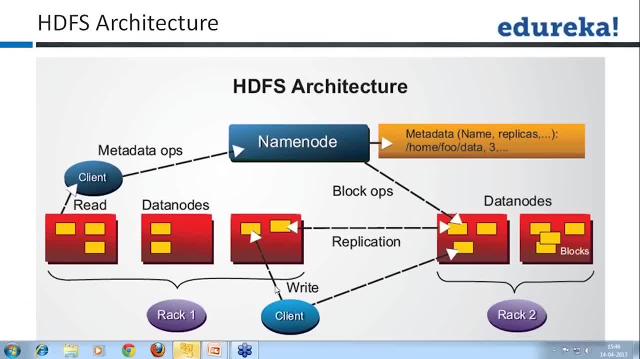 Of the name node. Is that clear to everyone, guys? Very important concept. And if you guys are preparing for an interview, someone can ask you what happens if the name node crashes. Does the secondary name node take over? The answer to that is what. 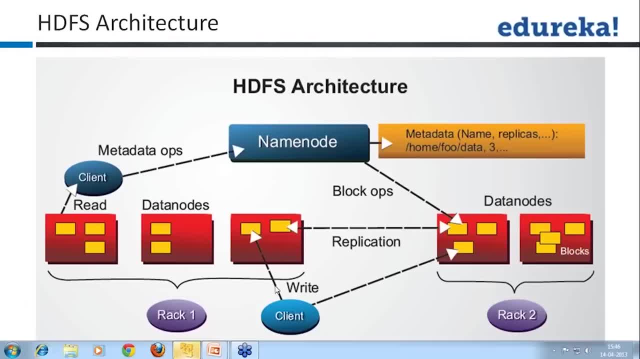 Yes or no? Very good, Everyone will crack that interview for Hadoop with this. I tell me, definitely not, Rahul You, you will move from Terra Delta to Hadoop man, Okay, so that's a very important thing now. Okay, Now the second thing. second thing which is very important is- and I'll take a liberty to introduce that as well- 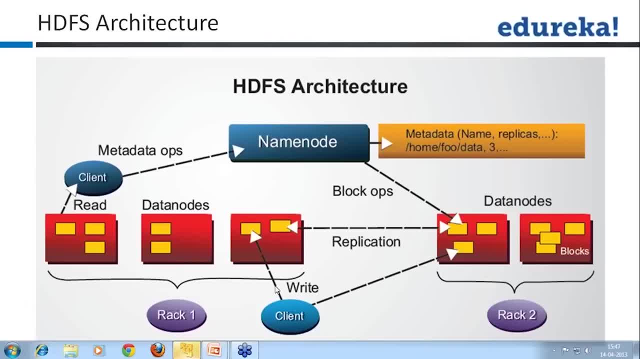 I talked about Gen 1 Hadoop, So now this: there was this problem with Gen 1 Hadoop that you, we had just in a single point of failure, and there the secondary name node was a misnomer. It's, it's actually a misnomer. 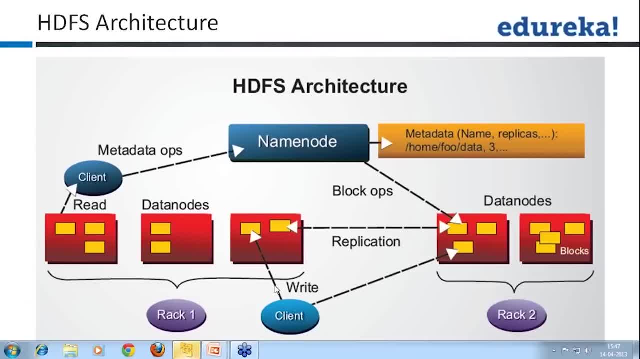 It looks like that the secondary name node, and it's actually used to fool people in interviews. Okay, so it's a misnomer in Gen 2 Hadoop Now the say: someone can ask you this question as well. Now, what is the difference between Gen 1 and Gen 2 Hadoop in terms of name node? 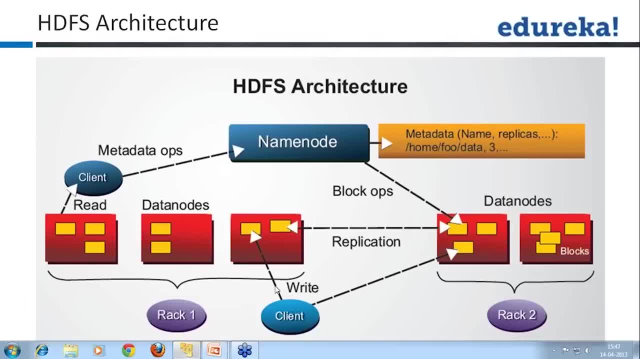 So in in Gen 2 Hadoop, we have an active, passive kind of name node structure where there are two name nodes. What is the active one? There is a second one which is passive one. very important to understand, Pawan, Are you. are you getting this point, sir? 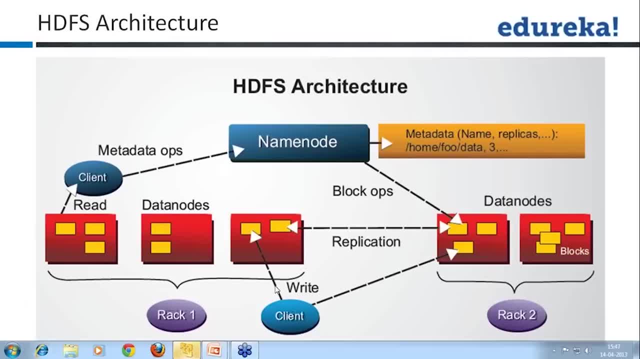 Anyone preparing for interviews. I was told that Pawan is preparing for some interview, So it's very important to understand this. So in a Gen 2 Hadoop we have: okay, great, Great, Great Sure, More with okay. 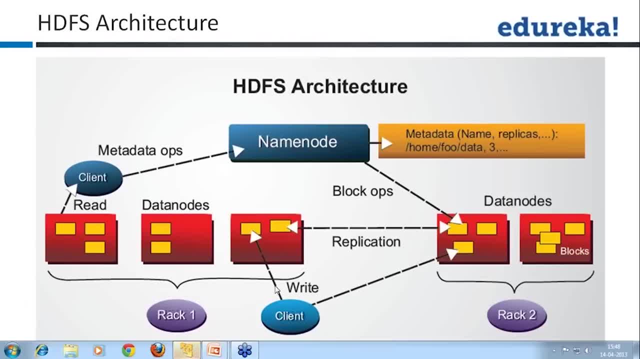 So in Gen 2 Hadoop we have an active passive. We have active passive kind of a structure where there is an active name node and a passive name node. So in that case if the active name node goes for a toss, the passive name node can take care. 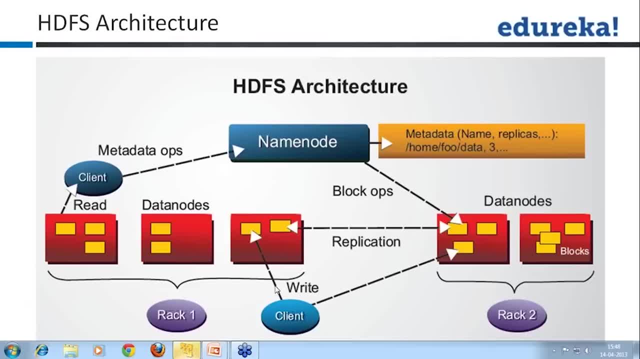 So that is the difference between Gen 1 and Gen 2, Hadoop. Is that clear to everyone? guys, I'll ask these questions in the next class as well, So you have to remember this. Okay, good, Yeah, it's a standby kind of thing. 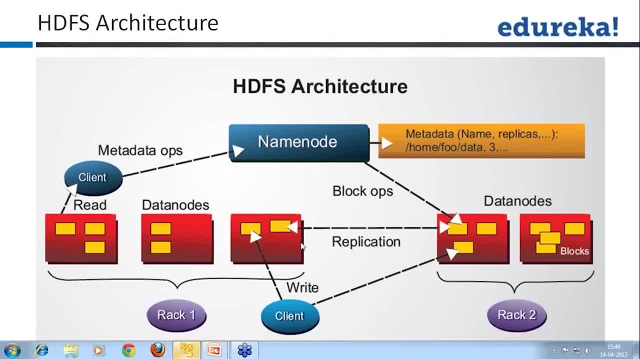 Right, Yeah, right, Okay, Just says okay. Can everyone give me a smiley If you like this idea, if you really like this, good, So there will be a secondary name node which will keep on doing a backup, backup data. 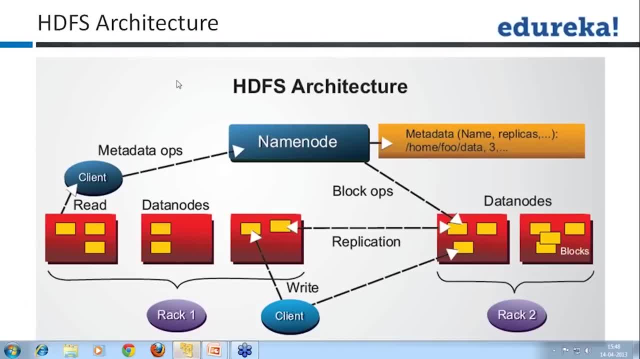 Okay, but actively active name nodes will just store data on the RAM. Okay, some deep name nodes will not waste their cycles. Yes, name nodes will not waste their cycles and writing data to the file system. Okay, name node Are high availability machines. 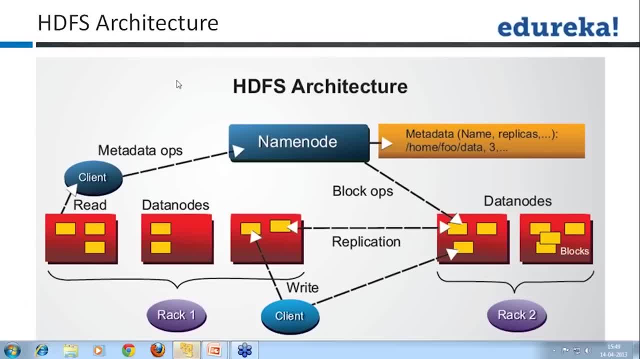 They're very fast, Very, very expensive. We will not use a Lamborghini to drop you to the mall- Okay, To is that, is that fine? or to take pick you from the railway station- Okay, let the secondary name node do that. 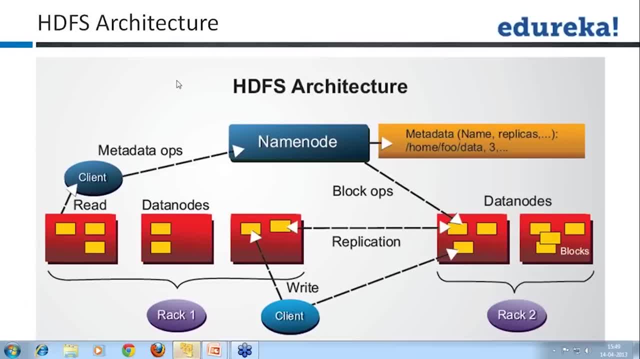 Is that fine? Raul will talk about it later on here, Don't worry. Okay, Yes, there is a secondary name node in Gen 2, Hadoop as well. It will be there because it we have to keep store this, all this data, persistently. 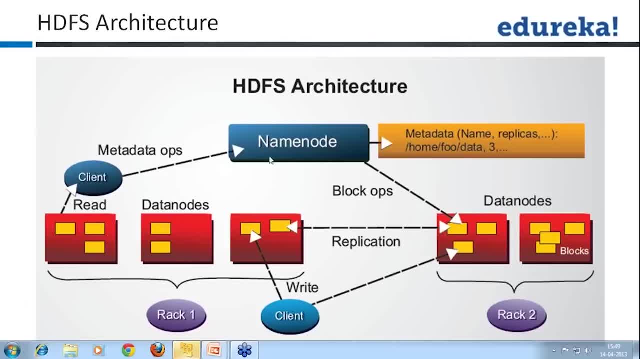 Put, you have to process all this data in the hard disk. Okay, So let's move forward, guys. If everything is clear here, Okay. So now, now we have, we have, we'll get into a little more details. Okay So where is MapReduce used? 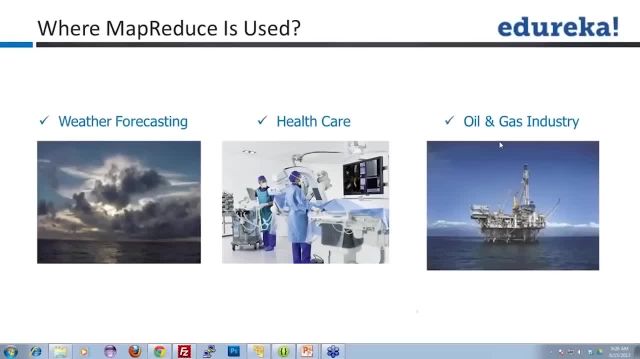 Okay, So now? so we have a lot of data from the weather, weather forecasting. Okay, where we we have a lot of climate data, which is say, from since the beginning of the century. We need to analyze what is the? what will the maximum temperatures? 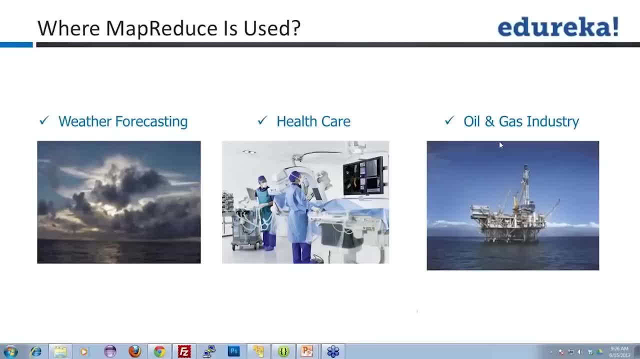 We'll do a lot of predictions based on that. So so that's one place where we'll be using MapReduce. Can you tell me where in healthcare can be? we will be be using Okay patient reports auditing product distribution right. claim processing right. 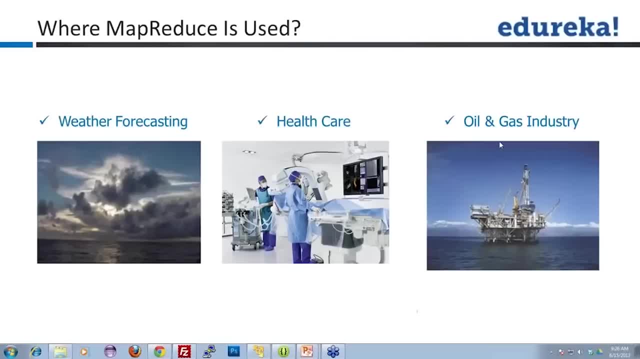 ECG monitoring machine data flowing into the in the tools says warm, See, right, identifying fraudulent claims, Okay, DNA research, Sachi, right, That's true, scaring data. So yeah, so there are a lot of applications, We have a lot. 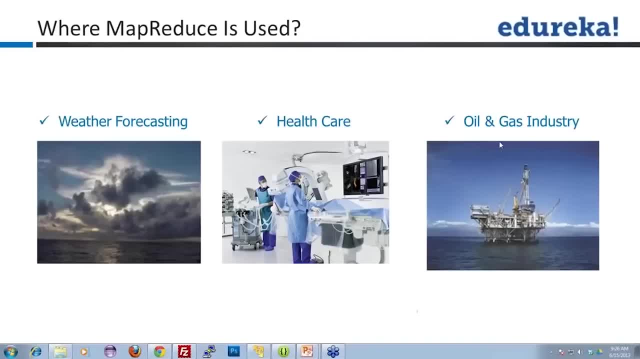 Of unstructured data from all these industries- and these are not the only industries. There'll be a lot of other industries. where, say, utilities side, oil and gas industry- that will will have a lot of data which we need to analyze and we'll see how we used to do that earlier. 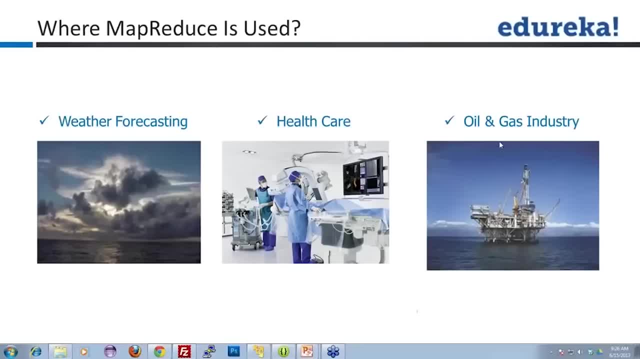 Okay, Now, okay, So we will just see how we used to do earlier and then we'll see what are the challenges there in the earlier methods, and then we'll see how Hadoop and MapReduce solve that problem. Okay, So let's look at one of these examples. 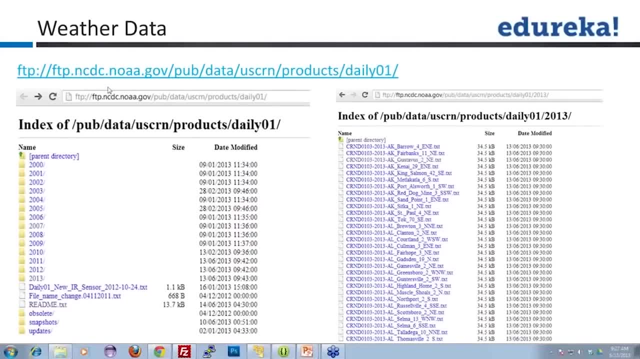 Now what I've done, As I picked some data from this site and CDC. this is climate data, Okay, and so this has for each of the years, right, It has the data here. Okay, let me show you some of this data. 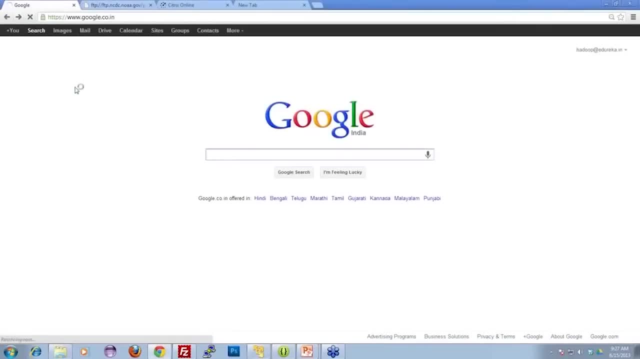 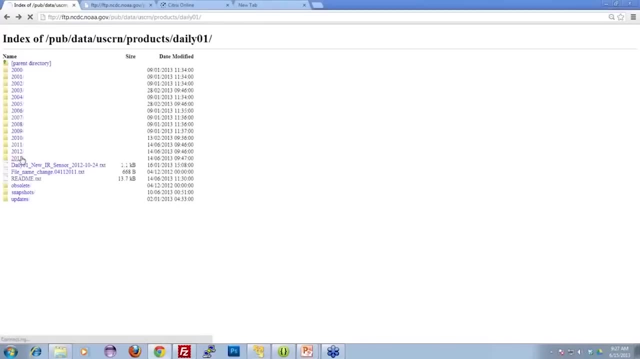 How does data looks like? Okay, so that was on the PPT. Now let's see this data. Let's see, I will there, I got this data and we'll see what do we do with this data. Okay, So let's look at year 2013.. 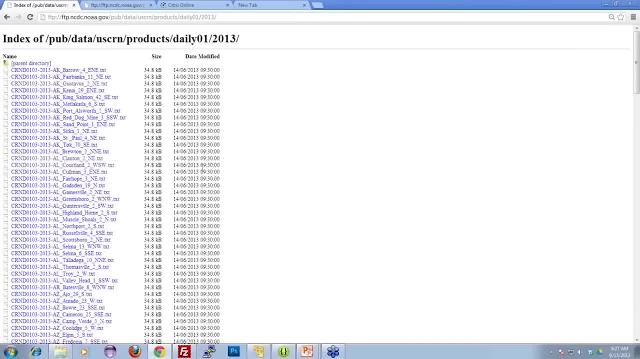 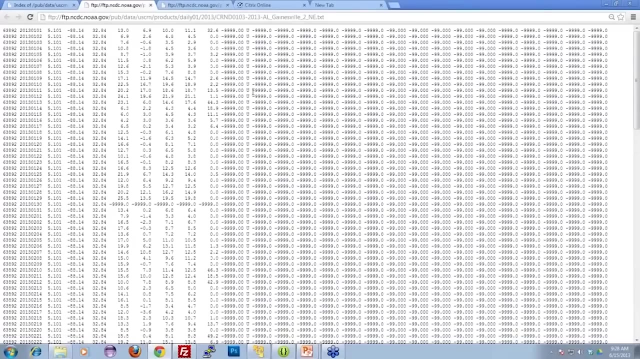 Okay, Raul, are you able to hear me now? I mean, I think there may be something wrong at your end as well, because everyone else says that I'm audible. Okay, So this is one data set, huge data set. So there'll be such data sets, and I've just picked up one from that file. 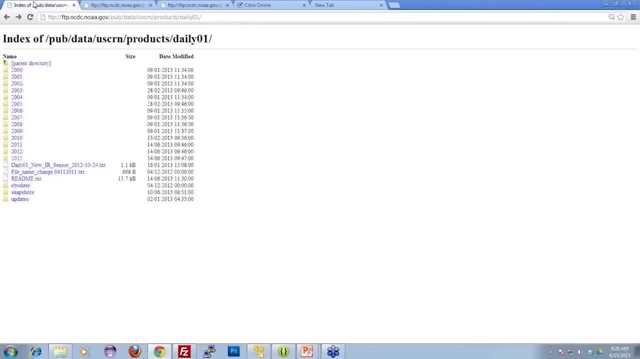 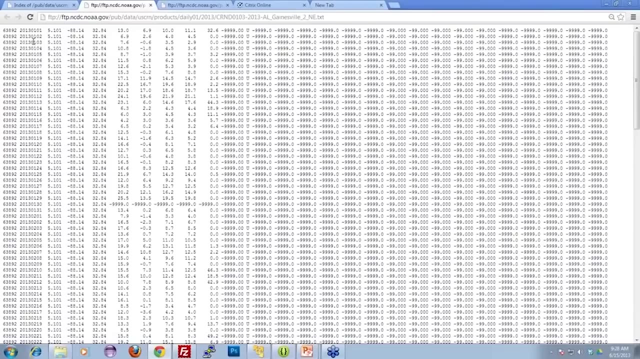 There'll be the terabytes of such data. Now look at this data. It's like a log data. Lot of Lot of columns are there and it is delimited by space and tab. Okay, So you don't have to worry too much about what are all the fields here? 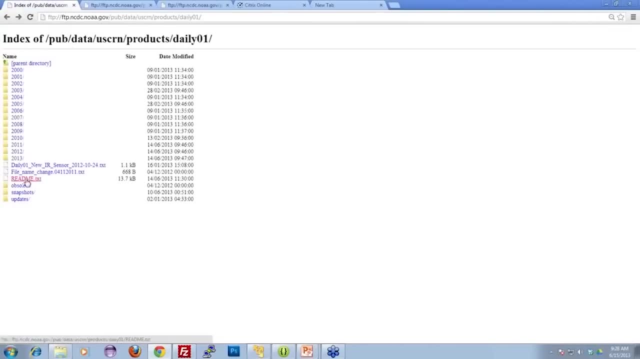 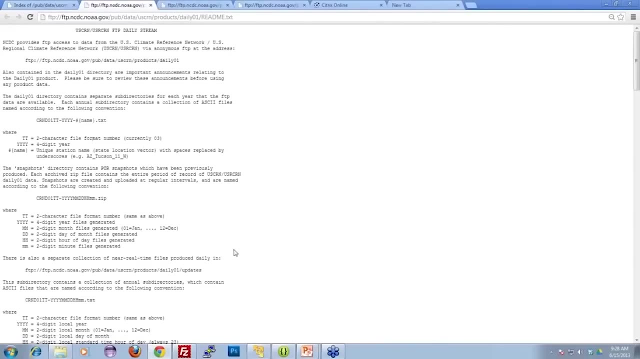 I think the whole idea is to present it to you. Yeah, So if you want to see what are, what is what? all is there? let's see what is there in this data. Okay, Yes, it is, It is. 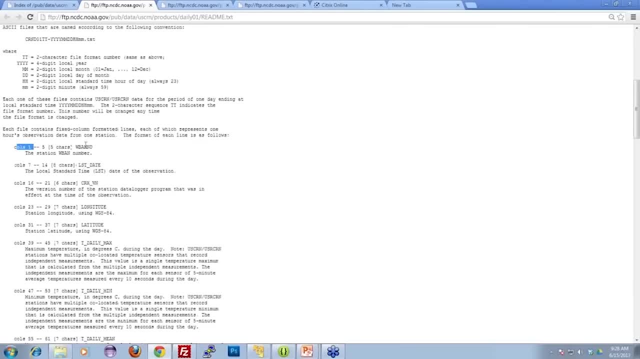 That's right, Ashish, Okay, Okay. So now it says that W band number is something which we do not care too much about. Then there is this local standard time, which is from, say, column 7 to 14.. We have columns: longitude, latitude, daily max temperature, daily mean temperature, daily mean temperature. 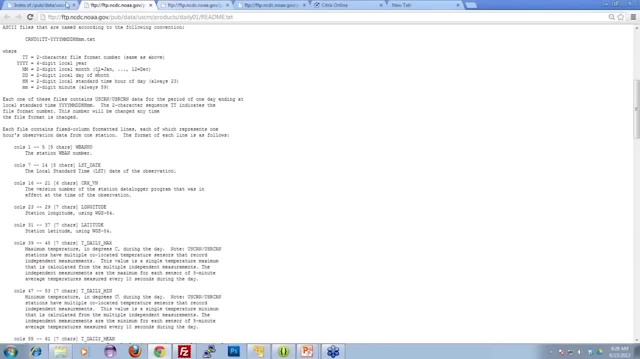 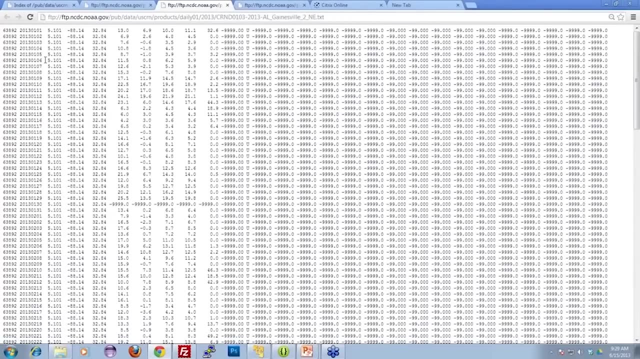 So a lot, of, lot of such data is there here. Okay, Now what we want to do probably with this is that, in this, if I have to say, find what in every year, right, What is the maximum temperature which occurred? 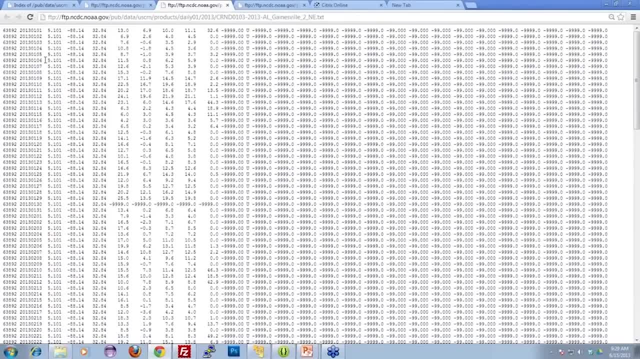 Or how many days were, can be classified as hot days. how many days can be classified as cold days, right? So can anyone tell me? how will you find it if you- if this I mean- forget about Hadoop, right? 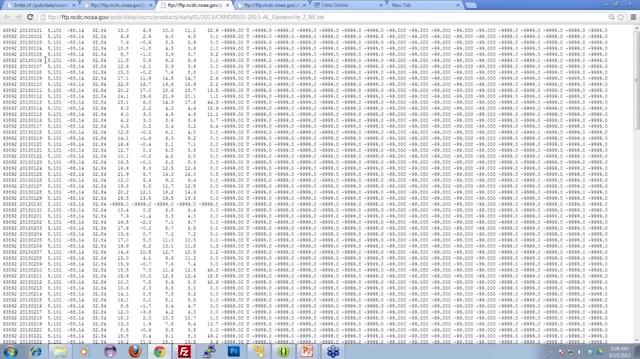 How will you actually find it out? So if I have to tell you that for each year, give me, tell me which is the what will be your traditional way of finding it out, What? how will you do that? Yeah, the columns are fixed, Vamsi, right. 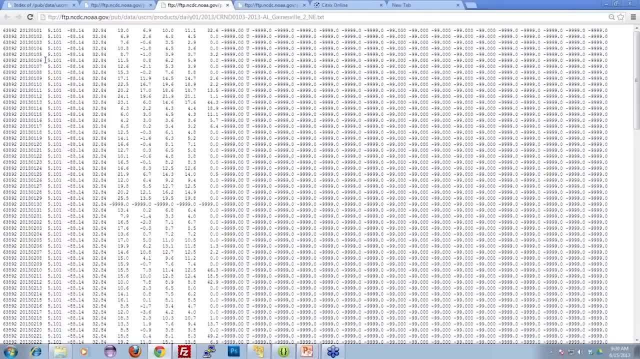 That's true. Okay, so Sachi is telling you will know data in oracle and SQL. it okay, Go through and column row and column value max function right, right, Vinay, okay and evaluate for a range. okay, meh, okay. 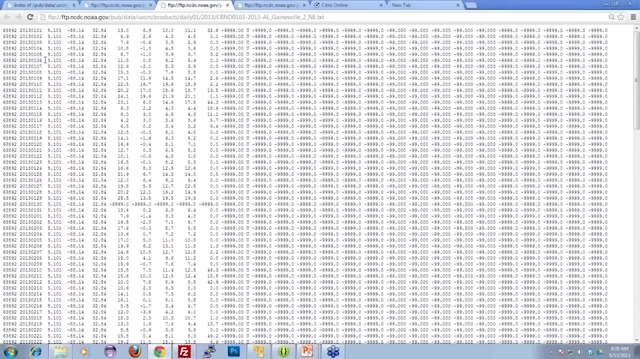 Is anyone from the Unix background here? Yeah, great, So Ravi has. Ravi has given me some some answer there. Very good, So Arka is. Arka has given me a very good answer. okay, Put it in a column. 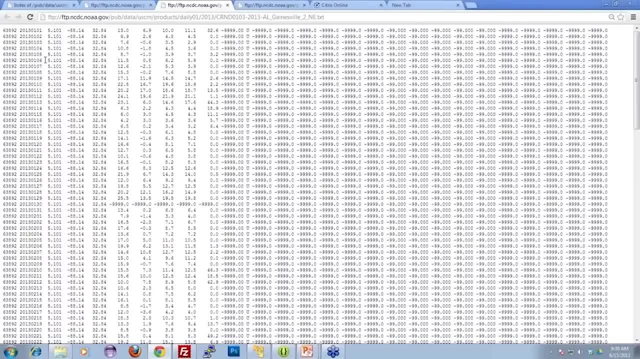 Put it in a file using awk. very nice, So that's what Rajat has also given me the same answer: awk. So how many people know about awk? A-W-K. Everyone knows about awk. Yeah, Avinash, you can write a script in Perl as well. great. 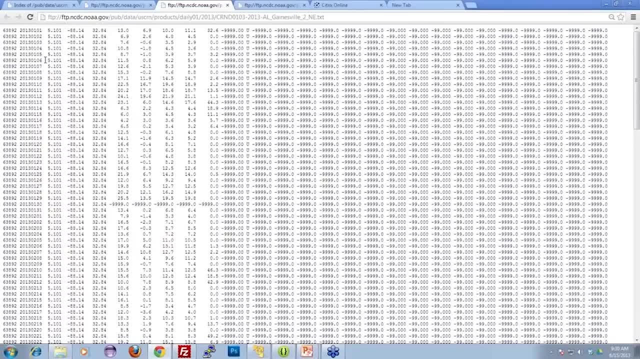 Okay, okay, so don't worry. whoever does not know about awk? Okay, that's not really required in this course, but but what I want you guys to do actually is I'll send you some code in awk as well. 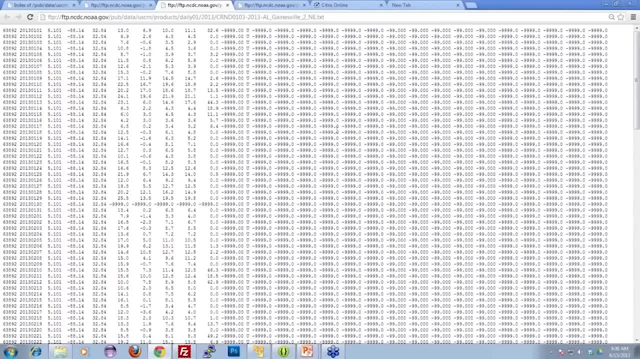 So what we'll probably do, see the whole idea, no problem, even if you are from the mainframe background or any background, doesn't make much difference. okay, so it is very simple. So in Unix, if you have to, if you have to take this file in, what do I have to do? 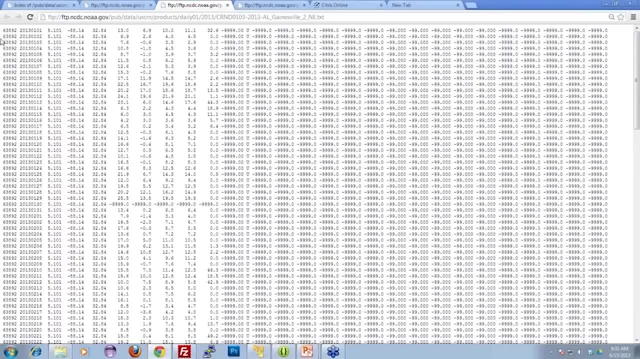 You see, the fundamental thing will be that, for each record, right for each of this record, for each of this record which has one record which has, so this is the maximum, this is the minimum temperature. I have to look at it. 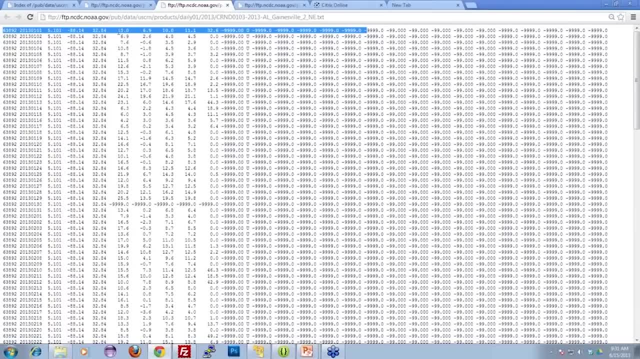 I have to look through this record, okay, and figure out if put this into a max temperature thing and see if, as I go further, whenever a max comes in, you know how to write a program to get this done right. 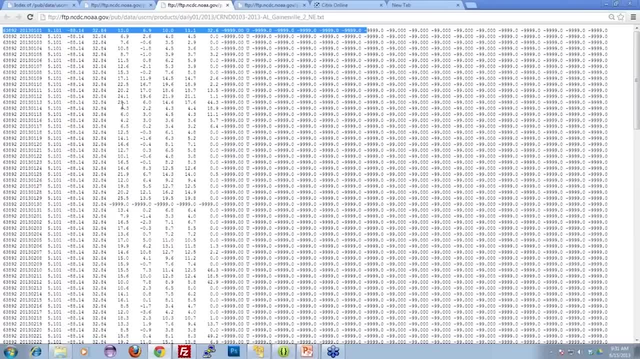 So awk or Perl or these are. these are scripts, scripting languages which can be used for record-oriented data, which can be quickly, which can quickly do those things right. So awk will be the fastest, Perl will be slightly slower, but again, very good for this kind. 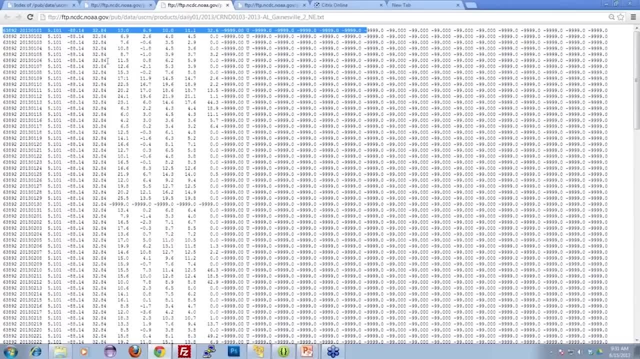 of thing. You can use Python as well. Okay, So it does everyone understand. what are what we're talking about here? Is there anyone who has no clue? I know a lot of people have understood, but anyone who has no clue can tell me. 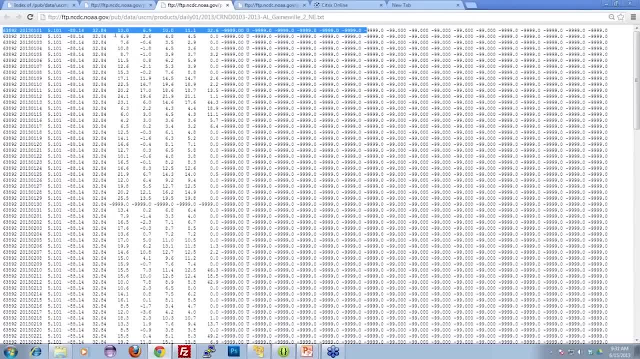 Okay, Everyone, most of the people have understood. So now, if I have to figure out, okay, Amrish is saying he has not understood. So, Amrish, let me tell you, let me make it very simple for you, Okay. 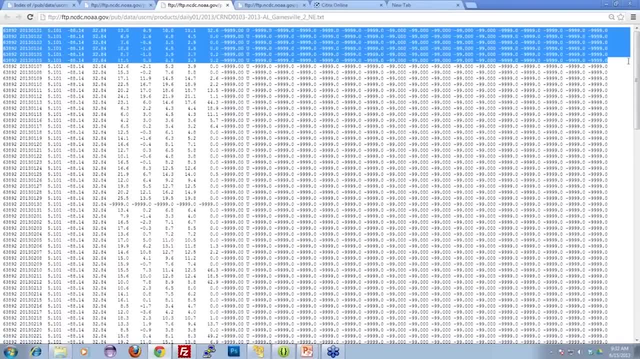 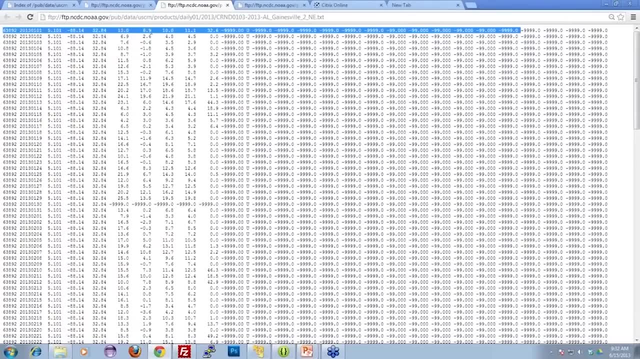 So now this is, this is this data has a lot of records, right, Each line is a record. Now, each line, This column is one value, Then this column is another value. This column is another value. This column, probably, is the date. 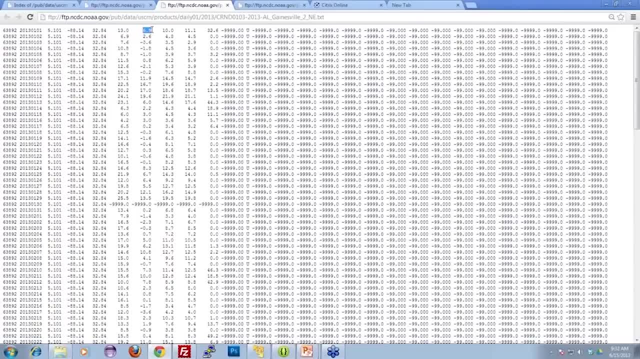 Okay, This column is the maximum temperature. This column is the minimum temperature on that date. Okay, And if I have to figure out that, what? what? I'll probably do all the remaining I don't care about, because I just need to look at what is the maximum, the minimum temperature. 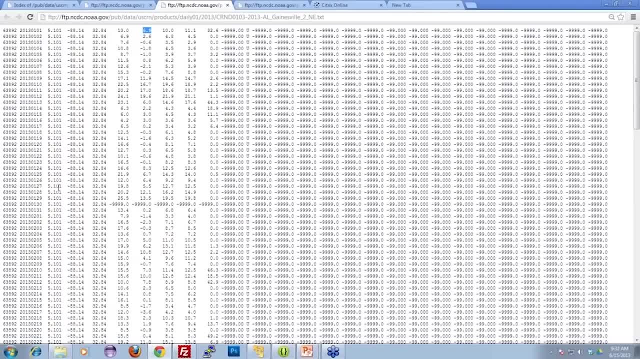 on a particular date, right, or on a particular year, right. That's what I'm looking at, only Okay. So if I have to look at that, all the other columns I can ignore. I can just look at these columns from each record and then do some processing to figure out whether it is the 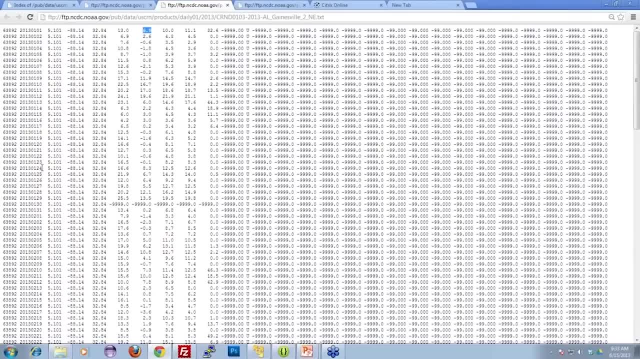 maximum temperature in that year, or not? Right? Is it making sense At a theoretical level? is it making sense? I'll show you how to do that. Great, Okay, So, yeah. So everyone has that idea. Good, Good Ravi. 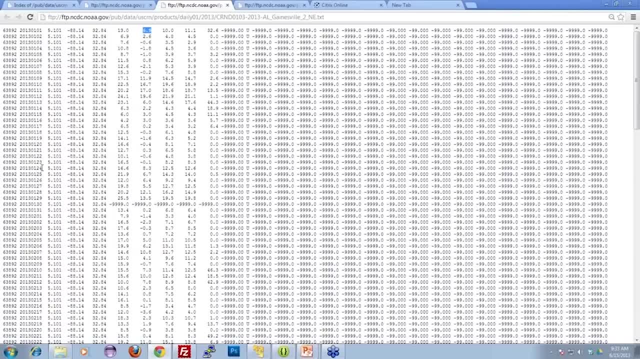 Thank you very much. Okay, Now, what I also want all of you guys to do when you go back home is to look at how does awk work. It's a simple language, Okay, It's a very simple language, But though you may not be required to do that, but it's always a good skill to have. 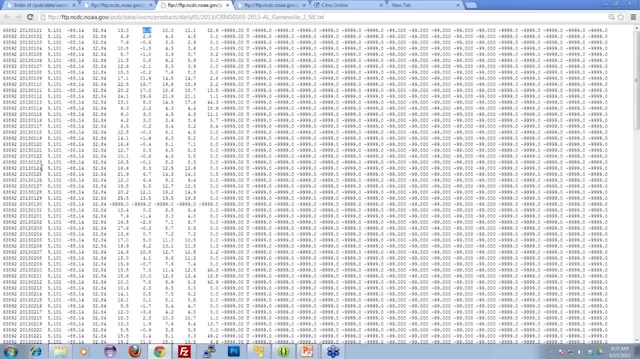 When you are working with data learning awk and a little bit of Unix is very, very, very handy Right, And I'm sure my friends, Ravi and other people who have worked on Unix- or maybe Dilip Dilip is a Linux administrator, I believe- 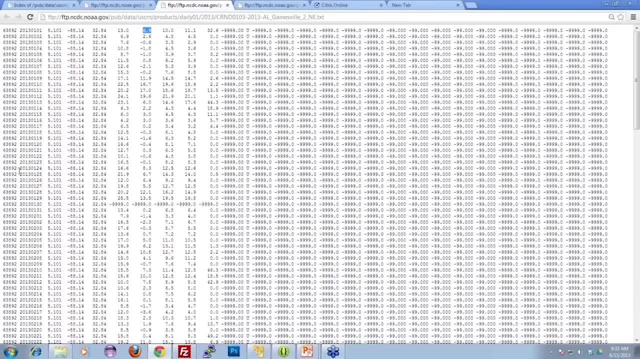 Dilip, you are comfortable with awk. Can I quickly get that answer? Great. So what I want, what I want you guys, Whoever is comfortable with awk, is to write a program in awk. Akka, don't worry about those values. 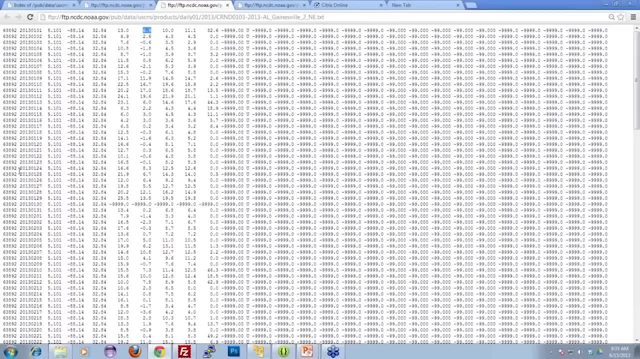 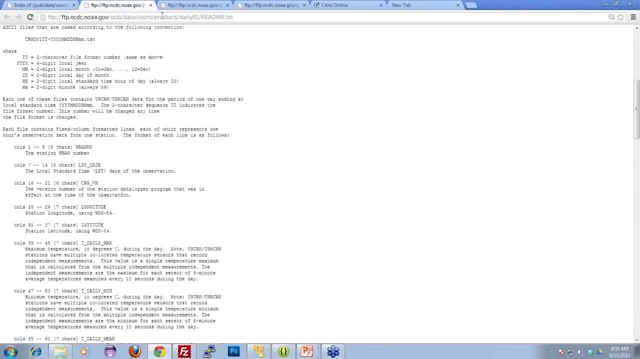 Okay, You don't have to worry about all the values which are there in the record. I also don't know. We just need to pick up some values. You can read this readme file to figure out. what all does this contain? Okay, 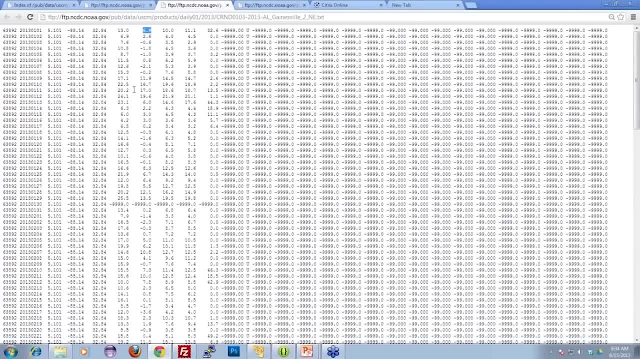 For now, let's concentrate on these three values. Okay, Now, whoever knows awk, I want them to write a program in awk Okay And send it across as an assignment Okay To us, In which we will give you this, one of these files and you have to use awk to write the. 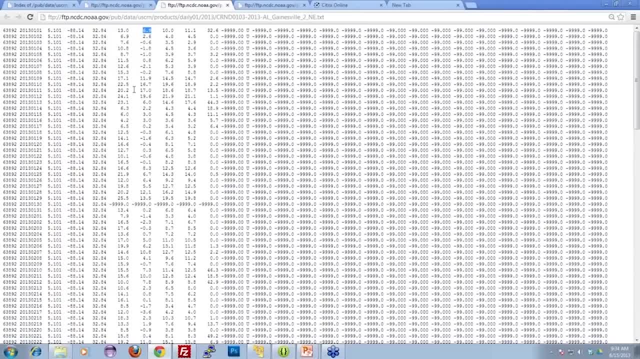 same thing which you're going to do in Java today. Okay, Is that fine? Everyone who knows awk. can you quickly give me a? yes, Great, And we will be sharing that with everyone else in the class. Okay, So I want you to write this by tomorrow, if possible. 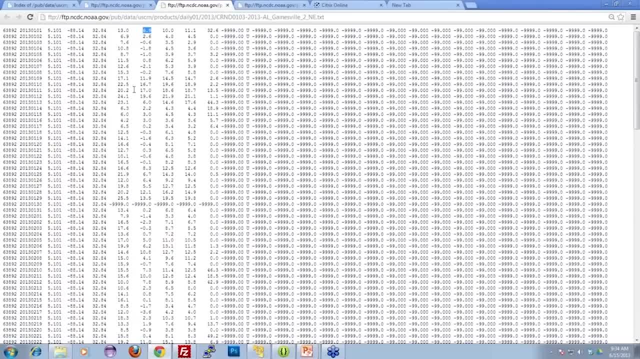 Whoever gives me the first answer, Dilip, and everyone whoever gives me the first answer gets some bonus points. Okay, So great, Sachi, Make sure. And other people who do not know awk- I want them to Google a little bit on awk. 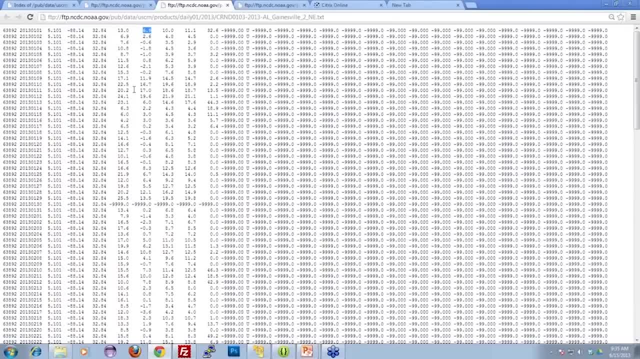 Look at this data and try to create a program in awk for doing this work. Okay, To find out the maximum temperature here. Is that fine with everyone? guys, We will be sending out the awk program as well. So by Thursday I will wait. 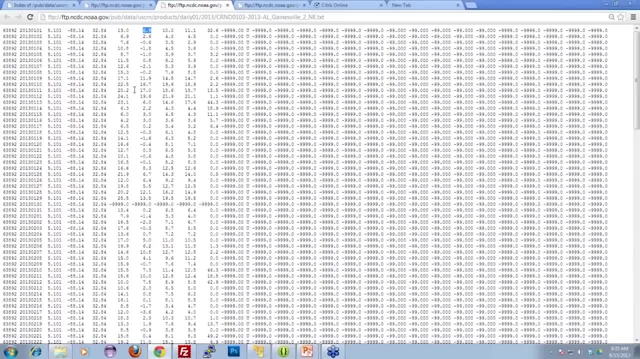 If I get an answer from everyone, then I will not send anything. Otherwise, I will write one and I will send one. Okay, Fine, So we will learn with each other, Right? So this is the same. Now, coming back to the slide. 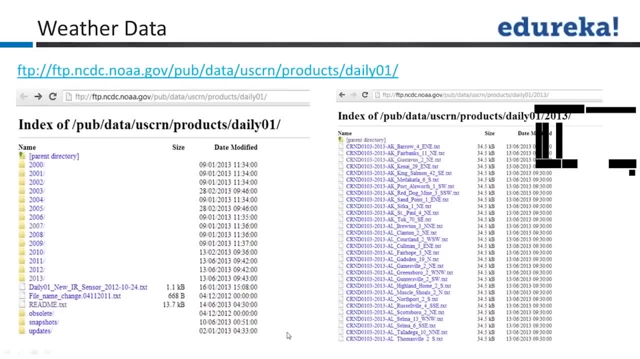 So this is what we used to do earlier. Yeah, we will be sending you the input files. We will be. this data set is available. We will be sending you the link to that. Okay, So input file I will send you. 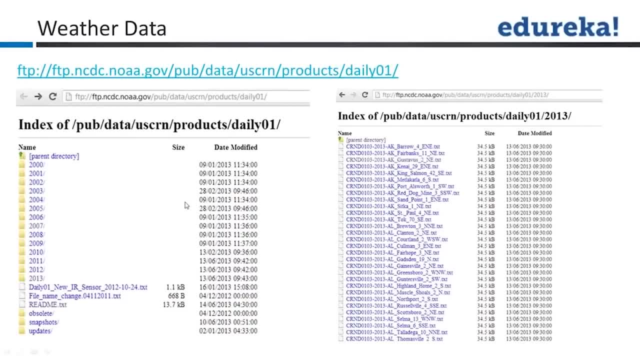 Okay, I will also. yes, Rajat, So I will also send you the exact problem statement just after the class. Okay, So do not worry. Okay Now. so this is this is what we used to have and, as you have- you have told me that. 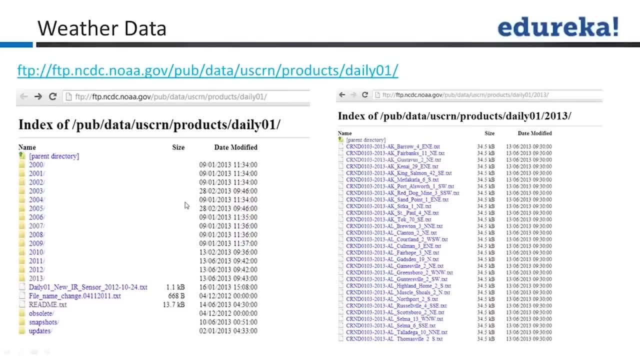 you could use awk to do this. So then we, if you could use awk to do this, then we could use awk to do this. Okay, So then we, if you could use awk, what is the problem then? Why do we need anything else? 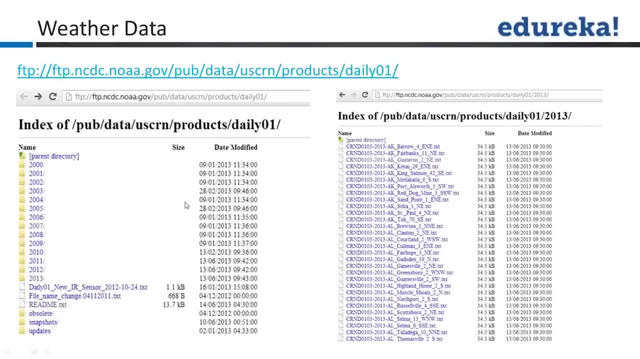 When I am so much. I am a big proponent of awk. I am a big proponent of Perl as well, So why do we need something else? Amrish? what could be the challenge there? Okay, Large number of files is what Vamsi says. 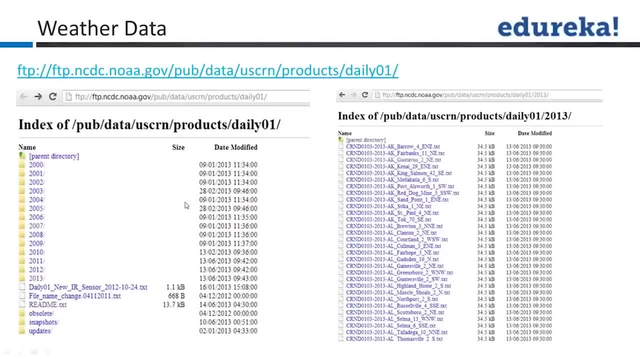 So large number of files can be done. portability is yeah. data volume with limited data set: Okay, Yeah. So there is a few things which we had to adopt, okay, Okay. So Sachi is telling you market is hard with adobe. 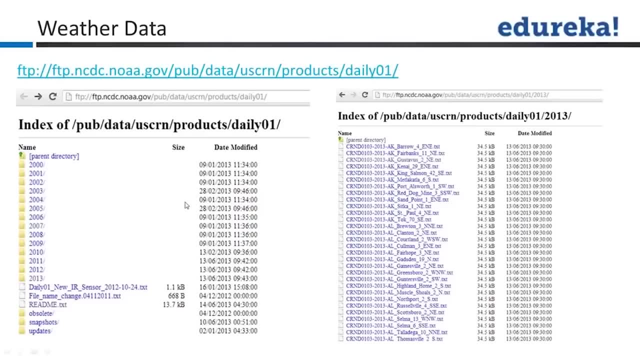 Yeah, that is a good answer. right, but okay. but the fact is that you can do a lot of things with awk. Now, the challenges are that, and I am sure you will yourself figure it out. So what I will probably ask you to do is write the awk program to run it on a small 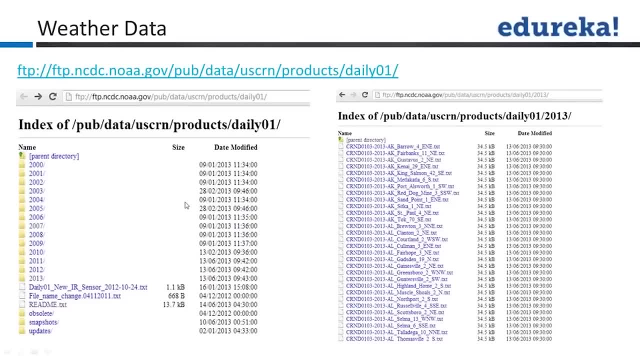 data set, which is one of these. These are few questions. Okay, KB files. now, when it becomes terabytes, then the problem is that, as we saw right from the first class when I was telling you what is the challenge in the world- not storing data, 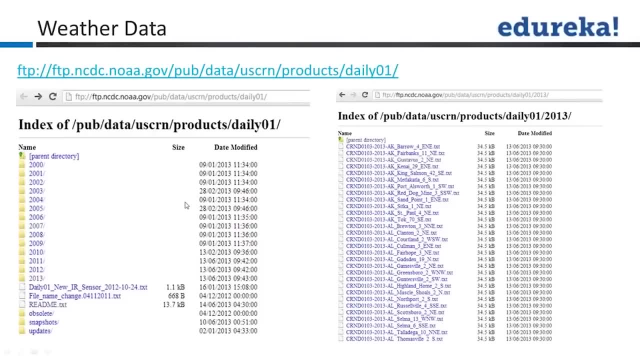 it is reading it and analyzing it. you remember that thing which we showed you in the first class itself, where we showed you the time to read from a single machine versus time to read from a distributed fashion. everyone remembers that figure. seek time is the problem. 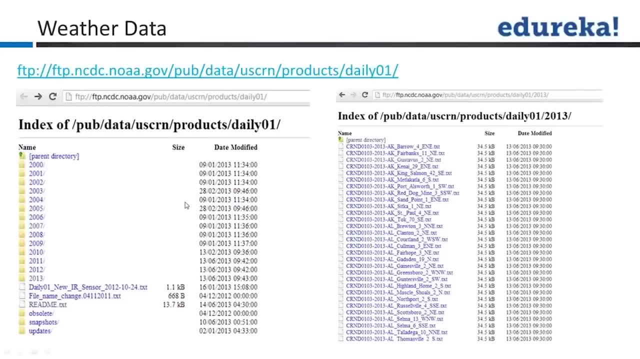 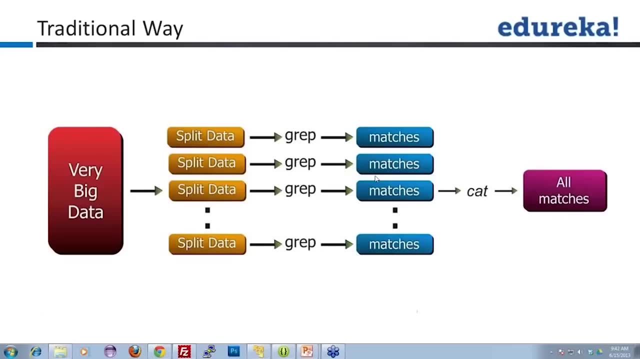 so that's why awk also, or any such program, will have a problem. So what could be the problem solution for that? even if we have, so we can split that data right. so if I had, if I had see, if I had so many files, I could split this data. 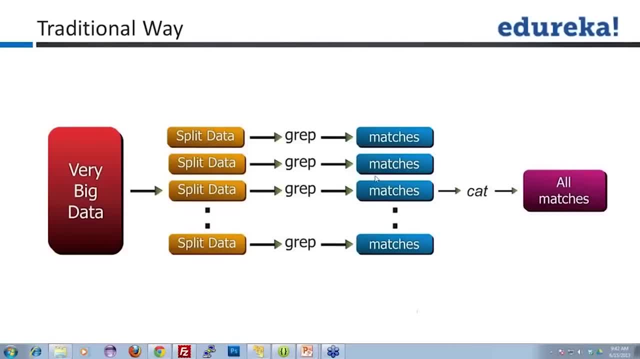 do a grep, or I mean, I have made it very simple. we did not need to do any awk, we just need you can do grep. also, for the people who do not know grep, please look in. grep is the command to take out a few regular patterns. 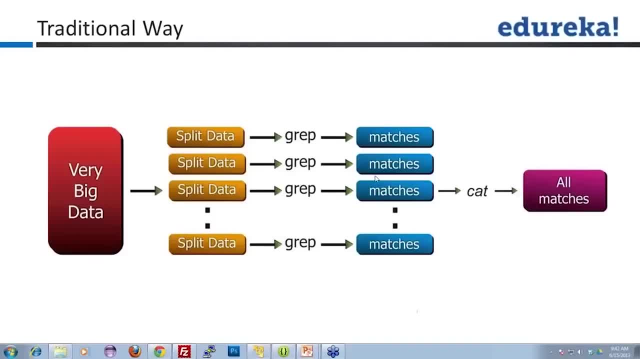 So whoever does not know grep, go to a googling on grep as well. right? so if we had, as we saw, right, if we had- huge amount of data, what would we do? this is your very big data. now, one of the files which we saw was this data only. so what I will probably do is split. 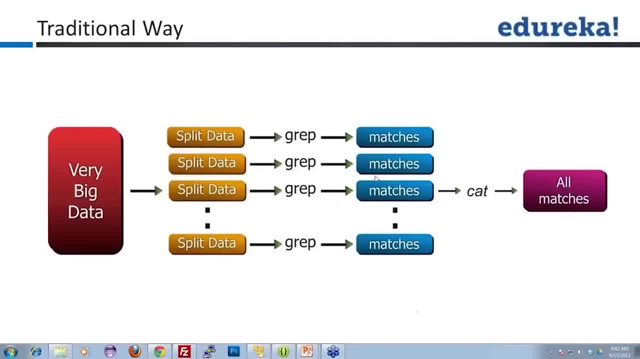 this data into multiple files and then do grep on each of these whatever matches, do a cat and create a final output. right, all matches can come here, right? So is it making sense? that would be. that will be that, obviously, the next thing, which. 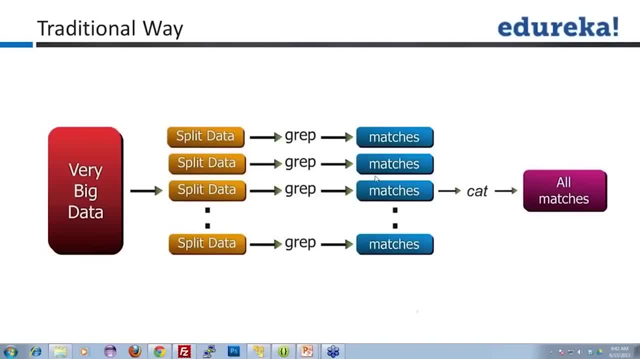 you would think of doing. is that correct, guys? anyone who is not with me till now just say no, everyone is with me. great, Now you have to tell me. the next question I will ask is: if everyone agrees with this, then what are the challenges in this approach? can someone throw some light on that? what? 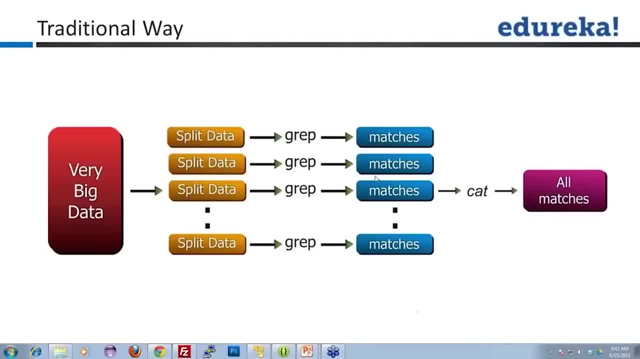 are the challenges in this approach? The approach is very simple. you have very big data, split it into multiple data sets, run it on different machines, splitting the data, time consuming. it was time consuming, that's why you split it. So don't worry, arc of what pattern? let just yes. so one very good thing, which the bunker. 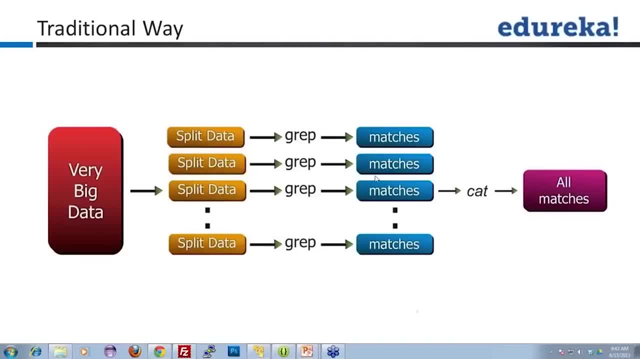 has told me is: yeah, reliability is one answer which I have got guys. yes, very important thing. reliability, failover mechanism is what the bunker is telling me. what else is there? anything else? computation is not done. Avinash at one place, we can compute it at multiple places. 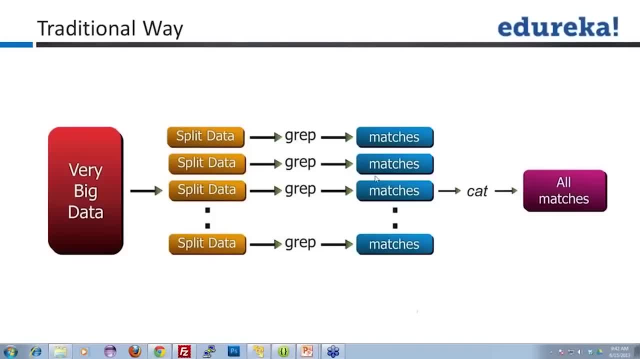 also. so the solution is simple, right. what I have done is what I am saying is all this: you split this data, put it in different machines and do that, Do that thing parallel, do it parallely. only now, I am not, I am not saying that, do it in. 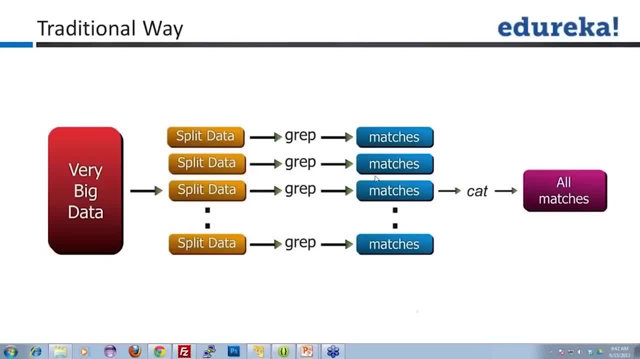 sequence or in single machine. I am. I have agreed that we can do it in parallel. so you have said one terabyte of data. ok, split it into, say, hundred parts and then do grab on different machines and then do a cat. so this is feasible. right, that's what. this is feasible. 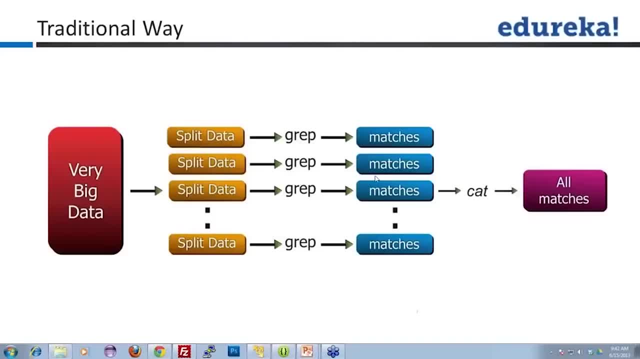 if I have to do these two operations is feasible, right, great. So now I want to know what are the, What are the challenges in this approach? why do we need something else, something, something which has taken the market by storm? so, once you see, Hadoop is also working on Unix only. 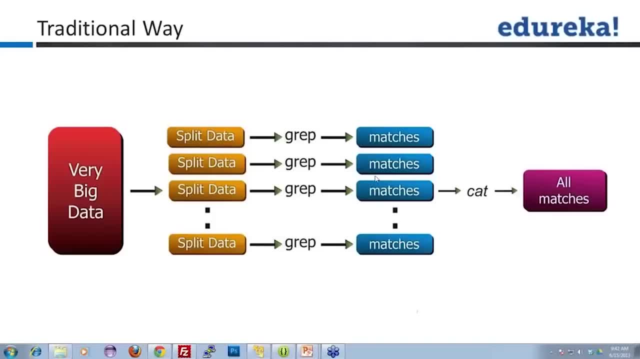 right, and this can be done in other things also, other languages also. Unix is one way of doing it. I mean, similar things will exist in other languages as well, right, other platforms as well. so that's not, that's not really the thing. so why do we, if we could do this here? 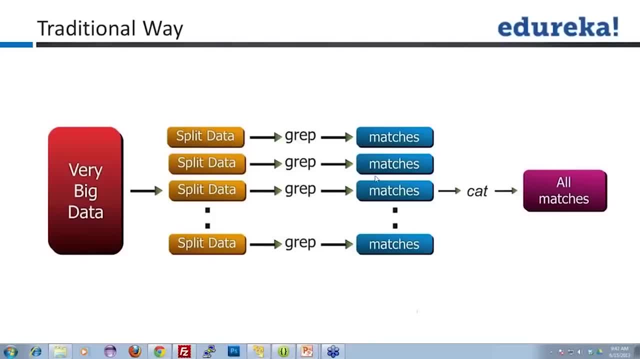 ok, ok. So So now Rajat has given me one answer. ok, Tush, ok, great. so Rajat is saying: failure on one machine can corrupt the entire matches. right, so that's one good answer. ok, it is not robust as Tushar is saying. Tushar is saying the job to split and integrate after cat is still. 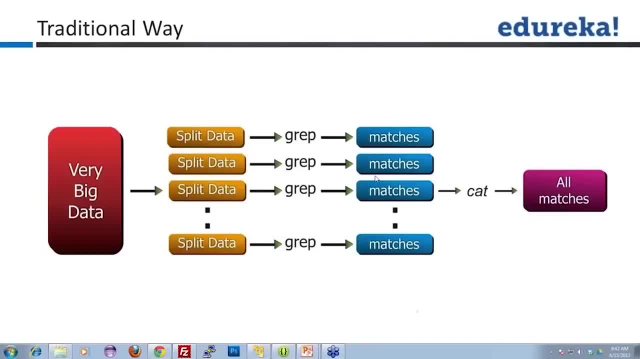 a manual process. well, my friends Dilip and Ravi will quickly create a script for that as well. that should not be a big problem. they can do that, but then? but then you have. I have got very good answers. now I think most of the answers I have already got right. Orca is. 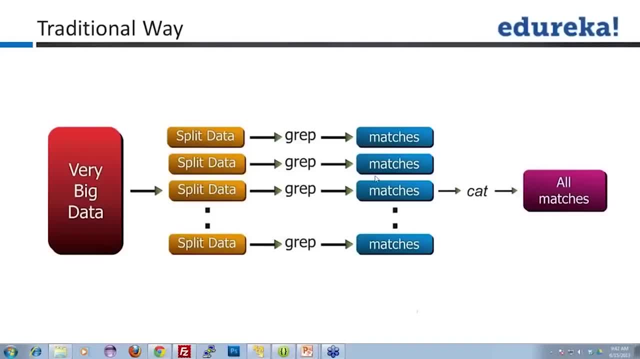 saying, instead of reading record by record, it will be read block by block. ok, fine, that's. but finally, see, finally, you will be doing a record. it will be read completely, block by block, but when we do a analysis over it it will still be a record by record analysis. 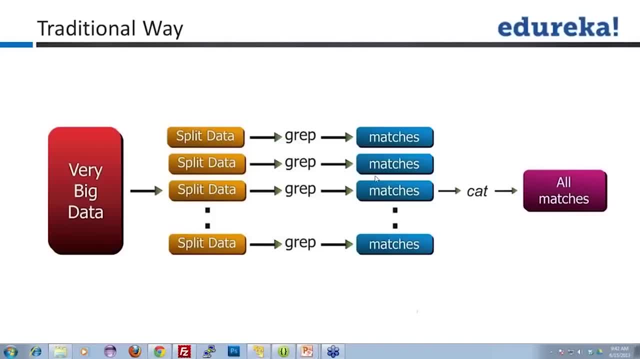 right and we will show you that. so that's not really the reason. see one, have you ever heard about critical path? Everyone knows what is the critical path, you know? ok, ok, some people have, some people have not. right, I am sure whoever has done a PMP exam, they would have. that is the first thing. 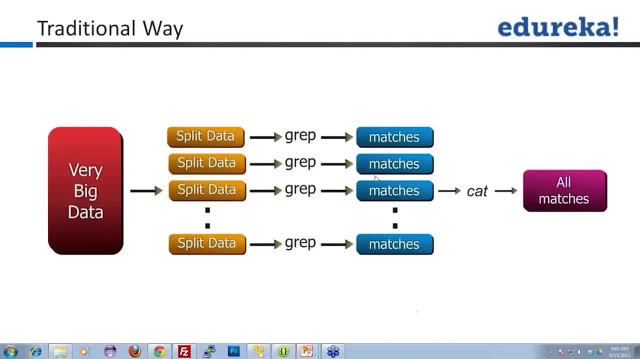 everyone will know, but you don't need to know. do PMP for knowing critical path? see. critical path means that: ok, Ravi, yeah, great, ok, ok, yeah, yes, Ravi, right, that's true. so don't need a PMP to know critical path. You can know critical path and still not be a PMP, ok, but anyways, you don't need any, see. 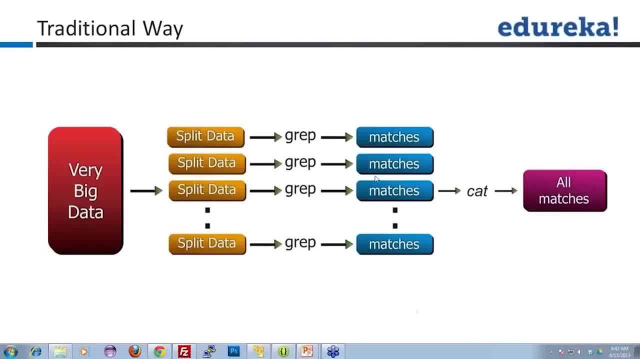 the reason I am putting this thing here is that one very important thing is that now it will also depend upon the machines which you are using. ok, and their processing capacity of each machine. ok, will be important here when we are splitting this data right, and if a machine is one of the machines actually is a smaller processing capacity machine. 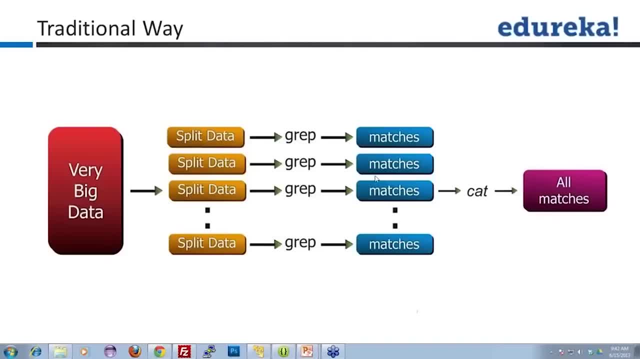 Then that will become the critical path and it will delay the process for everything. is this making sense to everyone? say, for example, this: this graph is done very slowly. all these were ready. this took two hours more, so everything took two hours more, right? is that? yes, so right. 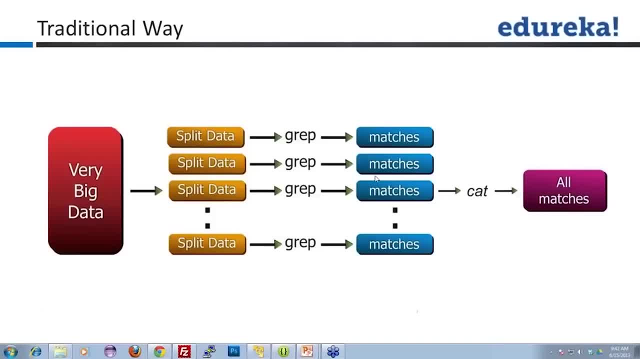 is that making sense? so that's what critical path is? so anything? now I want Ravi, who is a PMP, to define critical path for me and I will read out that definition. Ok, So that yeah, Ravi, I want you to actually speak, if you, if you, if you can, if you have microphone. 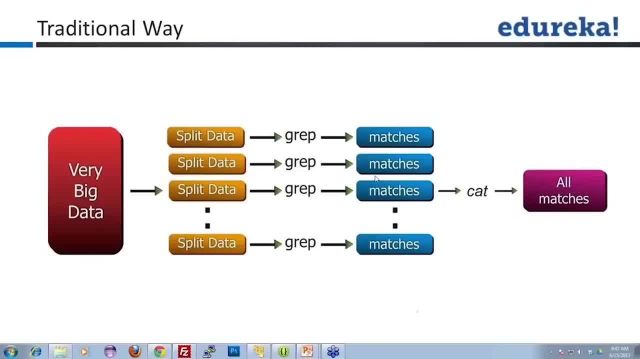 ok, ok, ok, ok. so Ravi. Ravi is saying, Ravi is saying I will not. I will not. who is going to define critical path for me? I mean, you have Google as well. everyone can go to Facebook and look at that, but you have to define. 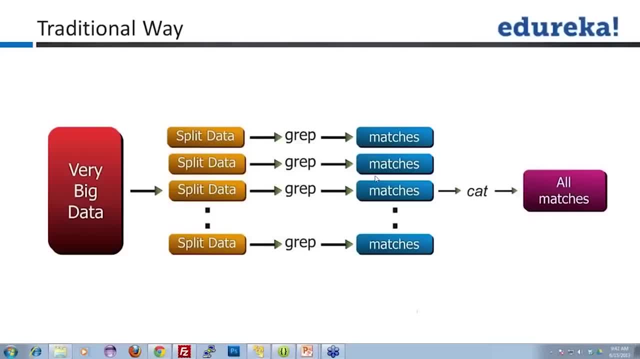 Somebody has gone there. Rahul has gone there, Ramesh, Ranjit, Vamsi, Vinod, all of all of them have gone there. other people, Sriram, you already know what a critical path is. you might as well appear for the PMP exam after this class, because you are going to know what a critical 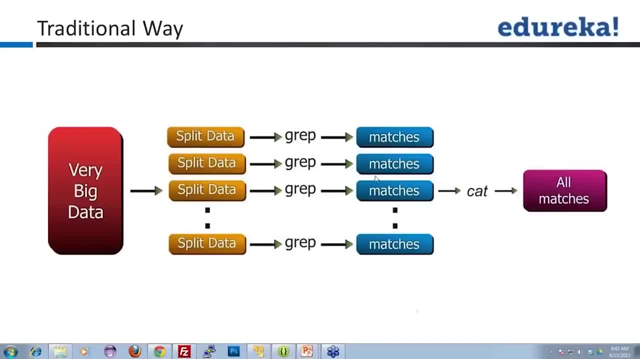 see how, how many of you are actually managers. very good, Rajat has given me the right answer and he is a. Ok. Ok, Vamsi, don't worry, you can check on your mobile. ok, So Rajat says I am PMP certified. congratulations Rajat for that, and it's a good thing to no. 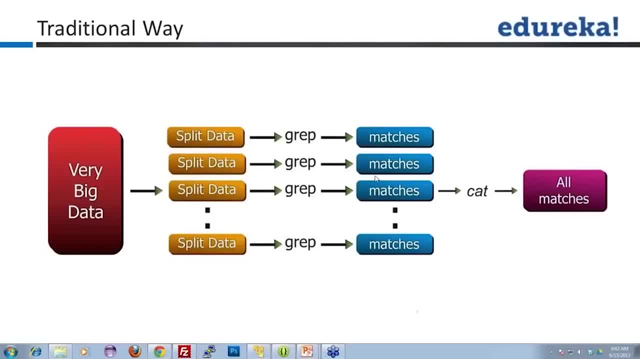 I can't trace mobile phone usage. you know I can't do that, I can't do that. So yeah, so Rajat has given me the definition. thank you, Rajat. I will just read it out for everyone: and and it's actually, it's actually a very good definition, a very accurate one. 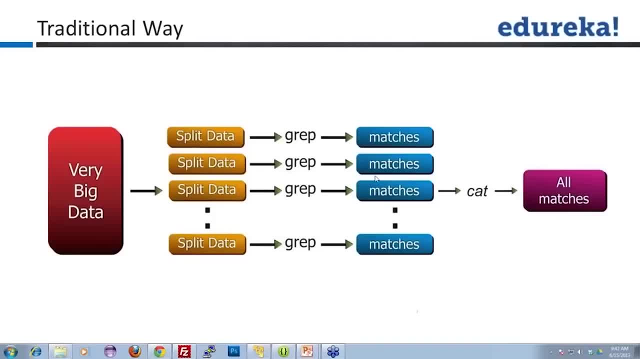 Rajat says it's the amount of time to take finish the job without delaying the next milestone or actual completion date. right, I will repeat it once. please pay attention everyone, and I want everyone to say thank you to Rajat for that. Rajat is saying it is the amount. 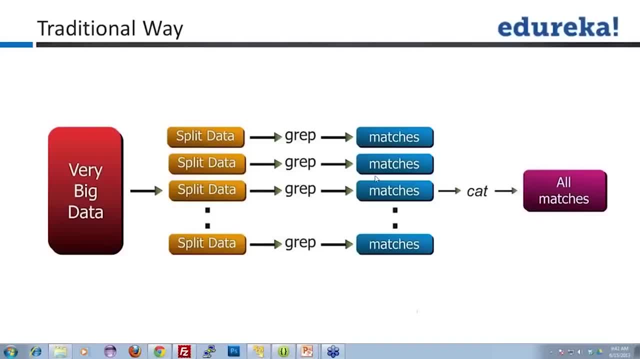 of time to take, time taken to finish the job without delaying the next milestone or actual completion date. right, so is it? does everyone know what is critical path? now everyone is saying thanks to you, Rajat. ok, great, So now see, this is. this is the beauty of having so many people in the class, because everyone 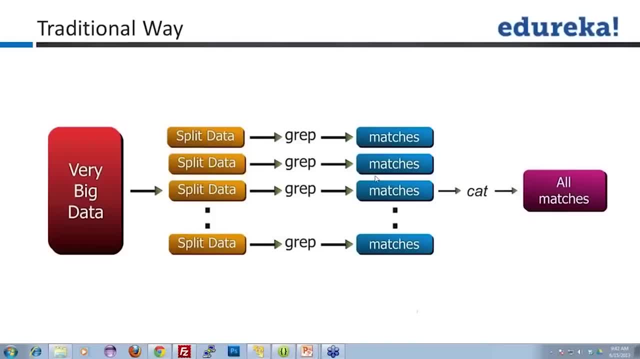 can give us something. So Rajat has take, yeah, great. so now, as I told you, right, if one of these graphs end up becoming a critical path, see, first thing is: can you really split the data into equal parts? that's one challenge, right, because you may not be able to split that now if this is yearly information. 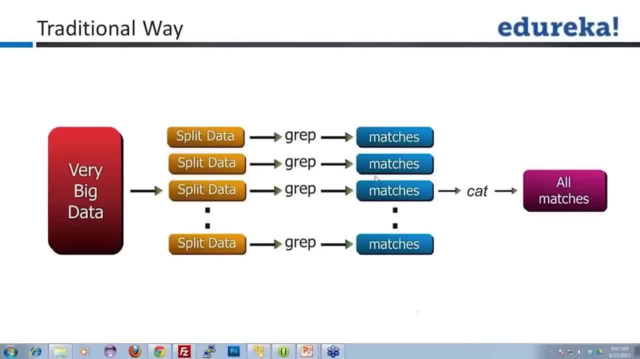 also, it is possible that in some years there are more records, in some years there are lesser records, right, and it is very difficult to actually split. that does everyone understand, that? Does everyone agree with that fact? and even if we split them equally, then the next challenge. 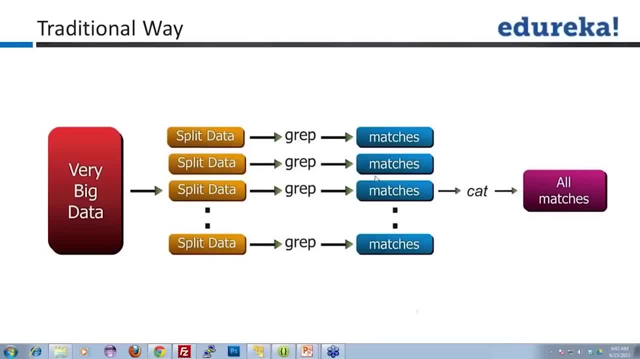 is the critical path problem right? so two problems we understood. first is splitting in equal proportions may not be the best way to handle this, because sometimes same data, which we would have actually easily managed it was in the same split would have gone into the next split and it would have led to a problem. I will show you this example of this. 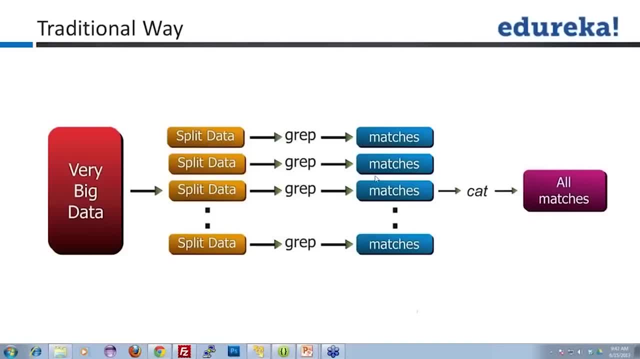 later on. ok, where where this could be a problem, ok, but on a on a higher level, you want the data to be in the same split, right? so if I am actually looking at the yearly distribution of something, and in one year that the number of values are more, and I want to just figure, 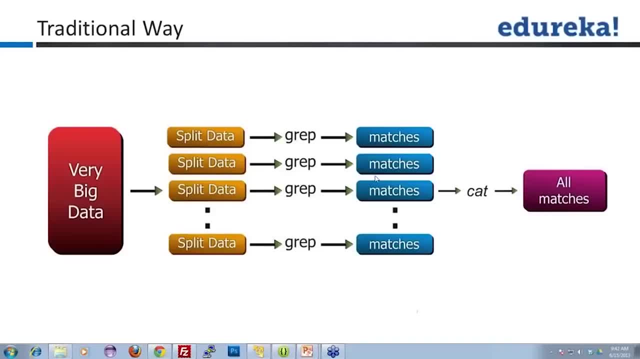 out what is the maximum in that year. it may be a good idea to actually put it in the same split, instead of splitting one years value here and putting it across the same in this. if you have two year values right, then what I get is not the yearly max, but the maximum. 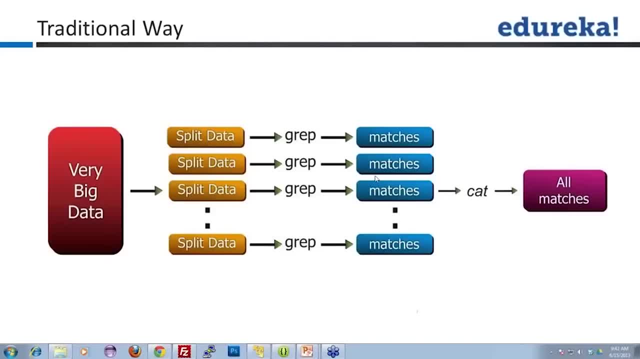 max of the split right. is that clear to everyone? if, whatever monologue I just gave on the equal split thing, anyone who is not clear, I will explain it again. great, so I am getting a lot of smileys today. thank you very much, guys. clear the bunkers is clear. great. so, yeah, keep. 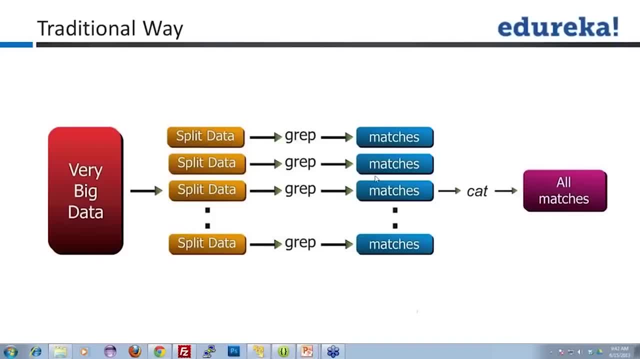 on. keep on sending smileys, if you are able to understand this. if there is anything which you are not able to understand, feel free to stop me. ok, great thanks, Parthivan. thank you very much. ok, Now, one challenge which we have understood is that dividing them into equal splits may. 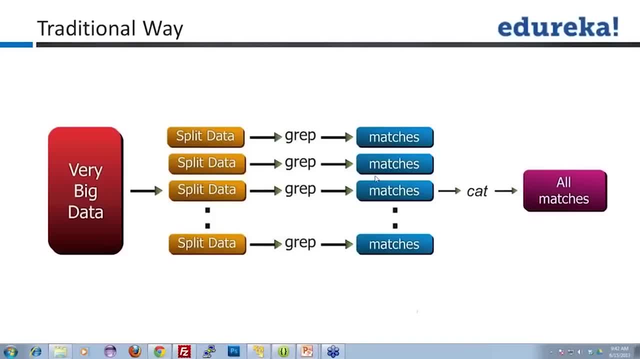 not be the best idea. and if we do not divide them into equal splits then we will surely get into this critical path problem. that is also clear to everyone. but even if we divide them into equal parts then also we might get into. look at the usage of the ring. we will. 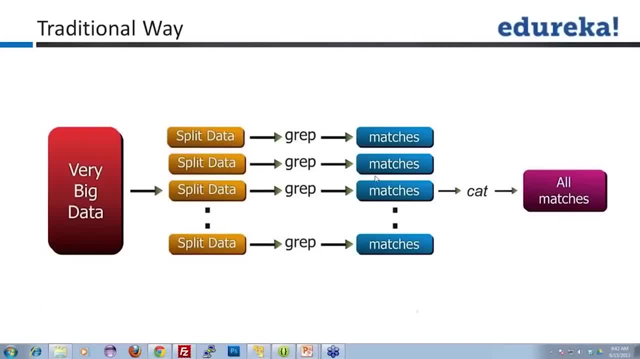 surely get into a critical path problem when we do non-equal splits. is that correct everyone? and if we do equal splits? So in a few minutes we might get into a critical path problem. is this sentence clear to everyone or has it gone over your head? ok, got a lot of smileys, so I agree. I understand it is clear. 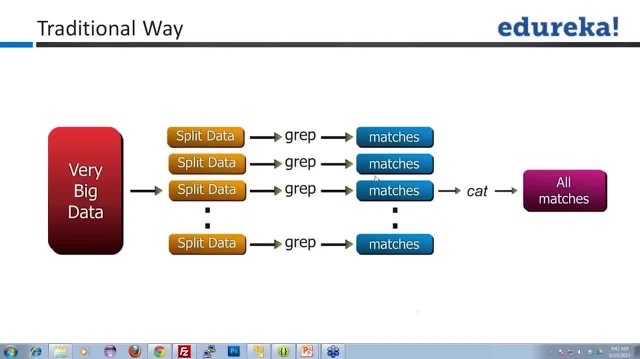 ok now anyone in the class Tushar Sriram who are not in the last class. if for some reason, you are not able to follow right, please do not hesitate in asking. all of our batchmates have agreed that I take a little longer to teach something. so they have agreed and they. 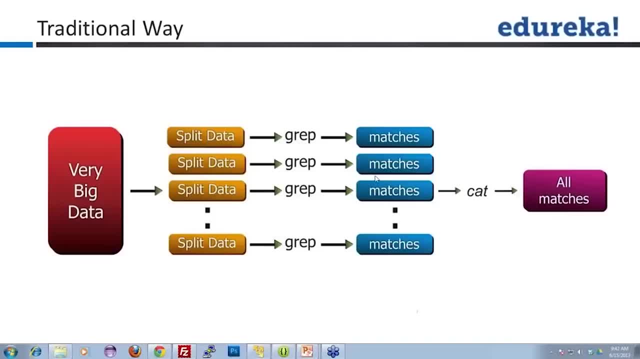 have agreed to this. They have agreed. they have said that it is fine, they are ok to wait a little long, so please make sure that do not hesitate to ask. ok, thank you. thank you Sriram, ok, and thank you everyone else. you know you are still with us. it is not too late for you not sleeping. 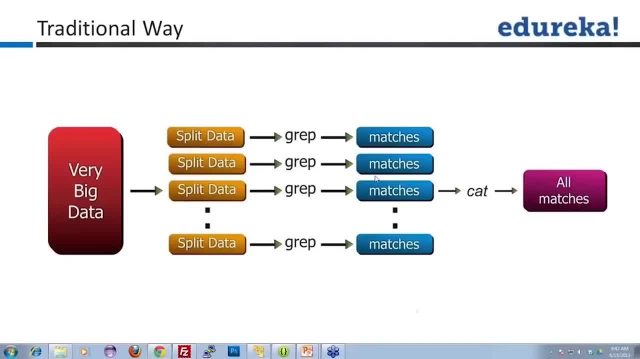 anymore till now. ok, So now these two things, these two things, ok, great. so two things which we understood. one was that splitting is the natural way of doing things, but the challenges with splitting could be that splitting equally has its own challenges. Ok, One challenge: non splitting equally has its own challenges, right? and then you do a cat. 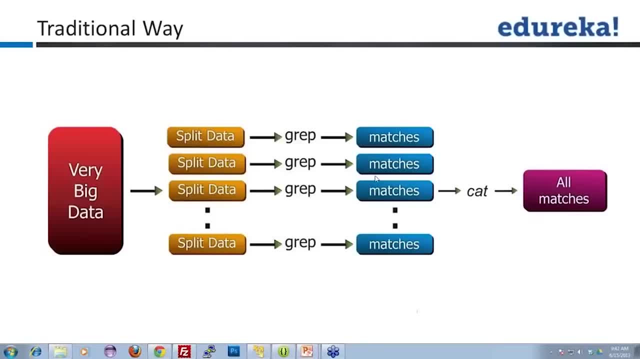 ok, now, these are the two very important things. the second, the more important thing, then another important thing comes in the reliability. one of the machine may fail, right? how will you make sure that the reliability thing is taken care of? right? that is another challenge, right, isn't it? guys? smiley quickly if you agree to that. if one of the job fails, then probably 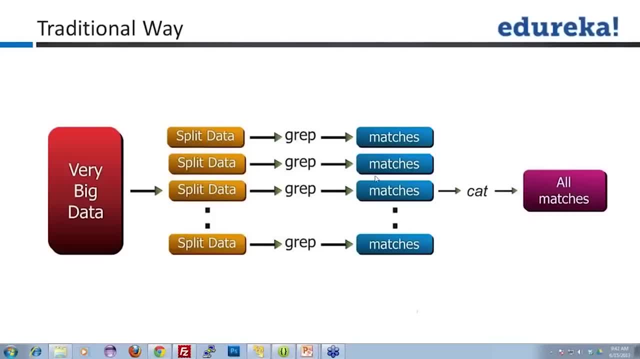 thanks, Sachi. thank you very much. Now, if one of the job fails, then you have a lot of trouble, right? you don't know whether you got the right answer or not, because if you are looking at the maximum temperature in a century and the machine on which the hottest year was there failed, then you get. 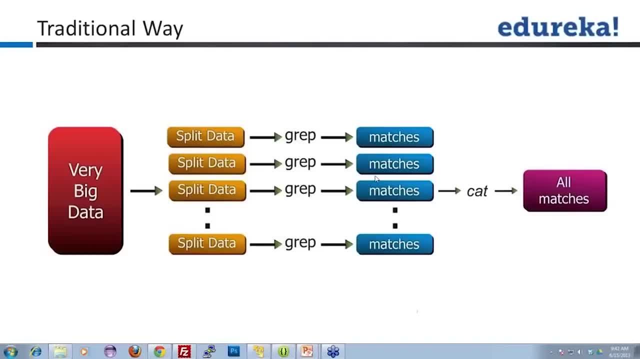 inaccurate results, right, true or not? So reliability plays a very, very important role here, right? so that's very important, thank you. thank you very much for see be interactive in the class. I am sure everyone will understand at the end of it. ok, Now. 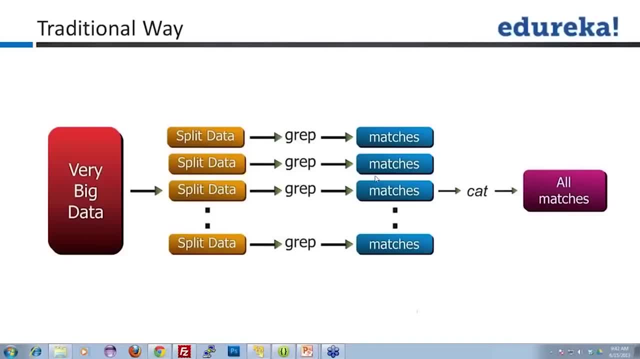 Now tell me, these are all running in a different machine. who is going to run the overall job? someone has to run this overall job also, right? which Dilip would have written in his script that split this. do graphs. graphs are done here, then do this cat and then final result. 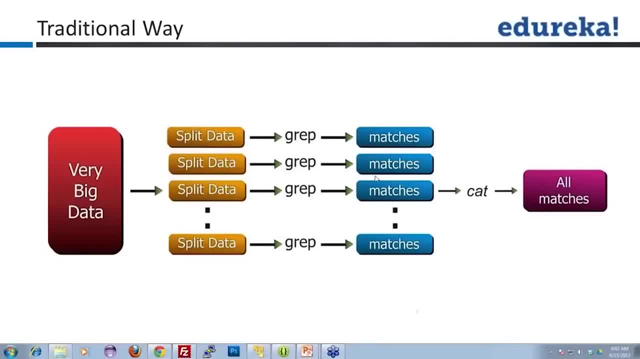 right. So now, Rajat, let's not get to job tracker. ok, let's not. I am not talking. we are not talking about Hadoop. we have not reached Hadoop till now. ok, let's try to understand who is going to. who is going to do this? 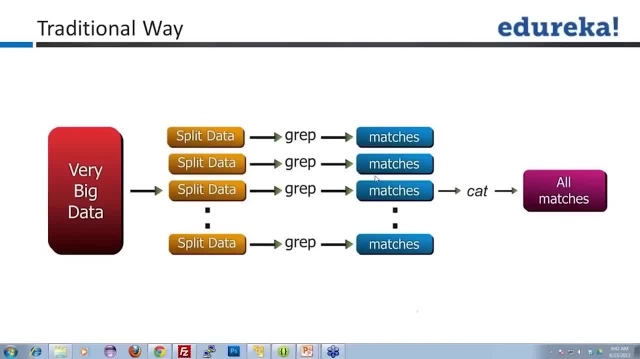 Who is going to do that overall job here, right? So that's one challenge, isn't it guys? So the challenges which we have are quickly- can you quickly write it down on the chat window- what all challenges I talked about till now. I will also repeat it once again. 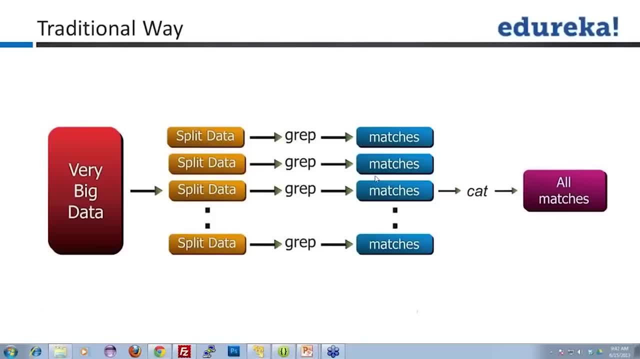 because that's all. those are the things which are important to understand. reliability: one: splitting the file- very nice. unequal split has its own challenge, right, master job, very nice. reliability, if one machine is down: very nice, ok, one more thing: critical path, incorrect results due to failure- right, very nice. 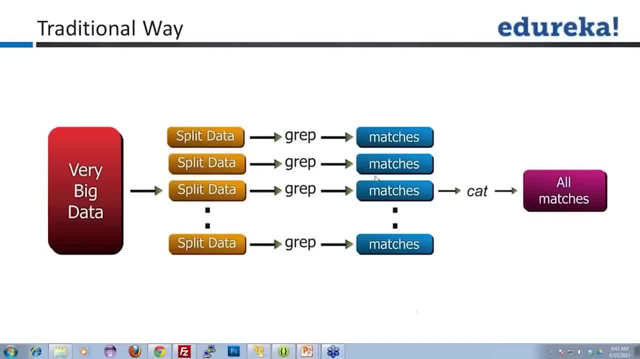 So these are the challenges right now, theoretically and practically also, this is all possible. right, you can write a very good framework, which I am sure a lot of you who are hard code programmers, and I will probably say Avinash and Ravi- I will just pick these names- of Dilip, 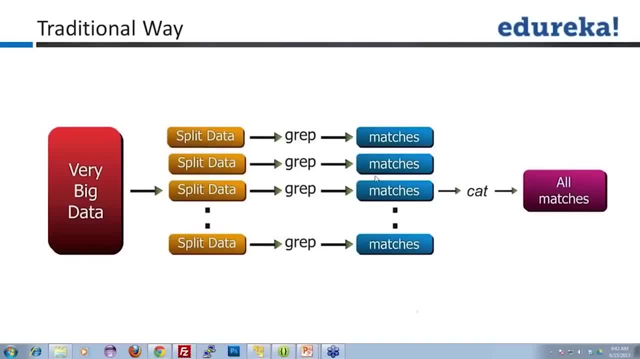 because they have told me that they are hard code programmers. scalability also is a challenge, right, Dilip tells me. right, who have done a lot of programming in Unix. they will claim that if a company gives them this job, they will be able to do it ok. 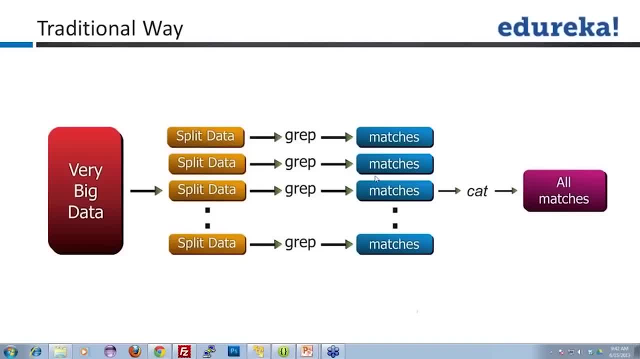 So yeah. so, Ravi, I will agree when you send me this org program by the end of this class. ok, I am just being a little early in the phrase, but I want you to send the org program. ok, yeah, ok, thank you. no, not at all, Ravi, not at all sarcastic, I am just. I know you guys last. 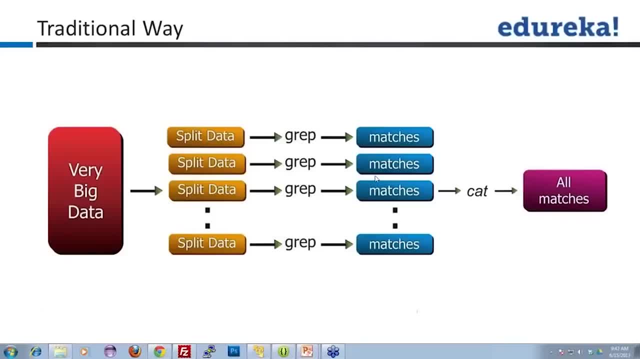 time also, I had a class with you. I learnt from you guys as well, so definitely you shown me that promise. so, please, so, yeah. so coming back to the, coming back to the fact that these are the challenges which we have now, any great programmer or any great guy who claims that I mean not even. 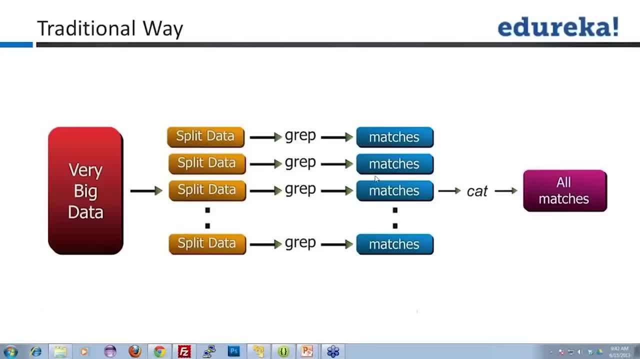 claim them. a lot of you people have been from the software background. I am sure a lot of you will be able to create such a program, right? how many people think they will be able to create such a program which can take care of this? Avinash says yes. 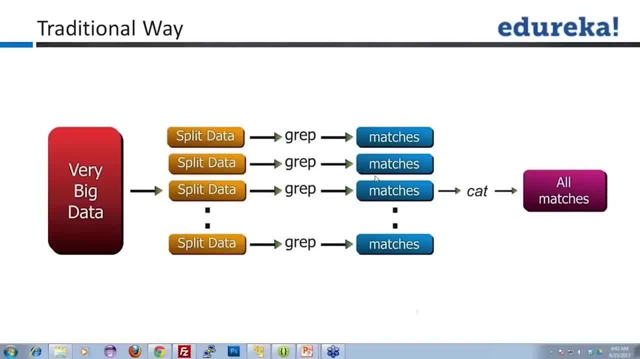 Rajat also says: yes, Rajat, I will come to that. ok, Rajat Behera- there are two Rajats in the class, so please don't get confused. I will call Rajat Rastogi as Rastogi and Rajat Behera as Behera. is that fine with both of you, ok? so Behera is asking me a question, just. 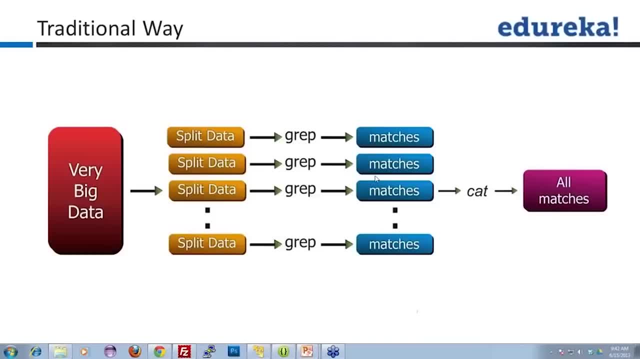 confirm my understanding of responsibility challenge: who will be doing what and when? ok, Rajat, I will. that is not a very good question. Ok, That is not a very good question to ask at this point of time. very soon we will come to know that, ok, but I will quickly answer that. so there will be one overall job which 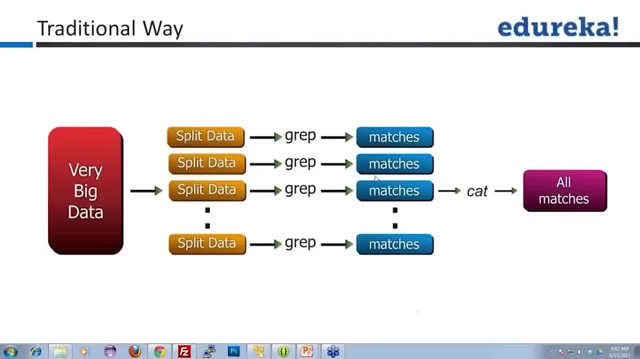 will be managing all these things, splitting and then pushing these jobs on different machines and then doing a final CAT and showing it that is the overall responsibility of someone who has to do it. then these machines have to do this grep, someone has to do this CAT right, so we have. these are the kind of problems which we will have. these are things we will. 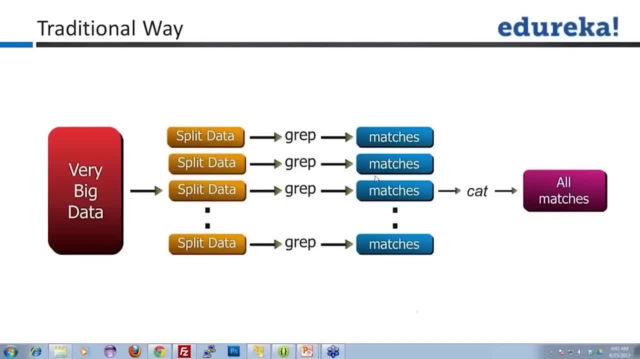 show. so Ravi says: difficult, not sure. ok, sync, sort is what? ok, sync and sort, right, Ok, so with JCL and COBOL the bunker will be able to do that. ok, now, how many people think they will not be able to do that? time taking is what Ashish says. great, so there will be. 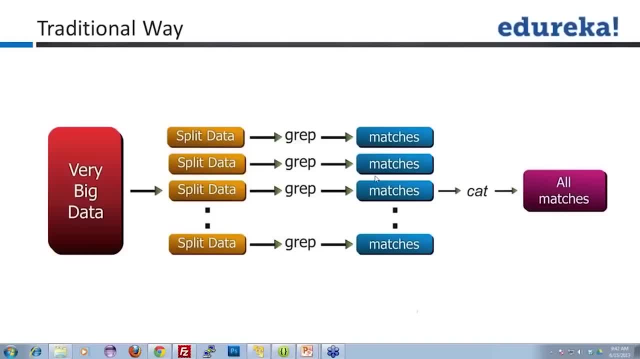 a sorting also involved, right, very nice. so I think by the time I reach MapReduce, right, you would have actually told me that. no, I am not saying at this point of time. if I give you two days time to write something like this, Ok, so through, ab initio, I can do that, says Orca. ok, so if I give you seven days time? 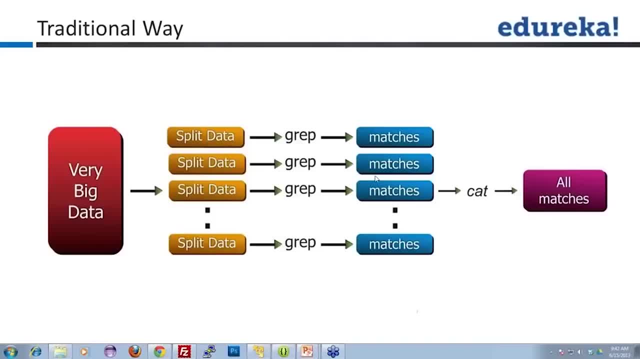 can you write this program and give it back to me, which can take care of all the reliability issues as well? see, Ram says I can create a OLAP queue and get it done. ok, ok. so I am sure some of the people can do it. some people cannot do it. they want to use different technologies. 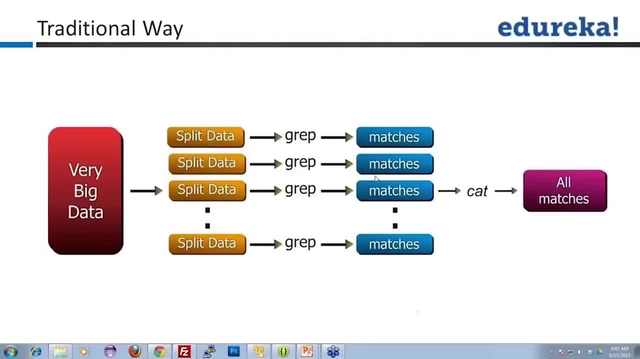 for doing it. it is impossible to determine the failures not speaking to each other, right? so it is. yes, it is very difficult, right, Ravi? that is true, Ok, So now, who does so? you know why do we need something else? now everyone understands God. 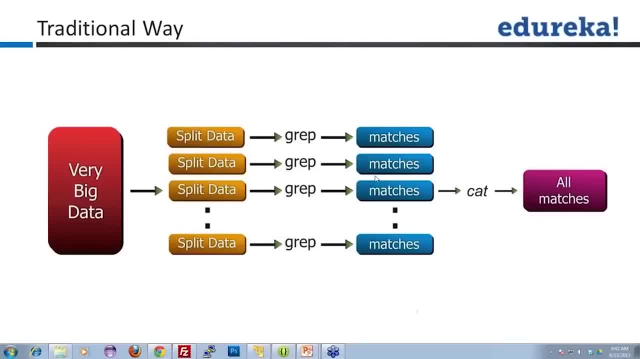 gave Hadoop. why you stairs when you have a lift? wow, yes, Ravi says God gave Hadoop. why you stairs when you have a lift? right, so very nice, thank you very much. thank you very much, Ravi, for that great piece of poetry is what I will call it. I am not very good at English. 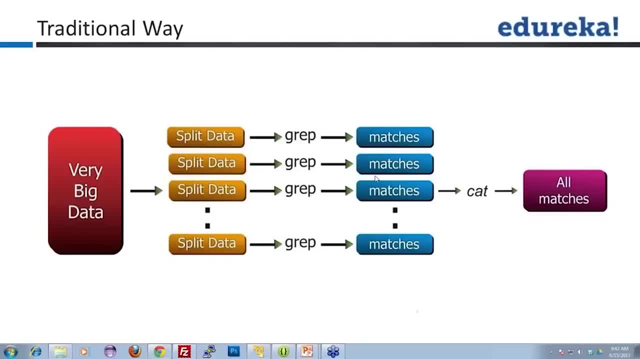 so, please, wisdom is what the Pankar says, right, so that is a wisdom nugget from Ravi. ok, my friend who is lift, ok, so I am see saying lift can stop in case of power failure, when we are over what do we need to? ok, so Ramesh is telling: when we are over with, then we need 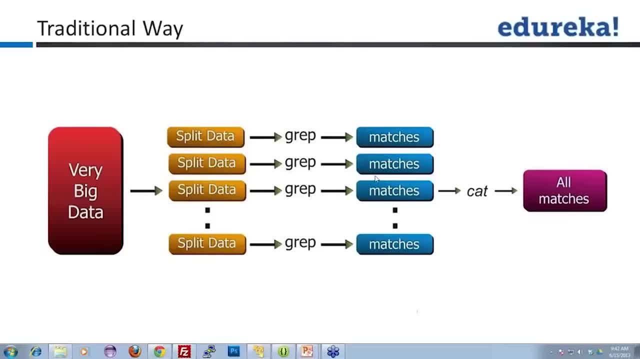 to use stairs sometime. ok, use stairs in case of emergency. that is why I am telling you guys: learn orc. ok, so not. Hadoop is going to come to your rescue every time, but if you do not, every time when you are given a job in the data set will, so use that you will. 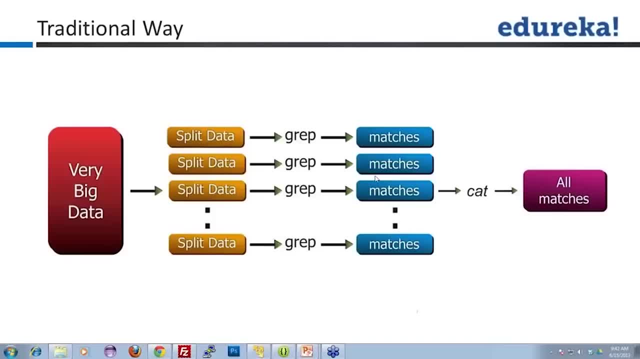 tell your management that I will use Hadoop to do it. ok, they will throw you out. what you will get in response is a pink slip. if you tell them that I will, I want to look at these logs and use Hadoop to do this. ok, so you should- all of you should- actually learn orc then. 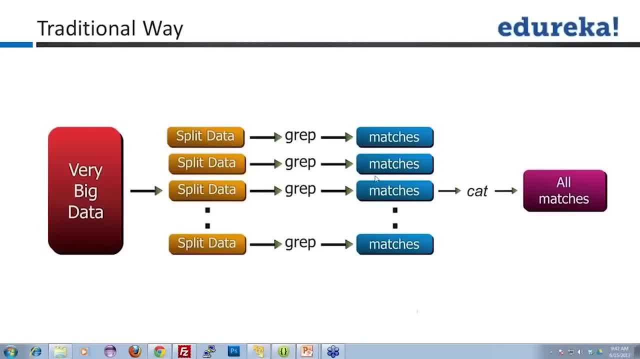 orc comes very handy. very few people know them. you can also boast that you know orc in your office. ok, so told. so definitely learn orc. ok now, now that you have started learning and established the fact that there are some challenges with the traditional way- and we have also looked at them- that processing capacity of each machine, splitting the jobs, the critical, 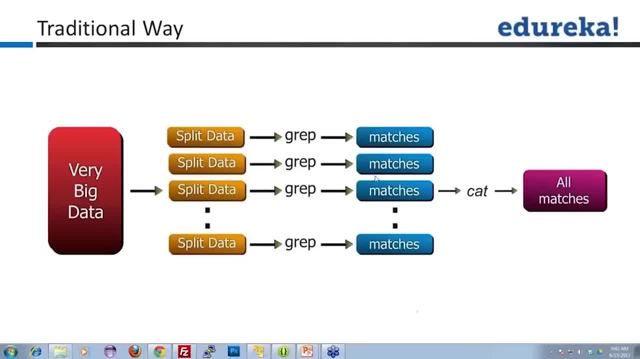 parts problem, reliability, field jobs, who runs the overall job? these are the challenges, and so we got a lift then right and the stairs could be orc, but we got a lift. as Ravi says, that is where our way of doing things, the MapReduce way of doing things, helps right. 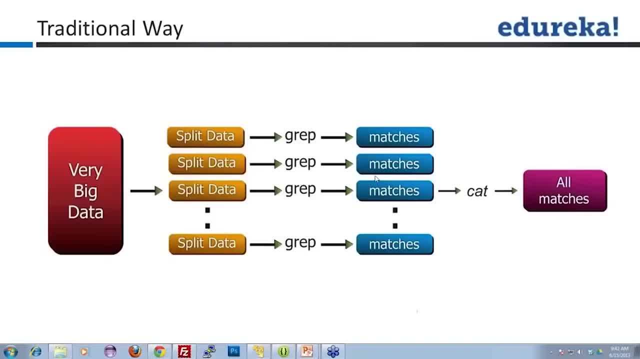 so, Dipankar, are you clear? why do we need MapReduce? now, Let's not go to. MapReduce is a MapReduce is a key value pair of programming which will be used to do this. is some definition, and then you, then you become some XYZ certified. 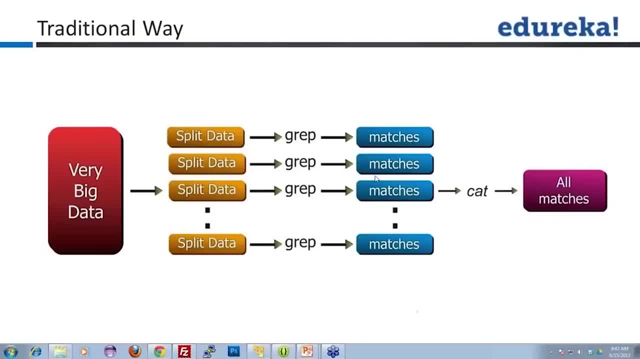 Hadoop developer. don't, don't just rely on that, ok, so let's. it's very important to you know where to use it and where not to use it. ok, So now can you tell me if the data set is small and if the files are small, ok, ok, let. 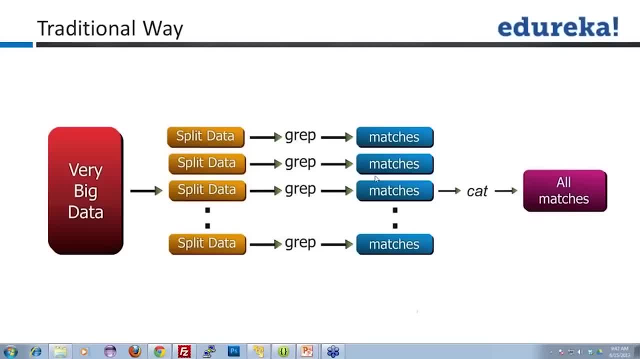 me ask that question Later. ok, not not the right time to ask that question as well. I'll ask you that question by the end of this class. ok, if I don't ask you this question, please remind me that you had to ask some question on file sizes. I'll ask you that and make that clear. ok, so let's. 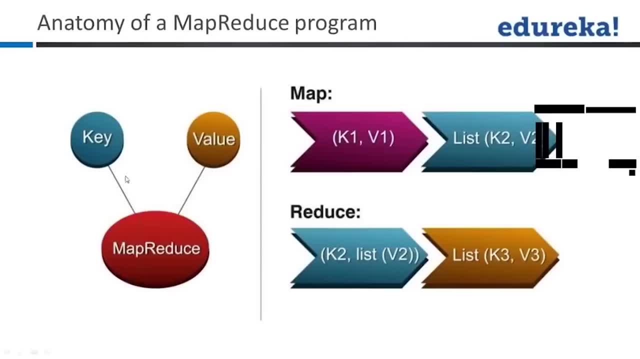 move ahead and let's see now. I have introduced the term MapReduce on this file, but I'll not talk about MapReduce. still, ok, I want to actually understand from all of you that did you, did you? I want to see what are the characteristics. 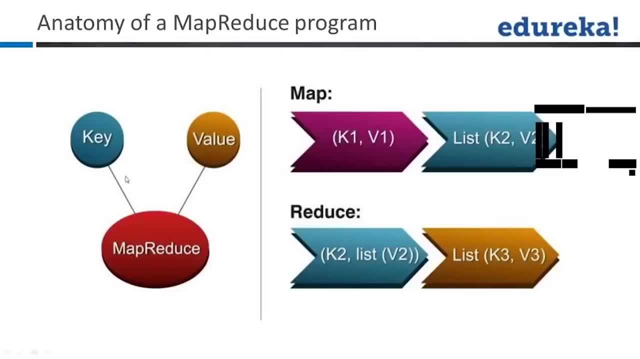 Of such data. ok, so before now, these are some equations which are written here. how many people, by looking at this slide, can understand what I'm talking about? just tell me yes or no. I mean, I says he understands, Rahul says no. anyone who understands yes, just tell me yes. 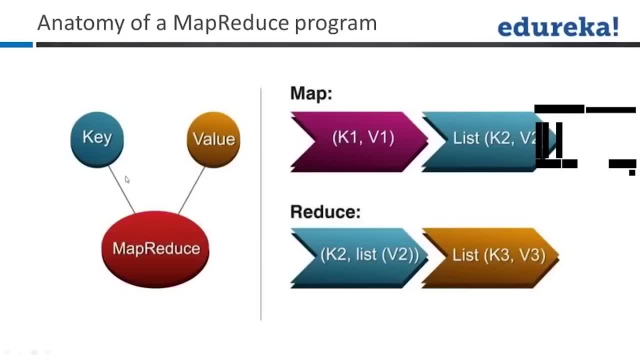 no, I know, I mean you will not understand. that's why you are here, right, such is the fifty percent key value. I understood hash map, hash table says. Vinod Parthaiwan says no, so anyone who and doesn't understand, no need to write anything. Vamsi says functional programming: ok, key value. 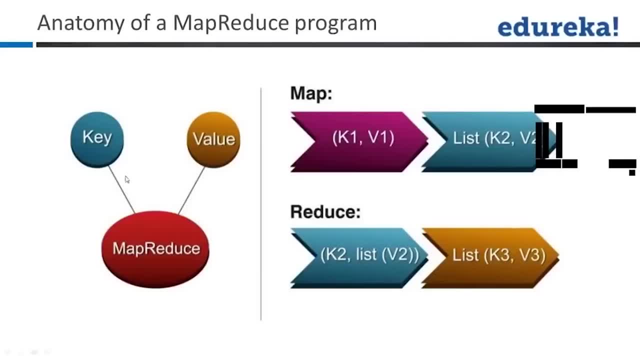 is the key for MapReduce. ok, Ashish says functional programming there. ok, now, guys, one thing which is very clear from the data set which we saw- and it will become much more clearer as we see more data sets- that what we were looking at are key values. ok, right, where key is the? 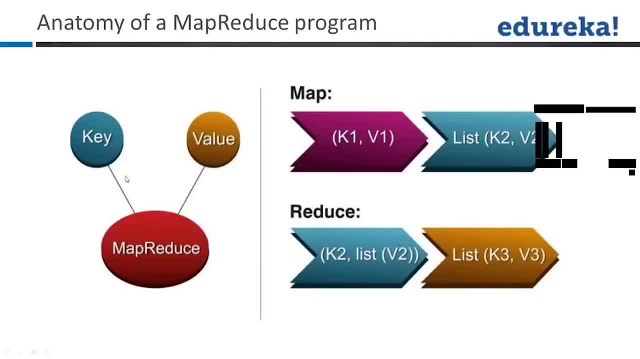 year and temperature is the value, and we need a programming model which can handle this very well. right so that that programming model is called MapReduce. but before we get to those terms jargon, Map and Reduce. don't have to worry about that. let me tell you what. 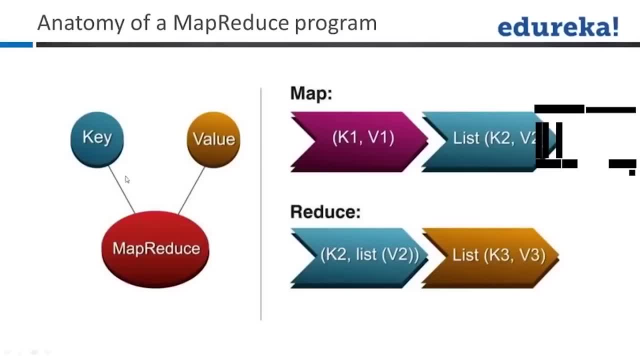 do we need to do first? now, the first thing which we need to do is extract key values from that data which we had right and create key value, key value, key value, which means that if, if some year comes some temperature comes Here temperature, here temperature, here temperature- that year may come multiple times the temperature. 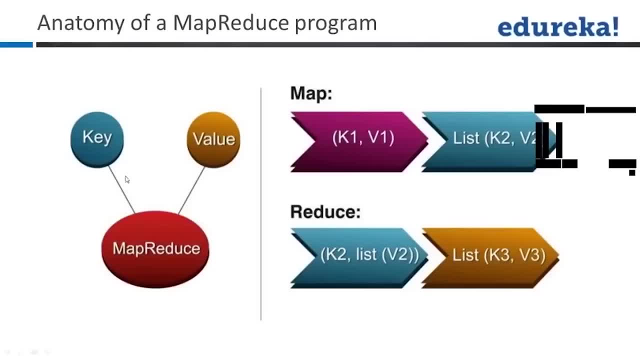 may come multiple times. so remove all the things which do not form, which are not required, from that data. come up with a key value pairs right, which is a, which is a key, and a value pair right here. k1, v1, right. do not worry if these equations are not making things very. 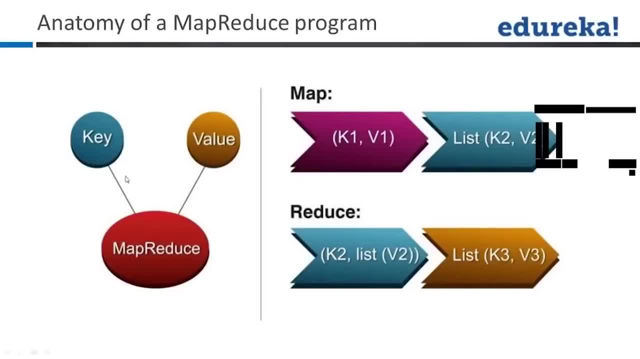 clear to you. I will just show you an example as well. let's try to understand with the equation, and then we will go to the example. right Now, next thing which we need to do is actually Do a sort yes, yes, we will. we will come see, we will go to that. we will exactly. yes, key. 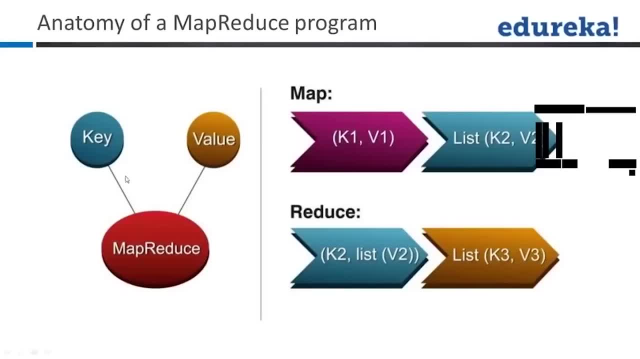 is always unique in nature. now let me tell you how are we going to proceed with this class. okay, now, right now, we will see this. then we will go back to our example which we saw. we will write a program, a MapReduce program, to actually take out those things. 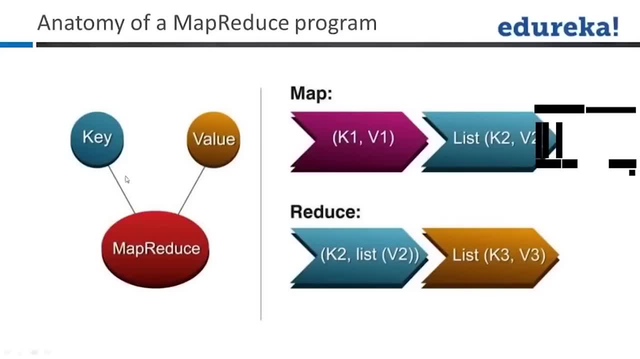 which we are, which we talked about. okay, Okay, so, okay, so is that clear guys? so just give me one second. I want you to actually look at this. I will explain. what is this list k2, v2, what is this k2 and list v2 and what? 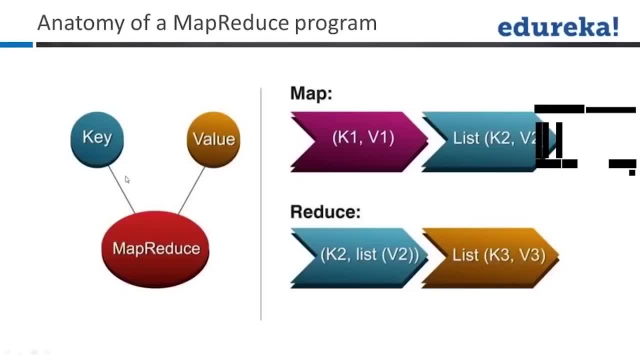 is list k3 v3. okay, so these are the four steps which we have, and I will. I will just explain it. I want you to actually just keep this termite, okay, Okay, so now. now let's look at that example once again, and then I will show you what is. 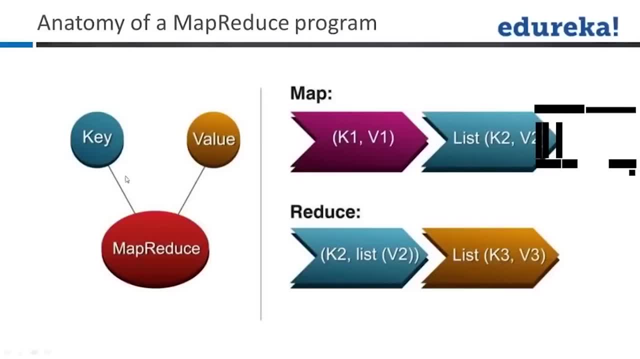 what? what are we actually going to do here and how? I will come back to this slide once again. okay, For now you can understand that initially, what we do from that data is extract key and value pairs. so these will be these key and value pairs. then what we are going to do is: 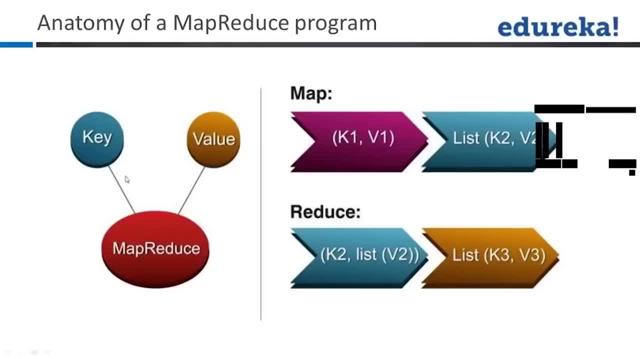 we are going to create a list, okay, which will have the key and the value list, okay, which will show me that, for each key, if there is a repetition of that value, we will get those values there. so that's what we are going to do next. okay, then we are basically based on: 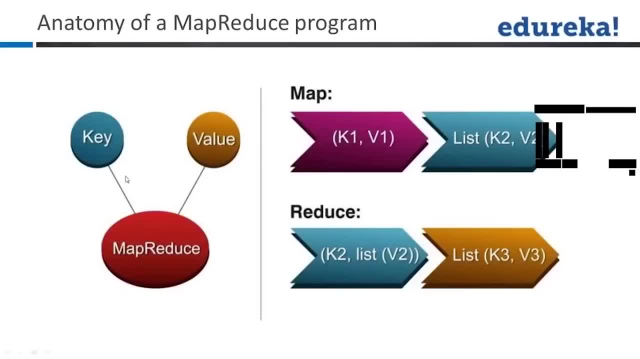 sorting and grouping them together. okay. Now, next thing which you are going to do is we will use a function which will do the actual thing which we want to do: if you want to do a match, if you want to do a sum, and those things we will do, and then, finally, we will come up with, again, a key value pair. okay, so, 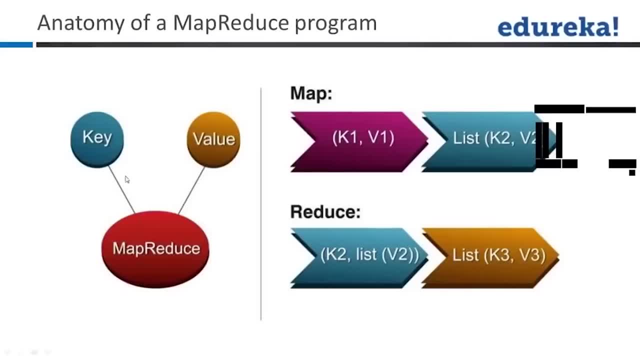 now. this is sum. okay, the bunker is asking question list. k2 v2 grouping is from key with in map. yes, so now. okay, now the bunker. that's a question which I am not answer going to answer now. I am just trying to confuse everyone right now. okay, so that they have this thing. 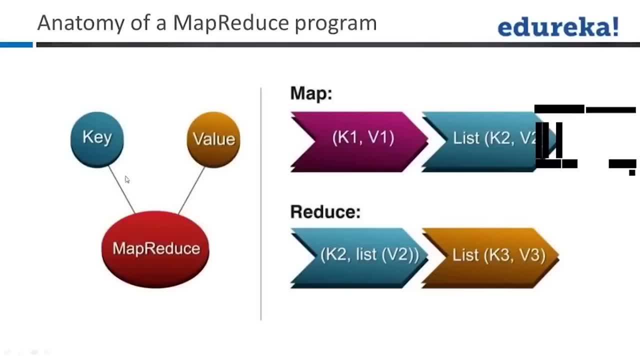 in their mind, because they will. this is something which they will have to see all the time. I want to them to become familiar with this term, so this is how it will be written in every book. I will explain with an example, so within 15-20 minutes, this will become crystal. 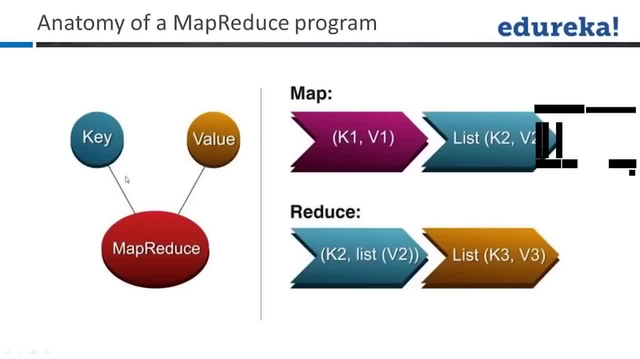 clear. okay, sometimes it is good to have chaos, okay. so now I will repeat this once again: what I am saying here Is that initially, we will extract key and value pairs- okay- from the list. key and value pairs- okay, may just understand. these are key and value pairs now we are going to create. 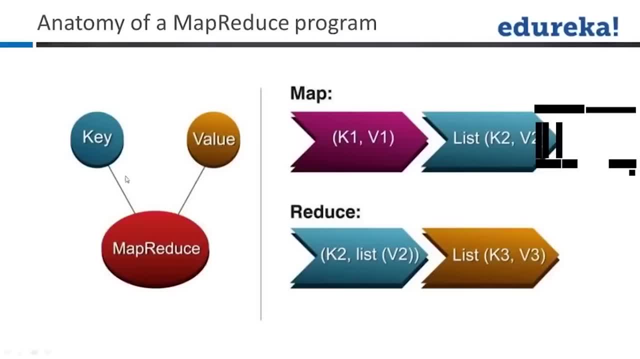 a list, a key and a list of values out of that so key and a list of values will be created out of that. okay, now, this will be done, obviously, by doing some kind of sorting and grouping from this key value pairs. okay, so that's the second thing which we do. then we will do. 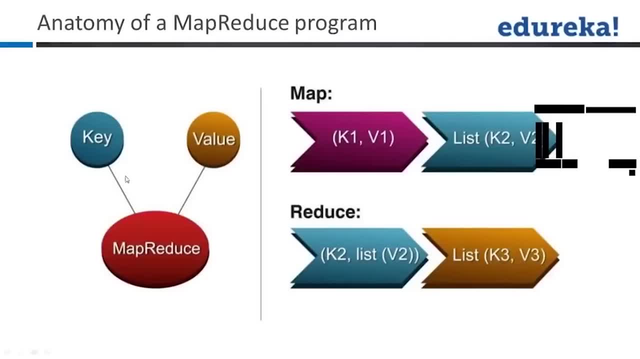 is, we will use this list, which was the key and a value list, and do some- just a minute, just a minute, mom see, it will be clear, okay, and then do some manipulation or some calculation on this thing to get another key value pairs. okay, now, when I am saying all this, it become: 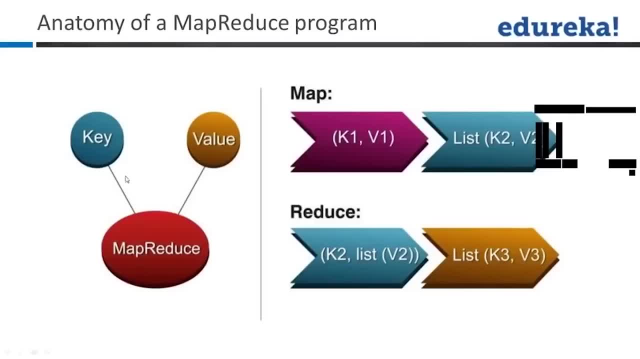 it doesn't. I know it is not clear to anyone, okay, but I still want you to remember these terms now as we move on to the next slide, then, as we look at the examples, it will become very clear. So let's move on. no need to stop here, Ashish. all those things will be answered here, okay? 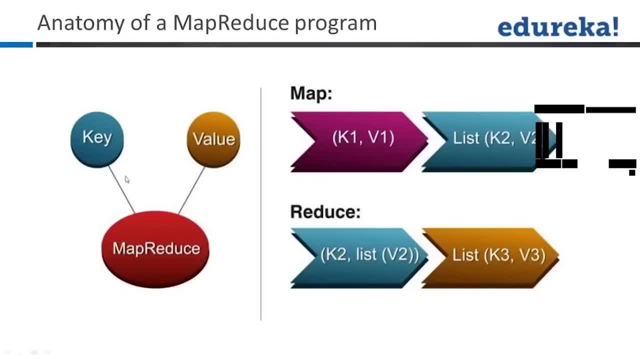 yes, so Sriram is saying: so say, I have this question I am going to answer. Sriram is saying: I have a location in each file and temperature for day in each file. key is location and temperature is value. right, that can be one of the key value, right? that's right. so this level of 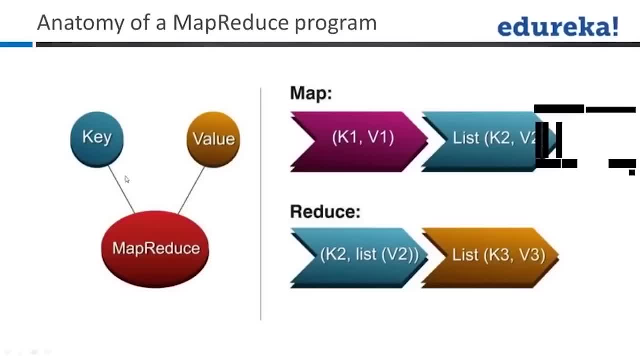 questions I am going to answer. I am not going to answer. output of map and input of reduce is different. I am not going to answer this question list k2 v2- grouping of the for a key within a mapper output. so all these questions I am going to answer a little later, okay, Dipankar. 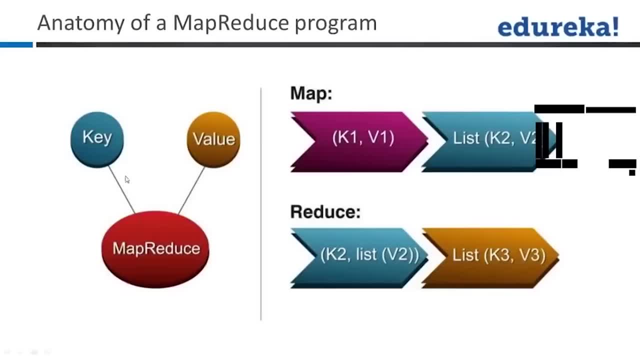 and Vamsi and Ashish, just give me some time. okay, how is going to split in this case is also something which I am just going to tell you, Ashish. okay, just give me two minutes. okay, let's move ahead. and there is one there. you will under very soon understand why I have. 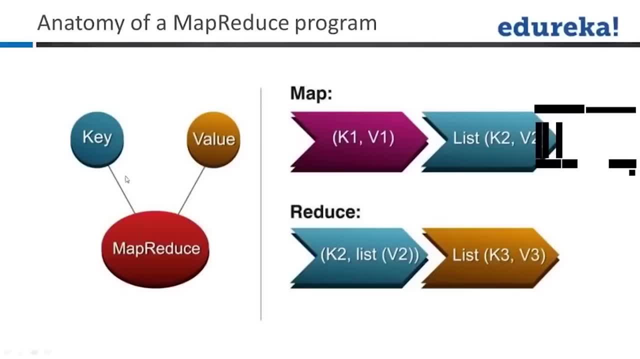 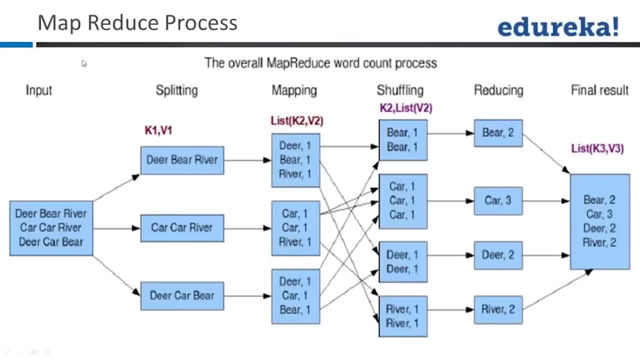 created all this confusion in your minds. okay, so very important to create chaos first and then figure out if it is clear or not. right, otherwise it will become very simple and you will go back thinking that you learned everything. okay, I don't want you to do that. okay, let's. 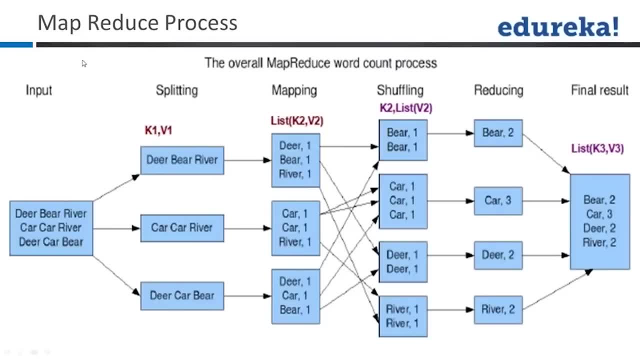 take this example now, it will become very clear. okay, So look at this example, guys. this is your input now. you remember I put this key value right. so this is the splitting. okay, so you have created all these. you have split those records that beer, beer, river, car car river, beer, car, river beer. okay, then, what you do? 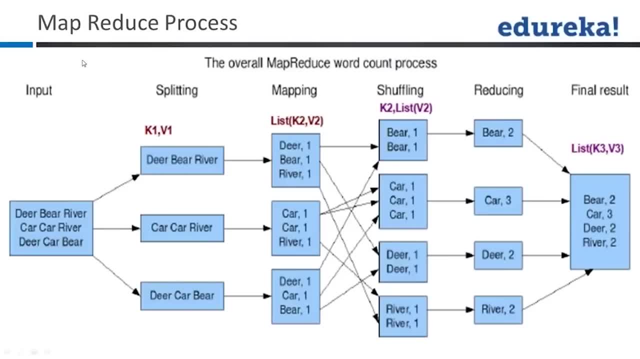 in this you say: beer come once, comes once. beer come once. river come once. okay, so this is that list of the mapping which you are talking about. don't worry about these terms which are there at the top. you will. these, Okay, These shuffling, reducing, finalize all these things. terminology will become, will become. 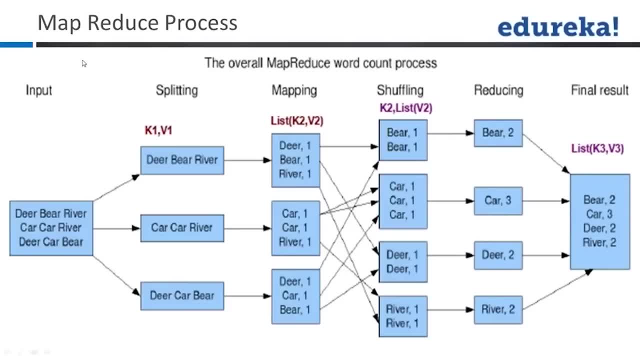 very clear very soon. okay, Now, what we do here is okay. so Ragu, Hadoop will do it. Hadoop will do the splitting. okay, you have to. you can configure how big split and all those things are possible, but Hadoop will do the splitting now, okay. so now does everyone understand this part? till now, everyone. 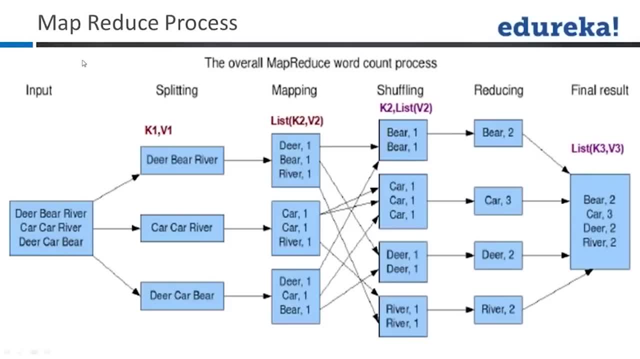 is clear what I am talking about. this list K2- V2- is clear to everyone. first, we created these key values here: K1, V1 values: yes, yes, yes, Avinash, okay, yeah, so now, okay. so Avinash Rajat is asking me Why every 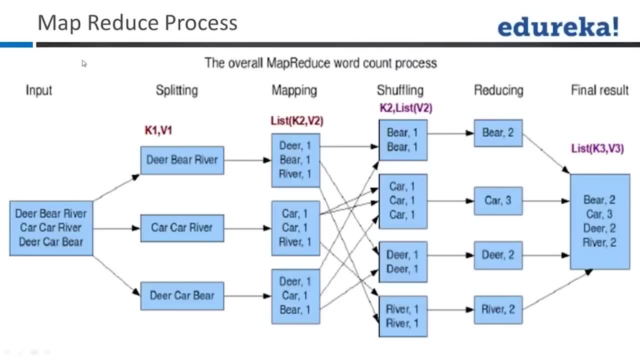 Why every? Why every, where value is one? okay, it is one because in this case, in this particular record, beer came once, beer came once, river came once. if it, if it was like beer, beer, beer, beer, beer and river, okay, then it will be twice here. is that clear guys? no, it will. yeah, so it will. 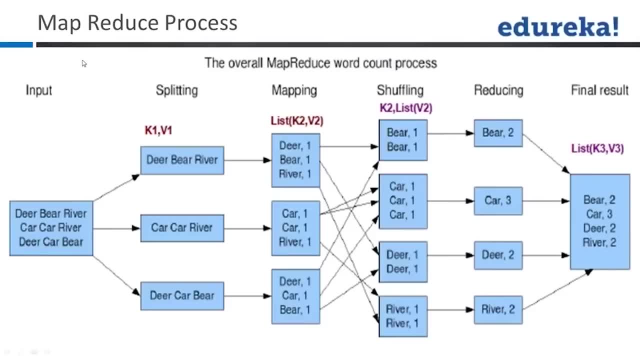 come twice, but not number two will not come here. okay, it will come like beer, one another, dear one, something like this: you look at this one, right, this example, can you see? yes, car is coming twice. yeah, so this is how it will be done. there is no calculation happening. 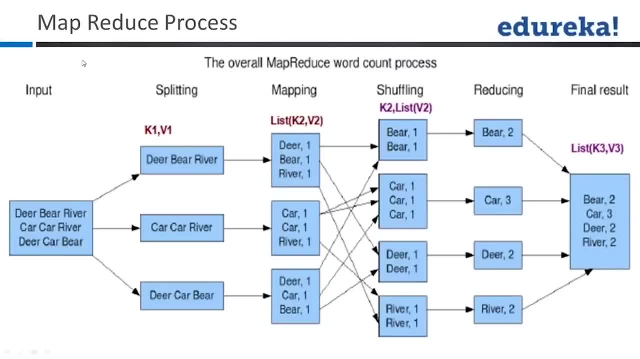 here. yeah, like car. okay, now the first thing which you do is you just thanks Ravi. thanks, Ravi says very concise diagram and clear diagram. honestly, very good. okay, yeah, Dhananjay, just wait on, wait, wait, wait, wait on, wait, wait, wait for some time. 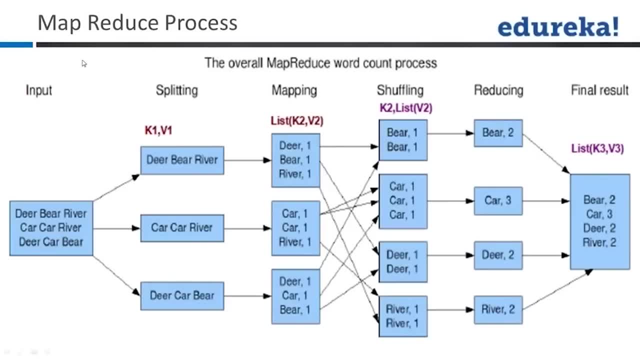 Okay, wait for some time. all these things will vary, become very. I have not reached that stage till now. okay, now there is the key, there is the value, right, so what we have done till now- okay, what we have done till now- is that beer is the key, one is the value, beer is the. 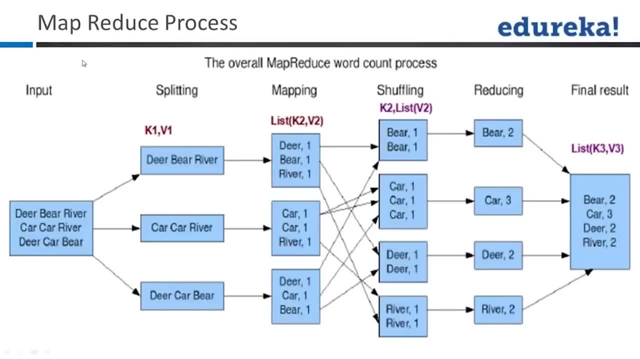 key one is the value. river is the key one is the value in this record. car is the key one is the value. another time car comes, I read once again: okay, right, and then we write beer, car beer, as Okay, now what we do. we do some. now, one thing which is important to do is it will be good. 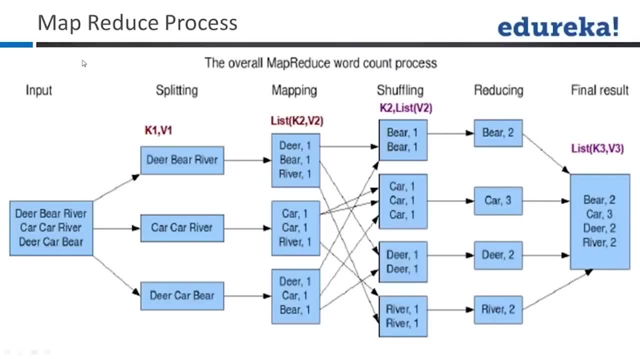 if we could do some shuffling and get these things like this. so wherever beer is coming, we will take all those records and put them together. okay, that is called shuffling, okay, obviously you call it shuffling only. okay, and you will group them together. okay, so you. 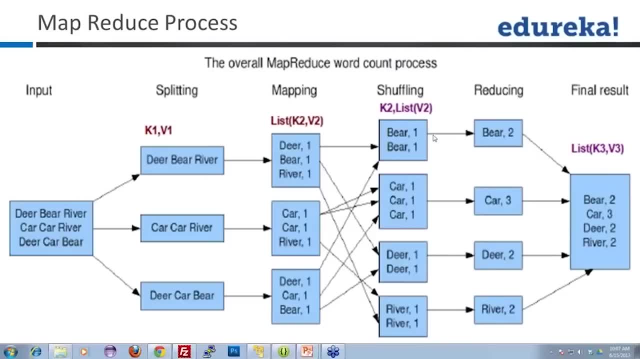 will have. now what you have is: you have beer, Beer, and that comes one one. you can look at it this way also. you can also write this as: let me just open a notepad. some people who already know MapReduce will ask me: why are you not writing it in the traditional way? so let me just quickly open notepad and show. 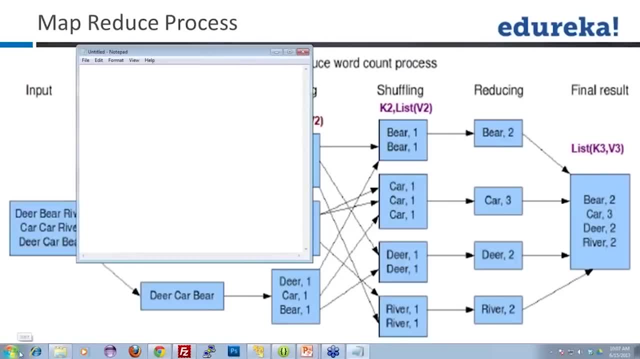 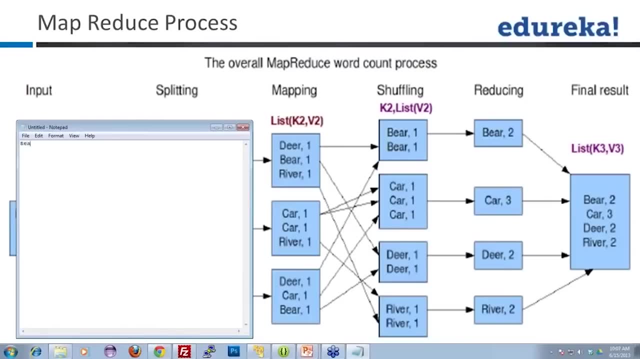 you how it will. also, it can also be represented. So it can also be represented as: Okay, forgive me for these parenthesis and brackets. okay, I am just taking a liberty here. okay, so this part which is written here can also be represented as this. okay, so this. 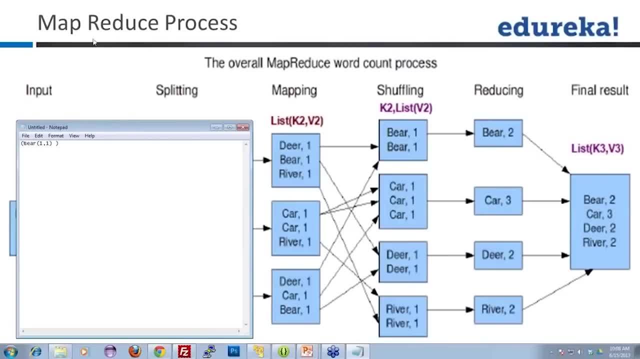 is grouping of similar items together and putting a value for those. exactly right. so that is what Vamsi has told me. this is what we will probably end up doing at this stage. okay, is that clear guys? Yes, Rajat, Hadoop does this for you. okay, I am now. I have not yet reached Hadoop, okay, so 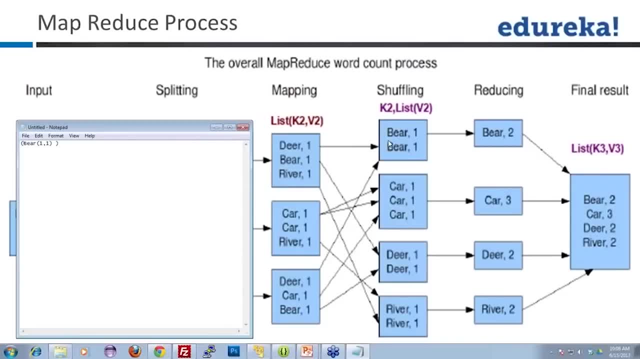 guys, I have not yet reached Hadoop, so please do not ask me questions on Hadoop till now. okay, I am just telling you a process which is slightly different than the earlier process, okay, which we used right, and then we will see how Hadoop is doing. that, okay, Rajat is. 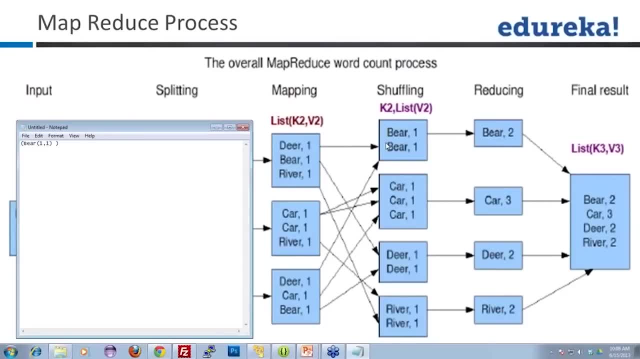 that. fine with you, Rajat, I mean Rajat Rastogi. okay, great, so now this is what we will get on this point. Okay, so for car. now Sachi is asking me a good question. I will write for car. so for car, I will write like this: okay, is that clear now everyone? okay for deer, it will be same. 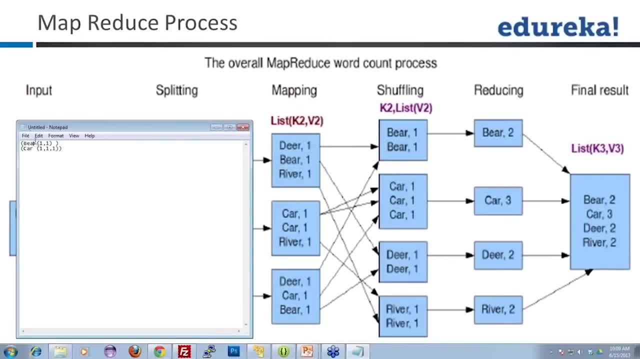 as deer, so any number of. so this is your. this is the thing which we talked about when we were on the last slide. let me go back to the last slide and see if things are the thing which was. This is looking very difficult mathematical kind of equation where I confused you whether 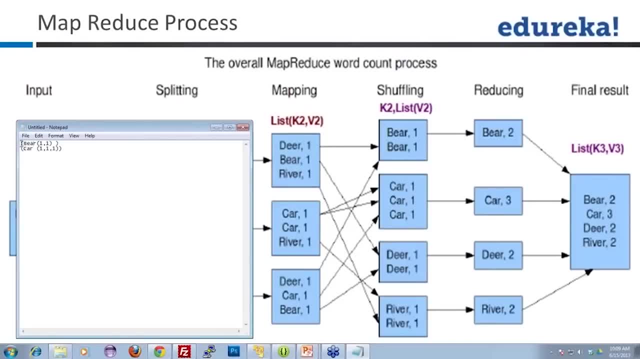 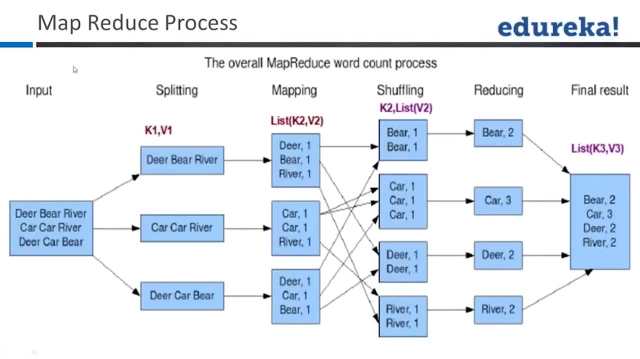 it is looking better now, or not? okay, shall I go back to the last slide, guys, if you don't mind, and I will come back to this one once again. let us see if we have understood something on the lab. Ashish. I will not answer that question right now, okay? Ashish is asking: why have we? 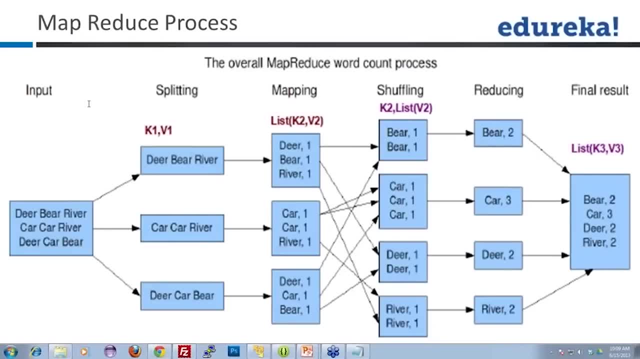 not done reducing in the mapping phase. does anyone want to know this answer? now? everyone is saying no and some people are giving you a big no also, Ashish. okay, so just, unfortunately, this is there is a group of people. okay, so I will have to respect. okay, yeah, so don't. 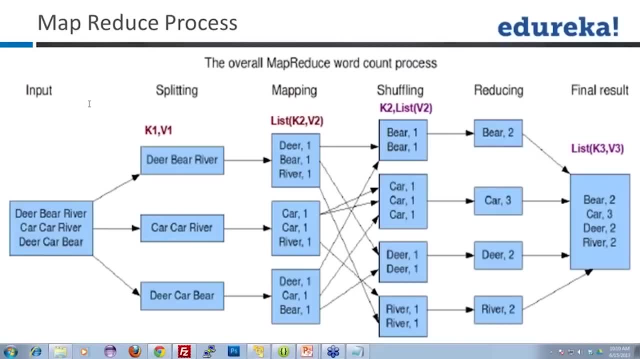 worry, Ashish, but I assure you this will be answered today only. okay. is that fine, Ashish? not now. I have not got answer from Ashish on that. okay, thanks, Ashish has given me a smiley, so thank you, guys, and you have all the right to stop me from diverting from the 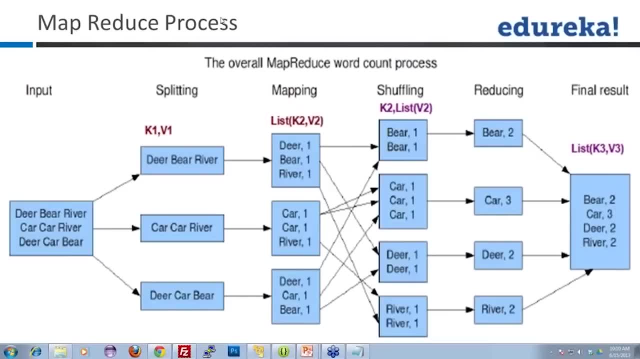 topic okay. Okay, now we have a lot of questions. let me read through those questions and I will see whatever I want to answer now. okay, so Dipankar says: because value of same key may be in different split. right, that is very much possible and that is why we have done this shuffling here. 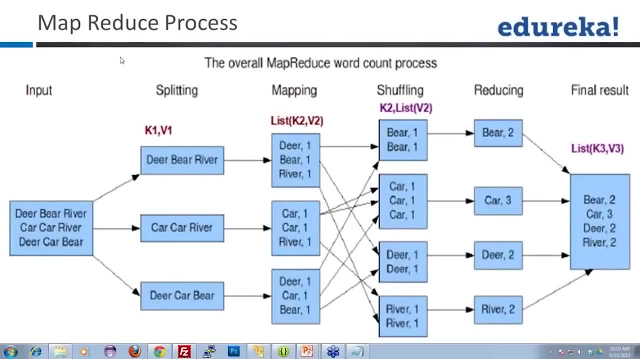 right. no, don't worry about Java list or not. this is not a Java list. this is just a representation here, Ramesh, where we say that this is a list of. This is a list of K2 and V2. so here is the list, right? K2 and V2 are the. so Ramesh is asking: 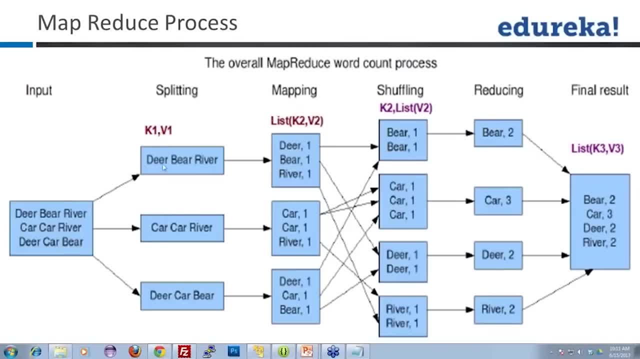 me. I did not understand list K2 V2, which means he did not answer. now, these are key values. that is clear to everyone. this is a list of key values. this is also clear to everyone, right, right, and if I represent this part as what I showed on notepad, then this is a. 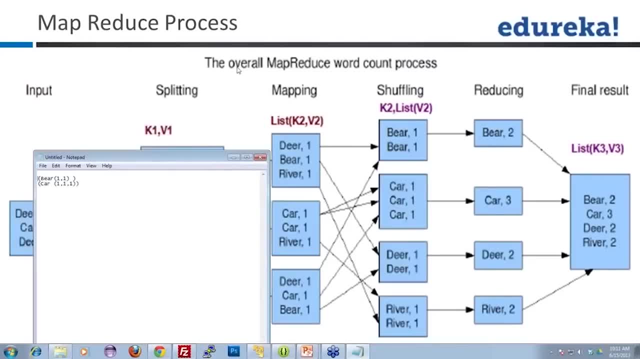 key and a list isn't it? is that clear to everyone? Yeah, sorry, Vamsi, actually it is written as bear and I pronounce it as beer because that's what I like better. okay, so Vamsi is asking me. he is trying to pull my leg as well. he. 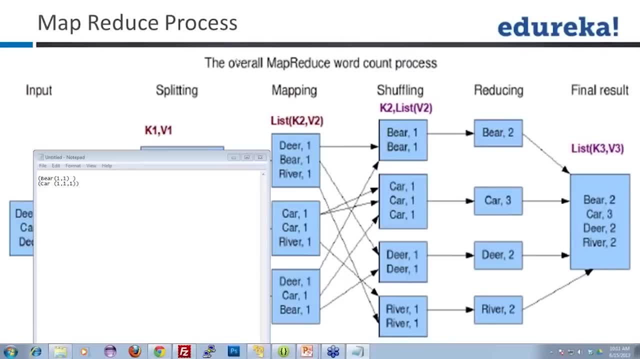 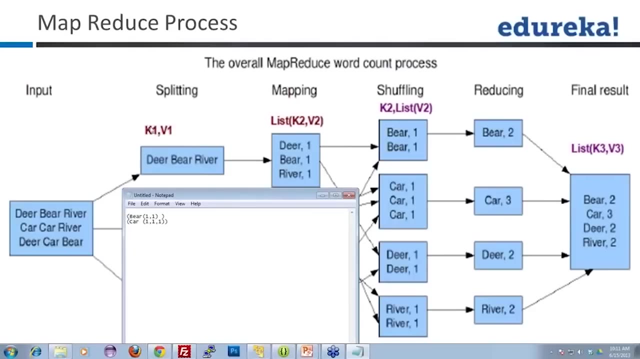 is trying to ask me: is it a beer or a bear? so it's a bear, but I like beer better. so, okay, okay, okay. now let me explain you what are these terms. okay, Now, everyone knows that this part which I have written here is a key and a value. these 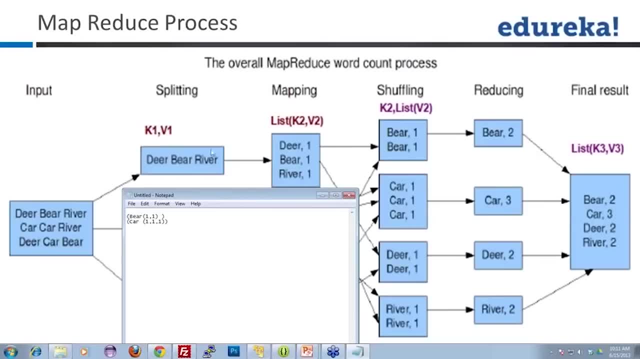 are key and values. right, these are simple values. there is no list associated here. right, this is just a. this is just a record, which is: there is no list. everyone yes or no? quickly, okay, great, now let us come to this. now is this a list? Vamsi, you can represent anything. 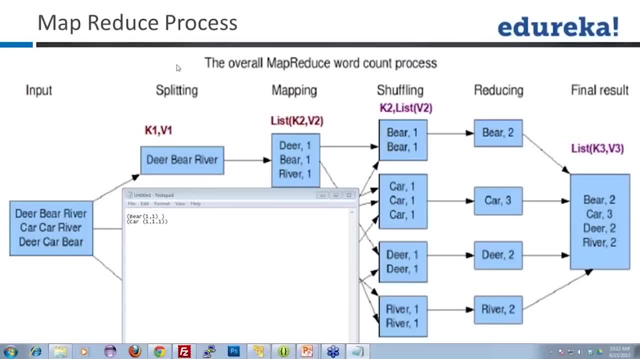 as key and anything as value. I don't mind that, Okay. Okay, you can. you can say anything as key, anything as value these are. if this is a key, these can be values also. who knows right, it's only after doing something which we will come. 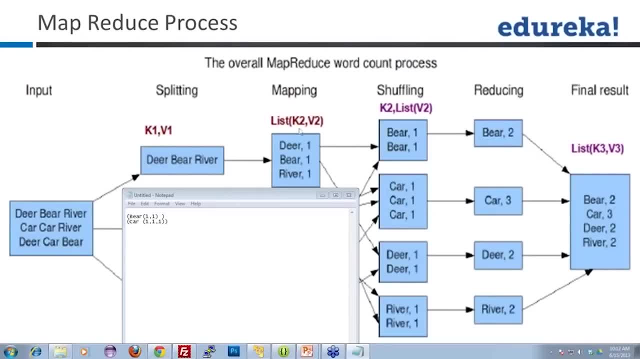 to know. but right now, look at it as a single record which has some values. okay, now, this is a list- everyone understands that- which have key and a value. yes, from that context, Vamsi, that was not a key and value pair, right, fine. but this is a list everyone agrees when. 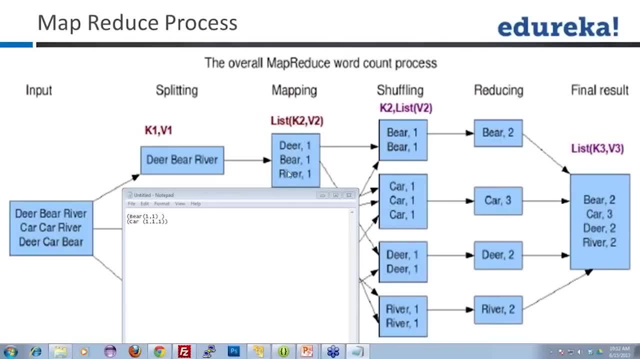 I say list of key and values, right? So deer bear river beer, right. so this is a list. everyone agrees to that. now, when I say that this is a key and a list of values, this picture may not represent that very well, right? so that's why I have written this. 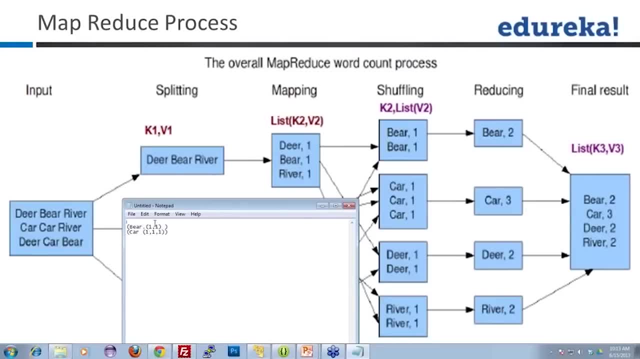 So this is where I say k2.. And list V2: is that clear? everyone has got it now. the reason why I opened notepad, I could have done it here also. great, right, So this is a list V2 now. great, So everyone is saying more clear now, thank you. thank you, Rajat. okay, Philip is also giving. 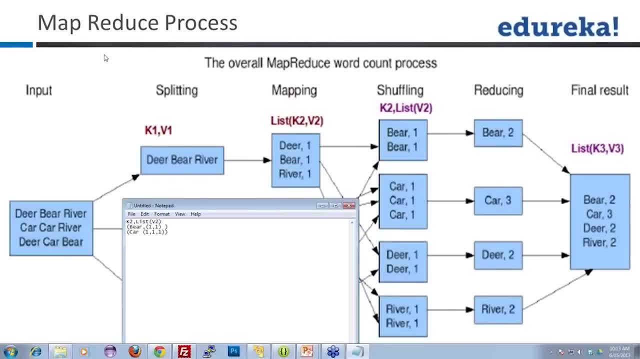 me a smiley. I think even in the slides also it can be represented as, yes, it can be, but it can be represented there. But what happens is Then people will not understand this process of shuffling right, so there can be one more thing. then it will add some people asking: what is this process called? okay, 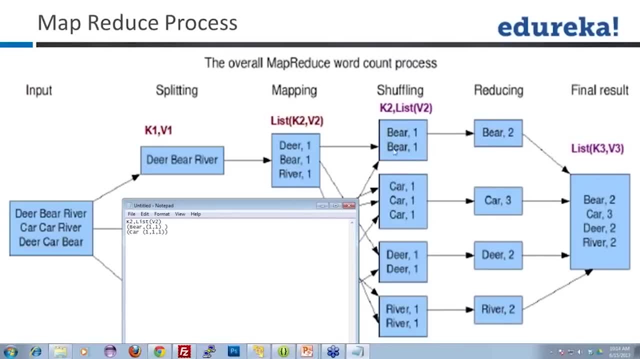 So in the slide. I think this is okay because we want to actually put them together right, and I will use this notepad to tell you that. how is this a list value? yes, Tushar, what you are saying is right, it is. it is not really list. no, Tushar, what you are saying is not. 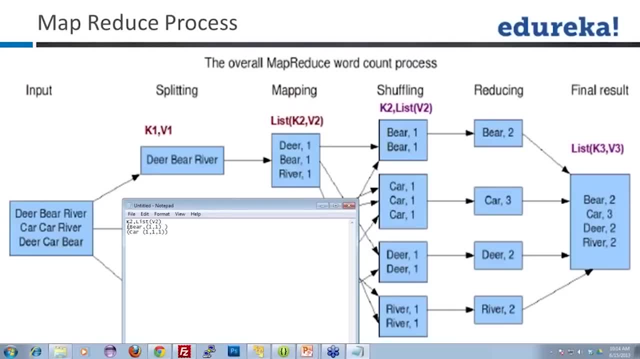 right, because this is not really a list. Now it is. when I write it this way, it is not a list, right? this is one part. this is another part. okay, and say a river, and do not quote me whether I am using the correct values or not. 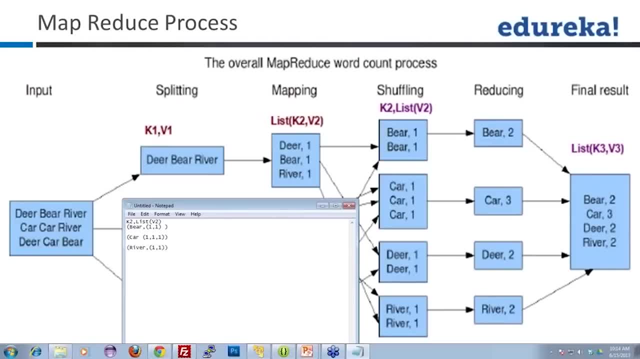 So if river comes here, then this is another part. So basically this is not Now. So Tushar is asking me: is this a list? this is what Tushar is asking me. okay, thanks. Parthevan says author explanation for MapReduce process. okay. 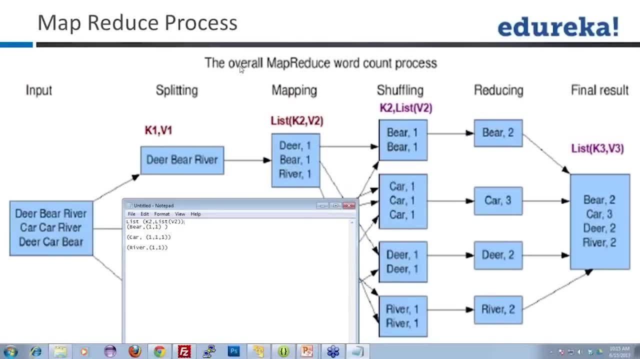 So before Parthevan. thank you very much. I really appreciate your words here, but just give me five minutes. I want to make sure that everyone is understood it right. So great. So now, this is not really this. Be careful, Because this list will not be there. these will be only this part, okay. 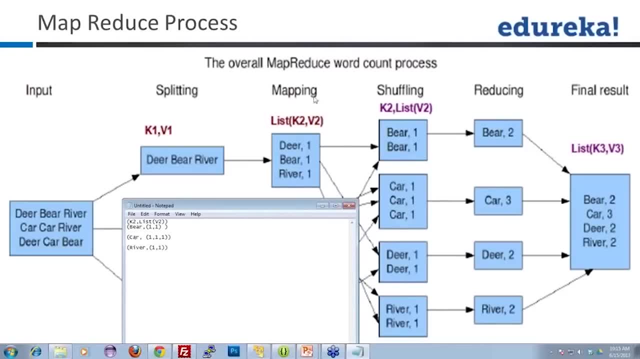 So we will have these as separate things, okay. Now, when we get to the next process, what you wanted to do, we wanted to do: how many bears were there? okay, Now, I also wanted to count how many cars were there. okay, So, what I do, I will take this part, okay, and use a transformation here, that transformation. 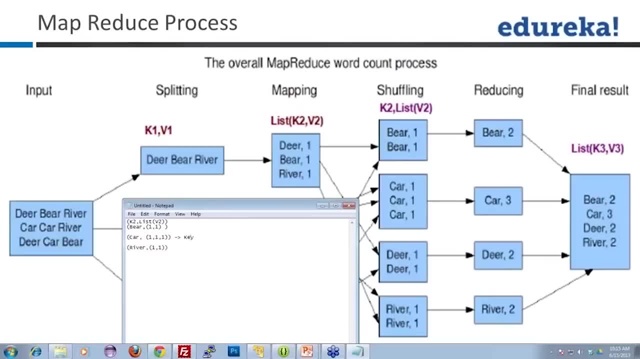 could be key. Okay, So what I am going to do is I am going to take this key some function on this value list, right, is that clear to everyone guys? So now this function could be a max function. this function could be a summation function. 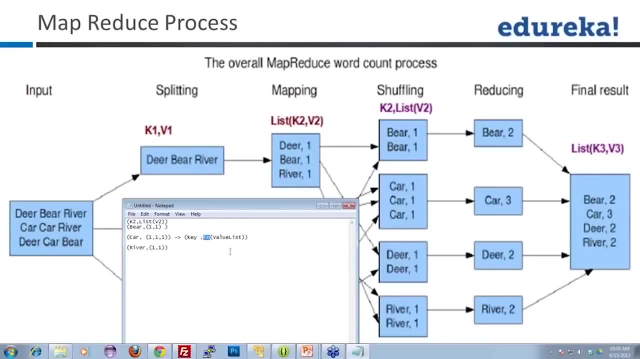 or whatever. this is the process which I will, where I will do the actual work, right? okay, and this is this is where I will find. if this is summation, then I will find out this here. Okay, Is that clear guys? Everyone is clear up to this point. 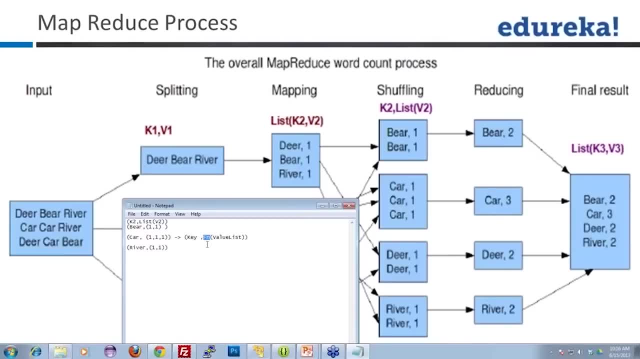 This function which I have highlighted here. Can I get a round of smileys? if everyone is happy with this explanation, Okay, Great. Is there anyone who has not understood it? Because, see, I will tell you one thing: there will be many people who would have actually, 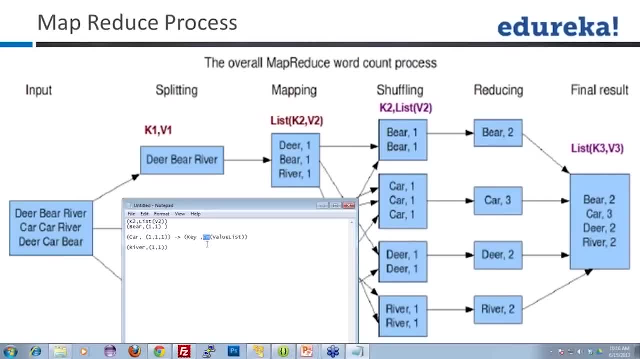 looked at MapReduce, they would have looked at YouTube videos, they would have tried everything, still they would not be very keen, They would not be very clear. So I want you to be very clear about after this class everyone should be very clear about. 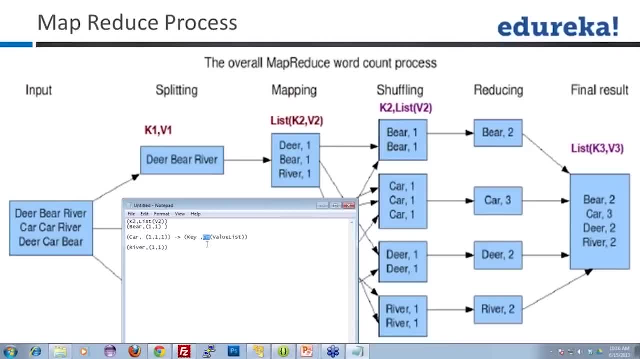 this right. Yes, in this context, Sushar, it is sum, the function is sum, it could be max, it could be anything. when you may write any function on earth here which can be, which can do something with this value list, Okay, And finally create what out of this function value list, what will you get? 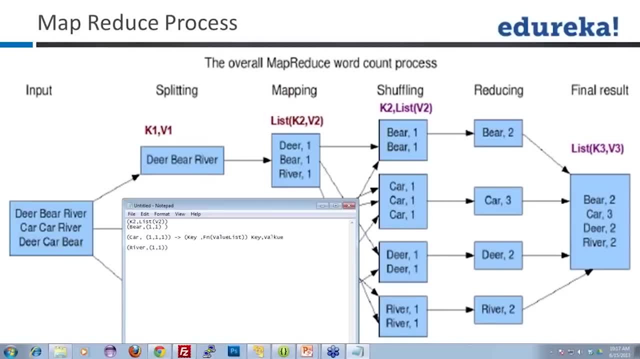 You will get again a key and a value, right. if it is a max, you will get the max value here. If it is a sum, you will get the sum. If it is a mean, you will get the mean, right? Is it clear everyone? 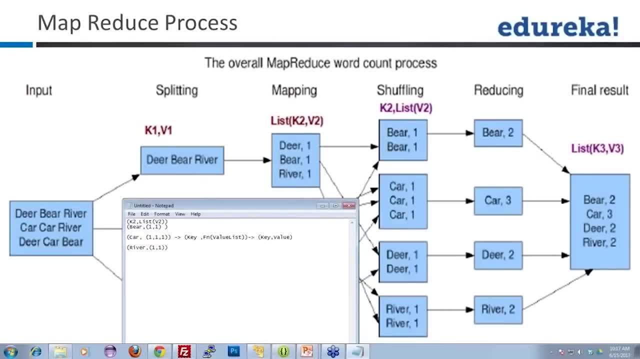 So this will be the output of this process. Okay, And then, finally, what we are going to do is create this, which will be the list. this will be the final list. This will be a list of these K3s and V3s, right? 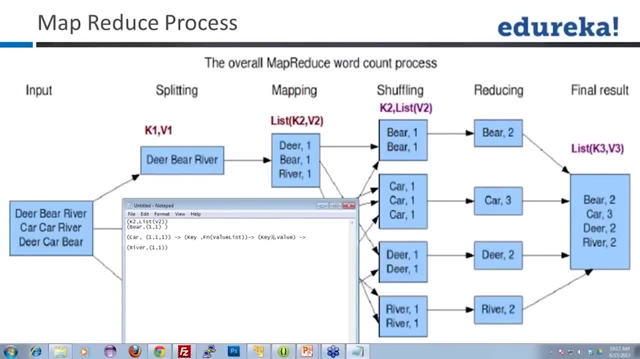 So this is K3 and V3, right? So let me write those numbers here- K3 and V3. And let me write. So let me write this K2 and list V2 so that everything becomes very clear to everyone. and let me write, just before this, where we started. 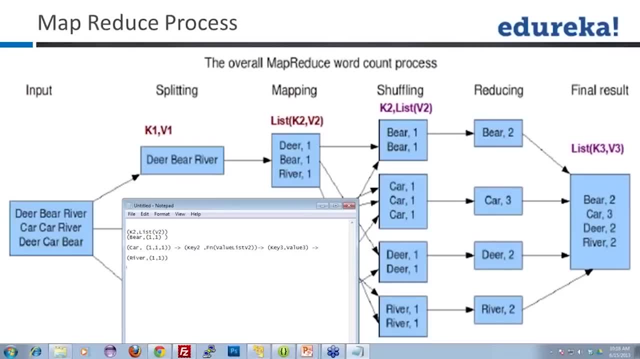 So we started with what We started with K1, V1, then we went on to create a list of K2, V2, right. Then we went on to create K2 and list of V2, and then we wrote a function here. finally, we got this: 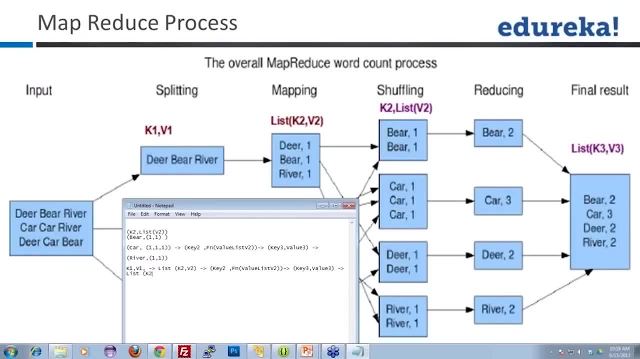 And then we got a list: K3 V3.. Is this process clear to everyone? Anyone in this class who is not very clear about this process quickly tell me. If everyone is clear, I can get a quick round of smileys for this. Pankaj, you were telling me okay. 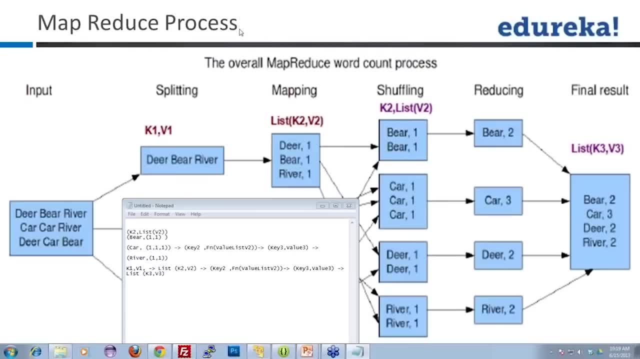 Okay, Sachi is telling me: let me fill gasoline for your Lamborghini, Buy a smiley. Thanks, Sachi. Thank you very much. I hope that Edureka gives me enough money to buy a Maruti 800.. I don't dream about Lamborghini. 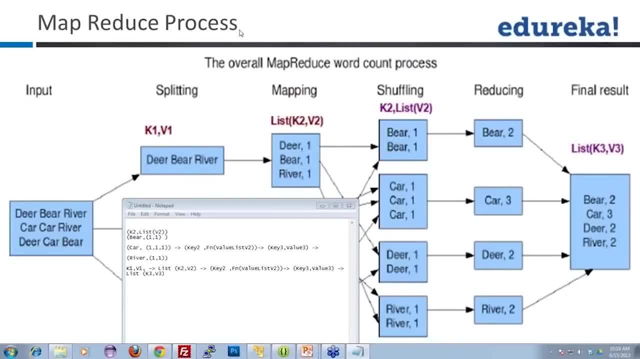 Okay, I am a very poor guy. I was a failure in college and I have a failure still in my life. Okay, And old as well. So Lamborghini is something which I don't dream anymore. Okay, Great. So thank you very much. 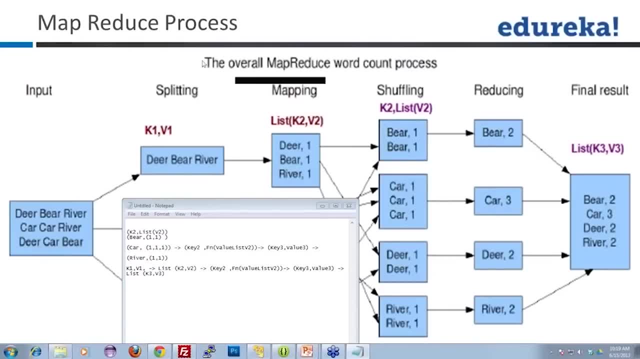 Okay. So Dipankar is saying: I will contribute. Okay. So Vamsi is telling me: then you are the next guy likes you. Don't do that, Vamsi, to me, man. Okay So, guys, Okay. 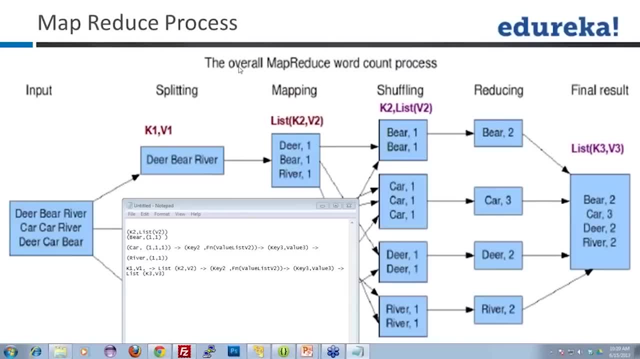 Now let's come back to this. Thanks for all the comments. Okay, I have already contributed by 50,000.. Okay, So I am going to give you a discount. Okay, Thank you, Thank you, Thank you. 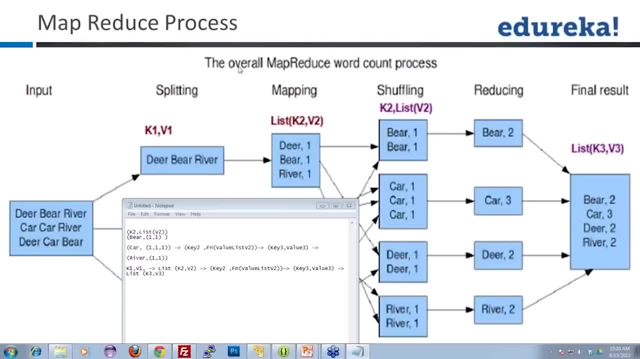 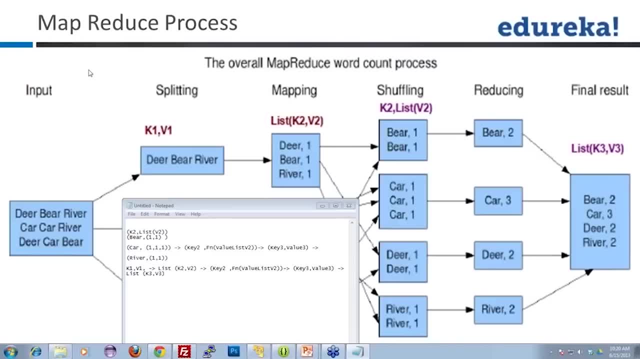 I am. I am really thankful to Avinash for paying that huge amount of fees which you have paid for this class. Okay, My children will be really thankful to you throughout their ages because this is because of your fees That then get some. какую était c御 какая? 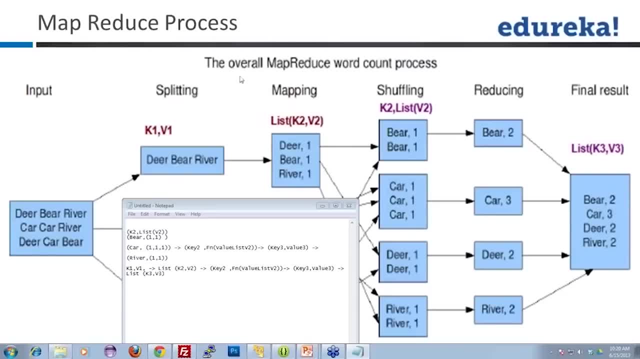 Thank you very much. Thank you very much to everyone who has paid fees for this class. Okay, And I hope that Edureka pays me a part of that. Okay, coming back to this now. everyone has understood this part. okay, yes, I am getting lot of. 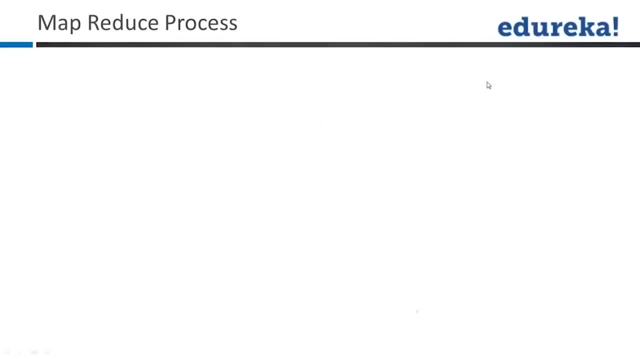 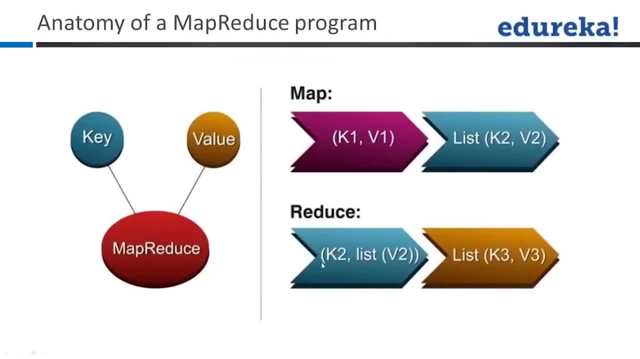 yeses. now let us go back to the previous slide, where all of you got confused. yeah, so is it making sense now, guys, whatever I showed you here quickly: yes, everyone has understood what is MapReduce. okay, so everyone is saying it is. this slide is clear now. so 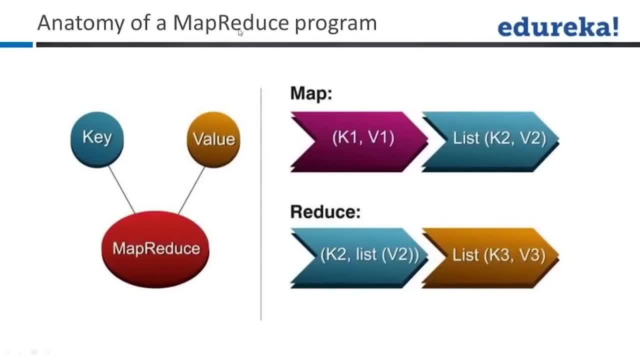 now. do you think it was a good idea to create that chaos in your mind then, to make sure that you don't understand anything, and then you understand Avinash? okay, any formal definition. can you put in one line? any formal definition? I know you don't like definitions. 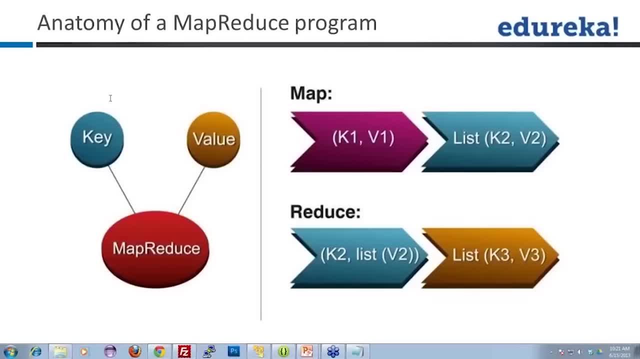 chaos theory pattern in randomness. I will let my friend, Rajat Rajat, who is a PMP, give me a definition for this. I don't know any definition here so, frankly speaking, I have never understood these definitions I have, so I will not be able to give you. 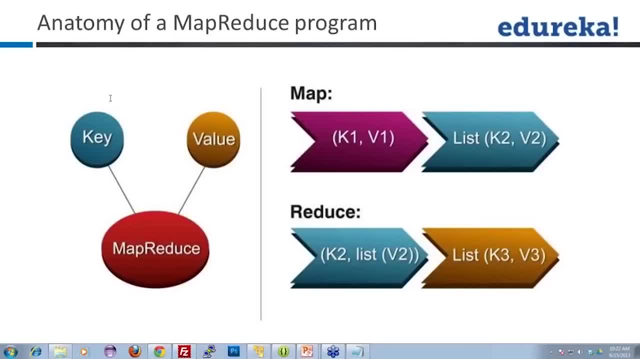 a definition. I have explained it to you, right. why do you need a definition? if someone asks you in an interview, define MapReduce, tell them that I am not going to define it. I will go to show you what it is. ask them the definition. okay, no one is going to define. 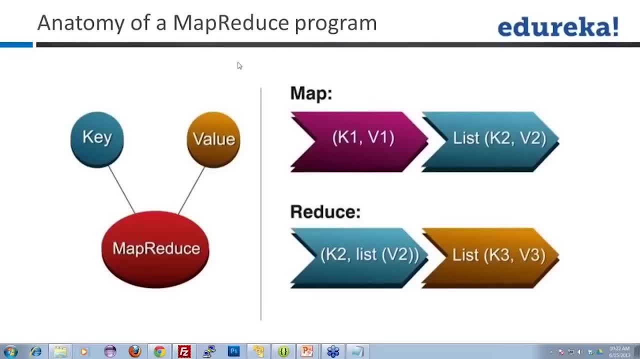 you that, Vamsi, don't worry, I will send you no. no, I know so in the interview you can explain this. I will send you a formal definition also. okay, I know, I know in interviews you will. 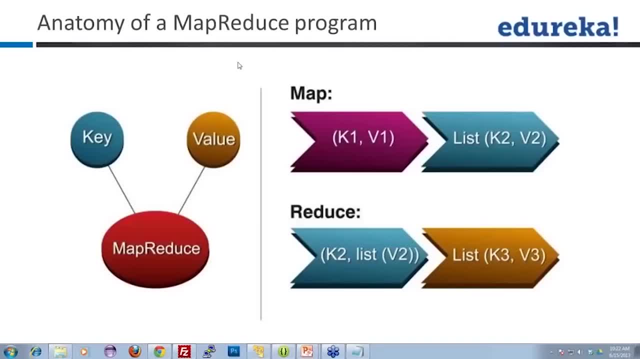 be asked such crap questions. define MapReduce: okay, okay, so Rajat is giving me the answer: combination of two words: Map and Reduce. okay yeah, that's the PMP definition of a manager for MapReduce, and that's really true, right? I mean, it's a, it's a combination of Map and 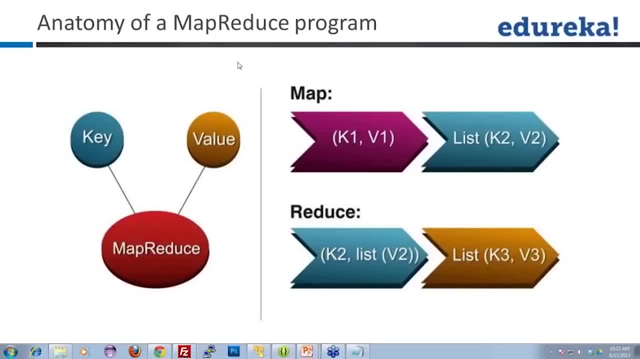 Reduce. okay, Now what is Map and MapReduce? get to the definition there. then they will ask you what? okay, Dilip has given a given. very good, Dilip, my friend has helped you. you should say thank to Dilip and you can be angry at me. Dilip said it is a programming model and 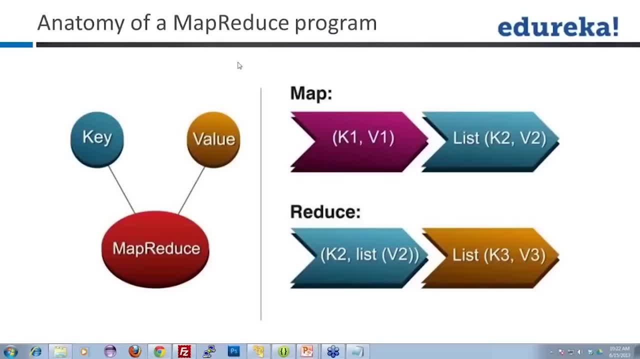 process for processing large data sets on cluster computers, great clusters of computers. The Pankhurst is determining logical unit of data, grouping them together and performing some operation on it. okay, guys, is that clear? is this? is this the Pank? let's. 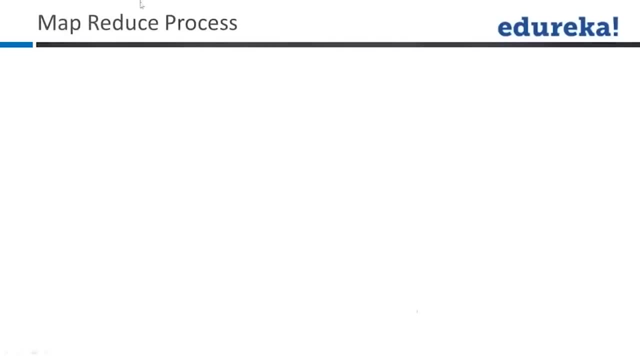 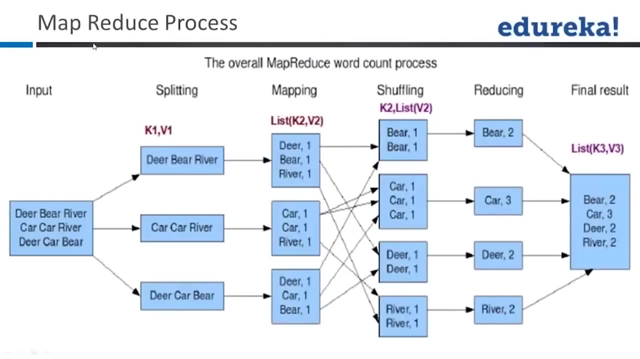 let's go back to our example slide and see: is this what we were doing? Thank you, the Pankhurst, for that definition. so the Pankhurst says: Vamsi, you can note down this definition. okay, I can also copy and paste and send it to you. okay, determining. 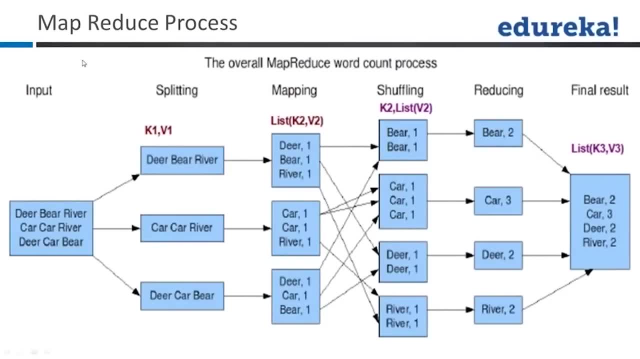 logical unit of data, grouping them together and performing some operation on it, that is, Map and Reduce in probably three sentences with two conjunctions okay, and a comma okay, and finally two dots after it, okay. so that's the definition. okay, so so is. 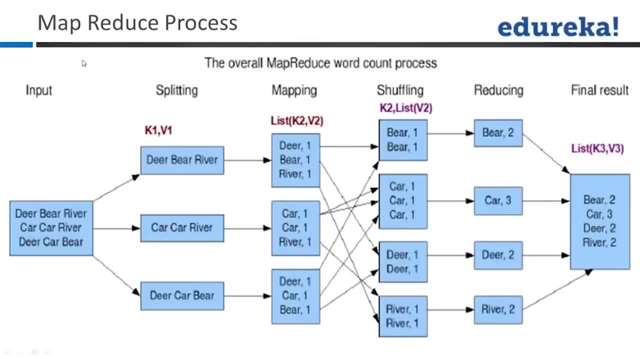 this what we are doing: Determining logical units of data. Okay, Okay, Thank you, the Pankhurst I will. Rahul is telling I will remember this only by car river and beer, and hopefully with beer as well. Ramesh Chaudhary is saying I it remembers me of three idiot movie where 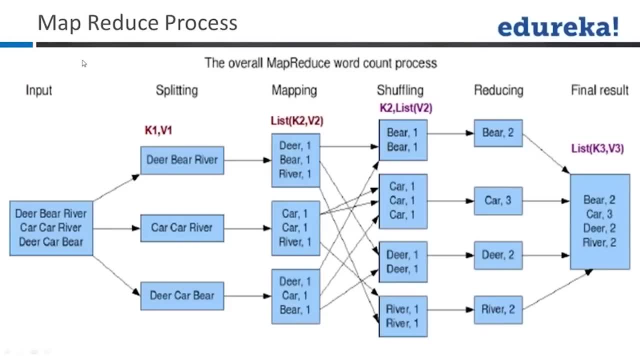 Ramesh Chaudhary is asking about definition in class. yeah, definition in class is very difficult one, so someone came to our rescue. The Pankhurst is laughing. okay, I will remember. my beer is what Avinash is telling me. the. 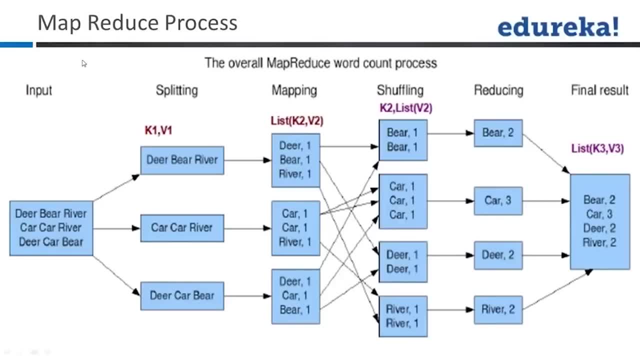 Pankhurst is okay. so, guys, now everyone understands, I know. see, I will tell you one thing. none of us have come here to study. we have come here to get entertained, okay? so whenever I get to studies, you start talking about beer and Katrina and all these things. 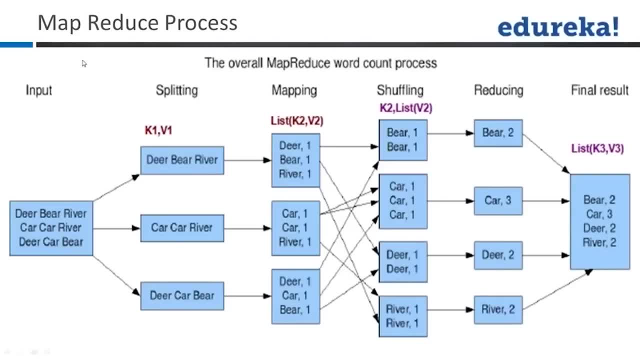 and then people blame me that you are okay. yeah, Vinay, that's what I am saying here. Vinay, I am really sorry about that. okay, let's come Now. we understand this. okay, Vinay, I am really sorry about that. I don't want to get. 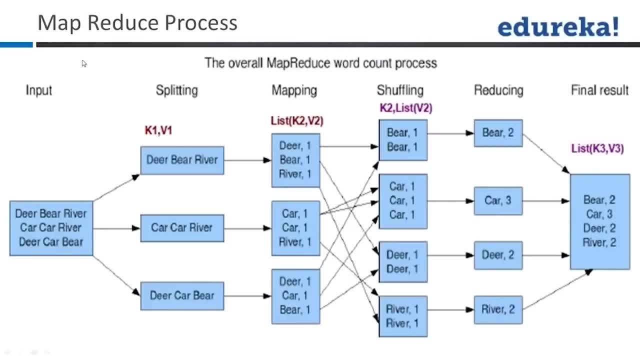 into all this right now. so let's come back to the point. and Vinay is telling you: please come to the point and don't waste my time, okay. so yes, Vinay, I am really sorry about that, so let's get back to the work. so now we have understood this MapReduce. Vinay has 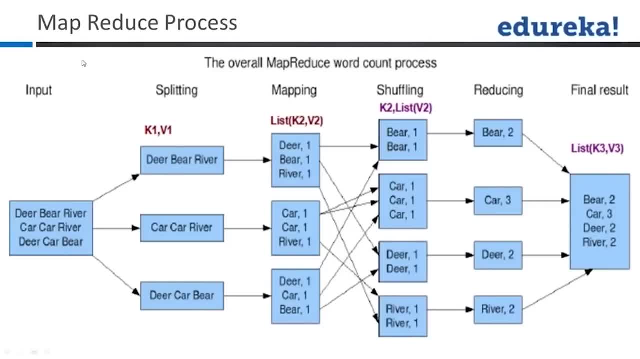 given me a smiley, so he was not all that angry. he was probably telling you guys that, come to the point, and he was agreeing with me because I was also telling the same thing. okay, so Vamsi is telling, but honestly, I wanted the definition to tell my mind about the whole. 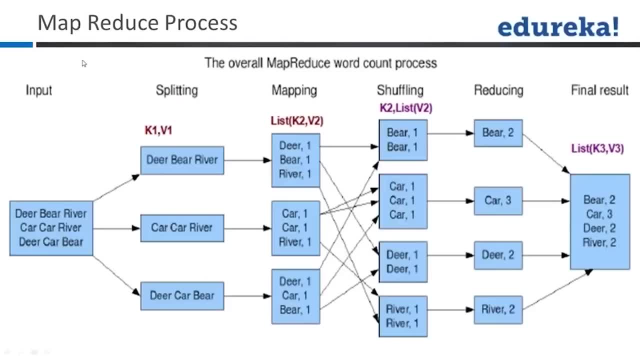 process in one liner. so I will repeat that definition once again, and you should say thanks to our friend Dipankar about it. okay, where he said- I don't remember that- okay, determining logical unit of data, grouping them together and performing some operation on it. Dipankar. 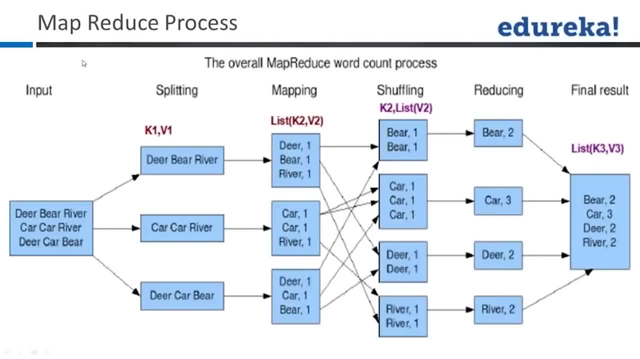 Vishwas. okay, So Rajat has given me another definition. Okay, And Vamsi is saying thank you to Dipankar. Dipankar, Rajat is saying: MapReduce is a programming model that's well suits for data set, where only one write and multiple read and to pass. 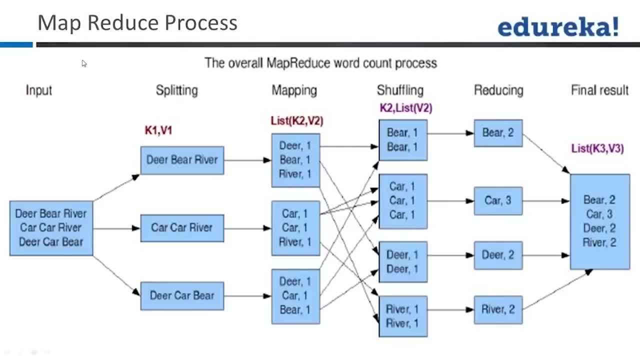 data to arrive at same conclusion. very good, Rajat. I think that's a very good definition, and the reason why I say that a very good definition- because that's where we started with in our first class- that this is for streaming data access, which means you write. 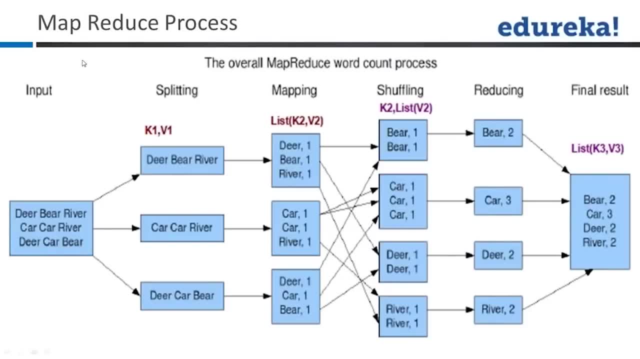 it once and you have to read things and pass them multiple times to arrive, right, great, so thank you very much, guys. So now I think all of us are contributing well here. Vinay, I am sure you like these two definitions, and this makes the whole process much clearer. right, and you don't think that? 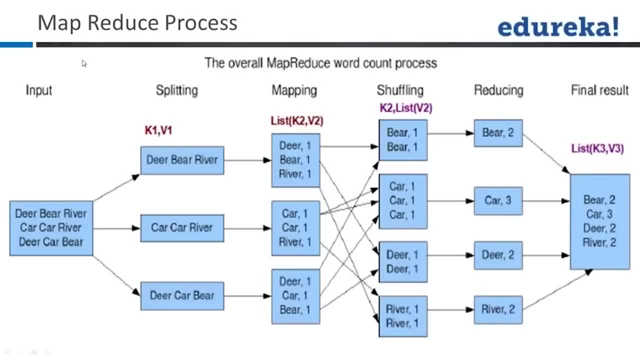 we have wasted a lot of time. we have just reached one and a half hours, well, out of which we have had fun for half an hour. okay, so not too bad, right, okay, okay, so let's go okay. thank you, Vinay. thank you for the smileys. 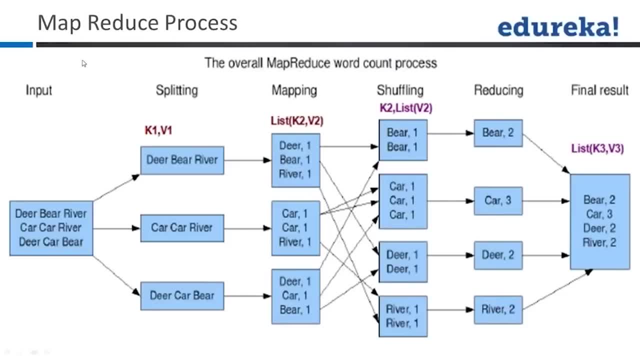 So now everyone knows what MapReduce is. anyone in the class or in the world who doesn't know what MapReduce is? everyone understands what MapReducing is. okay, great, let us go and see in. great. so I am getting a lot of smileys here, so let's- now- you will ask me show. 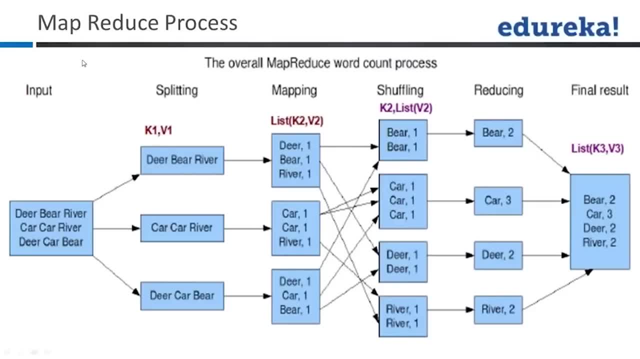 me in practical right, so let me show it to you in: yes, it is, it is Vinay, like that. okay, but let's not, let's not do that comparison here, because that's not the right point to do that comparison. we will compare that when we move further in our classes. we will not. 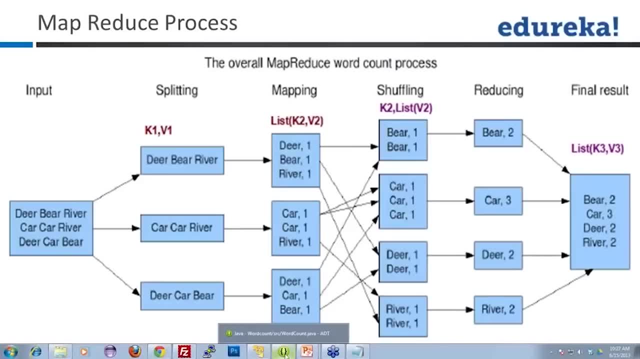 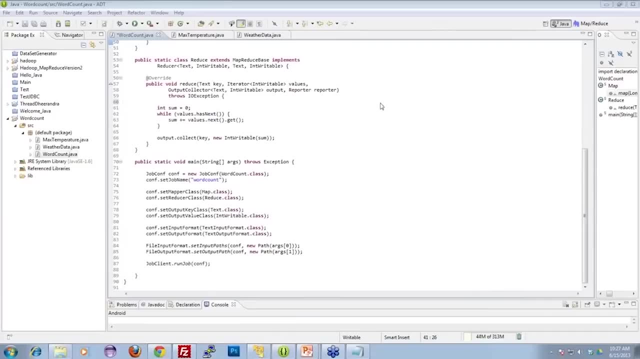 leave MapReduce now, okay, So let's go. So let's go and look at things. how do they look like in a program? now, though, I promised you that I will be using Hadoop streaming as well and show you in various languages. 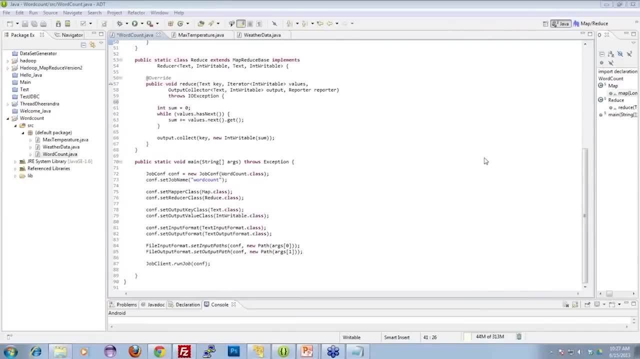 let me get started with some Java. okay, now, everyone knows Eclipse. let me show the same thing happening in Java. okay, everyone knows Eclipse. this is, this is a familiar thing to everyone. okay, you want me to match the window? I, what I will try to do is I will. 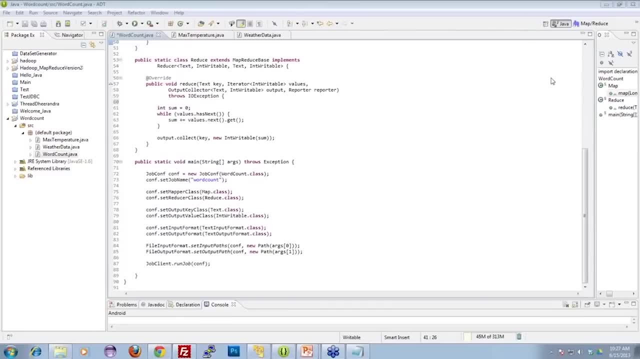 probably increase the font size here so that it becomes much more clearer. right, just give me one second. I will try to do that. which version of Eclipse are you using? is the question Avinash is asking me. Avinash, I don't know. here there is some version which. 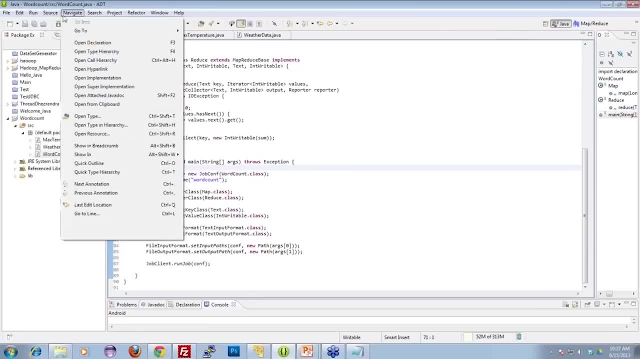 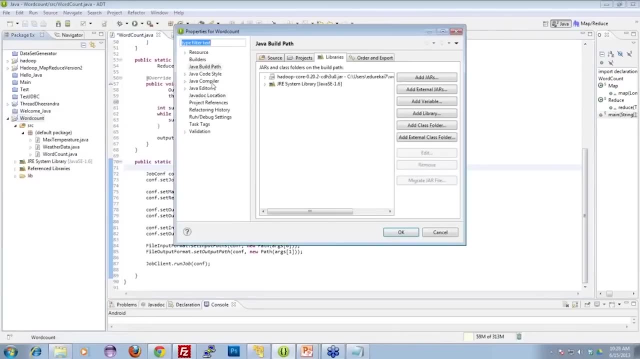 works well, so I use that one. but I don't worry, I will tell. I will tell you, Avinash, just give me one, I will tell you. I will tell you which one. I know how to find the version okay. 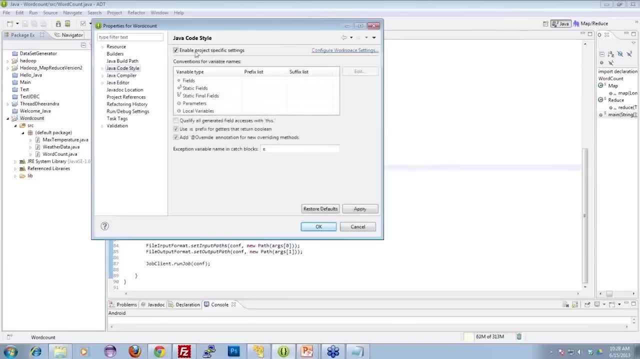 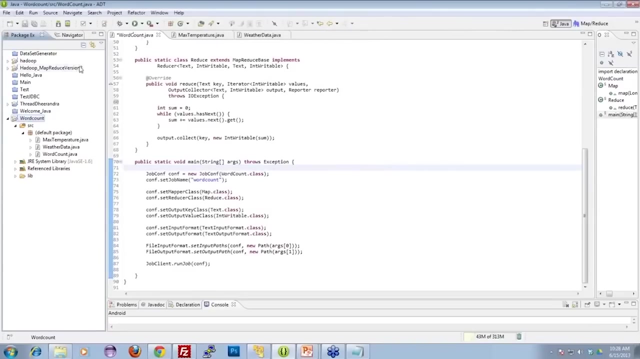 Okay, So let me just try to find out if I can figure out a way to increase the font size. I am not able to find that. anyone tell me go to editor is what my friend is telling me: windows. okay, Avinash, what next preference? okay, Avinash, what next preference? okay. 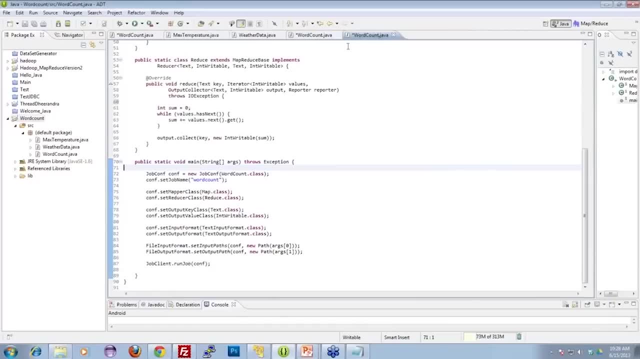 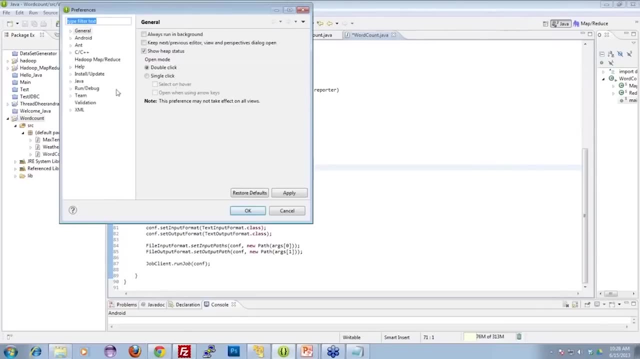 go down, go down, go down. I need to go down. right, there is a no, no, wait, wait, wait, wait, let me. let me just do that preference. okay, I think it should be in general preference. 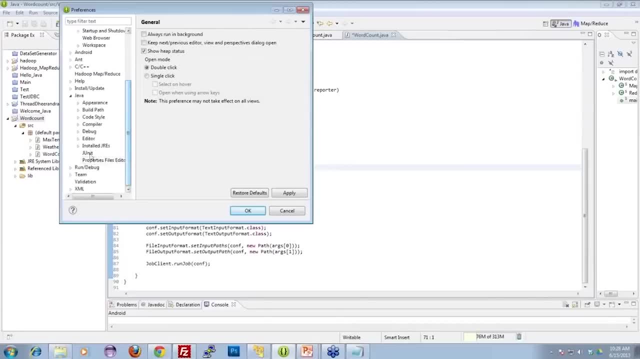 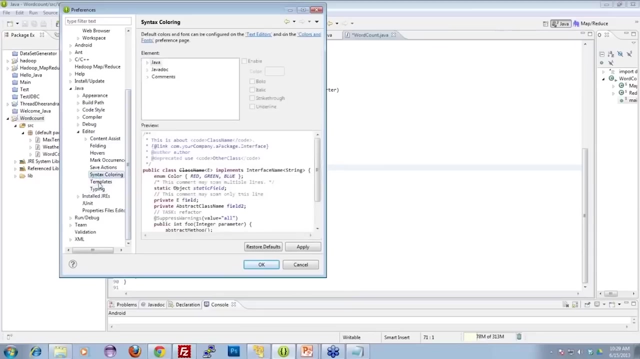 is Java, is what Avinash is telling me. okay, then what editor? okay, Where do I find the option to increase the font size? Syntax coloring general. text editor: okay. windows preference general: yeah, that's. 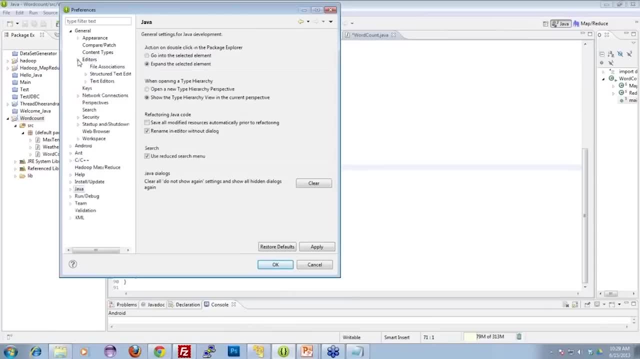 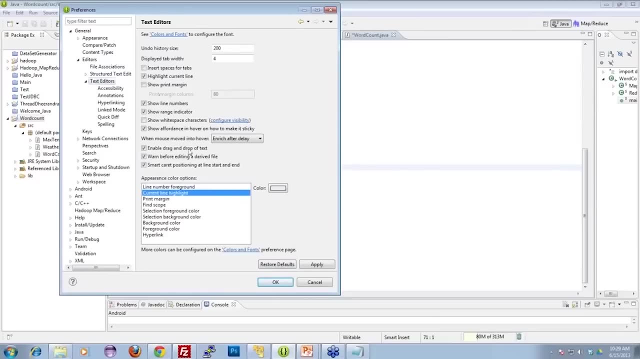 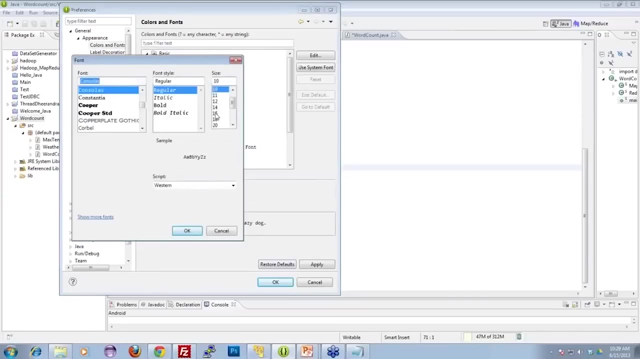 what I thought: text edit. it should be in general editor. go to text editor. okay, great Mikey, so providing I am there now, help me out. okay, got it, so I think we can just increase it a little bit. okay, so is this much better days? 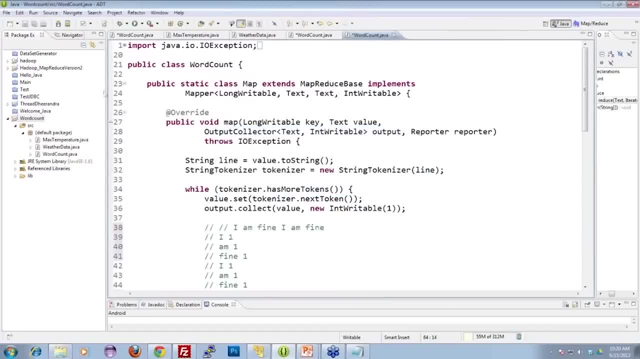 Everyone is able to see this, Great fine. so let me just talk about one offense. I have seen it in the last few videos with Uusell. this is what the purpose of Uusell according to. they are very important purpose, right. 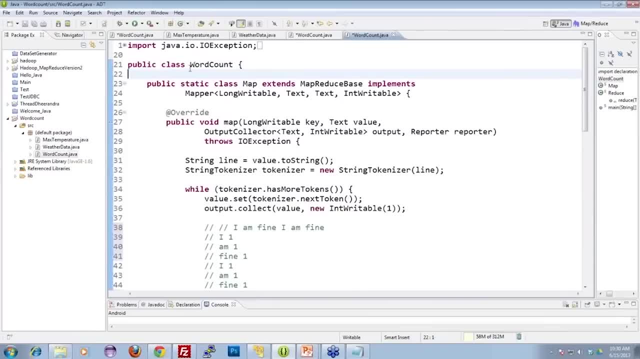 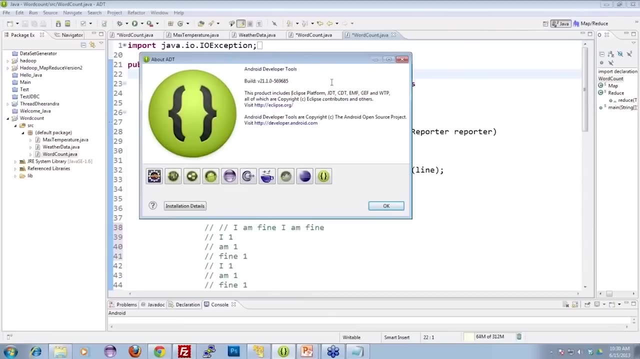 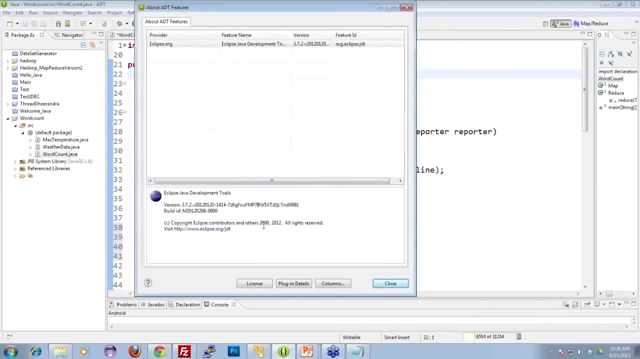 Let me show you this. I mean now, this program which we just saw is actually Avinash. just a minute, I will tell you which version are we using. okay, just give me one second. so this is the ADT Eclipse version. so this is the version Avinash here. okay, I will probably. 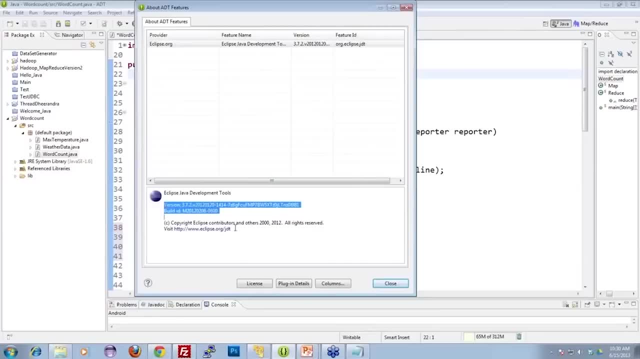 send you this. you can download the same version from. we will say: you can have the support team these people can give you okay. no, I don't think there is any reason. there is no reason why we are using the Android one, because just to tell you that there is a very 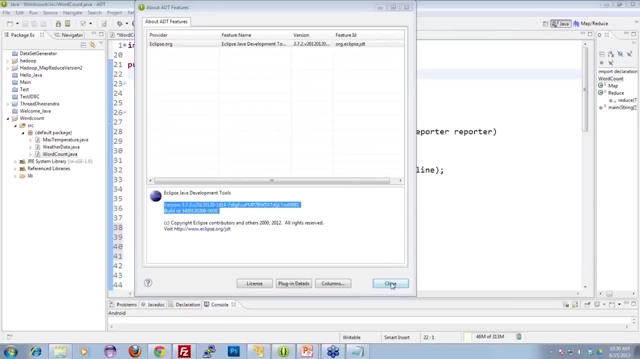 popular Android program which Edureka runs, and my friend here is telling me to publicize that a little bit, so I will do that. so that's why they are using this Android version. okay, there is a very popular Android program here, guys. 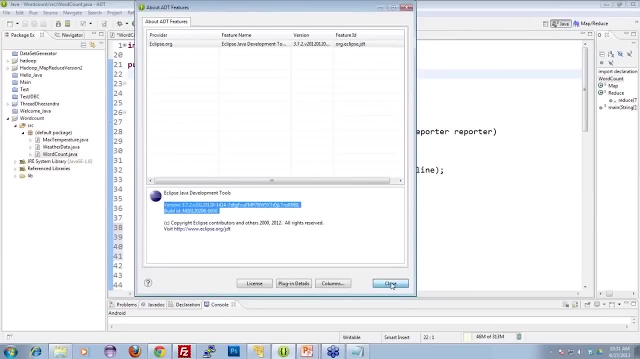 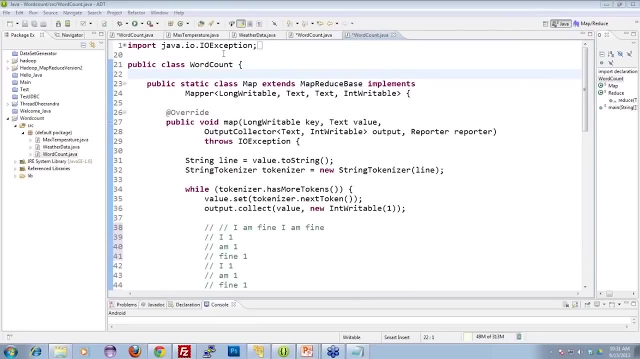 So anyone of you who wants to learn Android, or have kids who want to learn Android, ask them to join Edureka's program. okay, thank you. thanks, that was a commercial break. okay, so I will send you this version if you want Avinash, okay. 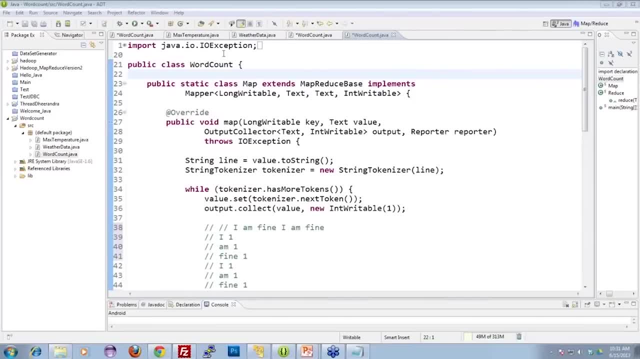 Now let us come to this. now, what we just saw was a word count program. okay, what we just saw was a word count program, okay, no, there is no extra, so there is some. what we will do is: we will- I will answer that question later. okay, we are not talking about. 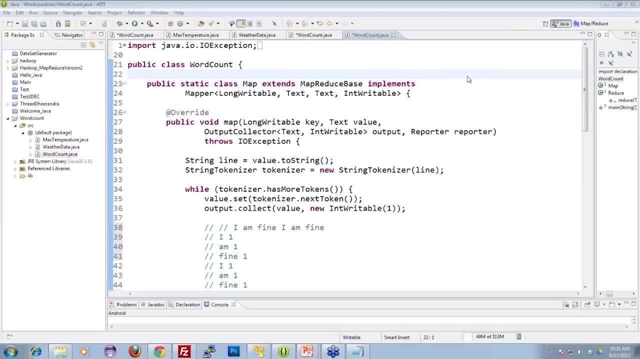 Eclipse right now. okay, okay, Deepankar, that also I will show you. wait, wait, wait. I will tell you one thing: what I am going to do now: what I am going to do now is I will show you this program, I will explain you this program in Java, then I will create. 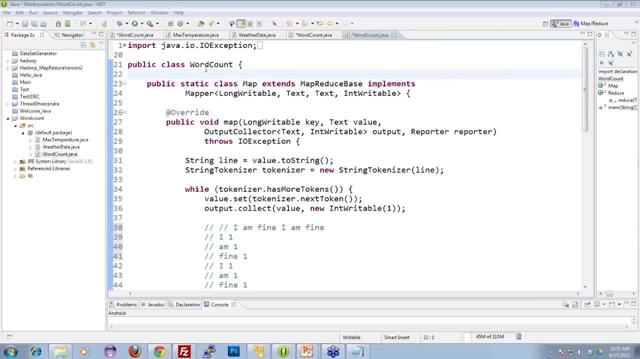 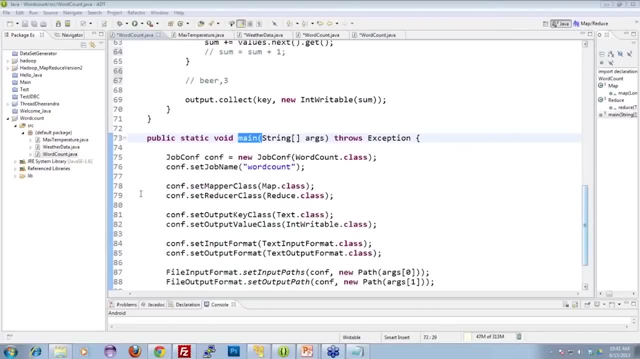 a jar file out of this, then I am going to run this same program on Hadoop and show you how the really runs. This is version. First thing which you do is we define a jobconf. Now we call it. we define a new job configuration, wordcountclass. You can set a name also. 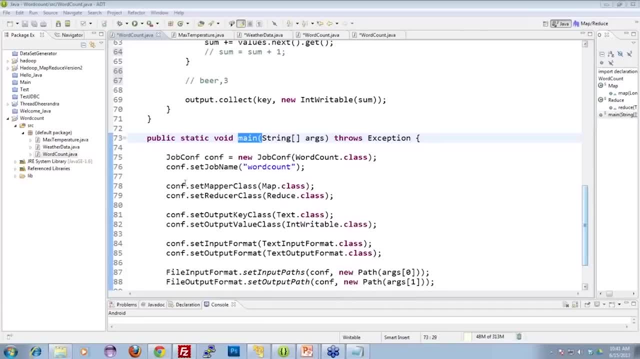 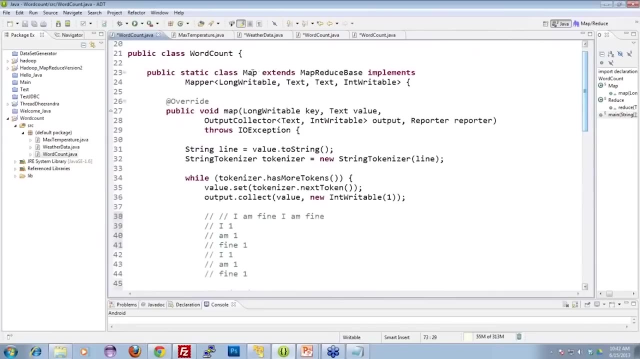 This is optional Wordcount, No need to worry too much about here. Then you set the mapper class Convset mapper class. So this is the class in which we set the mapper class. Mapper class is this map class which you have defined up here. This is the map which. 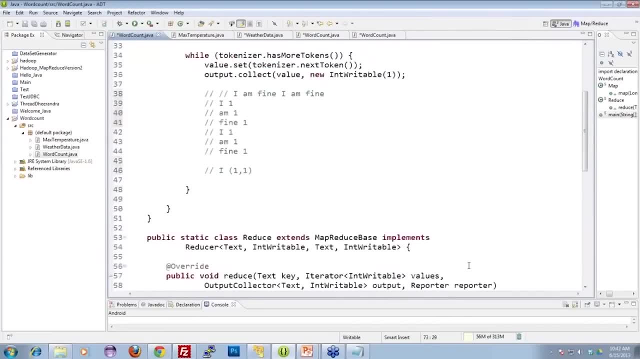 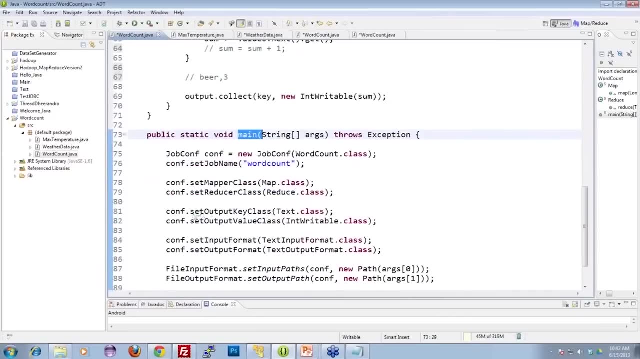 we are talking about Now, if you go down, we also define the reducer class here. Then we set the output key class. Now what will be the output type When the output comes out? we know the output is a key and value pair. We know, everyone knows that. 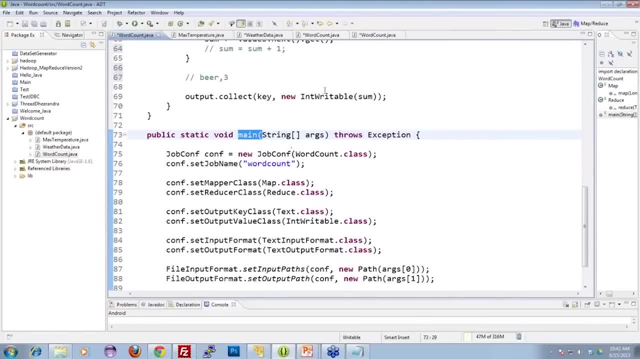 From the last slide we have seen that, guys, Is that correct Or is it not? You don't remember that. I want answer from everyone. guys, Great So, yes, great. So now we know that: the output. So here, this is where we define what will be the output type: The input. 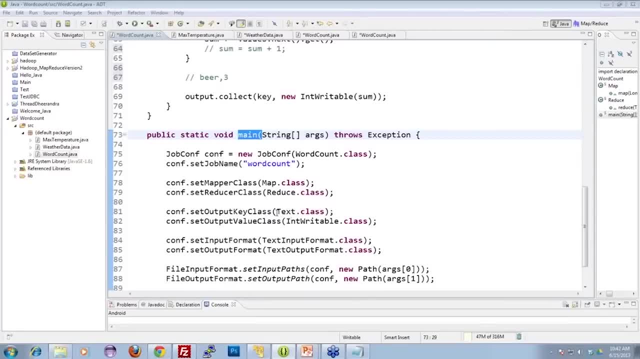 types can be different. The output types can be different. Now in this program, since we have text as the output key, where it could be bear dare whatever right. And int writable is a special type of int for Hadoop And since it is integer output, we 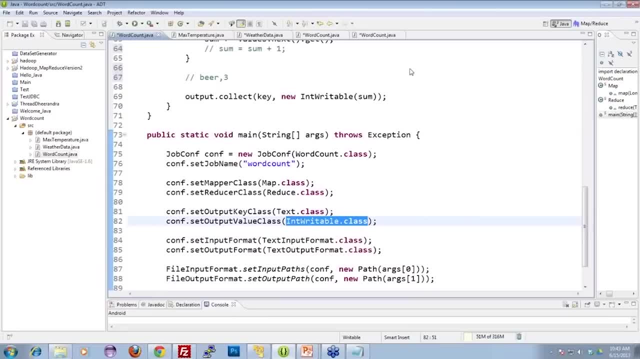 will be using that. So Dilip, my friend, is trying to help me out. Thank you, Dilip. He is telling me here are the four basic parameters of mapper: Long writable, text text and int writable. So we will talk about them a little bit, But let me explain you from a top level. 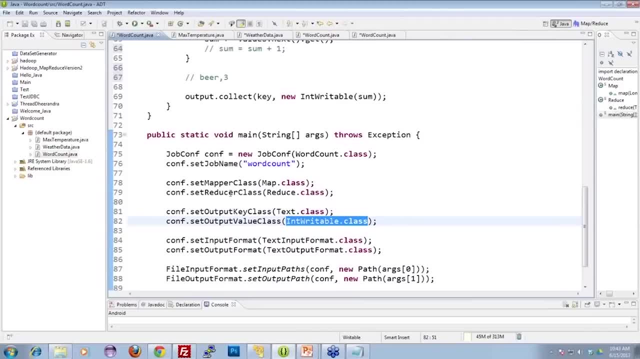 where we are looking at. we are looking at the black box where we are just talking about what is the output and what is the input here. We will go into it just now, Just in a while. we will go into it For now. understand that the output is a text. The key output is text. 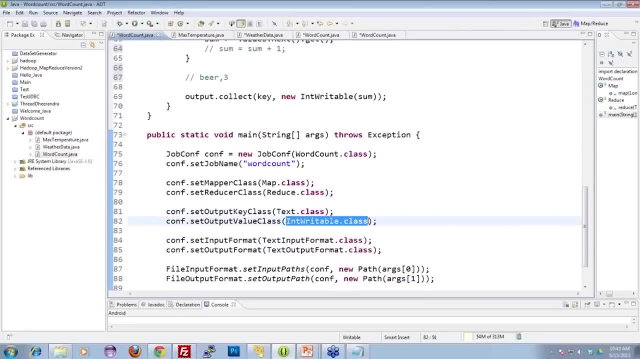 type. The value output is int type In this particular program which we just saw, where we are talking about bear, dare and whatever right. Similarly, there is no reason why we have defined output before input. It doesn't matter, It doesn't matter, It doesn't matter. 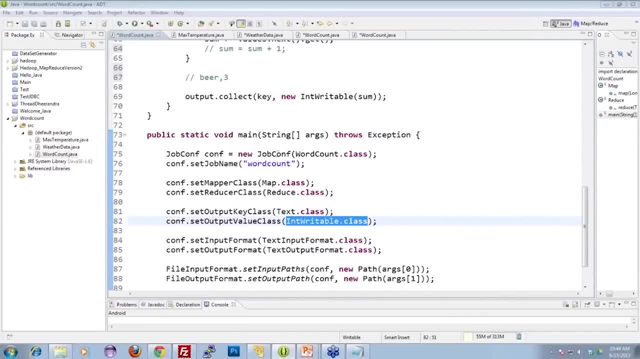 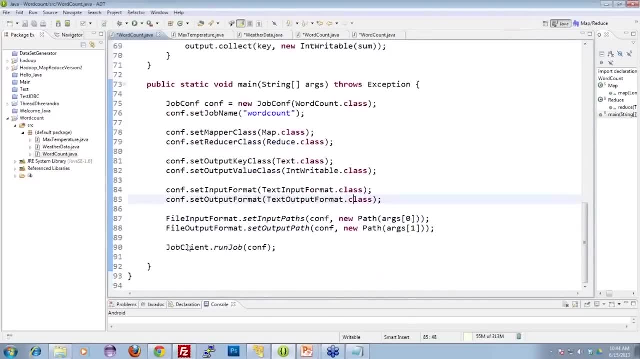 Avinash is asking why we have output before input. Okay, it can be in any order. All these can be in any order, right? There is no problem with that? Okay, is that fine Now, finally, this is where we set the input types. Now, as I promised you right in the beginning of 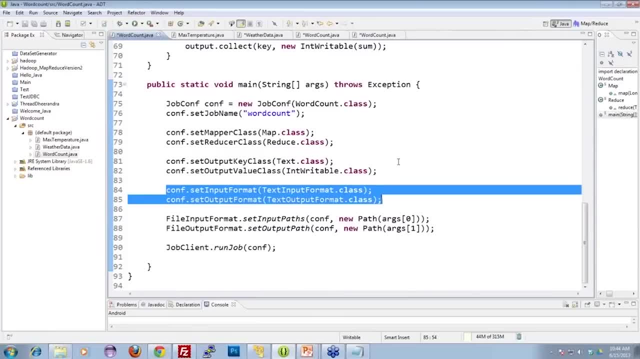 the class that I will be discussing about different input types and different output types input formats. Just assume that right now we are setting the text input format for this class. for the input format, Okay, the set output format is text output format. These are the default values, So 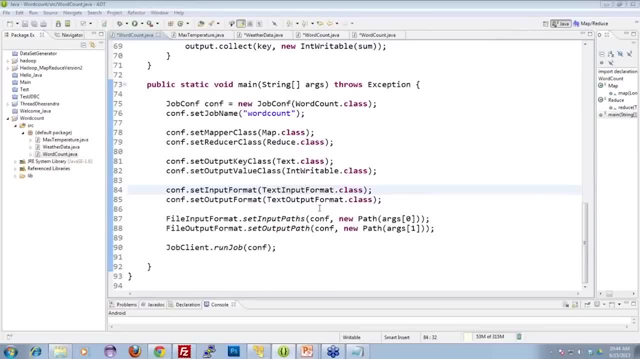 don't worry about, these are the default values. We will look at more types in the next class probably, where we will talk about sequence and all those things which I mentioned in the slide first. Now, this is very important and this is one of the things which you should. 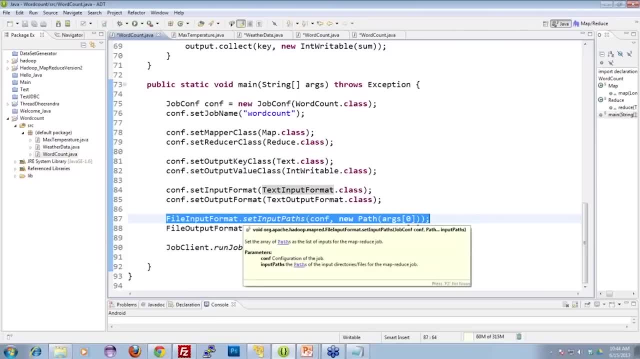 really look at. This is file input format, that's dot set, input paths, conf and new path, which means this is the path from where I will pick the input files Okay, on which I will be doing the processing. Okay, and arg zero. everyone knows what it means. Everyone knows that, Anyone. 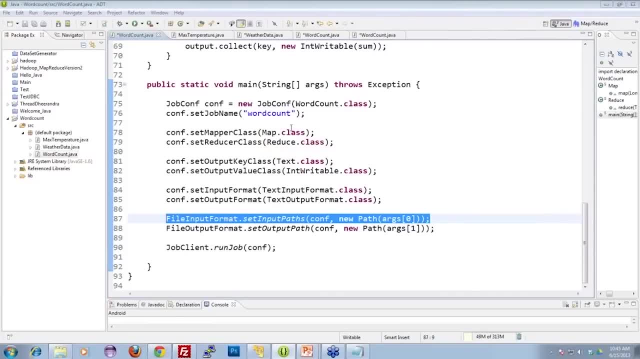 who doesn't know that? Okay So okay. So basically, command line argument number one will be arg zero. If you are passing command line argument, that's right. So arg zero will be the first argument which you pass. Okay, So basically, command line argument number. 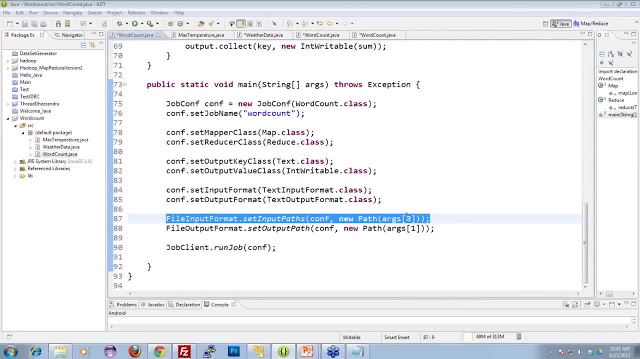 one will be arg zero. If you are passing command line argument, that's right. So arg zero will pass along with that command. Okay, Okay, Gaurav, is that clear? And arg one will be the second one. Okay, So when you run this program you will say program name, then input. 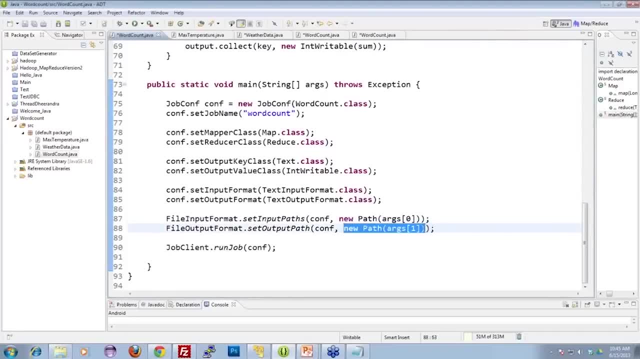 file path and the output file path. Okay, That's how we are going to run this. Okay, If you remember, last time we showed you a jar file and we showed how to run a program from that. We will be doing the same thing here also. Here, these are the inputs, and: 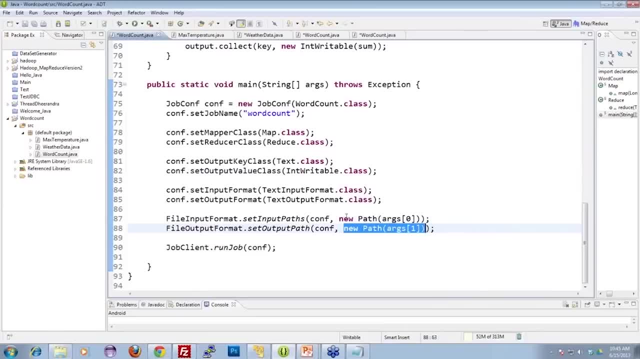 the outputs of that. Okay, We will just do that as well. We will show you this. Okay, For now, let's try to understand this program. So this part is clear. Then, finally, we will say: this is the run job method. Okay, There is the run job method in the job tracker. 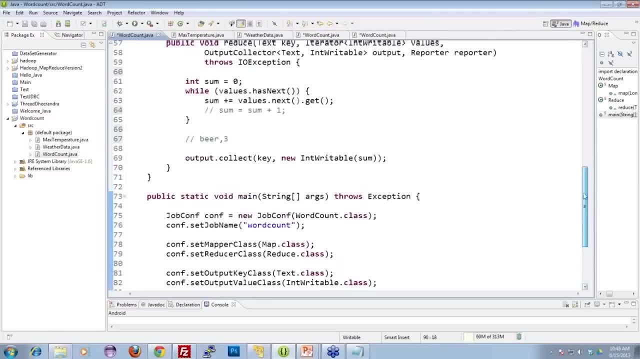 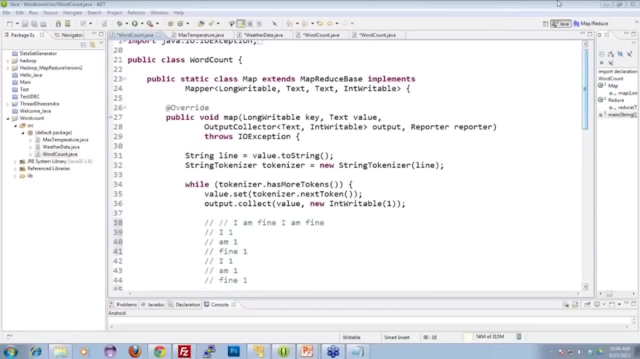 Okay, This will tell the job tracker to run this command. Okay, Now let's go up. We will understand more of this. Let's look at this map class and what is it doing? Is it doing really what we showed in the presentation just now? Okay, Let's try to find that out. 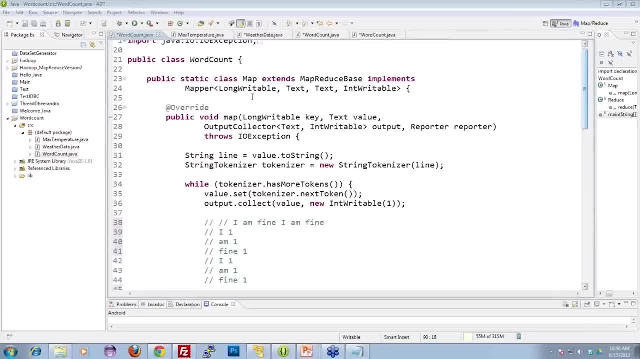 So basically we have Now. this is when we say implements, which means this is what This is: a class or interface. Whoever knows Java has to answer that answer. Give me that answer, Okay, Great, So our 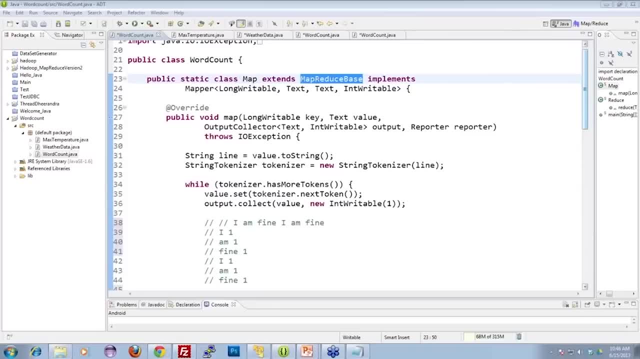 class map extends the interface, extends the base class and implements a mapper interface, Right, Is that clear guys? So this is the base class and this is the interface, Right? Everyone is clear with this. This much Java, everyone knows. 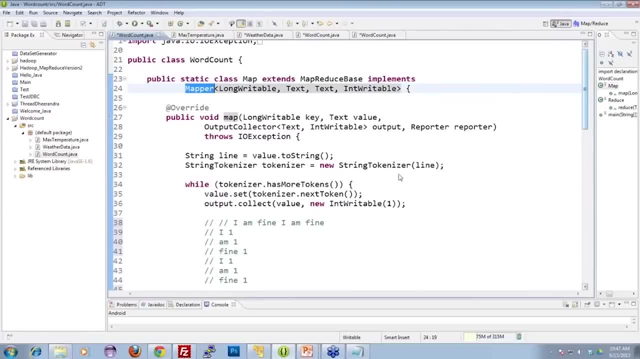 Exactly Extends base class and to implement method in mapper interface: Exactly. Okay, Just a second. Is my voice not clear to everyone? There are some people who are saying the voice is not clear. Great, I got it. So let's start this. 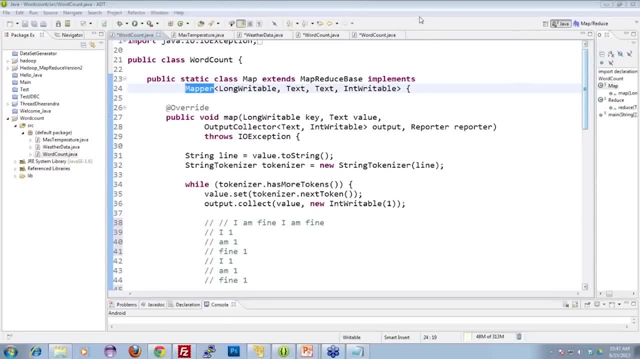 Okay, the bunker. Okay, Fine, Thank you, So is this clear to everyone? now, Right, What we are doing here? This is our class, which extends this class and implements a method mapper from the interface. Okay, So that is how. and these are generic inputs, Generic types: Okay, 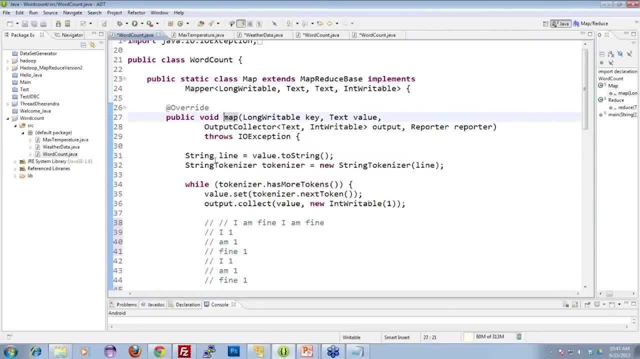 Now, when we come to this, we talk about a method map Okay, Which we are overriding, Right. We are overriding a method map Okay And defining it here, Right. So we have inputs, long writable key text value. These are the inputs And there is a output collector, which 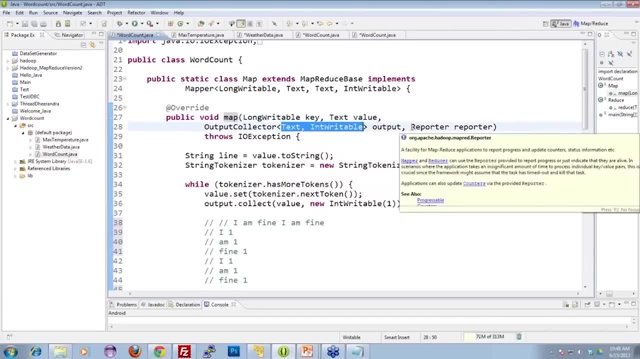 is text and int writable from the map. And reporter is basically, if you remember, when we run a MapReduce program it tells us that 0% done, 2% done. that reporting which happens on the command line Right On the screen. We will show you that as well, Do you remember? 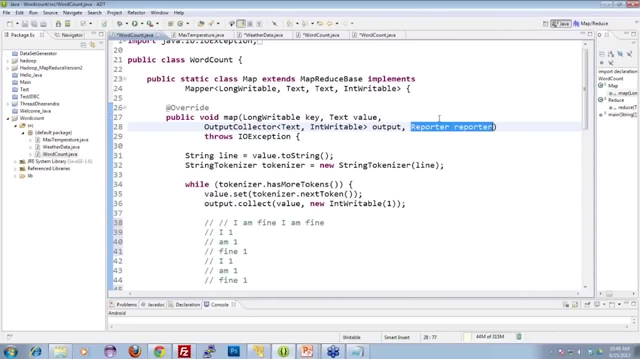 that What happens when we run a MapReduce program? It shows on the screen that 0% done, 10% done, reduced process done. Remember that? Okay, Let me explain. Let me explain that once. So these are the input types. This is the output. collector: Okay, And reporter is the. 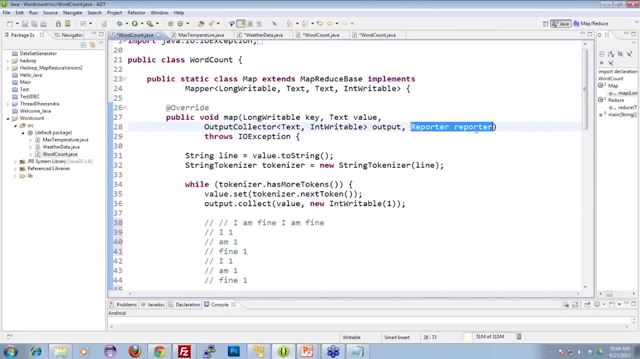 thing where we actually report what is happening. Okay, Yeah, It is a progress updater. Exactly, Rajat. Rajat has given me that answer. Thank you, Great. So is this clear? everyone, guys, And it throws an IO exception Now throws everyone. 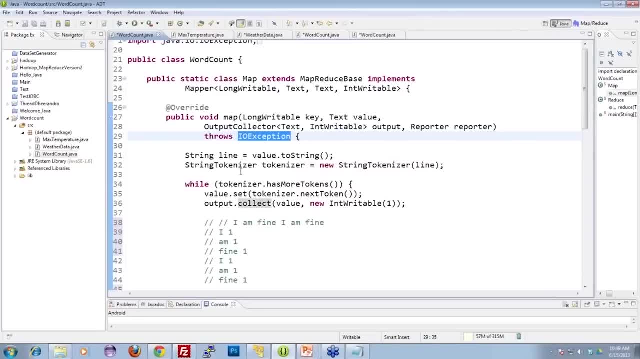 knows what throws is. Whenever it finds an IO exception, it will throw a. whenever it is not able to find that input file, it will throw an IO exception saying that file not found, or something. Okay, Is that clear, guys, everyone? Very simple till now. Quickly a. 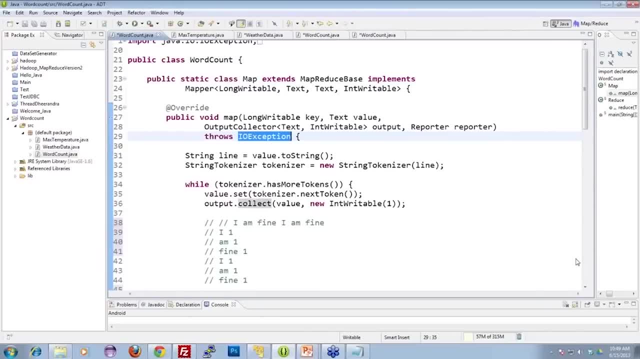 yes and a or a smiley very quickly. I want a yes from everyone. Great, Very nice, Very nice. Now, what we are doing here is we are saying: a string line, value to string, Okay. So basically, 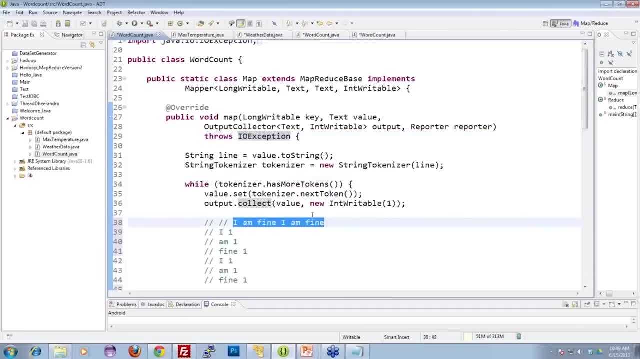 if this is my complete line, okay, it will go in this. You convert this value into string using this. Okay, This is my complete value and I will convert it into a line using to string method. Okay, Is that clear guys? So this, let us, let us see. I am fine. I. 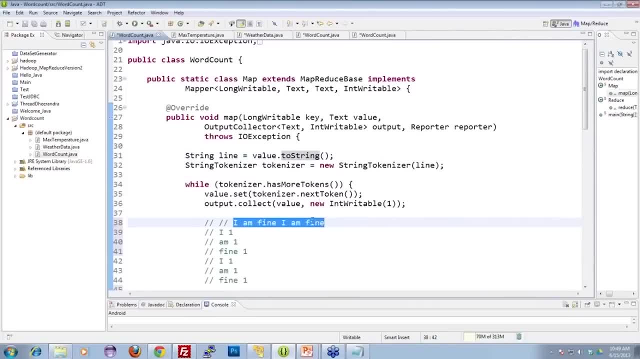 have written twice. Okay, Great. Now string tokenizer: we create a tokenizer out of it. Okay, Now, when we tokenizer means it will split these values. Okay, On what? can someone tell me that Avinash has sent me something, Okay, Okay, Great. So Avinash has sent an. 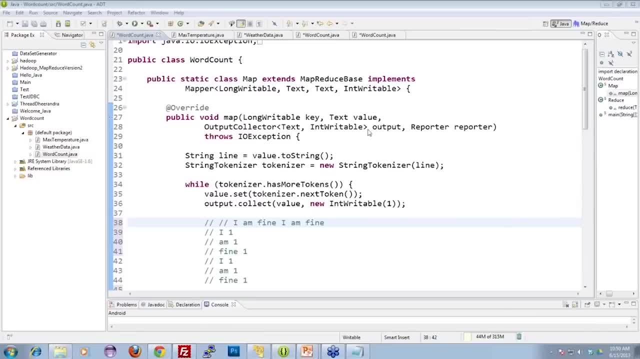 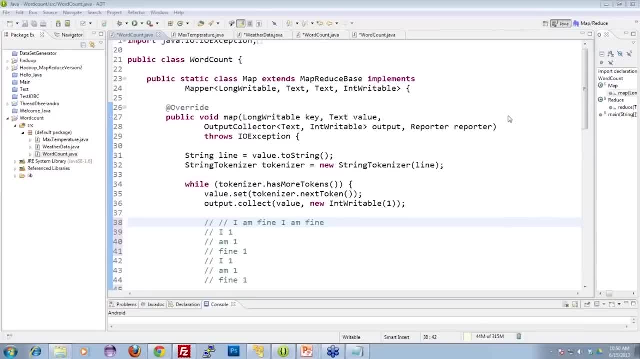 unless till the end of line. Rajat is telling me very nice default delimiters and space D-limiter and space each word. Okay, So I have got my answers here. Okay. So string tokenizer, this is test. Okay, Very nice. So Avinash has given me an output which. 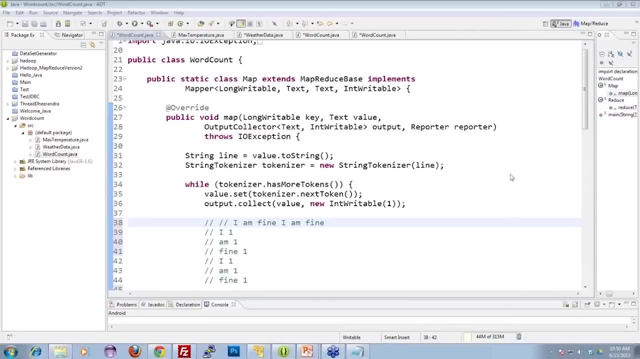 I will copy and paste. I will try to do that, Okay, Wa, And I really like this way of learning guys. Everyone is contributing. I really like that, Okay. So now For people: do they know, people who are not very familiar with Java Gaurav and all who have not been able to do? 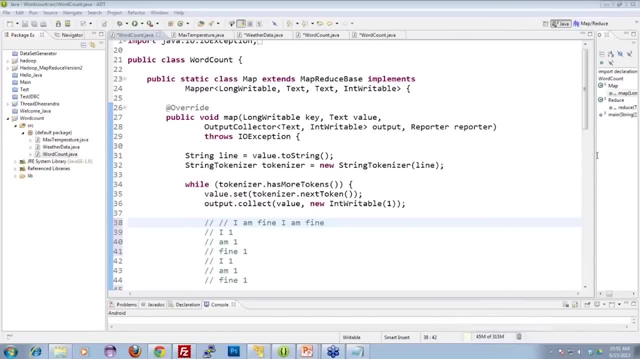 a lot of practice. this is what Avinash has sent us and I am sending that to you. okay, very good. so everyone has got this here where he has written us quick program which is string tokenizer st- new string tokenizer. this is the test. this is the complete string, while. 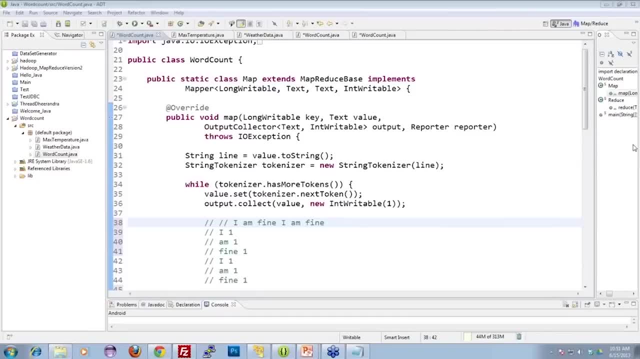 it has more tokens: println. println will print in the next token, so it has clearly told you that this is a test, has been splitted into four parts on the delimiter space by default and every delimiter has been printed here. okay, so this is a test, will come one. 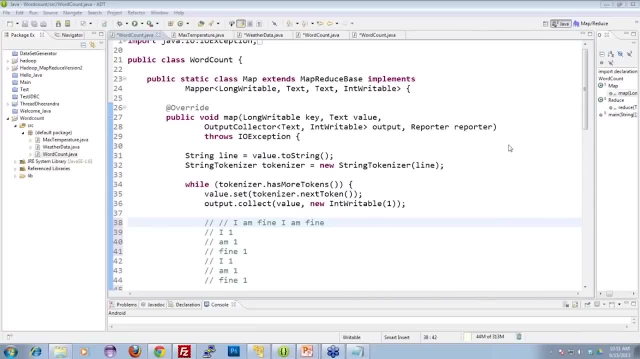 by one. is that clear to everyone? guys, let us give a quick round of smiley to our friend Avinash. okay, Dipankar has given me a said good one. okay, thank you, Avinash. thank you everyone. lot of people are saying thanks to Avinash, so now we have learned this part. 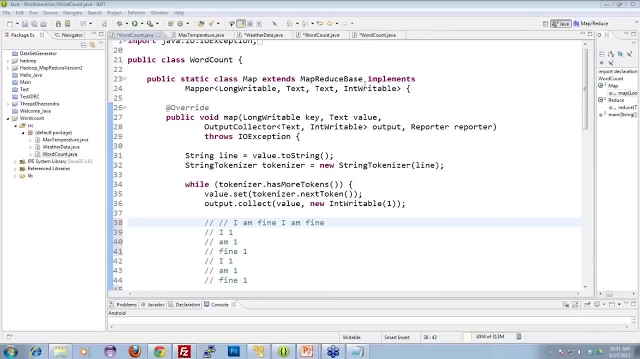 okay, smiley. Thank you, Avinash is what Shri Ram is saying. okay, okay, so Avinash has fully accepted all the things. okay, very rarely does he does that. okay, but okay, Avinash, just pulling. 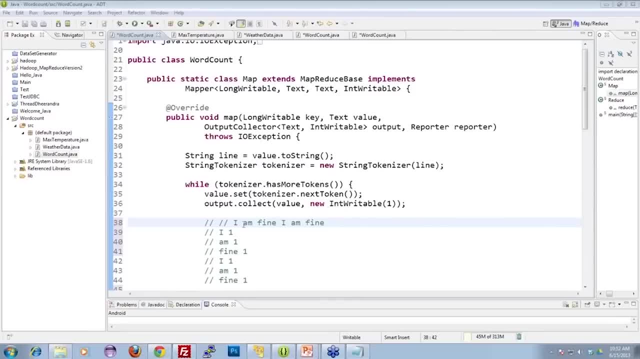 your leg, man. you are my friend, okay. so, okay, now, looking at this, now that Avinash has told us everything, we know what is happening here, right? so let me show you what is happening. so if we had this? 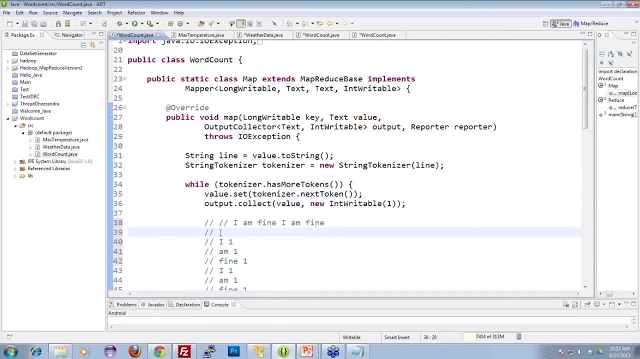 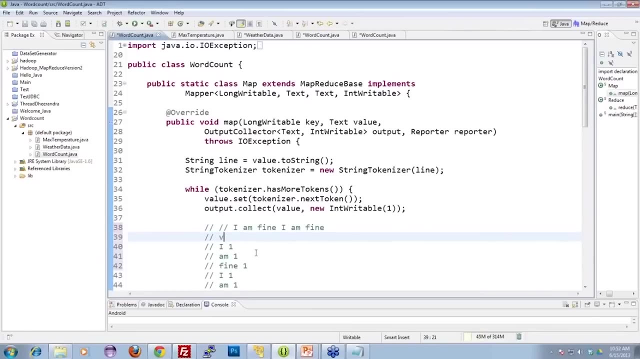 So this is the value. right, that I am fine, I am fine. okay, so this is the value. sorry, this is the value, okay, so I1, M1, like we saw in the last example, very similar to that. 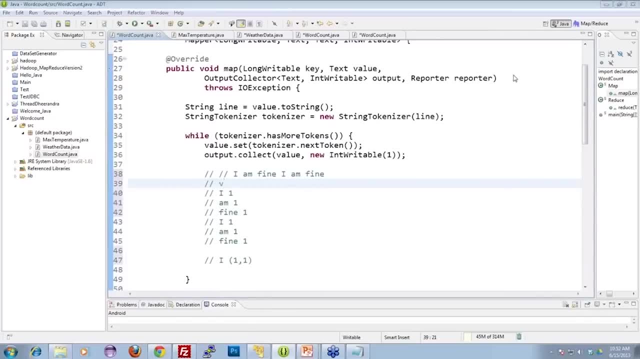 this will be the output of this. is that is this clear to everyone, guys, what is happening here? So what you are doing is, whenever you get a value, Yes, You say new value, will be assigned a value. new int writable outputcollect: okay, value. 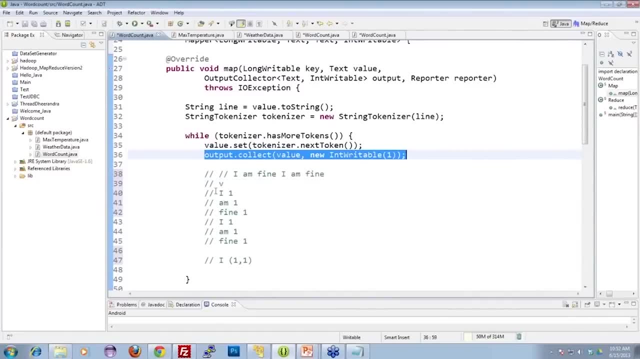 and new int writable. so this is what is going to make something like this: whenever you find a new token in this, I is a token, M is a token, fine is a token. then again, I is a token, M is a token, fine is a token, everyone- every time you find a new token, you print. 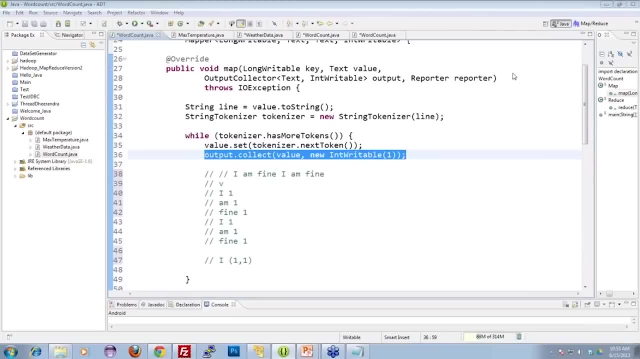 new int, writable one along with it. okay, is that clear to everyone, even to the folks who do not know? Java Ravi, are you still with us? Did not get it. Yes, No, are you still with us? Great, great, okay. so the guys from the EST time zone: I know it is a little late, but 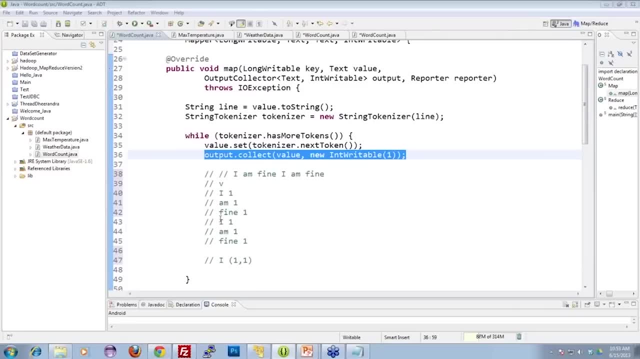 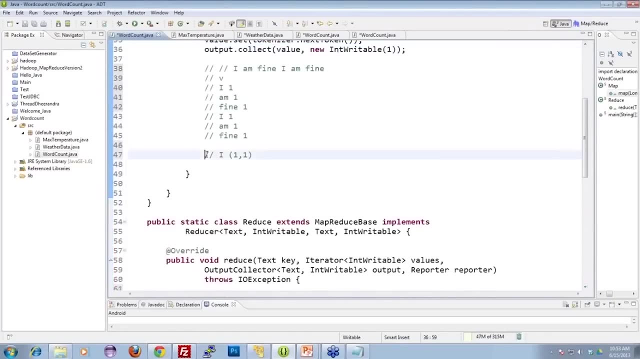 we will quickly be able to finish this up. okay, great, so now this is what we will get as out. okay, is that clear? Now let us go to the. so this is what will finally happen. as I told you, this will be. 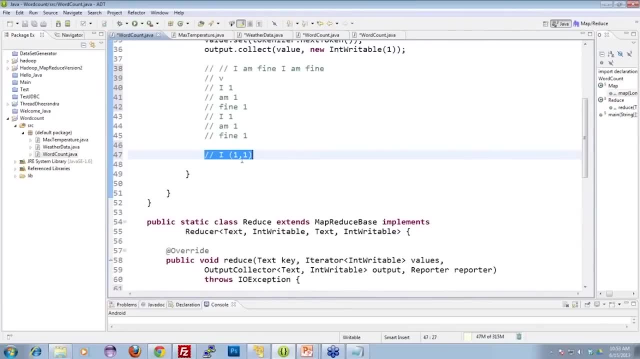 done automatically by Hadoop itself. okay, so this will be converted into I11, like we have done in this presentation. right? is that clear guys? Something like this is going to happen: I11, M11,, fine11,. this will be the thing, okay. 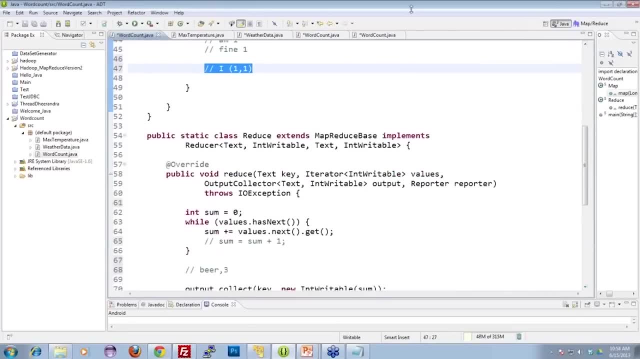 keep on writing. yes, if you have understood it. if you have not, then keep on writing. no, okay, great, let us go to this. okay, now and see what is this reduce thing doing. okay, now, the reducer input is again the same thing. the text which is I and int writable: okay. 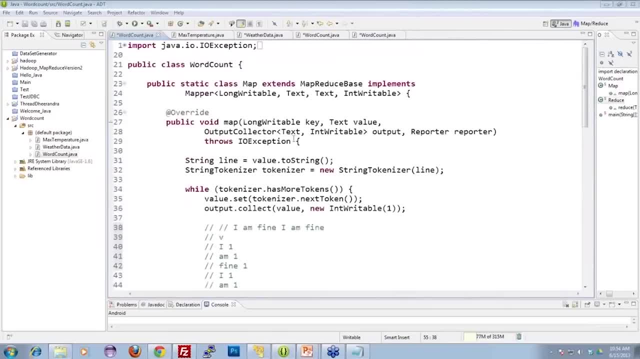 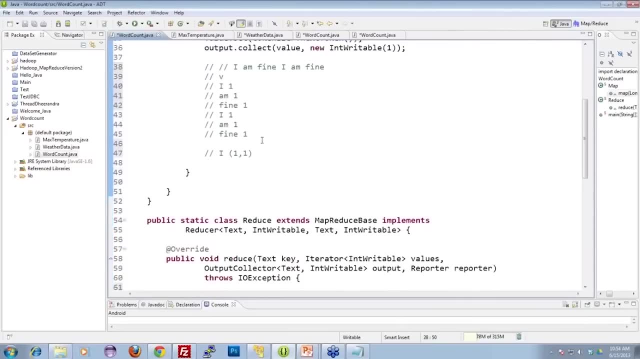 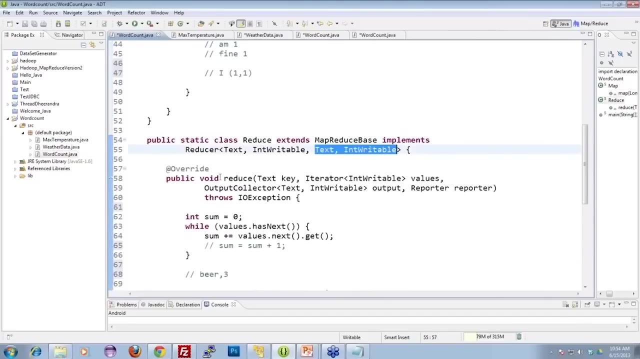 now look at this: The input to the: yeah, so this is, this is what we outputted from here. the same thing goes as a input to our reduce function: reducer function, right, and finally, the output will be text and int writable. okay, now, if you look at this method, what we have here is: 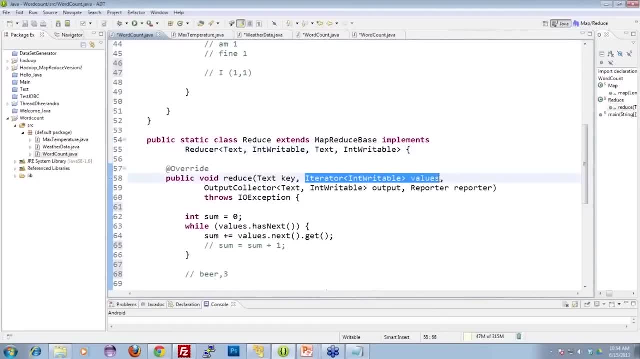 text, which is a key, and then there is something called iterator. what is an iterator, guys? Quickly, what do we need here? List, right? no, it is okay, so it is a list. list of values is what Vamsi tell me. 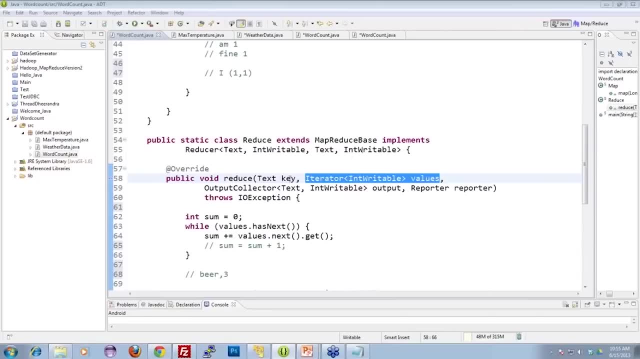 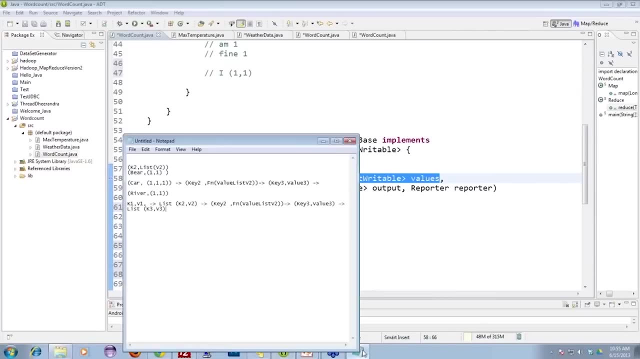 oh, iterate over the list. very good, so iterator will iterate over the list. so, as we saw right, this is the input which we will be getting here. so, as we saw initially, k and list v2, you remember that thing which we did where this is the thing which we had right. so 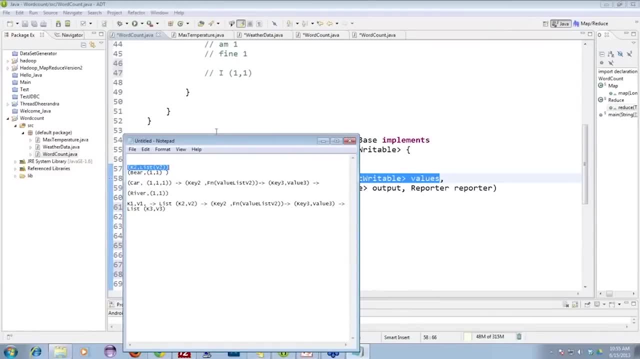 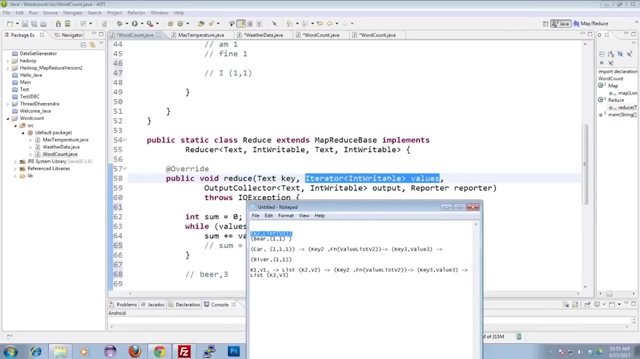 this is. this is where we use the iterator thing, right? Okay? Is that? is this clear to everyone, guys, the relationship between this part, this mathematical equation, and whatever we are doing in Java here? quickly, yes, good, very nice, very. 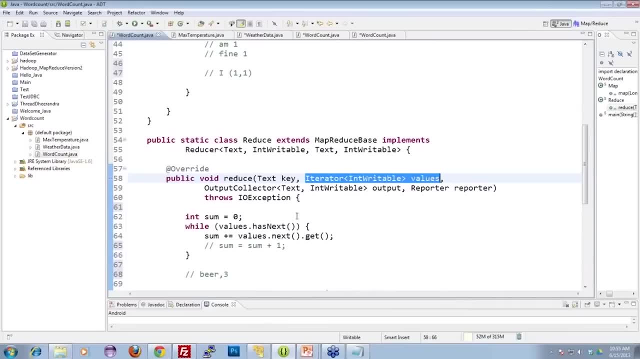 nice, okay. now then we go here and say IO exception, throw the IO exception again, again text and int writable are the outputs- and report reporter. same things. we saw now what we do, since we had to do a sum and tell, tell you how many times we have to do a sum. 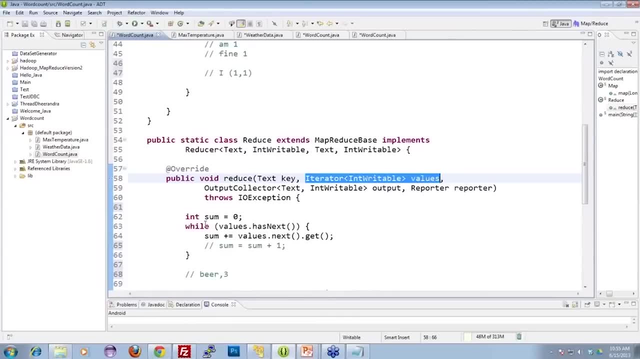 tell you how many times does beer comes and how many times does bear comes and how many times does does car come. what we have to do is, on this values, this was the iterator has next tells me if it has the next value, okay, it will come, false when we reach the. 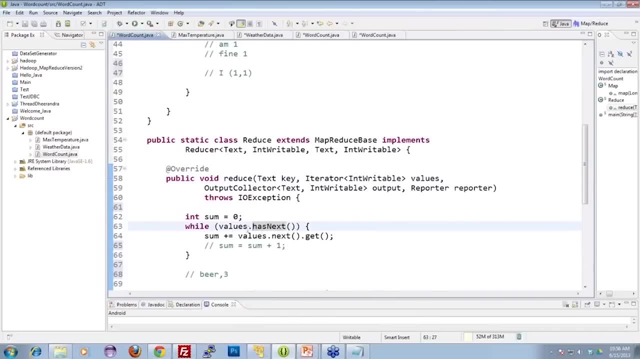 end of the list. okay, guys, everyone who is new to Java, this is, this is how it works. okay, what you do is sum plus value next, so the value of the next. you will get it here. okay, this will. this will take you to the values next and this will give you. 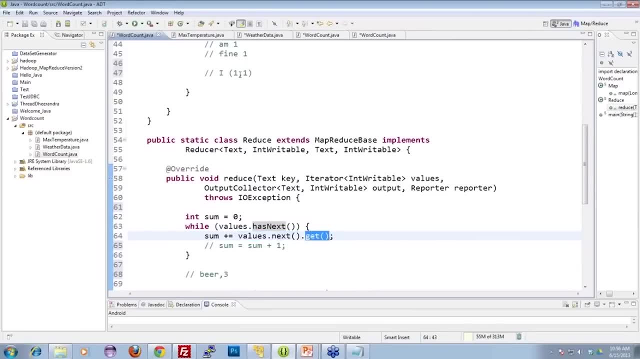 the value which you will get here, Which is there in the next. okay, so the value here will be one, right. every time on this list, sum is equal to sum plus one, so every time you go through this loop, you will come. 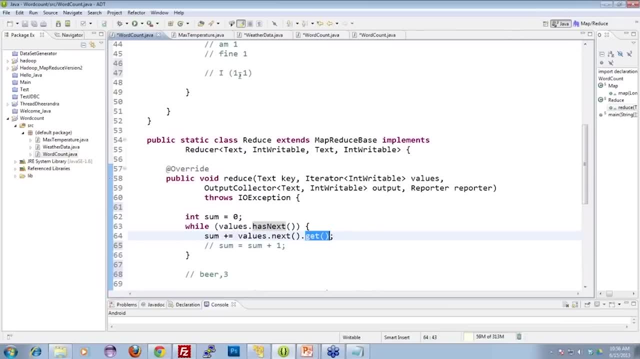 up with one addition into it. if, say, if this was the input, then it will come with one first and it will come with two. finally, when we get out of this loop, when we have finished this list, it will come with something like beer three, beer three. is this clear to everyone? 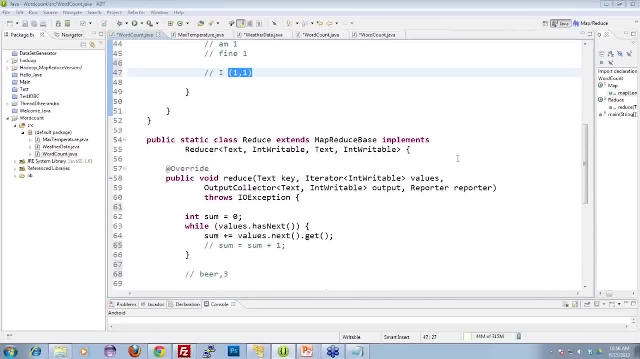 what is happening here quickly, yes or no? so now, if this is clear, then you have understood the matter. So this is what we have produced in Java as well. okay, now let's look at our original program, if you've understood everything here. yeah, yeah, Ravi, I'll answer that later. 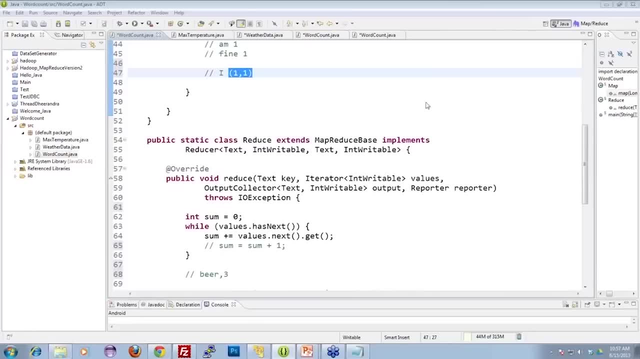 okay, it's a it's an old API. okay, it's a deprecated API. okay now, where is the flow of sorting of data take place? okay, so this was this. takes place. okay, so we will also be looking at some. there are some more steps which happen. there's a very simple way to. 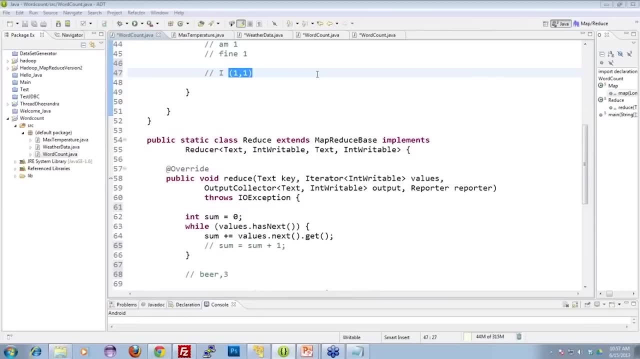 do it. there's a very simplistic program. is the shuffling steps itself? okay, yes, in the shuffling step itself, the sorting also happens, and we will be looking at the other things also: partitioner and combiner, which we'll look in the next class. okay, let's. 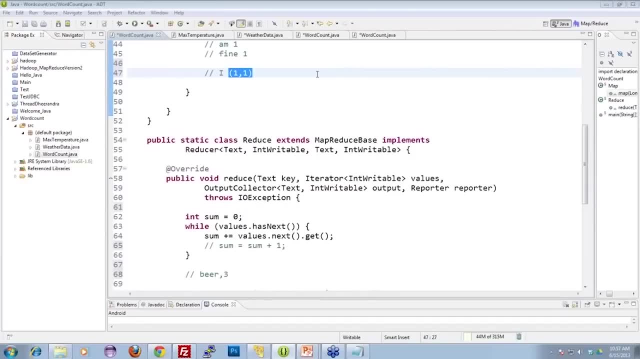 not go into that. I'll also tell you where we need it and what are the limitations with this program. this is a very simplistic program. okay, guys, is that clear? this is clear to everyone. now, what I'm going to do next is great. can I quickly get a round of smileys? 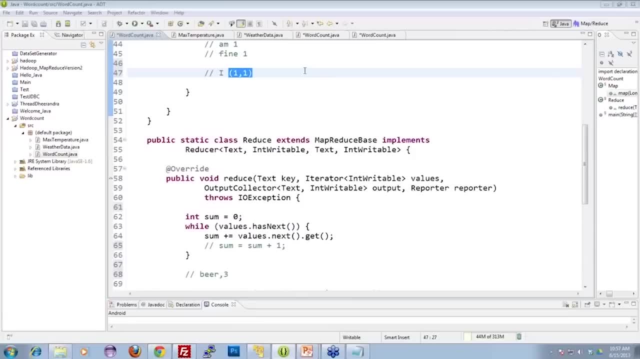 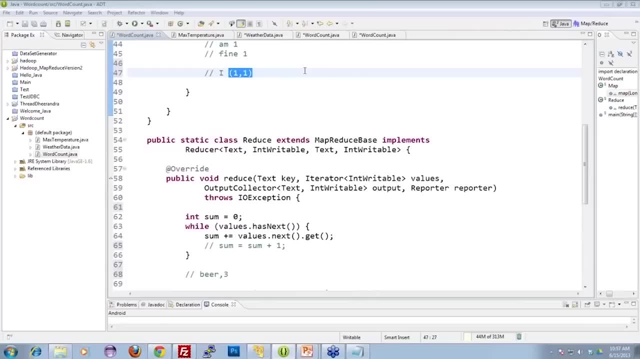 you understood what is MapReduce. you also understood how to write a MapReduce program in Java, right? isn't it great, right? so now let's see how do we actually run it in a cluster, right? so before that, let's go to our weather data. okay, let me show you. 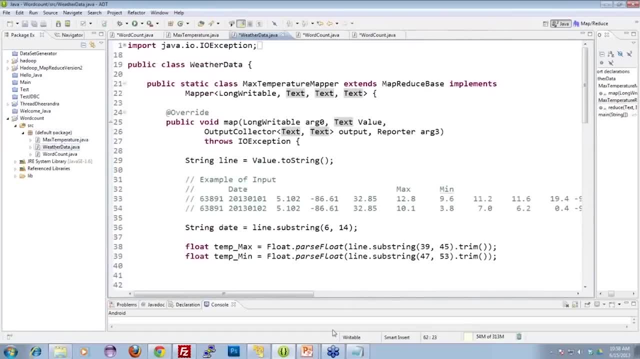 the same program where which we saw the initial data which we saw- you remember that right, the first data set which we took out, which was looking something like this: you remember that, guys? I don't have to explain these things. I'll go back, go down into this. 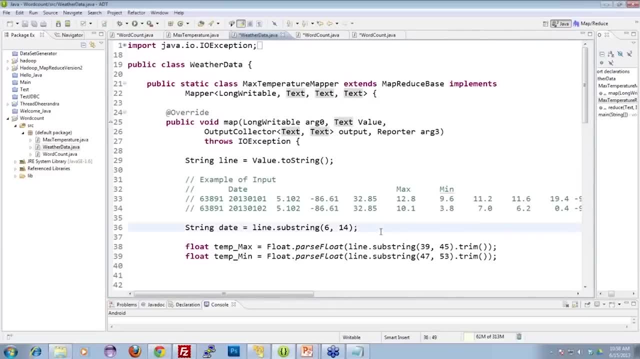 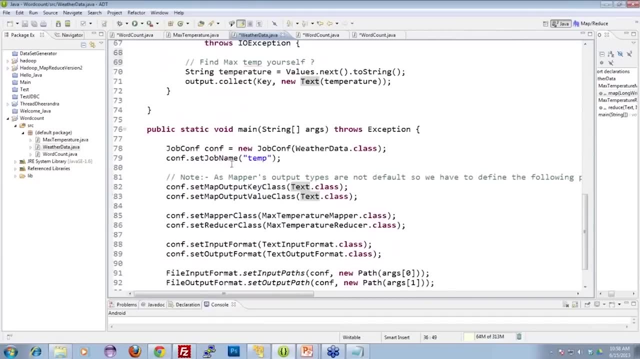 program. I'll quickly go down into this program and show you the same things which we saw earlier as well. okay, there's one difference though: we same thing: create a job set job name. now here I put a quick note for you. there the class was different, right. 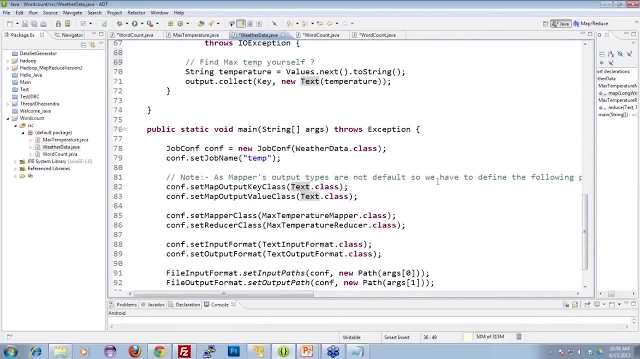 set output map class was different. these are not default here, so we have to define them. okay, so these properties had to be defined earlier. it was not defined at all, right? so these are the two new things which have come up in this program. I want you to 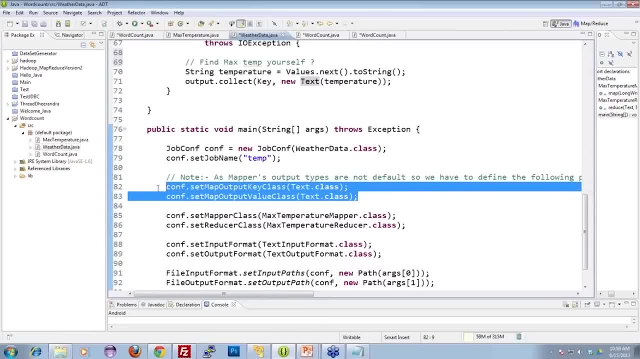 look at these things. when we get out of the class, I'll be sending you both these programs: default input types. there was what text and int writable? you remember that? yes, yes, Fancy. now, in this case, the output is what you have to give me. 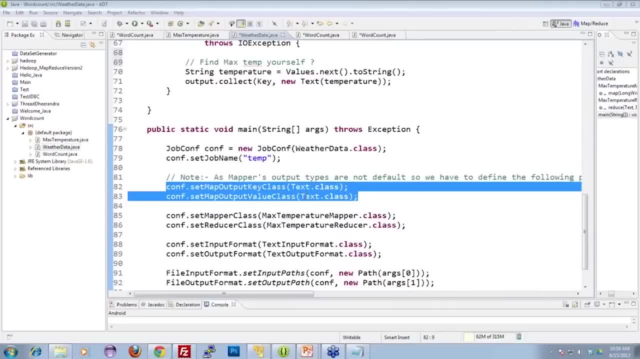 a text only, right. what is the maximum temperature there, right, whether it is, I'll tell you what we're going to do with this. so that's why we have to redefine this right. so that's the only difference. other than that, there's no other difference. everything remains same. 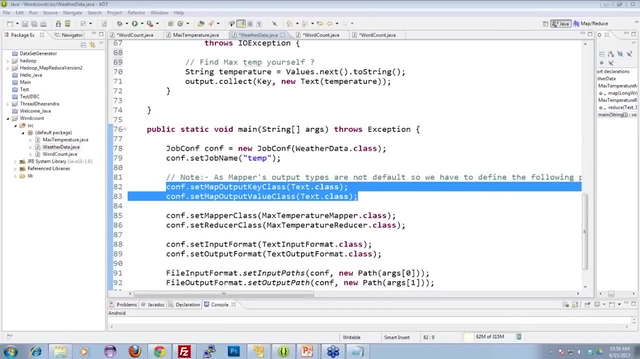 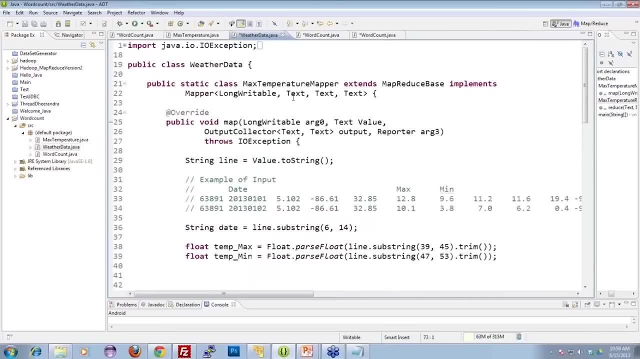 same way we define the input file path, output file path. let's go to our quickly to our map function and see what we're trying to do with this. okay, so in this, what we're trying to do here quickly is that again we do the same thing: value to string we got. 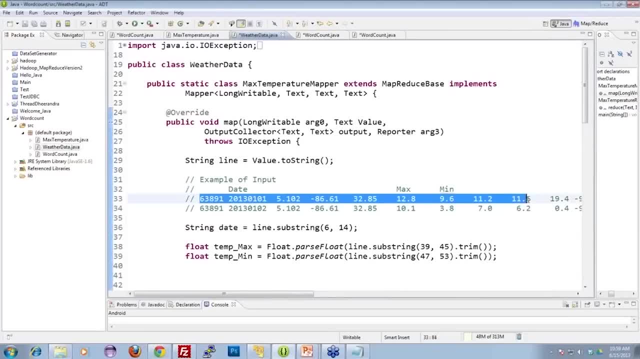 everything in this line, Right. so this becomes a string type, this complete thing. now what is this doing? line substring 614, okay, this guy tells me where is the date. so date is here, right. so you pull out a substring out of this and this is how you get the date value. here is this: 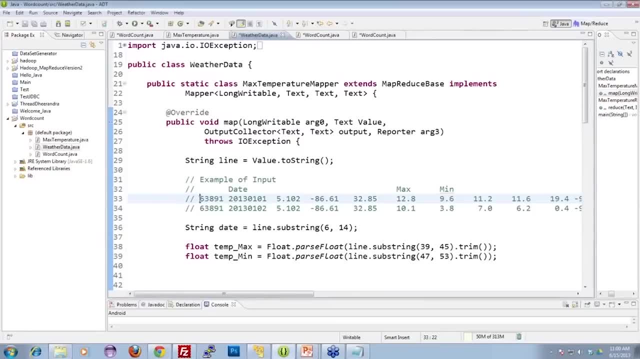 clear to everyone. this line 36, what we're doing here. the line contains this whole thing, whole record. okay, and substring 6214, this guy will contain your date, okay, so you're. similarly, we'll get the minimum temperature and the maximum temperature and the minimum. 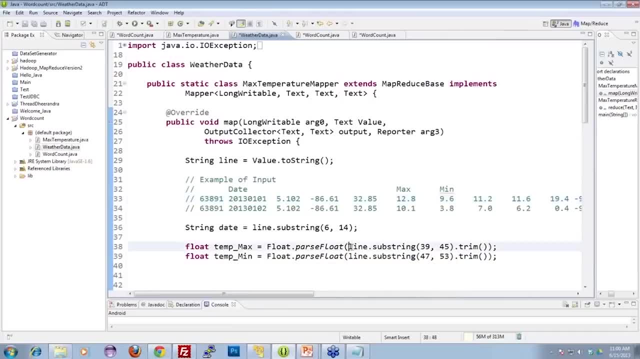 temperature, we store them into float. so what we do is first we do this 39 to 45, with just being a little. why are we doing this, guys? 39 to 45 is not the exact number, any idea. so, yes, yes, Sriram, Sriram has a very good question here. we are able to. 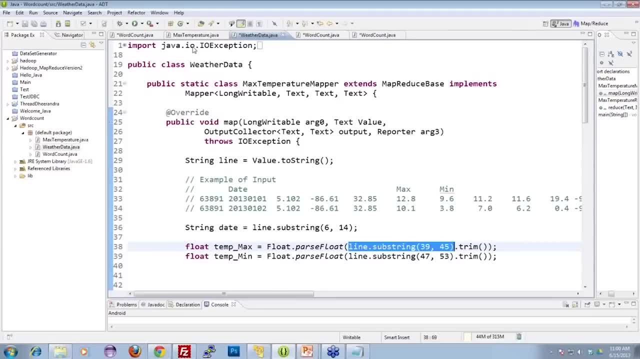 apply substring as we know the form. So most of the times you'll be knowing what file format are we having, right, the data set may be completely may not tell you what this is, but data will be dumped in a specific format so you will always have that Sriram somewhere or the other. you'll be. 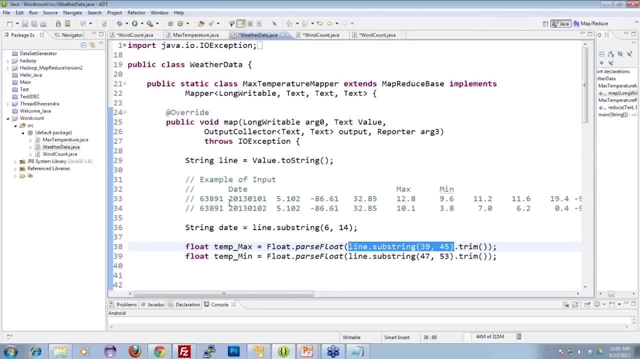 able to figure out what value is what, though it may not be written date here, but you'll be told that, okay, this is delimited by a comma or it is not delimited by anything. it can be completely splitting, right? is that clear, Sriram? 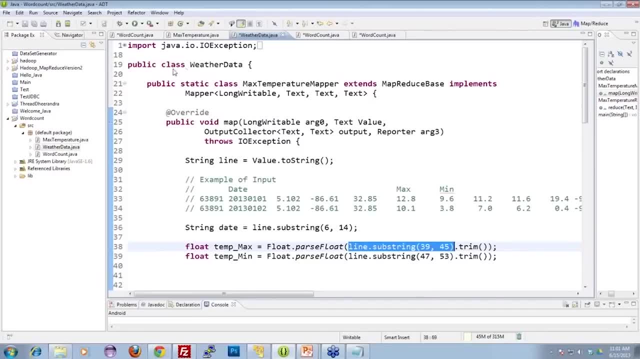 Okay, Well, this is not a structured file as such, right? it is actually unstructured data, right? this is a log file, right? there are other things like: if you have image file, what do we do then? don't worry about that question now. I'll answer that question next time. 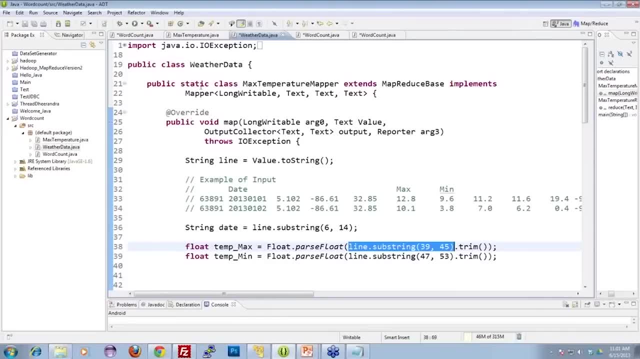 okay, Sriram, for now. okay, Sachi, I'm not. Sachi is asking temperature of the numeric data. then why the output? The parameter has to be set as text. the output of this program I have not yet defined, so 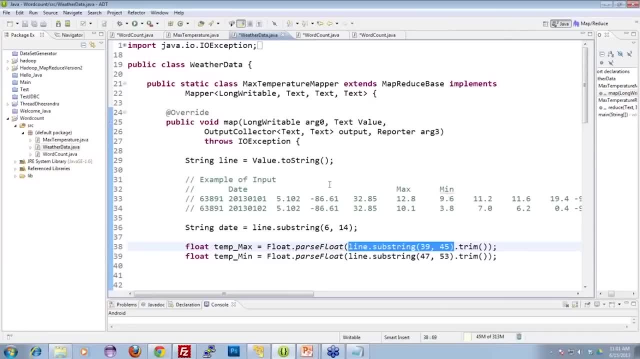 I've not told you what I'm going to dump, right. I'm not going to dump right, so just hold on, okay, yes, so now what we're doing here and the reason why we've taken a range. it is not 39 to 45,, it is 6 values right. why we've taken a range is because sometimes 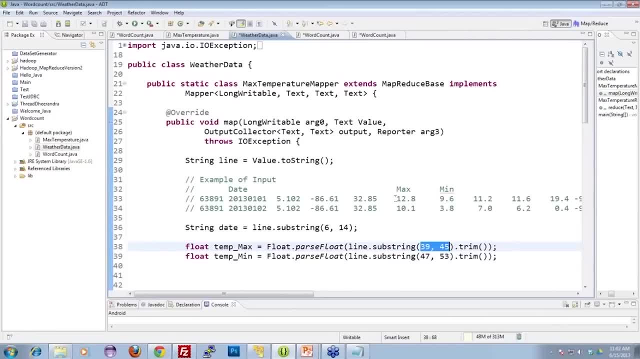 the temperature may be 33,. you can have, say, 99,, 100 also, right. so we want to make sure that we take a range in which it will come right to accommodate for exact values. Exactly, Ravi, thank you very much. right, and Dilip, my friend is telling me just like. 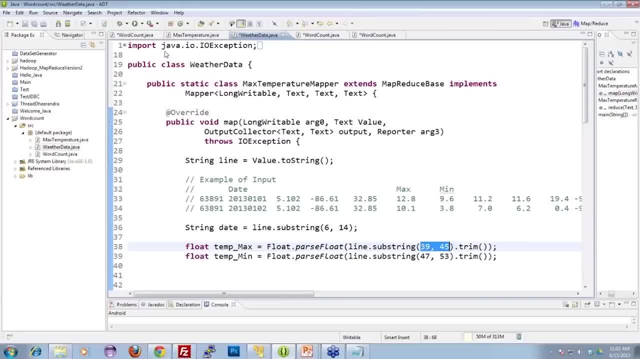 cut command in Linux: exactly exactly Dilip. so in cut command what we do? we take out specific columns from a file which is delimited by some parameter. okay, Dilip will also send us the cut command. I can also show it to you, but right now that's not required, okay. 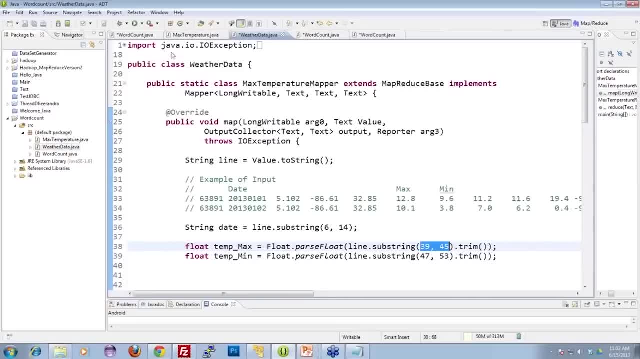 but remember, awk and cut is something Dilip is going to send us. okay, yes, so it will take one line per record to accommodate extra digits. Once we do this and then we do a trim, trim will remove all the spaces out of this and 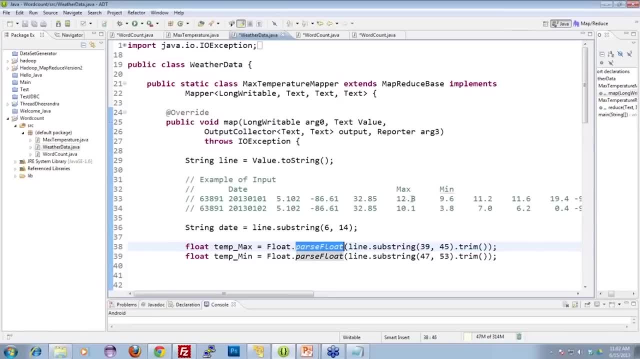 then we make it a float. parse float will make it a float type. it is a text type right now from a string. it will convert it into a float. so you get that temp max here, right? is that clear to everyone, guys? 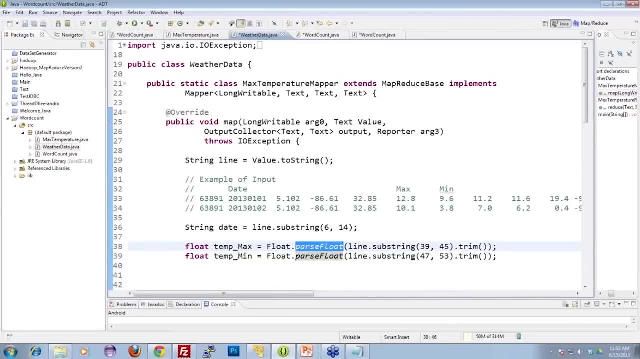 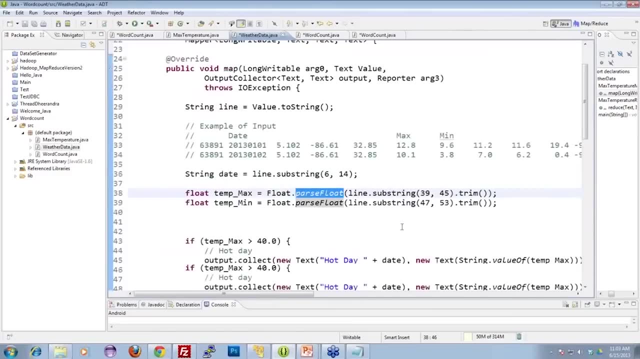 And then, and then we have okay, and then we have a temp min where we'll be trimming it again. we'll get the temp min again. so this is how we get it okay. is that clear to everyone? Now, what I also do here is that I put a condition which says: if the temp max is greater than 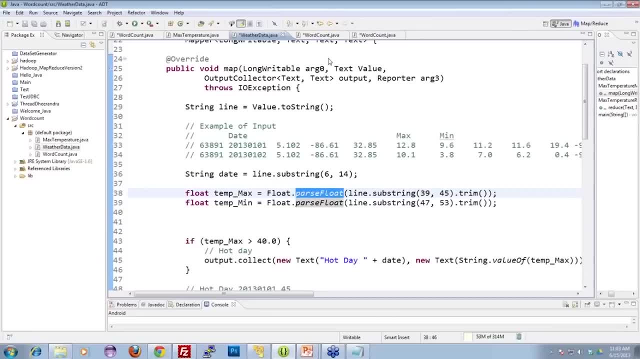 40,. I'll call it a hot day. so now it will be clear whether that my purpose of this was: to declare whether it is a hot day or not. that's why we are using whoever asked me that question, Sachi, probably that temperature is a. why are we using a text type? okay? 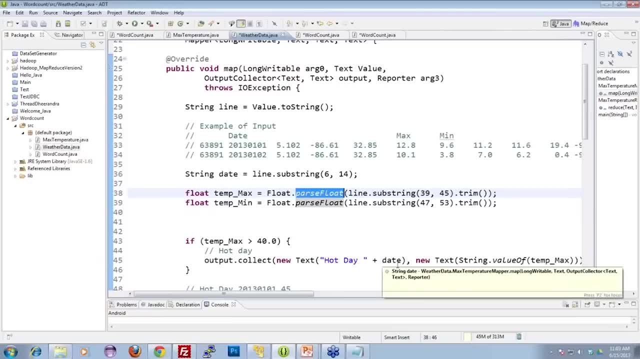 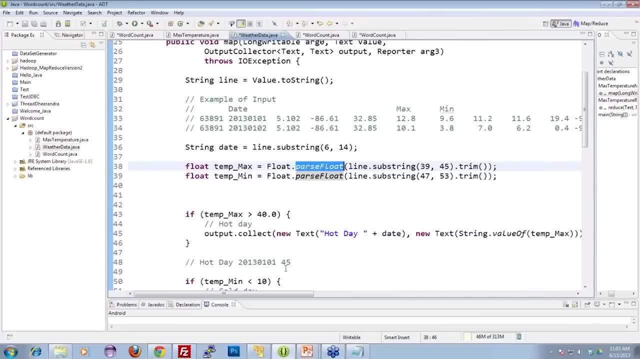 so what we are saying is: output will be a hot day and date okay, and value of: based on the value of this right. if the value is this, it will be writing this. so what are we going to write? We are going to write hot day if it is more than 40,. we are also going to write the date. 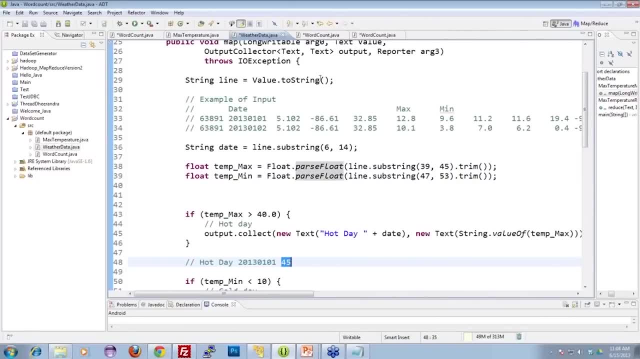 here and we'll also put the temperature out. okay, these are the three things we are going to put here, similarly, for a minimum thing. if it doesn't fall in that, there is no output for that record. is that fine, guys? if the temperature is below 40 and between 10 and. 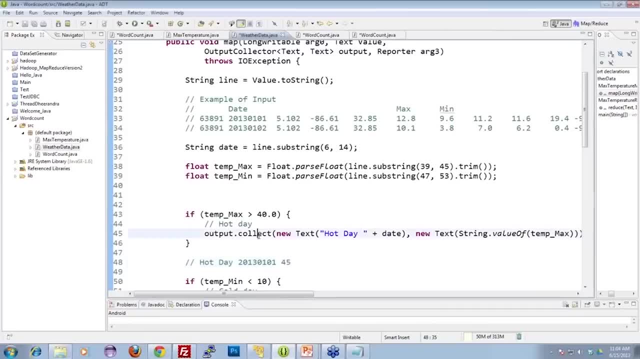 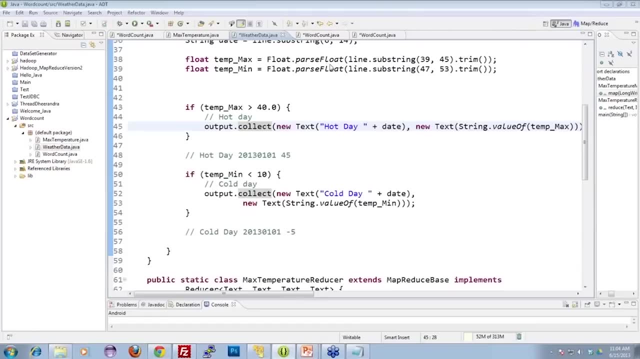 40,. there is no output in this program for that. okay, now, if the temperature is less than 10. Then we will write cold day and this right, is that clear to everyone, guys? so this is the output here. okay, quickly. yes, can I get quickly get a round of smileys? we are. 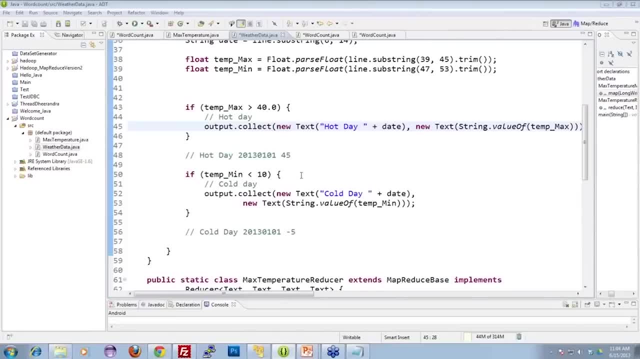 almost there, and then I will also give you assignment on this. everyone is clear. no one has a confusion here. even the people who did not know Java are able to figure that out for each record. we are doing that, Avinash up. 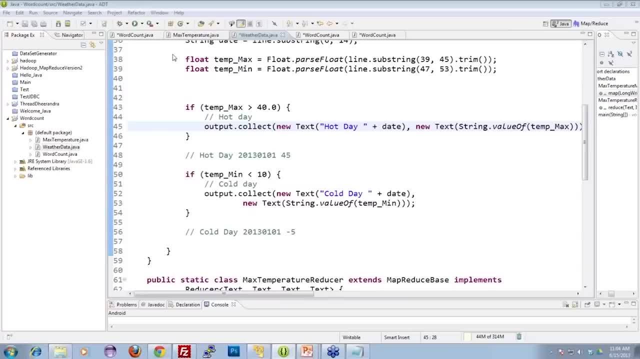 Yes, we will be sending all these. see, all the code which is there will be given to you. okay, all the code will be given to you. there are many more other programs which are, which lie in your LMS. I'll show you them as well. okay, so don't worry about whether I'll get. 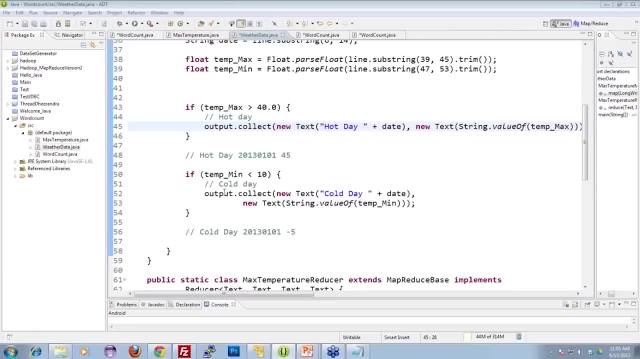 the code, you don't have to note down anything. So Tushar is saying: I could understand, even if I don't know Java. very nice, that was the purpose of this small exercise. this example is clear, but I'm not clear will be so structured. 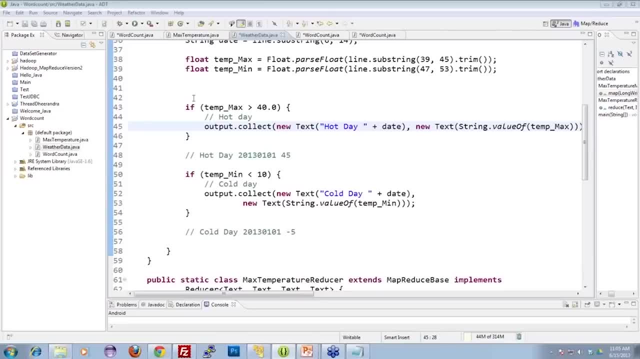 that we know the exact location. Okay, So, Vamsi, don't worry, I'll show you more examples on how to do that. okay, now this is this is this data is a real data. this is not something BRB or something which you 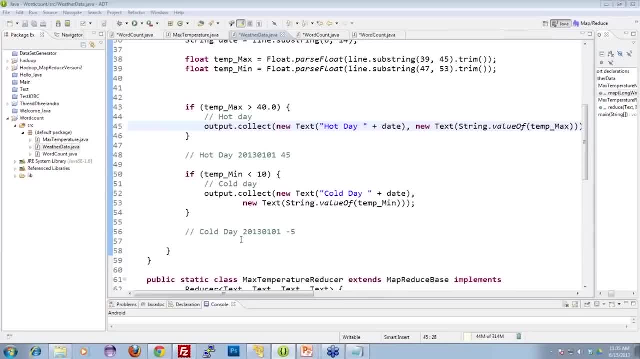 have created. right, we got that data from a real location. right, you remember that we got it from that particular website. Vamsi, you remember that usually you will be dumping that data in some format. we will be sending everything to you, don't worry about sample. 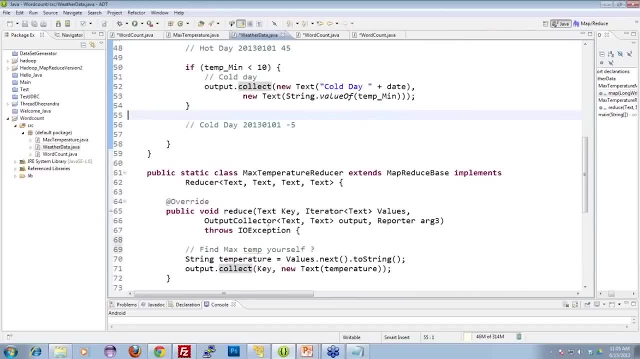 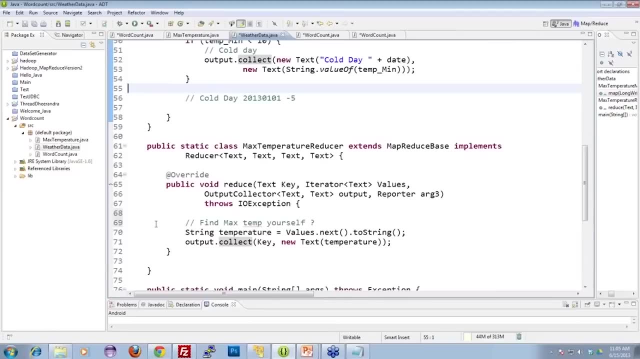 code and everything okay. now let's go to the max temperature reducer. this is the reduced program. Now, in this reduced program, I am not doing anything. I am just dumping the values, okay, what I want you to do. so what this means is that Fn, which I had defined, there is no. 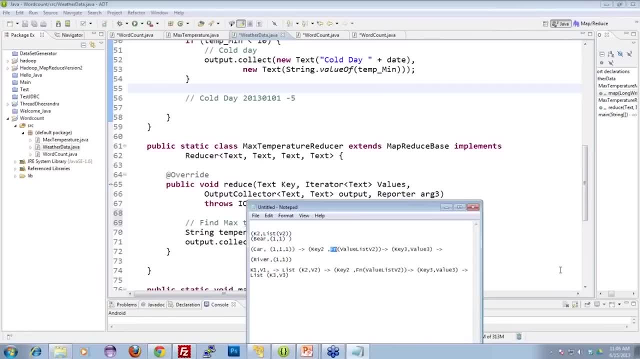 Fn here? right, there is no Fn here. I am just dumping these values. okay, I am not doing any function here, so it will straight away dump this. there is nothing if I have to just dump whether this is hot or cold. I don't need any function here, okay. but 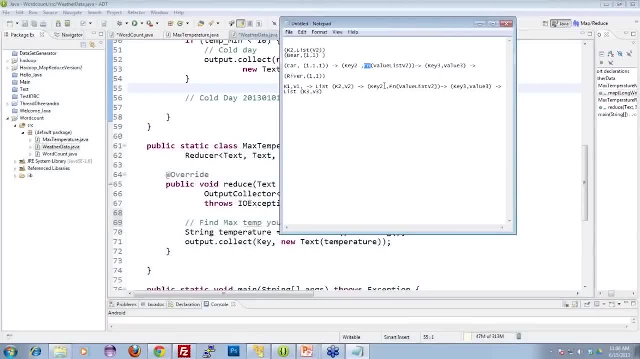 if I had to say: do something like this, where I have to say which is the maximum temperature in a particular year or in this complete thing, which is the maximum temperature, okay, then I have to write a function- max here. so then I have to implement that and that. 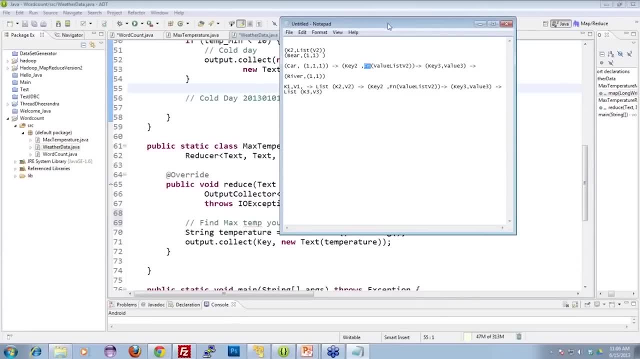 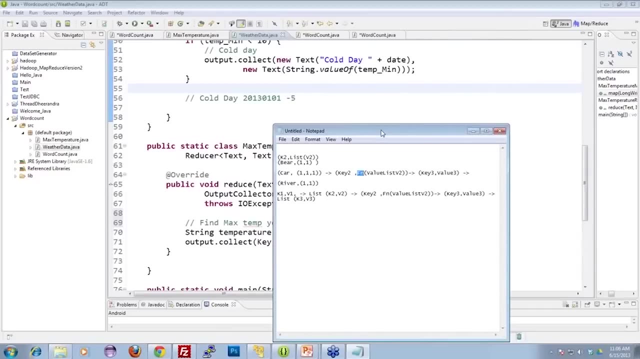 is your homework as well. on this data set, you have to find out which are the maximum. what are the maximum temperatures in particular year? okay, is that clear to everyone? how will you do that? very simple, is everyone clear on that? this homework? can I get a? 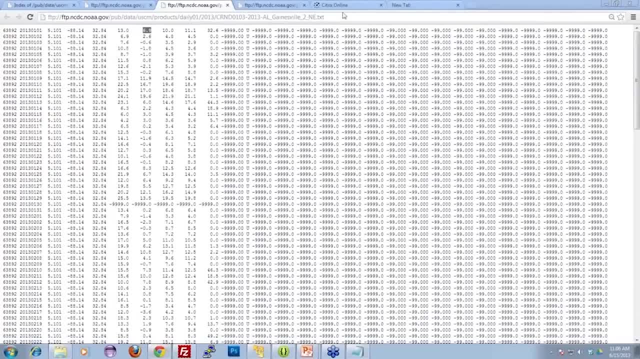 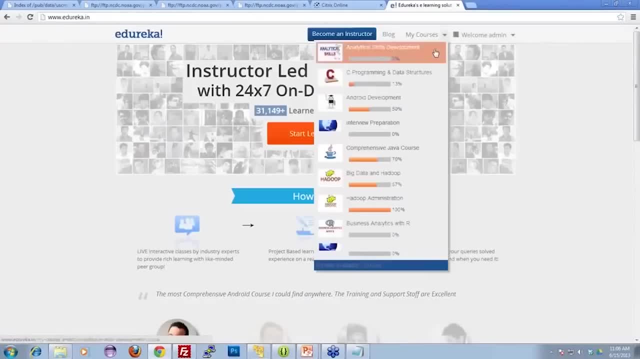 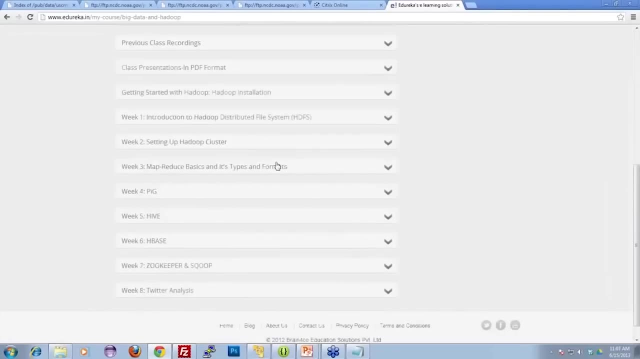 quick, yes, great, very nice. So this is the data set I want. yeah, so let me show you the LMS learning management system, show you where all these things are kept. okay, now everyone is asking questions that where will I find this data recording? everything is here, so there is this word. 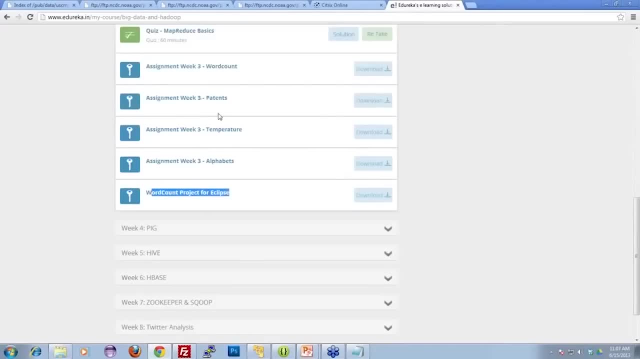 count program for Eclipse. there is the project. okay, there is a temperature thing also here. there is a slightly different thing, but very, very similar. we will be sending you this data set also. So all these things are there. So all these things are there. 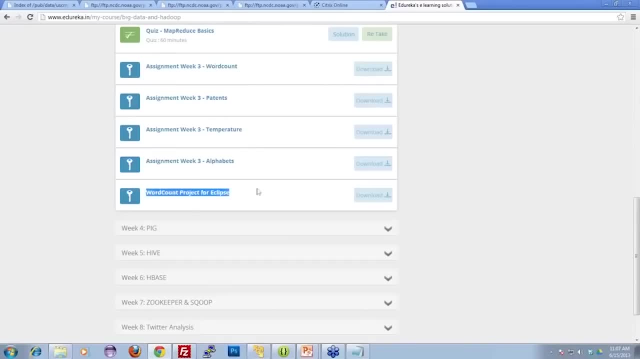 So all these assignments you have to do. okay, this is the program which we saw earlier, right, and you can quickly download it like this. So when you you have to load this, this project in Eclipse, when you download Eclipse, so the 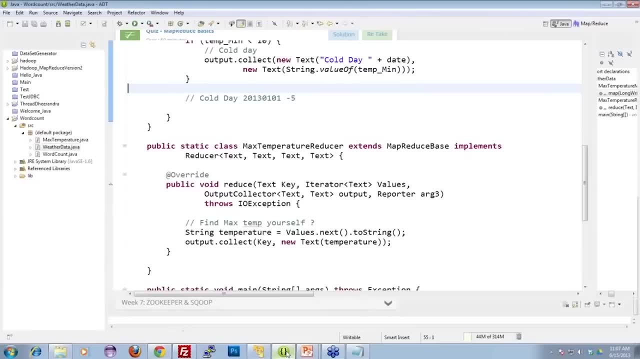 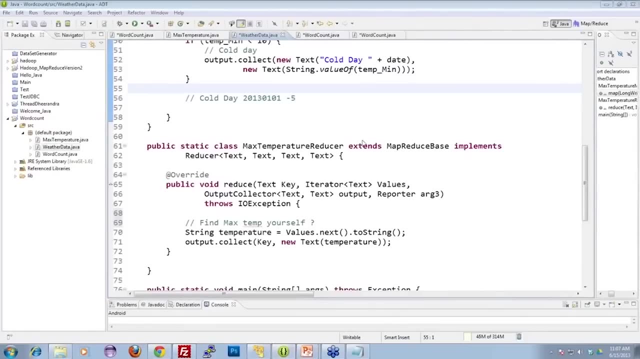 complete environment will be created like this. okay, is that clear to everyone? guys, And I also want you guys to do this on your own. okay, I will monitor how much support you are taking from the support team. I am going to monitor that, okay, so now, now that 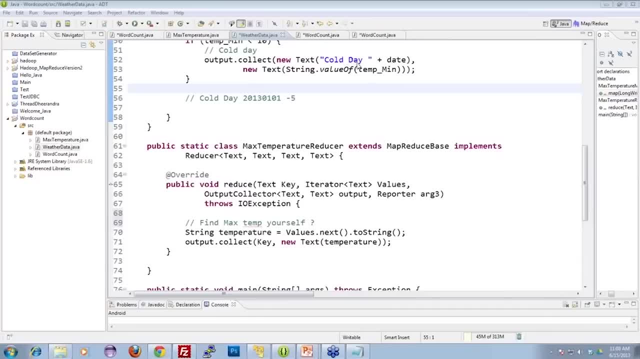 we are here, right? okay, so you have to do a lot of these things on your own? okay, it is very simple. I am sure you will be able to do it. Next step: what we are going to do is we are going to create. how does this? yes, so Vamsi. 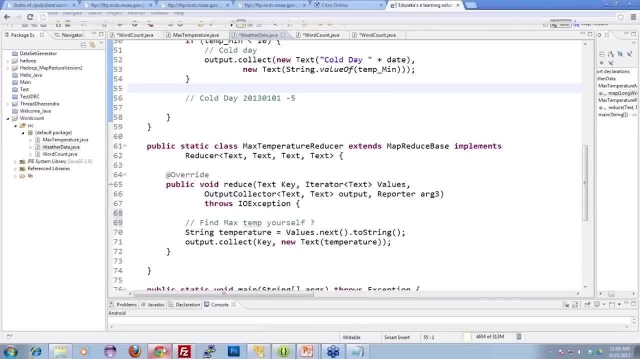 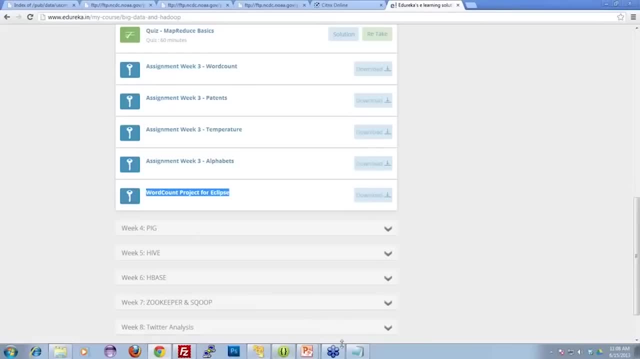 this is the thing, just thing, which I just showed you on the LMS. if you download this part, it will show you how to set up MapReduce on Eclipse. this guy is going to do this. okay, Vamsi, great. so next let us get back to the class once again and see what we are. 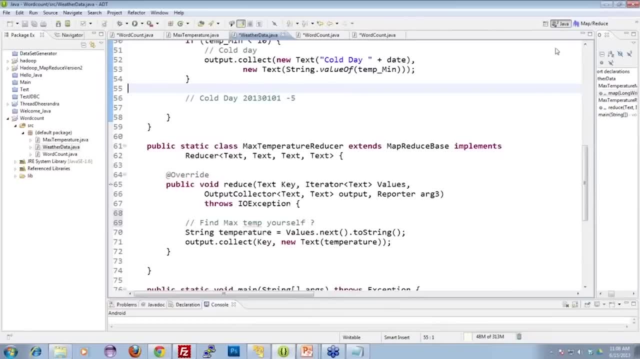 going to do next. okay now. the next thing is, now that you have created this program, we will be creating a Java archive of it and we will be running it on our Hadoop. okay, that is the next step we are going to do in this class. okay, isn't it exciting. now we 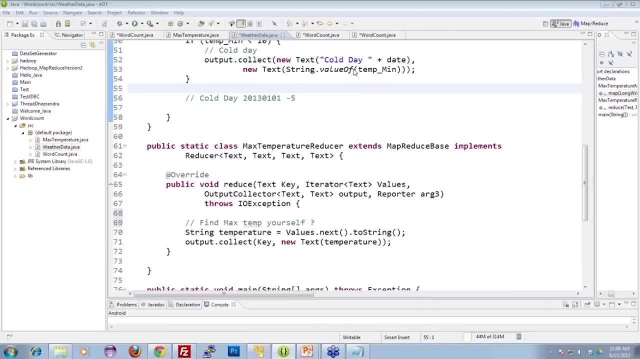 are going to actually run this program on Hadoop On our cluster, on that dataset which we had. okay, so the complete process will be completed and then we will go to the next things. so let us go. let us go to our cluster. now see, 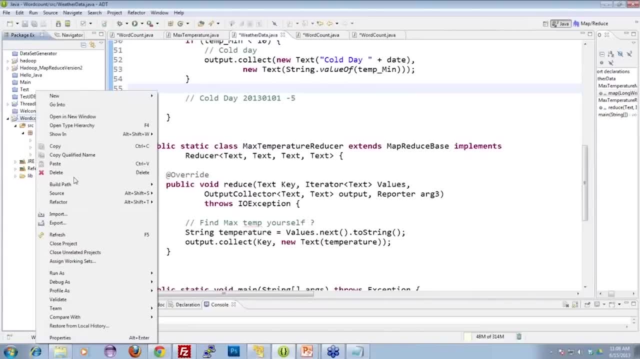 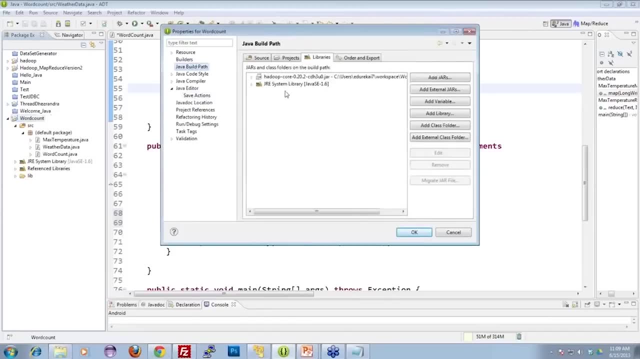 the quickly look at the process of creating a jar. I will also be sending you, I will also be sending you a quick video which will show you how to create a jar out of it. yes, Vamsi, thank you very much. I am getting a little late for the doctor's appointment. 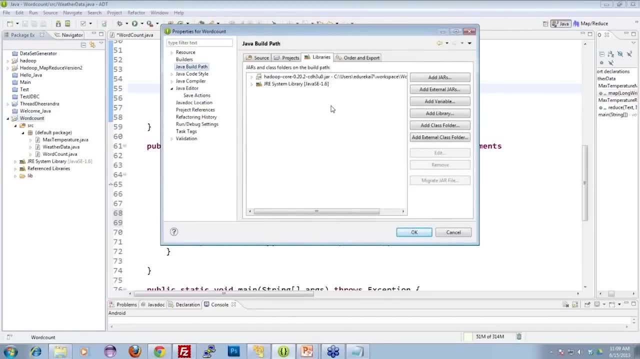 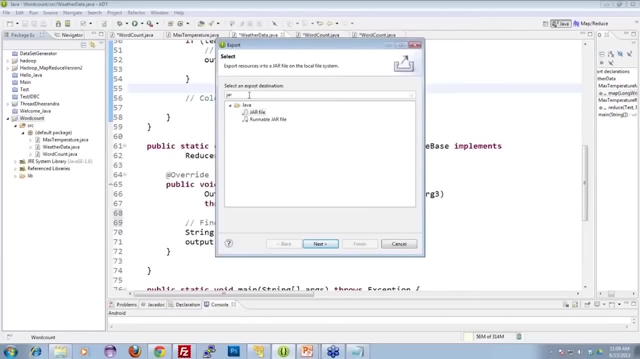 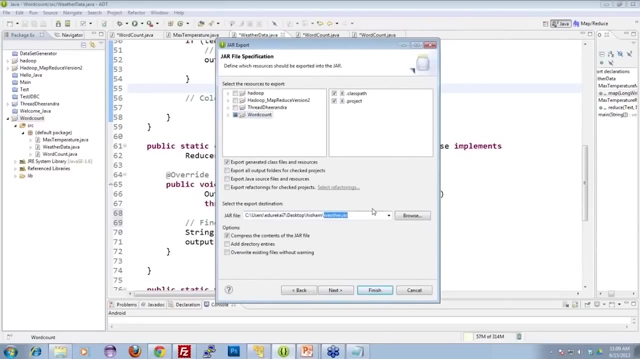 thank you very much for your concern. I will just take five more minutes and then after that I will take a break. okay, So what I am showing you here? look at this clearly: we are creating a jar file out of this. okay, so this is a jar file. okay, I will also be showing you. so this is the jar. 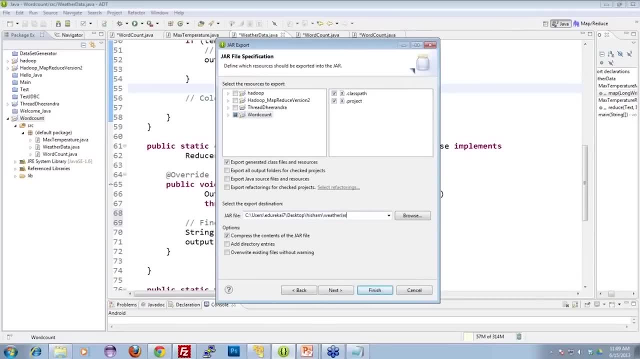 in this path. we are creating it. I will also be sending a quick video of how to create a jar file and a document as well, so don't have to worry too much. I am just showing you how it is done here. Now let us look at which is the main class of this jar file. right? so we are looking. 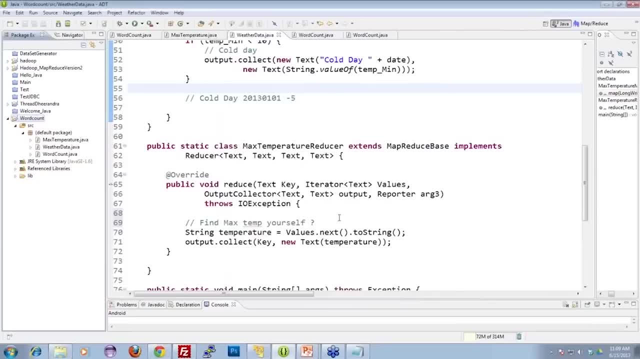 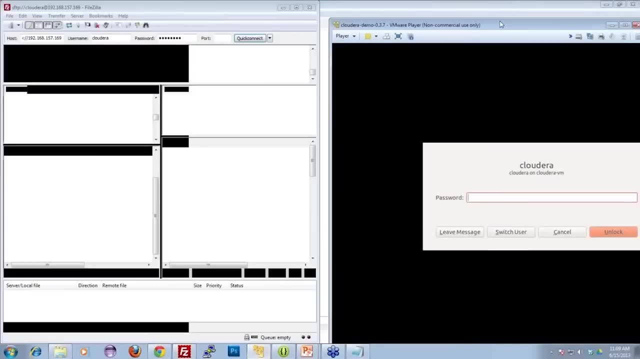 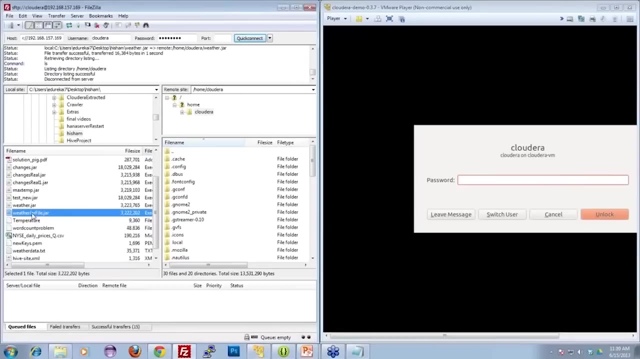 at whether data. is this clear to everyone quickly? yes, thank you, Vamsi. thank you very much for your concern. the old man will give you a lot of okay. yes, so let us look at this. let us look at this one. and this is the jar which is created. now what are we? 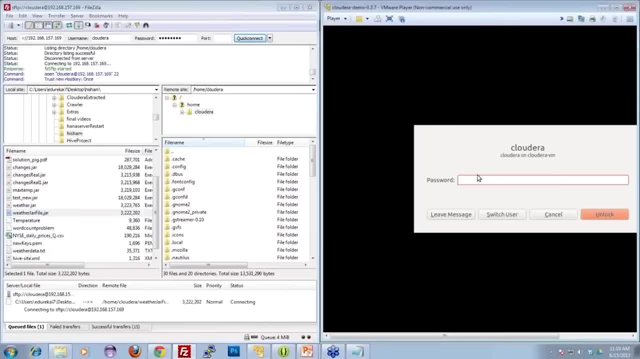 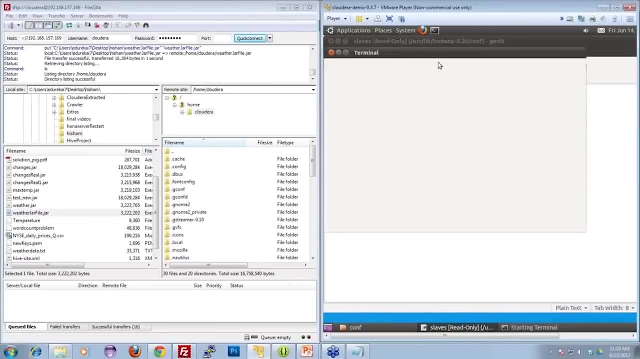 doing here. we are FTPing this into our cluster. so this is the file zilla thing. we have put it from here into our cluster Right and in our cluster we will see that we are able to see this or not. so we got. 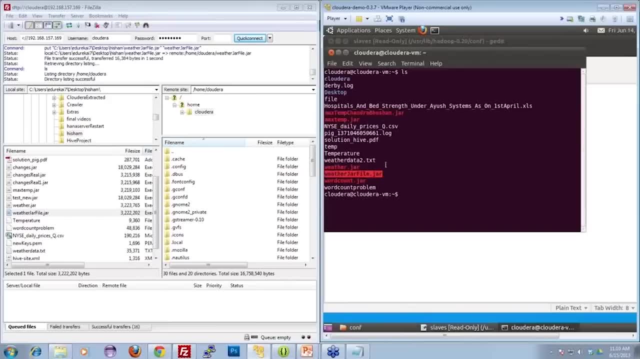 it here. is this cool guys? is this clear to everyone what we did? we created a jar file, exported it from our system into the cluster and this is where we got it. and this is the jar file. this is the data set. okay, so the data set is where the data tool now. 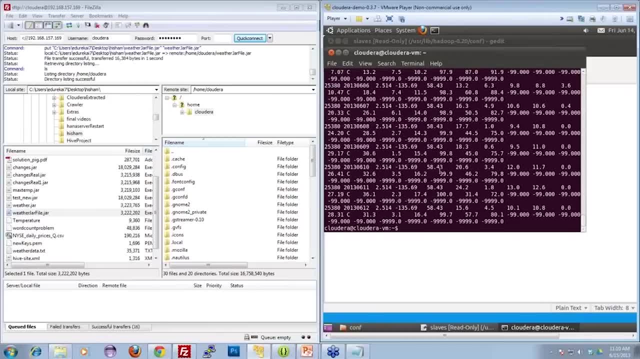 let us look at the data set quickly. So this is the data set which we are looking at. these are the dates and the temperatures here. okay, now we are going to do a Hadoop. DFS, you remember this? we showed it last. 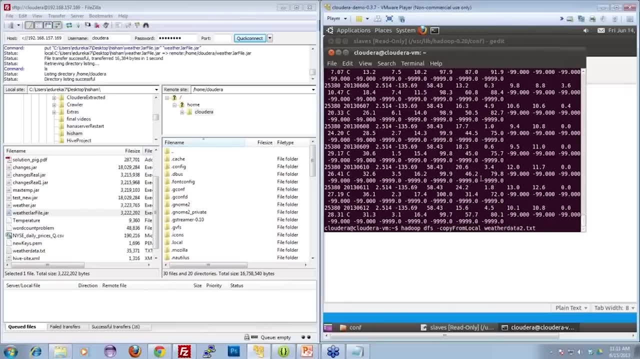 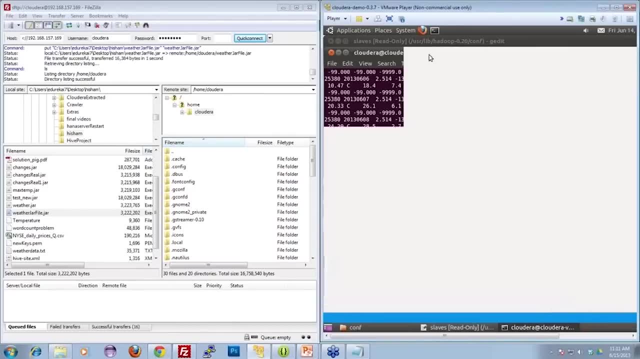 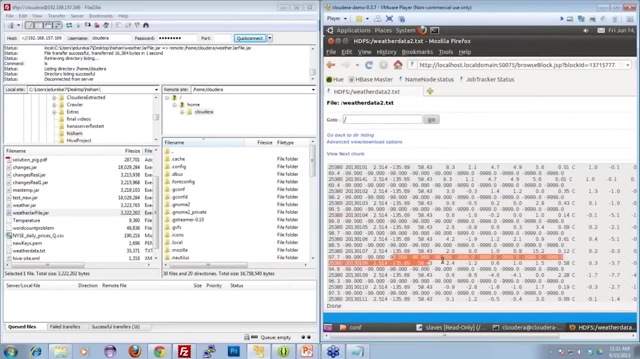 time. copy from local. we will copy everything into DFS here. right, is this command. you remember this command. let us look at this in a file system now. This is our HDFS file system. we got this file here right quickly. keep on writing. 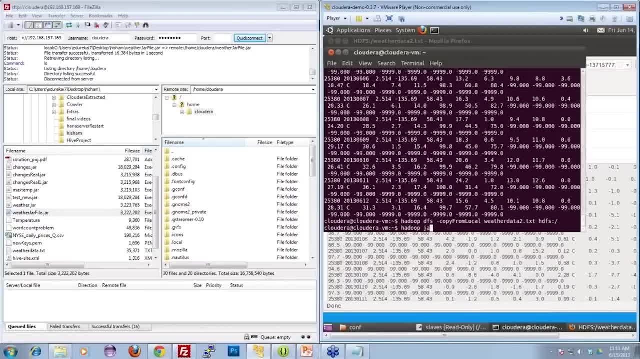 yes, guys, if there is some confusion, just keep on, keep telling me. So what we did? we copied this jar into our. we copied the text with the input file into our HDFS. okay, now we are going to copy the. now we are going to do this. yeah, so now. 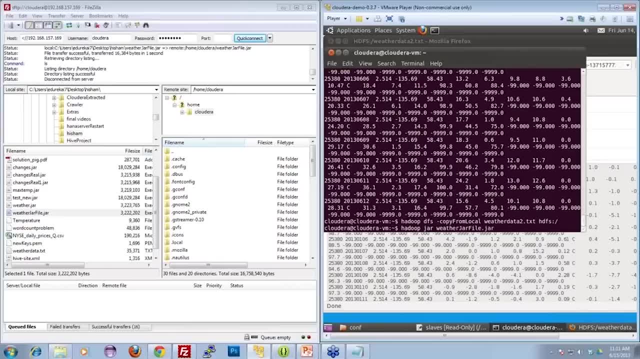 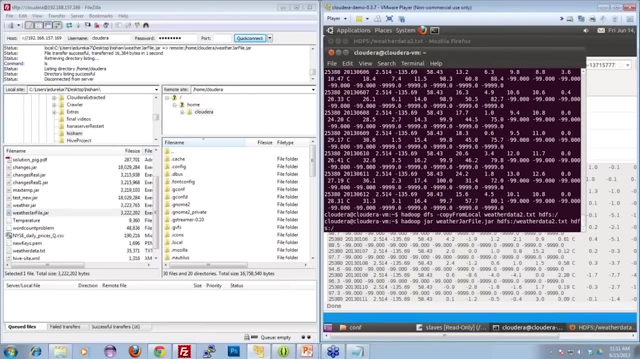 we are going to run that program. What was the program? Hadoop jar? Okay, So now what are the inputs and outputs there? arg0 and arg1, input file path and the output file path. right, you remember this. now these will be the arg0 and arg1 in our program, right? 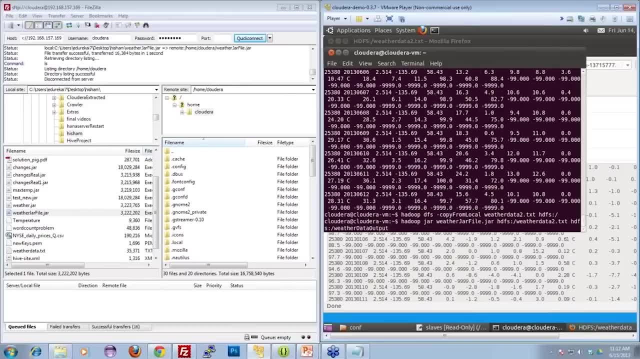 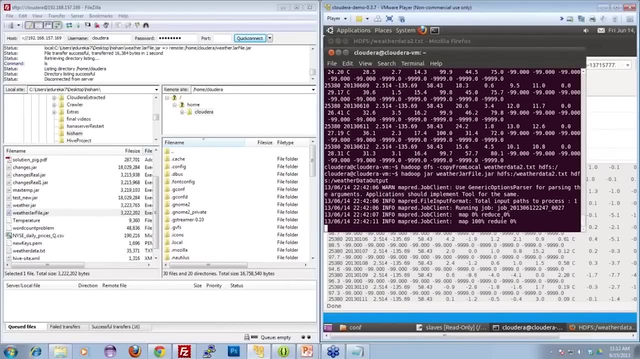 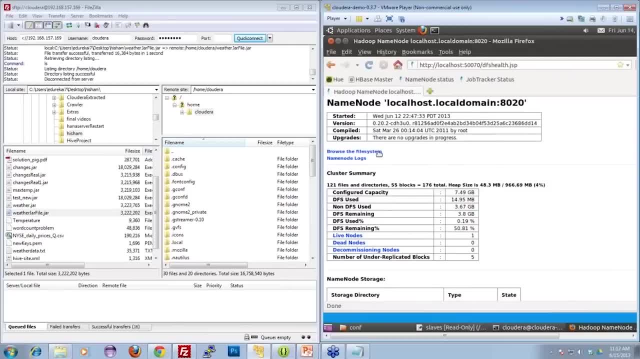 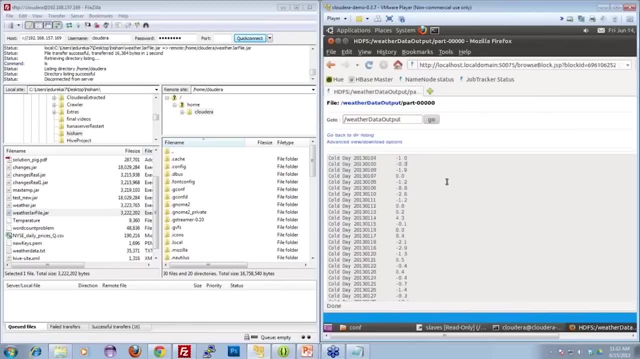 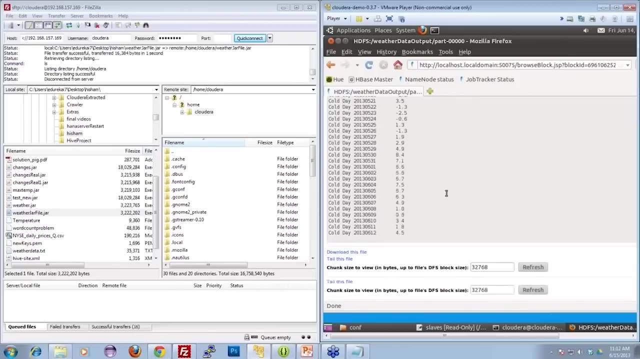 Now let us look at this. what have we got? we have got one. okay, great. so it has told me these are the cold days. okay, it did not find any hot day because probably the number which you have said is a large one, it would find only cold days, okay. 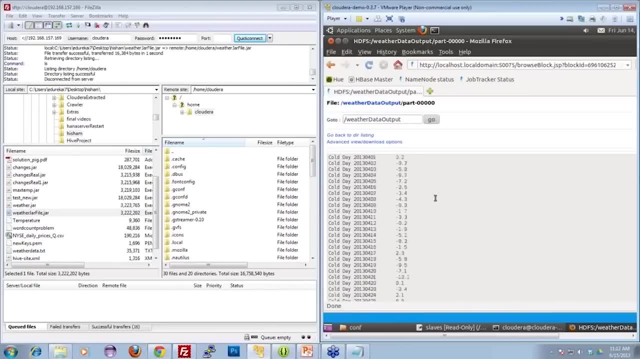 Okay, it would find only cold days. okay, that was the data set on which we had that. so this is how a sample program runs on Hadoop. is this clear guys, everyone, the steps, great, wow. so now I know some of the things will not. 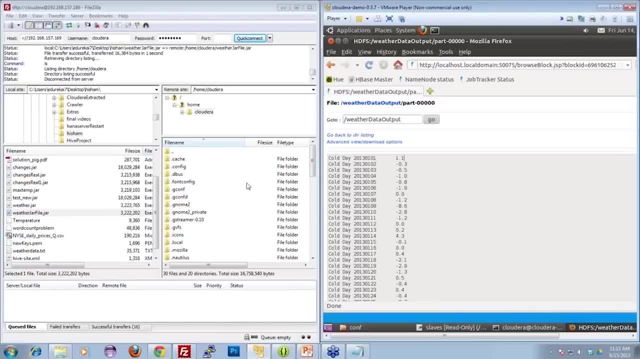 be very clear, Sachi. I will take your question just a minute, okay? Rajat is saying: it is not clear. Rajat, please ask me a question and what I will do is, for today, we will stop here and we will go into more things. where is the class name? okay? 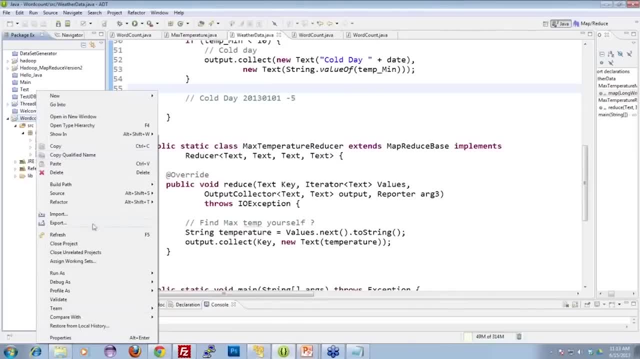 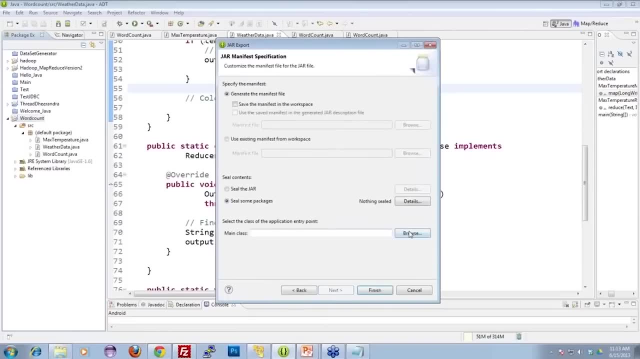 show him the class name from the Hadoop jar. okay, good, so last time we saw that. so here is the no, no, don't worry. don't worry, I will show you the class name. so this is the class name here. now let's look in the jar file. last time, 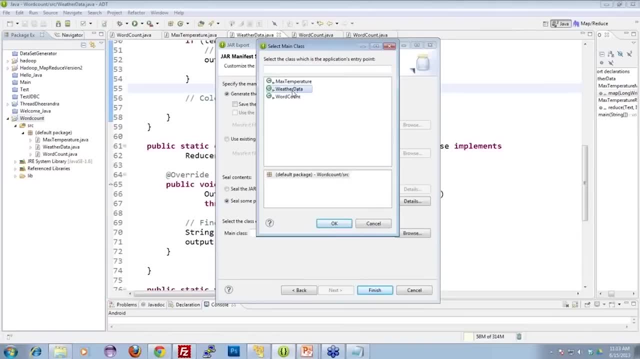 we looked at all the classes which are there in the jar file. okay, this is the class name here. okay, just okay, now there is a way to do this. okay, so let's look at the class name here. okay, so let's look at the. 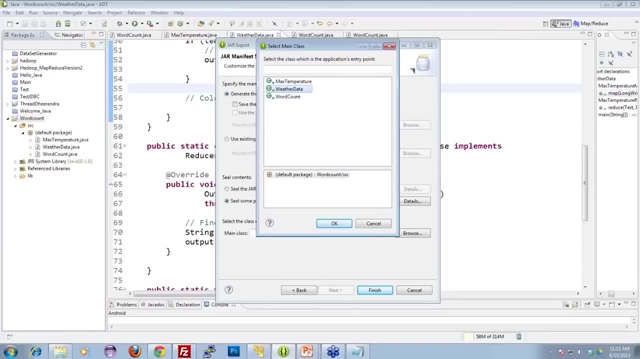 say, to show that, show you that, I will show you later. okay, just this is the class name which we used from that jar. since the jar had only one class, it ran. the default thing is that: clear Rajat. yeah, yeah, so. 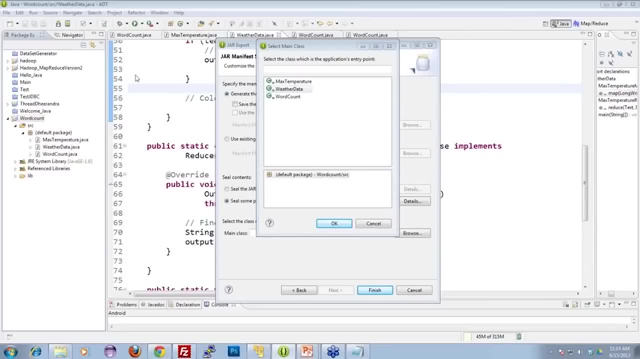 the bunker. you will get all these things easily. okay, don't worry, you can get touch base with Rajat, he will give you all this. okay, Rajat, is it clear? yeah, yeah, right, Great, Okay, So everyone is clear with what you have just done. 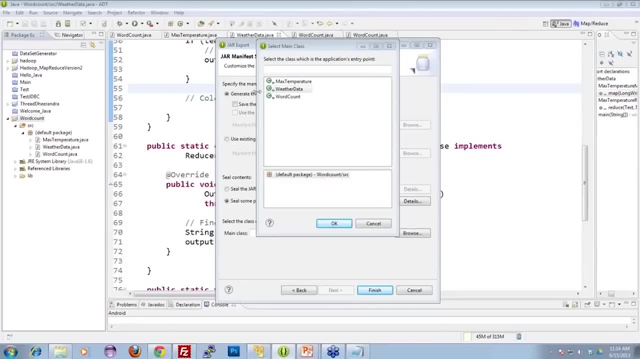 Let me quickly tell you what you have just done before I rush out- And I am really sorry, guys, I had to leave today a little early. Next time I will compensate for this one. So what we did today was, we understood quickly, keep writing yes or no. 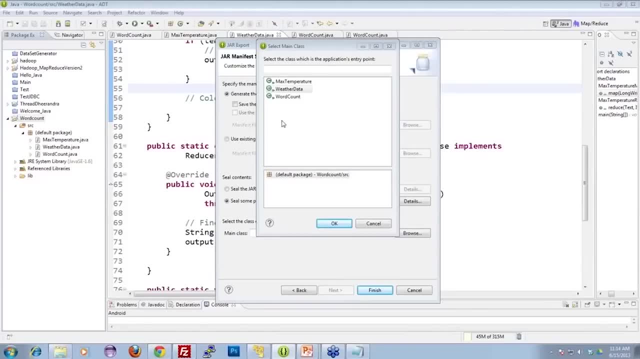 I am not taking a quiz also today. Next time I will take a quiz on all these things So quickly. we saw where the applications of a MapReduce kind of program will be required. We looked at a large data set. Okay, You were supposed to ask. thank you, Rahul. thank you for that question. 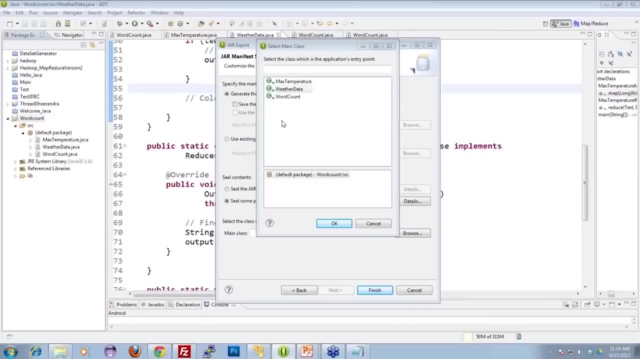 I will ask that question next time You remind me that. next time, Okay, I will show you a larger data set and I will show you what to do. I will also send an email on this today evening to everyone, Okay. So what have we done today? 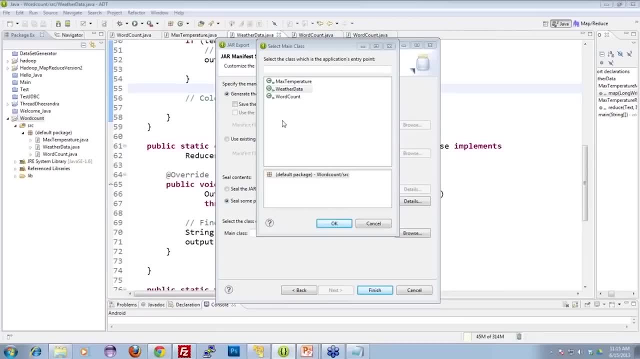 We have quickly looked at what all is. we started with a large data set. We saw a weather data set, Then we looked at what are the traditional ways of doing it. Our friends have promised us that they will send us all. Okay, So who are our friends? Can they quickly send me a smiley? 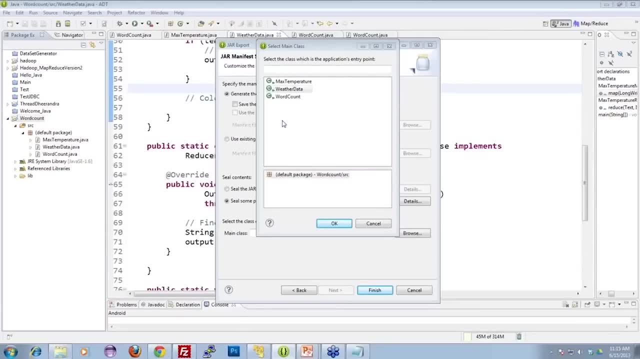 You are going to send me the awk command on this data set to do this particular operation, which I have done through Hadoop MapReduce. Dilip has given me a smiley. Ravi is hiding behind somewhere. Ravi is taking over to me. 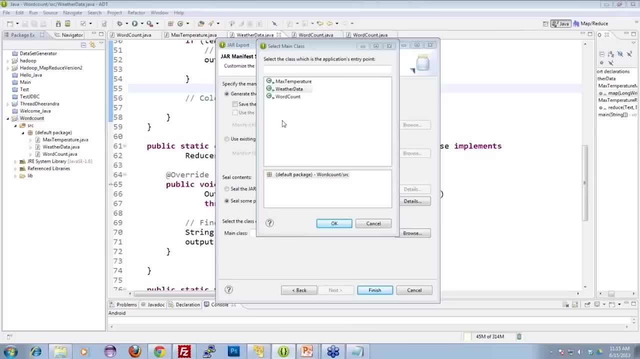 Ravi, you have to send me that awk command here. Okay, Avinash is also going to send me that. Okay, So same thing has to be done in awk. Okay, And yes, Vinay, we will have a MapReduce class only next Saturday. 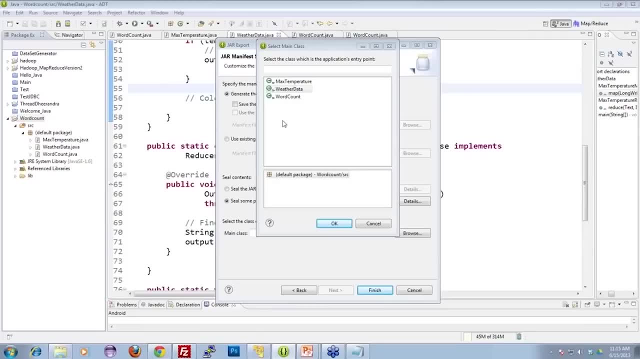 Right, So we will extend this further. I will tell you what I am going to cover there. Okay, Now, some of you guys were also supposed to write a blog last time, Right? So, okay, No problem, No problem, Ravi. No problem, Ravi at all. 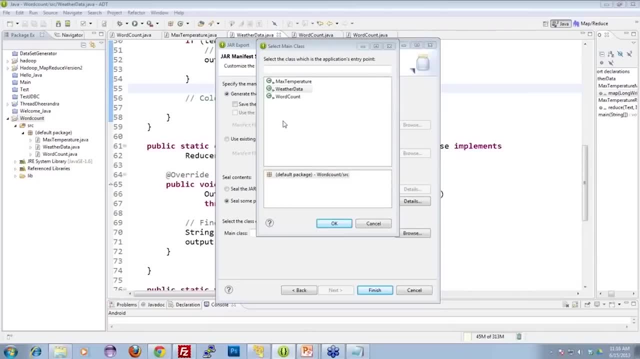 Okay, So yeah, So we will be integrating a forum also. Thank you, Thank you. Thank you, Ravi. Thank you very much. So Ravi is telling me I will show for sure This blog thing. Okay, Thank you, Ravi. 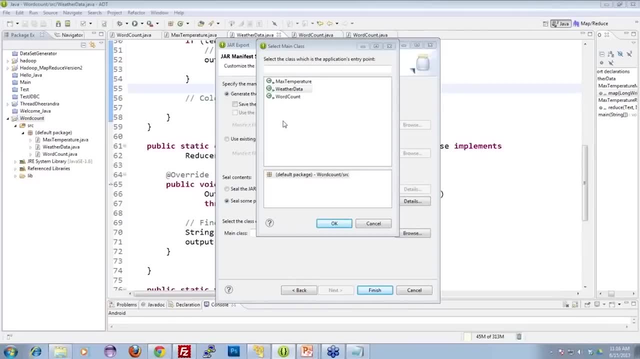 So now what I want you guys to do is see one exercise, if you don't mind, will be to write a blog on this class itself. whatever you learned here Right, Step by step, you can tell us. So simple thing would be. take a quick data set, use awk to do this traditionally.